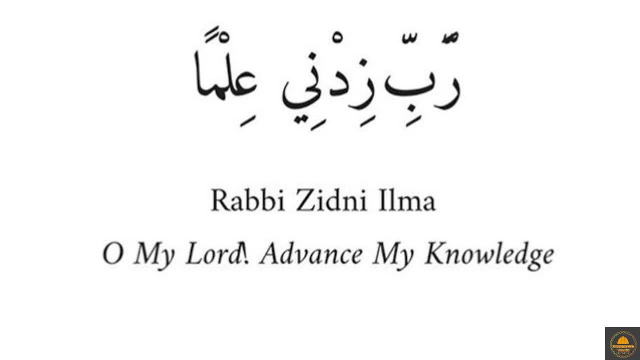 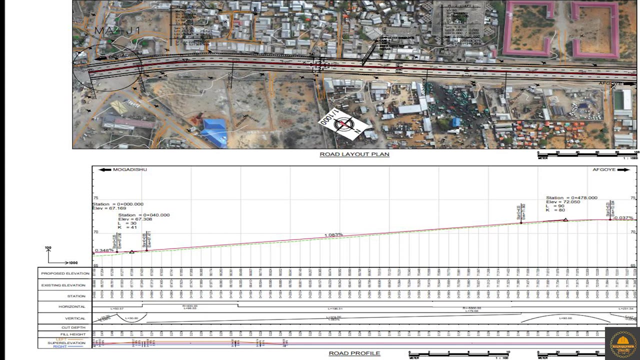 assalamu alaikum, dear friends, welcome back to cyber designing and civil 3d video series by murad farooq. dear friends, today, video tutorial, i will explain with very details how to design a road. and this video i am going to explain each and everything with very details. 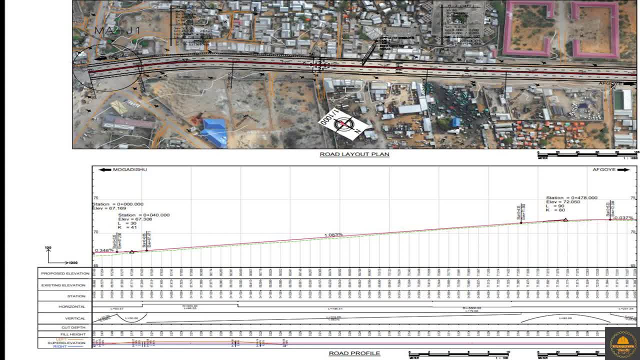 these video tutorials maybe take a time, maybe up to one house, but this video will help you to do and learn from only one video. you don't need to go to one to another and another to other. so in this video you can see the picture on the display. we will explain alignment- how to draw alignment surface. 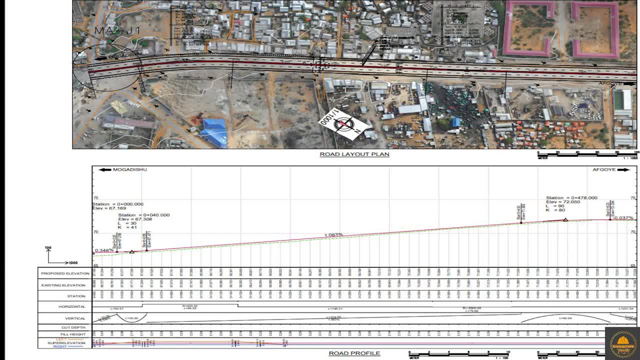 how to import the points, drawing settings, and also then we try alignment, road corridor, road surface, sample line. then in this video we will explain regarding the profile, vertical profile, and in vertical profile i will show how to draw and then again how to create a design profile and you can. 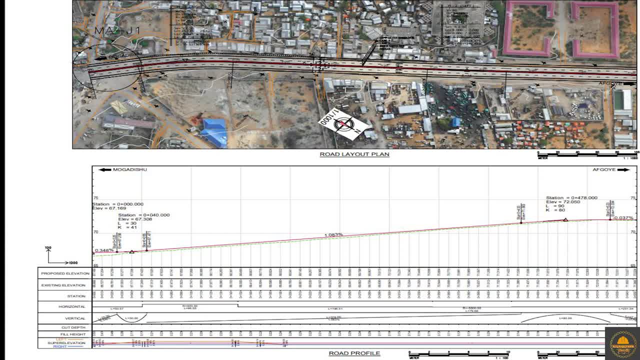 also see the profile bands. we will be explain how to set the data bands and how to create new data bands and also i will show the design levels and propose ground, proposed design levels and ground levels, how to change and how to make, cut and fill difference between them. so if you watch this video, 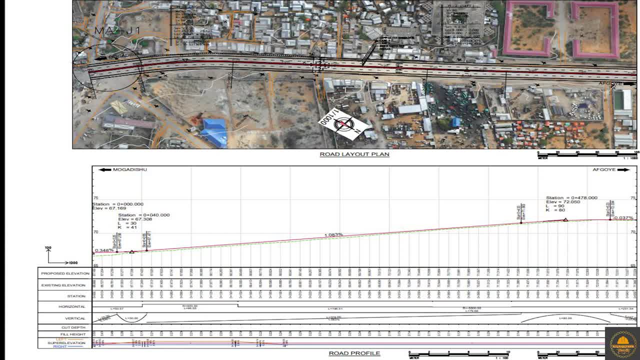 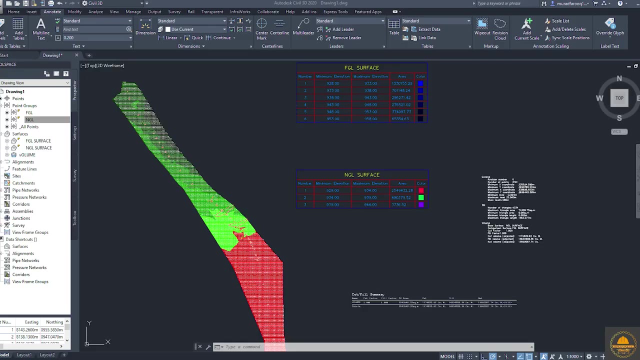 from start to end one or two times. then you can able to draw a simple road design for any client or for any freelance market or for your company. you can do it very easily. my suggestion is that watch this video one to two times, then you can able to draw this. you can see the some highlights. 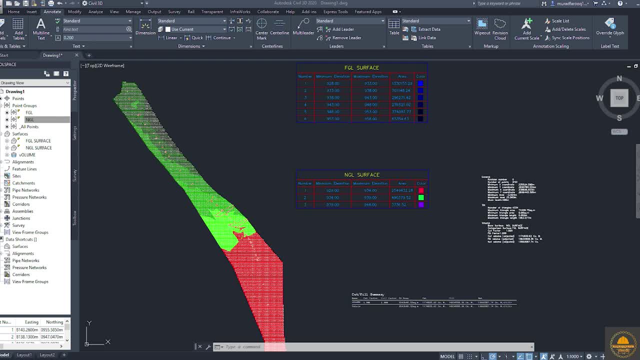 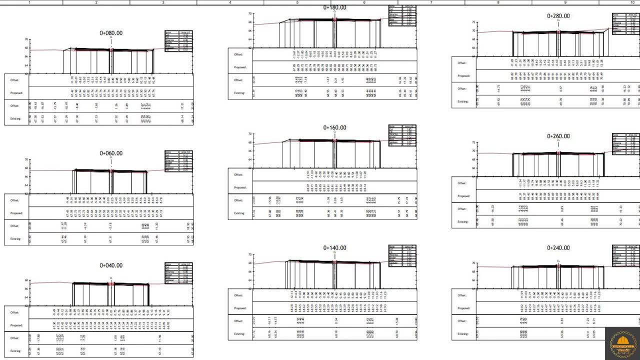 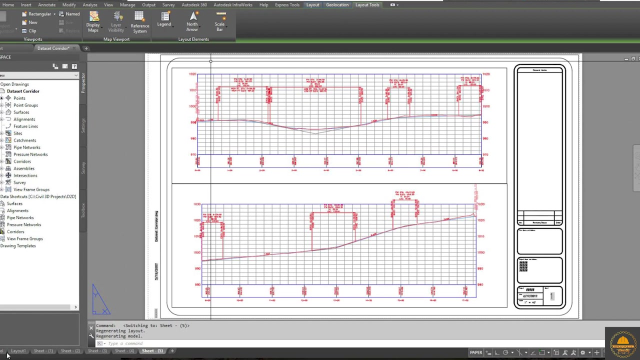 picture. from the video you can see the cross section. i will show how to draw the cross section for each change and i will show this very detail. and in the last of video i will show how to create plan production, how to create sheets from your design and profile. please must watch, like and subscribe. 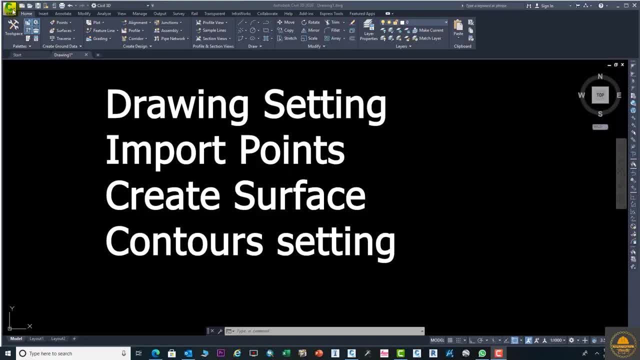 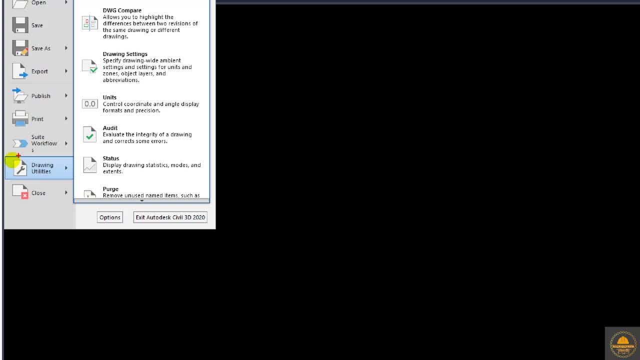 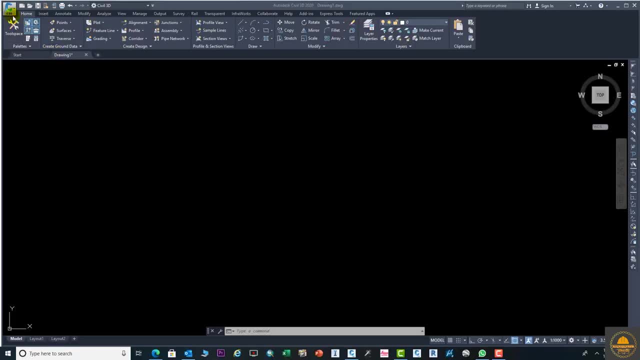 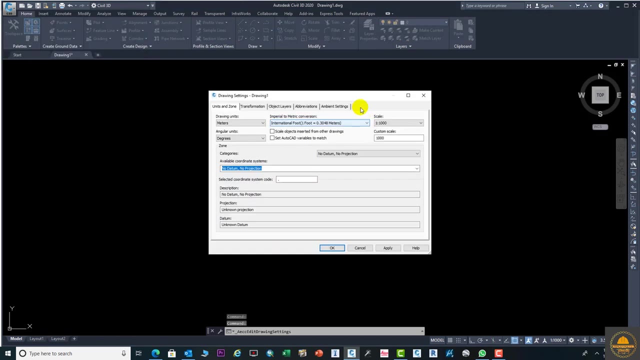 okay, let's start. dear friends, we need to go to drawing utilities from here. we need to select our drawing setting. we need to change our drawing setting according to our coordinate system. go to this option and select drawing setting from here. just i want to zoom this one. we need to select from here the unit. 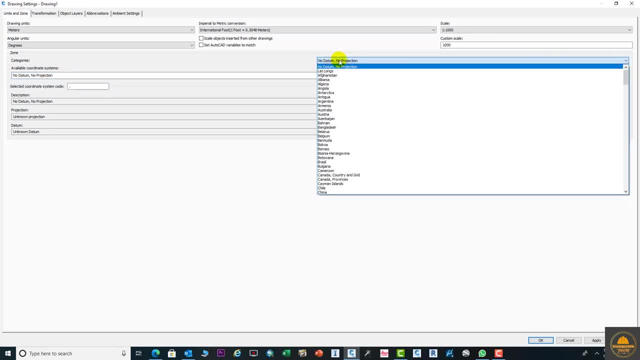 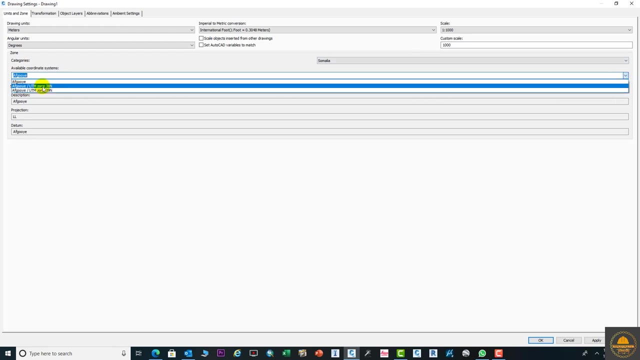 and from here we need to select our datum or projection country. you can select in which country you are working. okay, select the country and from here you need to select coordinate system, your zone, utm, adding one zone in where you're working. apply and okay, now your drawing setting is changed. we need to change our drawing setting. 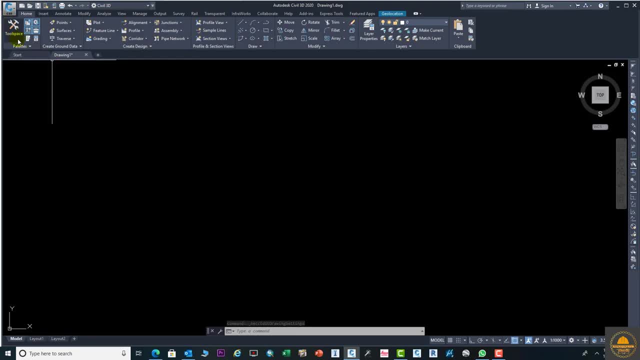 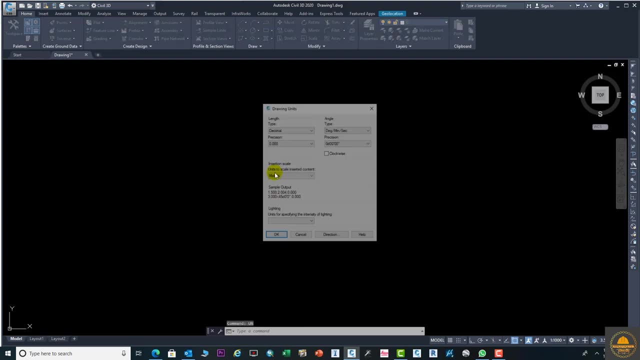 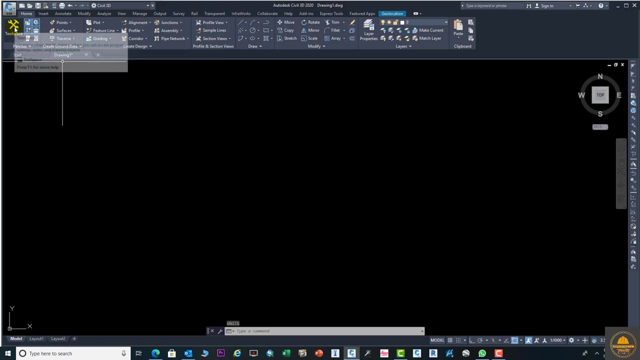 you can start your work. first of all, we will check our unit. just press un and select your unit. unit is definitely good because we already corrected this is normal drawing setting. select from here your unit. okay, let's okay. and now, if your tools is off, you can turn on from this option. 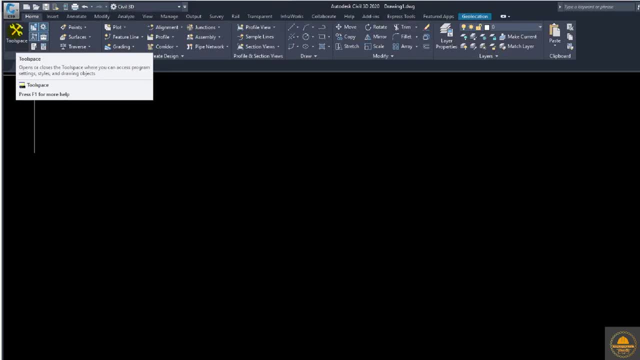 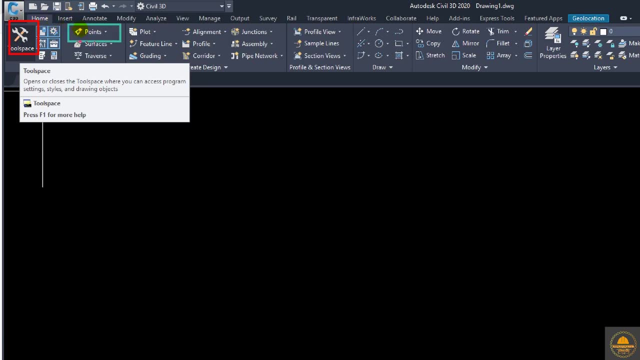 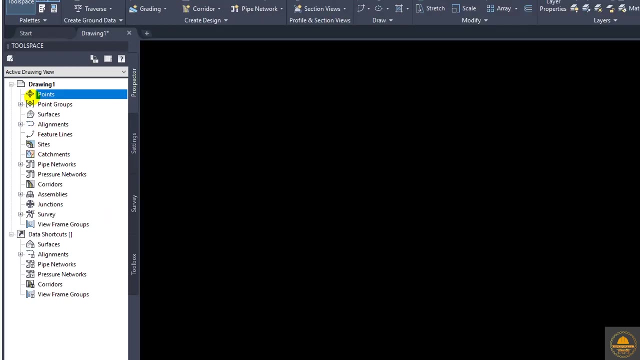 just select on this. you can turn on from this, this one, and from here you can import your points from this option. and also you can import from your tools. just you can see the points option. if you right click on this one, then you're able to see. 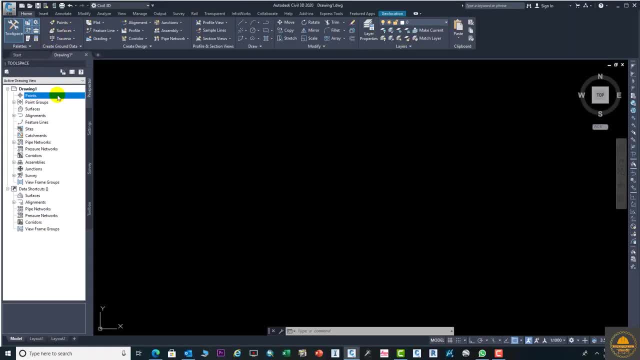 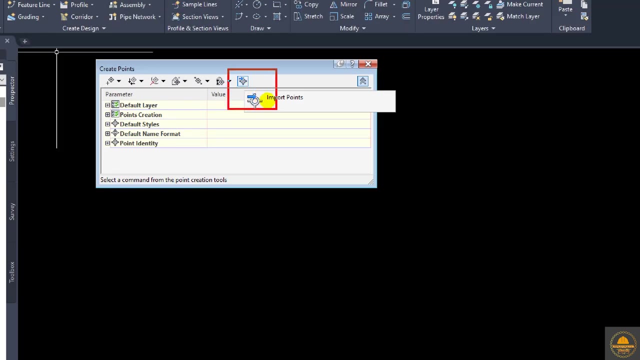 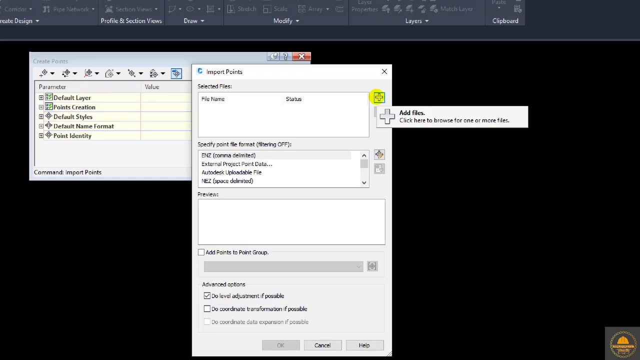 create. from there you can create your points. see this one, okay. and from here you also select this one: create points and select and this click on this: import points. once you click on this, you can import your points easily, just click and from here you need to select add files. you can say this option: okay. 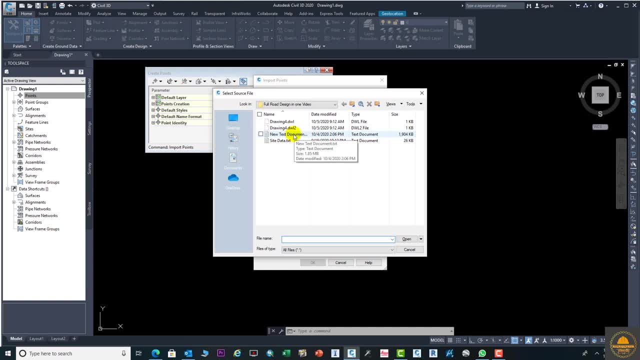 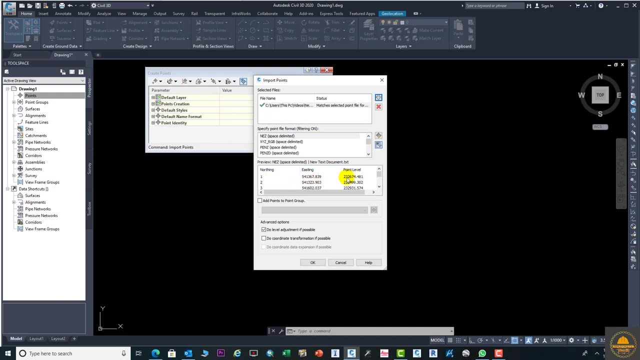 click on this and search your location where your file is saved with you and your computer. okay, select this one. and here you need to select all files. you can import your csv or text file, okay, and also look on your files. in which format is your file? suppose my format is in. 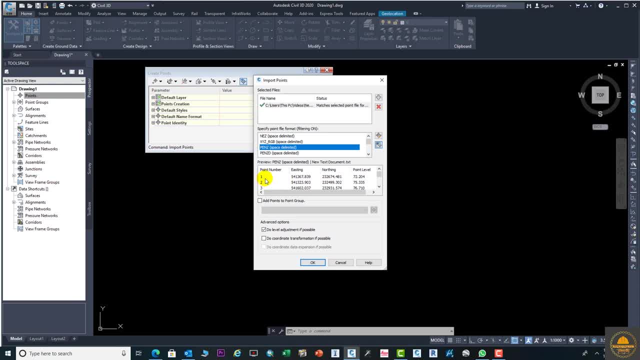 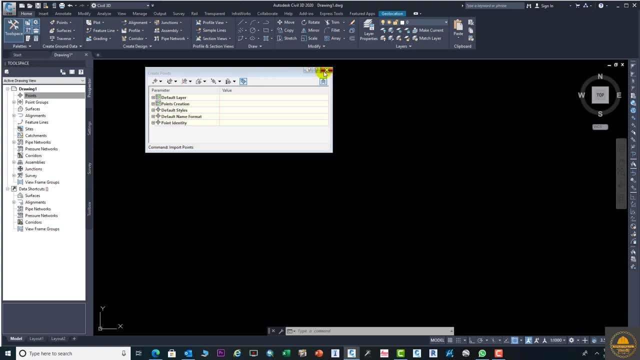 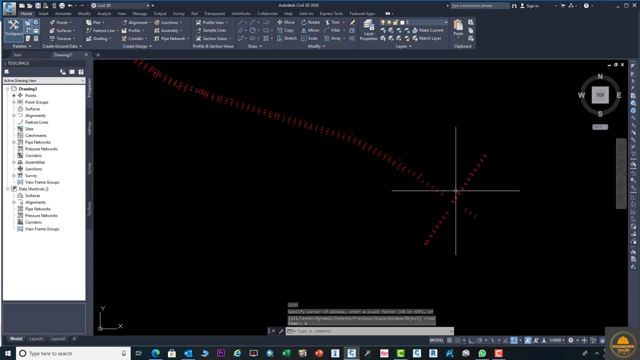 point: easting nothing and elevation space dynamic. you can see this one. just click now your points will be import. okay, let's wait. the data is height. you need to intersect spacebar and a spacebar. your points is here to a totally points is import. points is here. this is the data which we pick from the site. 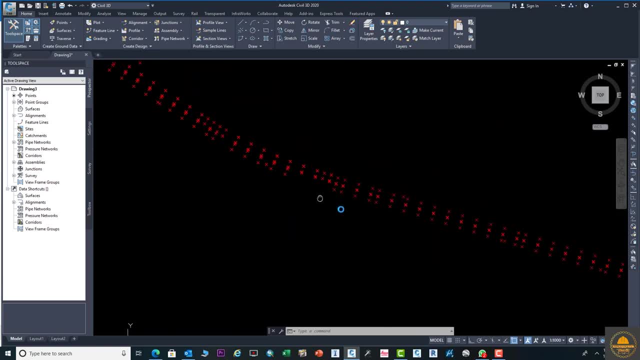 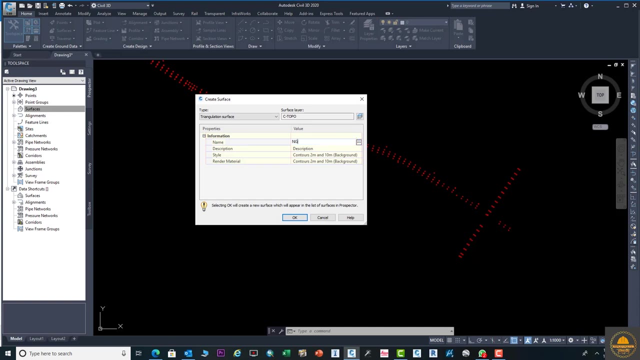 and as per this data we can design our road. you can say: this is the spill data, okay, and you need to go to this option- surfaces- from here you need to create your surface. first of all, we need to create our ngl- natural ground level- and from here you can select. 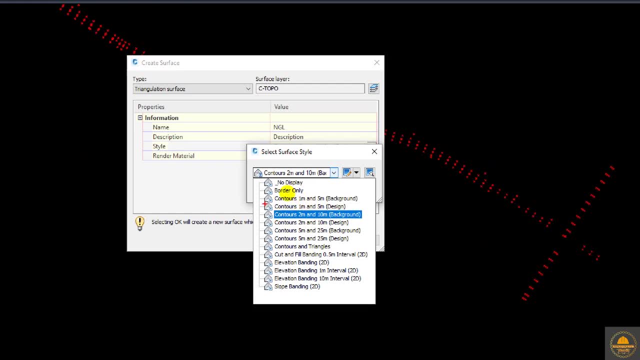 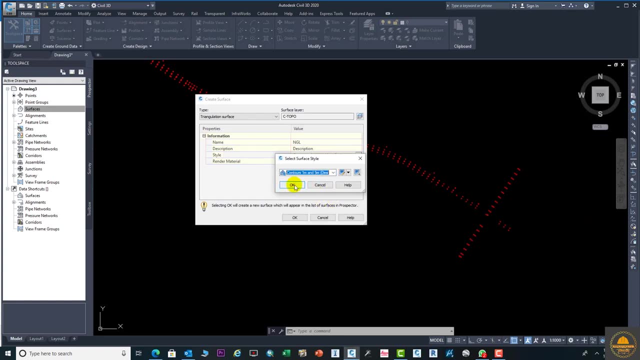 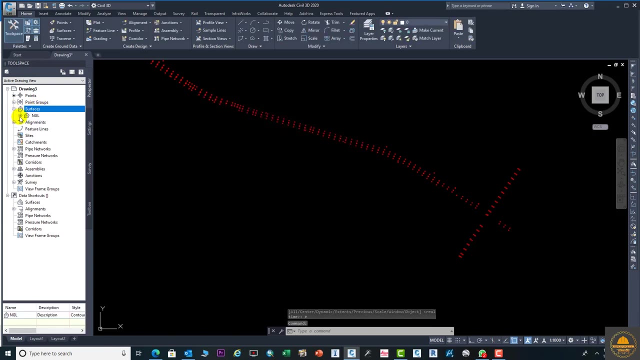 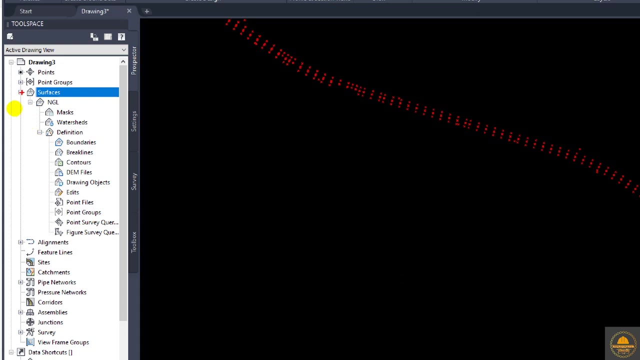 the surface style. suppose i need to select this one contour, one meter and five meter design and click on this and again. okay, now if you click on this plus button, you can see your surface from here very easily and go to this definition. okay, just i wanted to explain this thing. plus here again. plus here, you need to go to the. 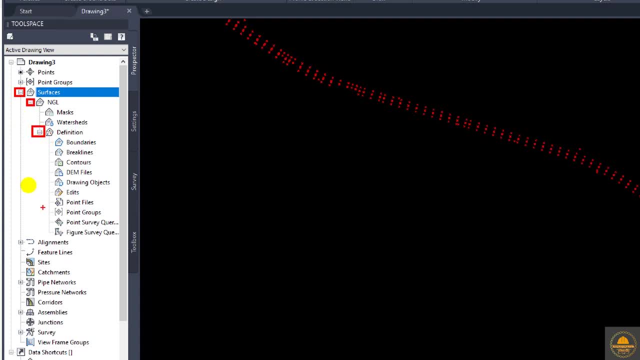 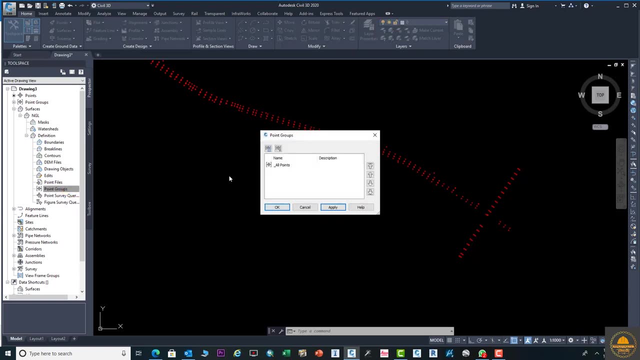 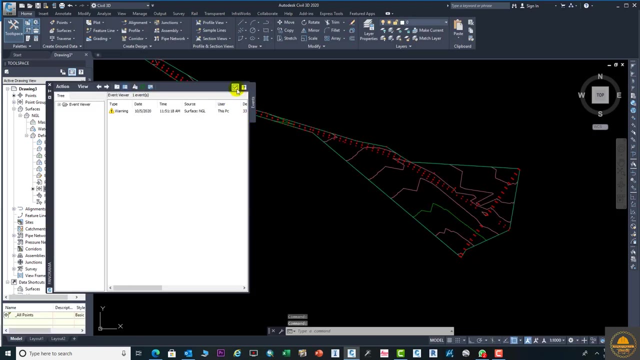 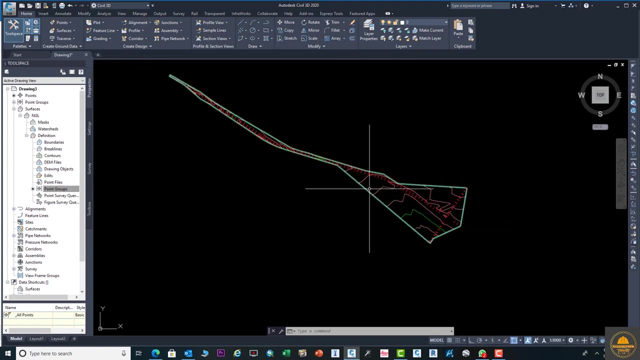 option. then you can find the points group from here. we will be at our points. if you click right and add the points, you can see your all points which you import and apply, know your this points is stored in your surface which you create on the name of ENGL, okay, and also you see your control is draw on. 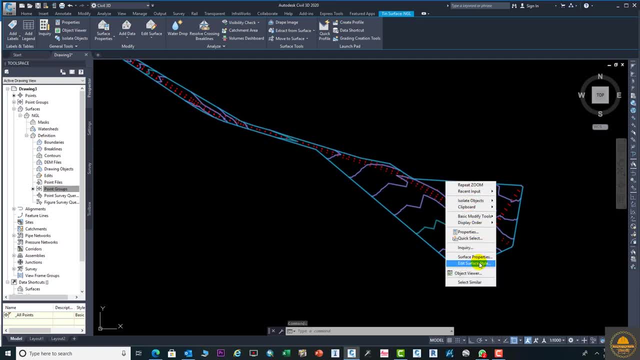 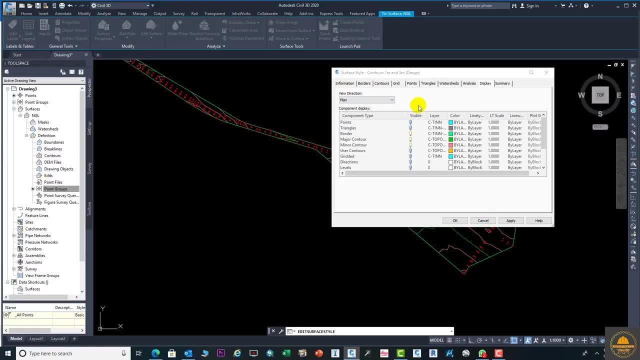 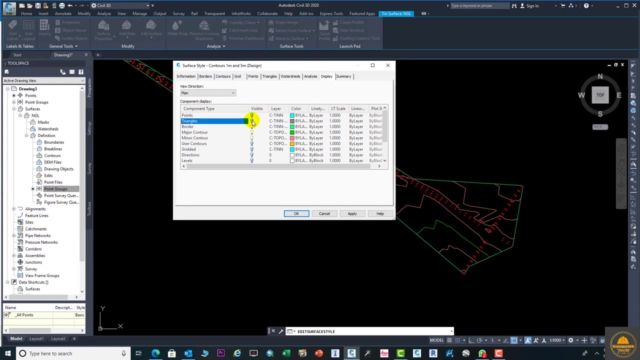 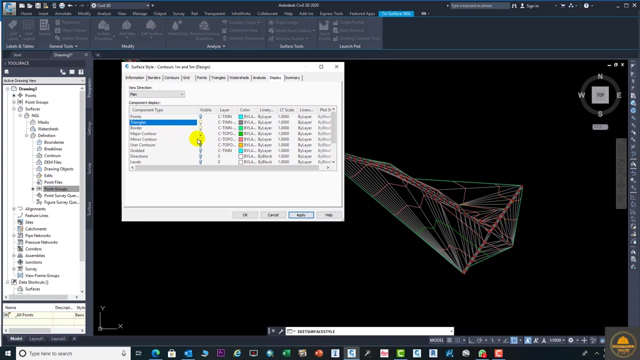 your points. now you can edit surface style from here. you can edit if you want to do any change, you can change from here, from the display. you can change the colors. you can turn on anything's. you can show you if you see the triangles. if you turn on this, turn off definitely the. 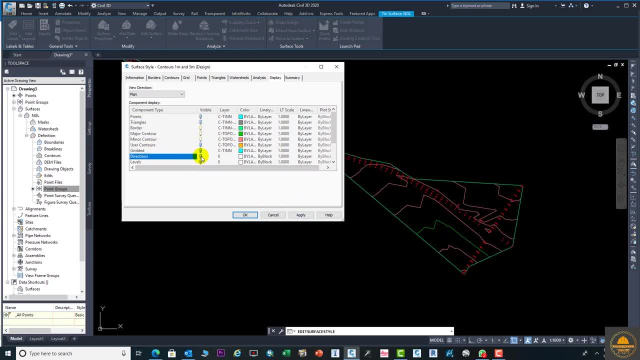 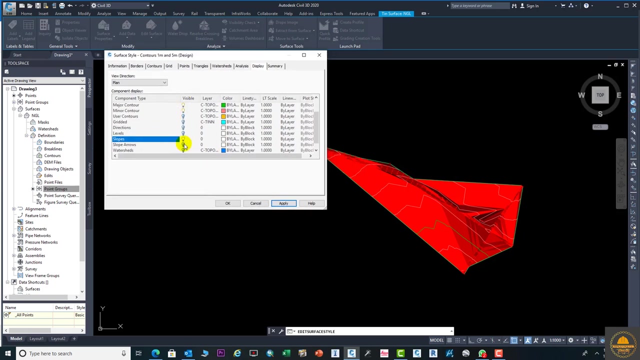 change. you will be see very clearly. if you need, just click. you can see this one. this is the direction: slope directions, levels, anything you can see very easily and with detail. okay, this one. you can see slopes. this is slopes and slopes errors. you are able to see the errors. where is? 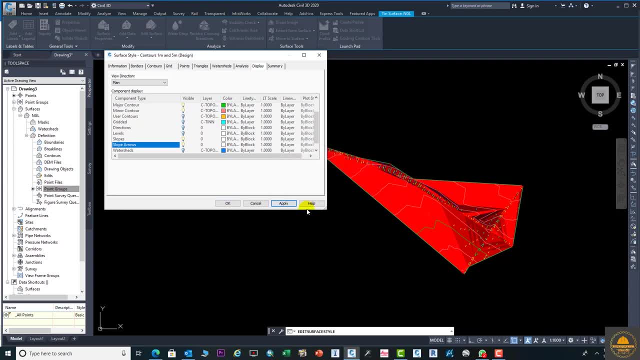 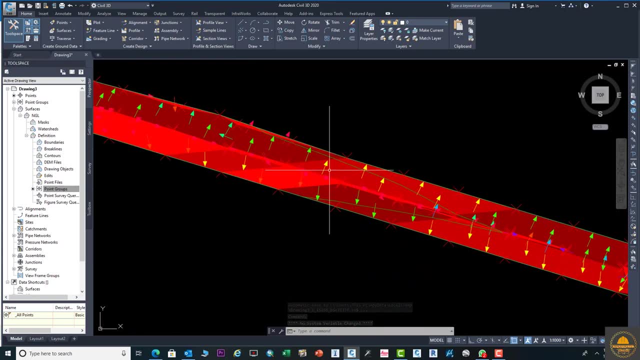 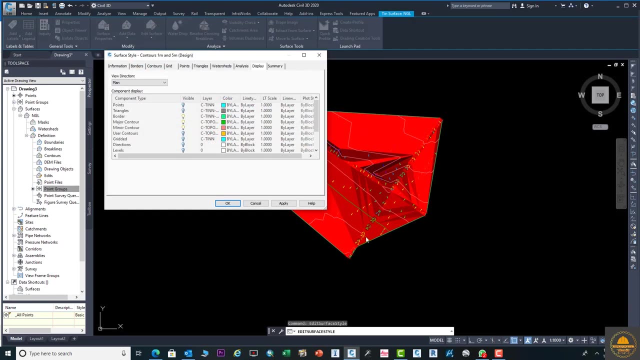 your slope is going, any kind of change you can do in your surface that you want to just assume. this one you can see. it's very easily, and which detail I am going to explain. you will never found a lecture on YouTube like that, and no, we need to. 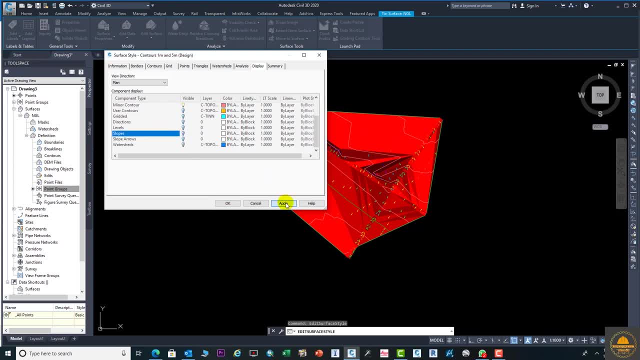 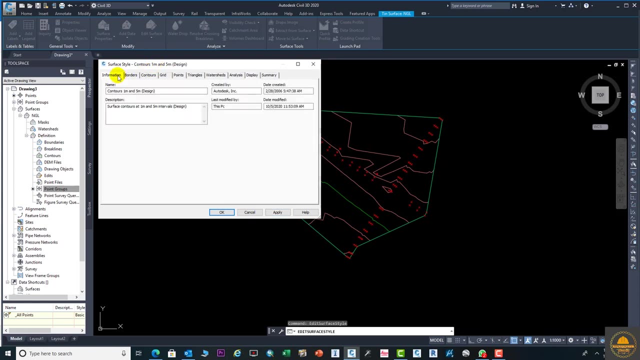 should not even go around cheat for esteem, because we're going to teach it and go from here. what you can easily, entonces, all this is our purpose. we don't need this because we are going to see the watershed, because we are going to explain how to design or to apply, and 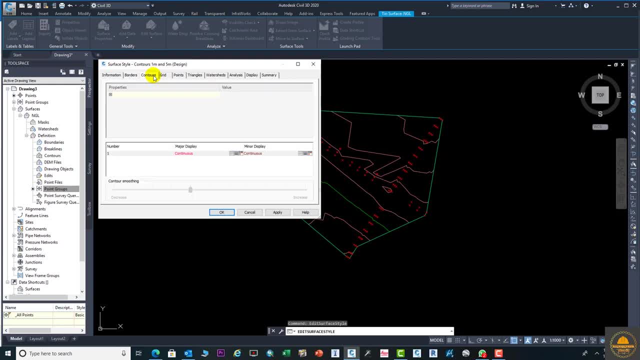 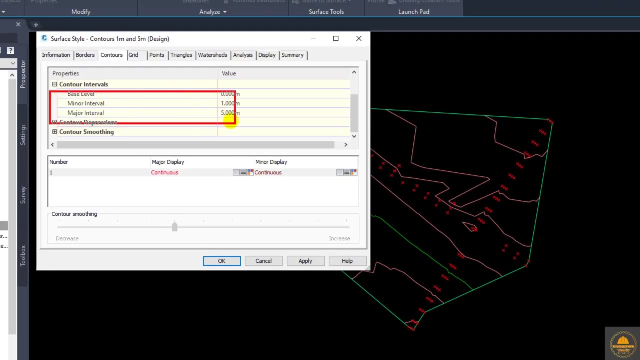 from information. you can change the name from here. if you want to change and this your control smooth. you can change your control intervals from here. this is 1 meter and 5 meter. that's mean major interval is 1 meter minus 3 and the major interval is 5 meter. if you want to change this, you can change and from here. 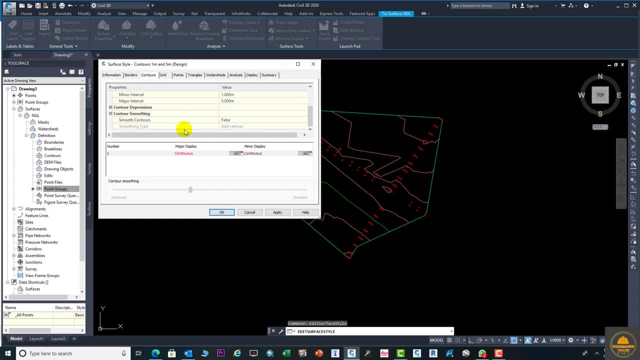 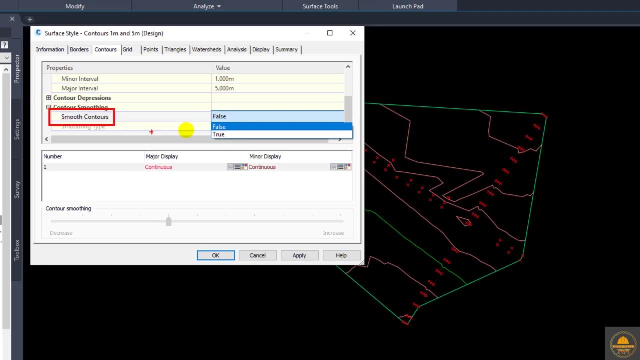 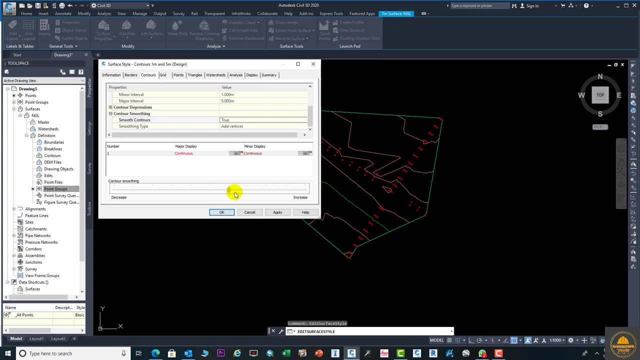 you can change your control smoothing. but first of all you need to select here from true, fast-true, then you can able to make it smoothing. they click this one true, and from here you can see this is able. you can see your control is smooth. now okay and apply and from here you can select the grids triangles, what are? 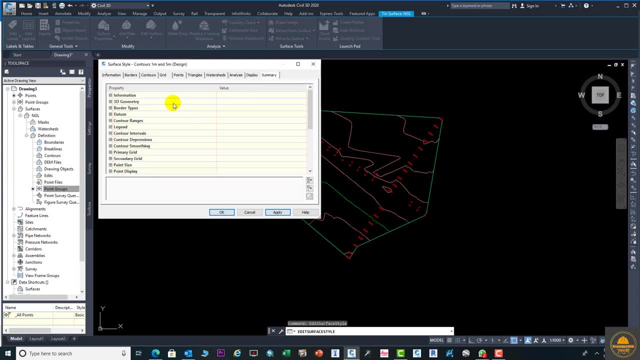 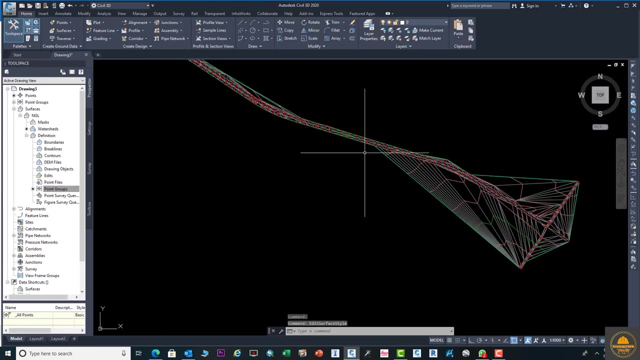 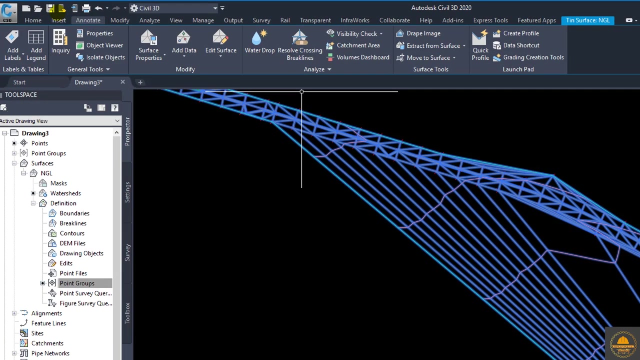 shared analysis, display summary and from here you can select the grids triangles. what are shared analysis and display summary? any kind of information if you need, you can do very easily. let's apply this and click on OK button. okay, know your surface, your points and your control is ready. just click on this and go to this. 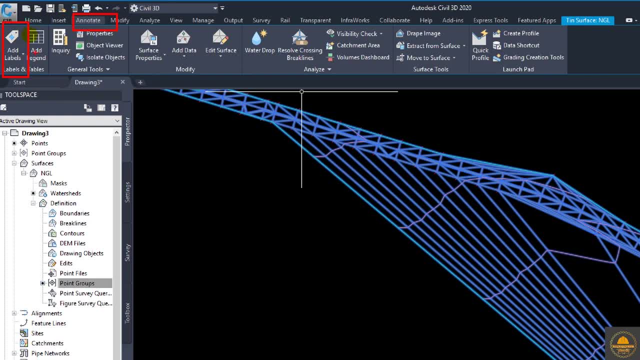 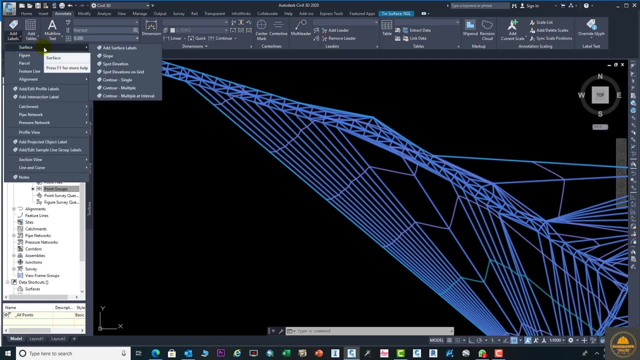 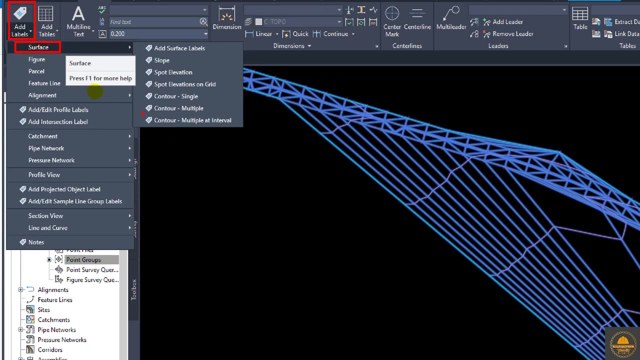 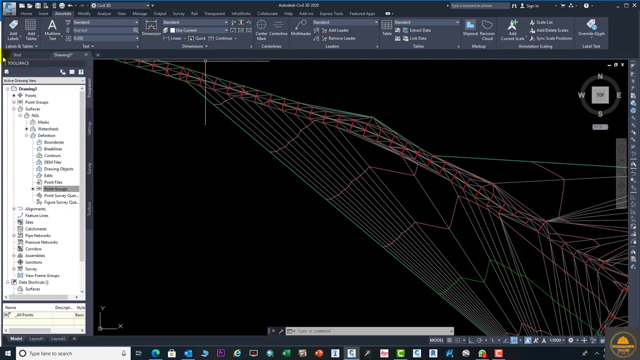 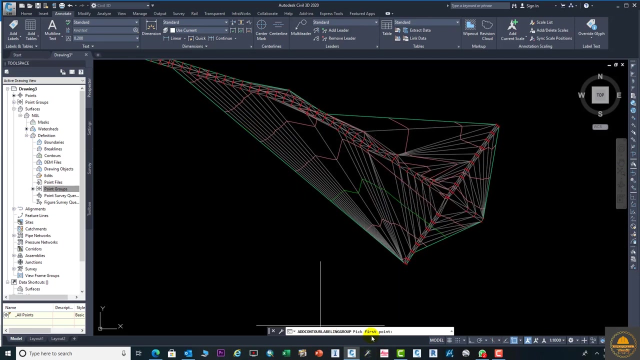 option and add labels. from here you can add your labels. go to this option and go to the surface- okay, surface, we need to do some changing in the surface. and go to the contour multiple at control. just click okay and you can select here. click here and click here. you can enter your interval and we change you need and how much. 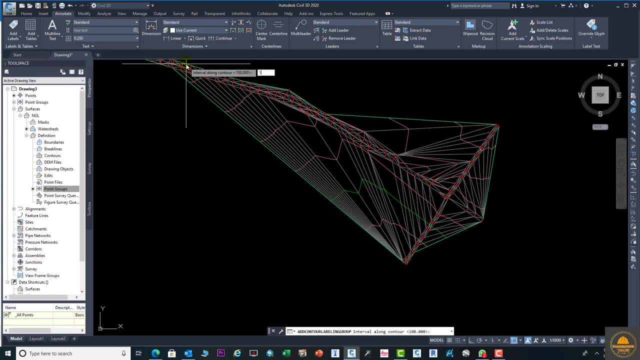 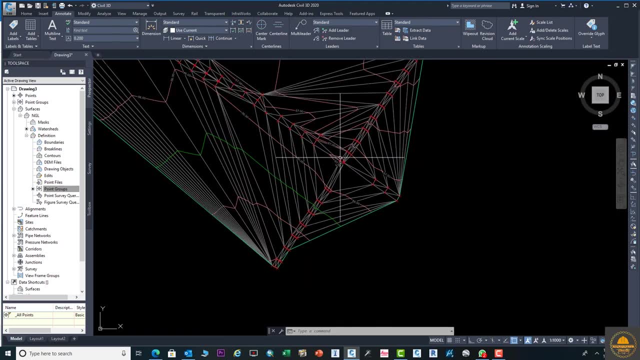 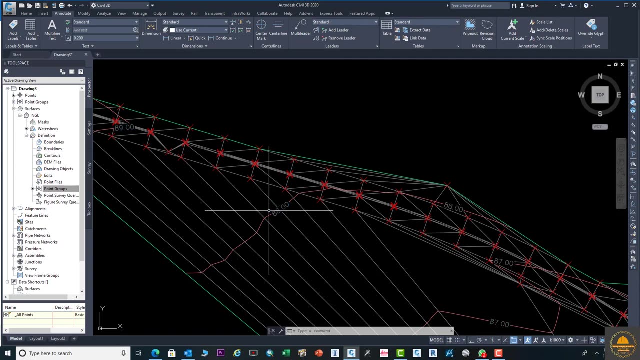 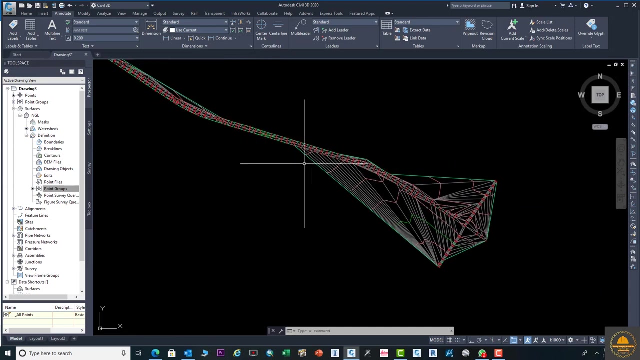 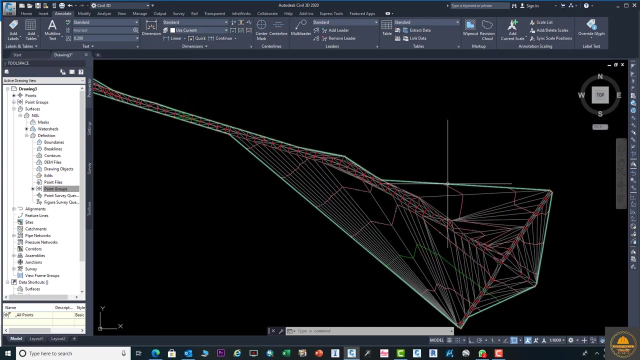 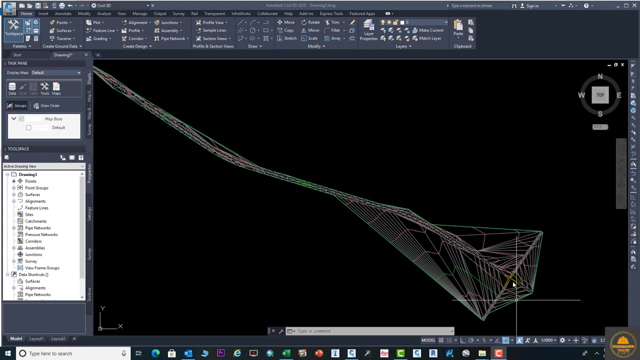 spacing. you need the interval. this is the interval, along with contour. you can see 100 width, right, you see this one. you can run 50. yes, for your requirement. you can draw your interval, okay. so this is the common things which we need to do in our contours, okay, okay, you can see, or? 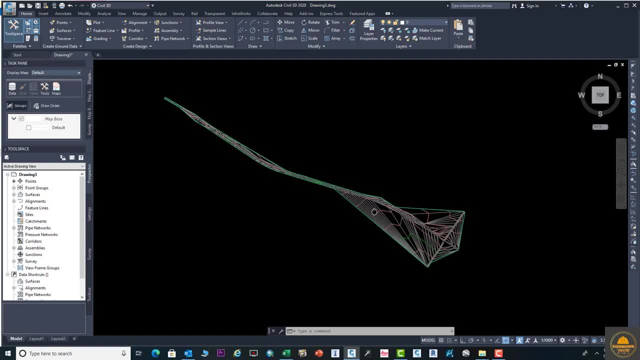 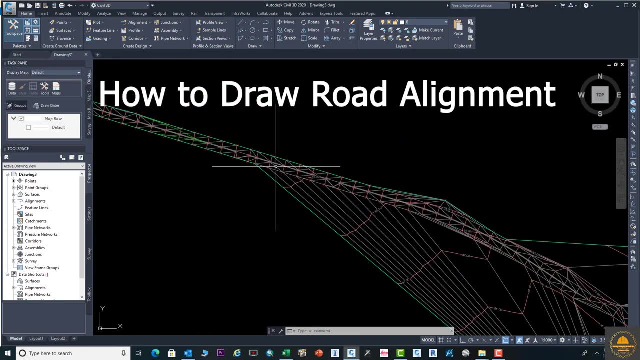 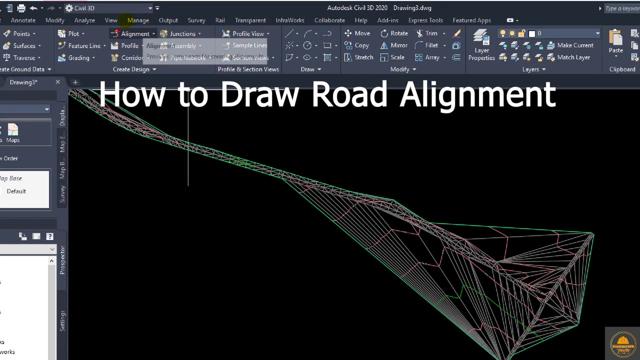 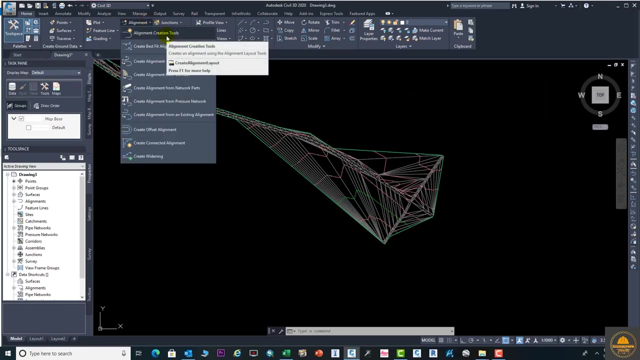 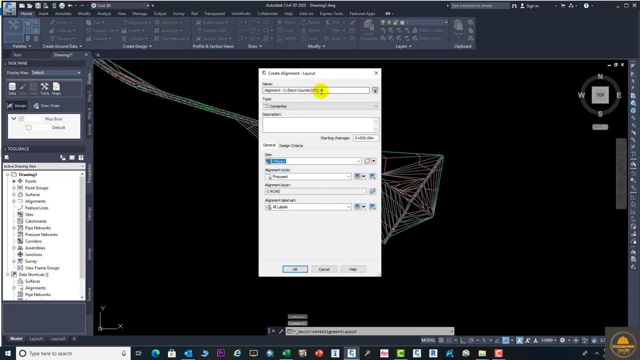 surface and all setting is no done very well. so the next step is that we will be intra or alignment. okay, we will draw our alignment. just simply go to this option, to the alignment option. okay, click alignment creation tools from here and this popup menu is open. you can add the alignment name here. 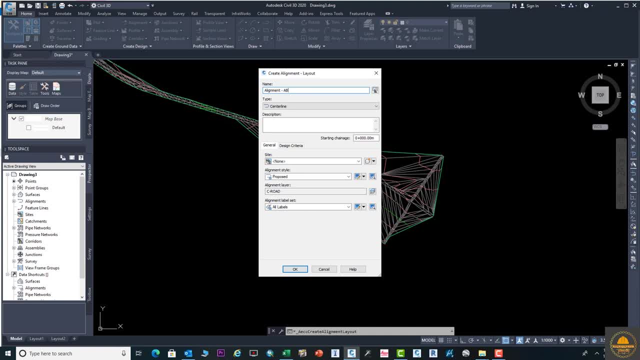 suppose adj, mark, adj, mark R, i Excel: this is the alignment a, b. see, oh, okay, okay, all right, alright, see, here we need to have alignment create tool. also, she were measuring and you can here, let's call it alignment A, B, C and then weually, and from here you can select the change, starting, change, and here you need to select label, all label. 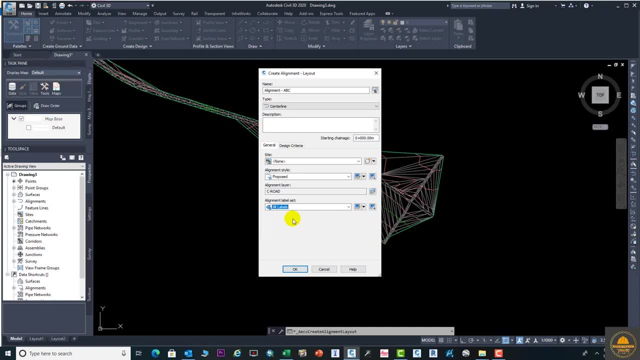 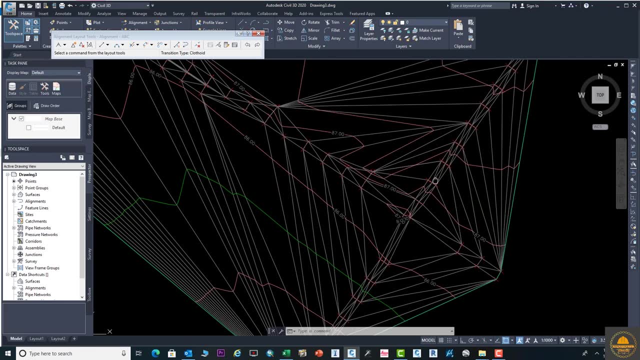 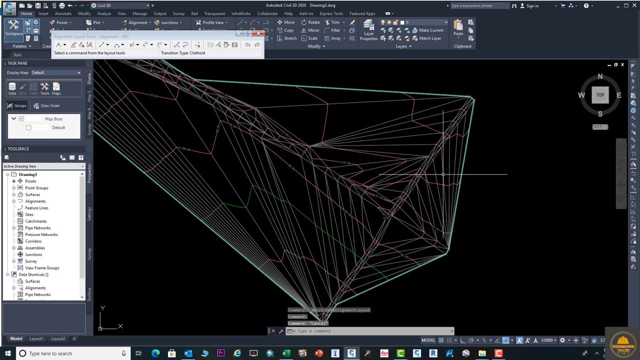 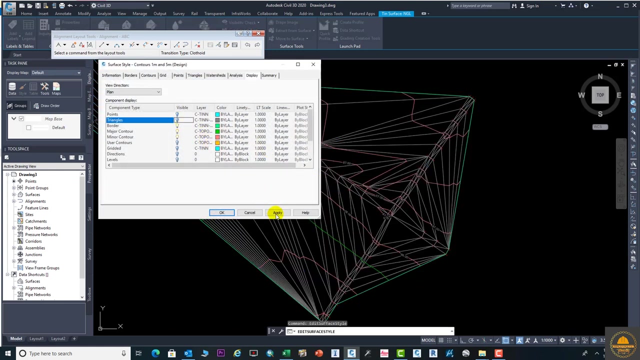 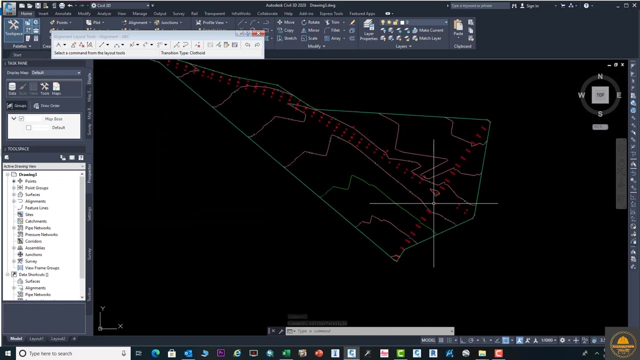 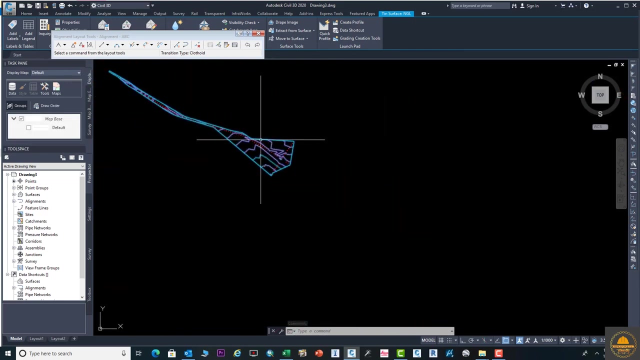 any one option as per your requirement you can select. let's we select all labels and click on ok button. now you see these tools- alignment, layout tools- is open. okay, go to this option. we need to open this, need to close the triangles. okay, here we have three. suppose we have three roads to is the small service roads and one is the main road. 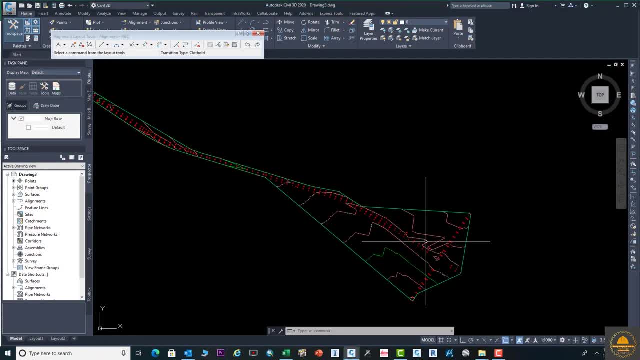 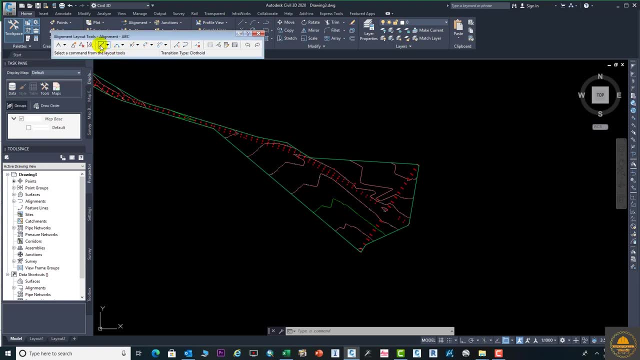 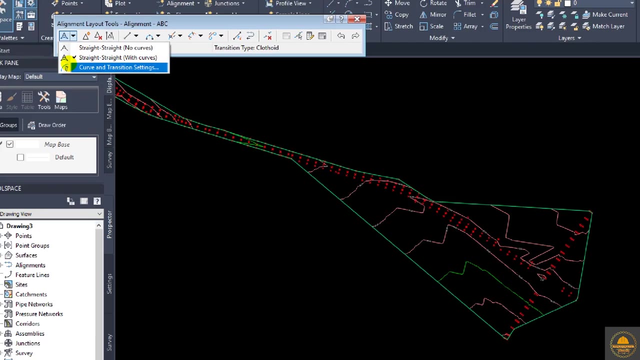 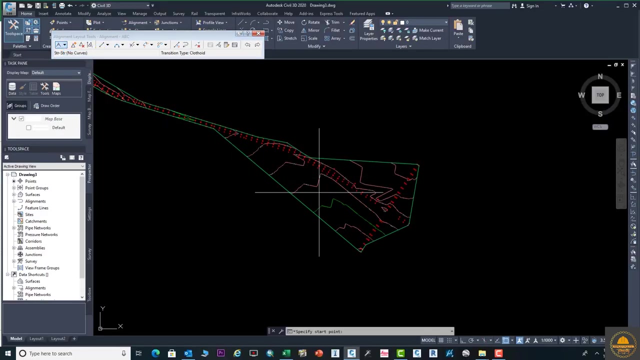 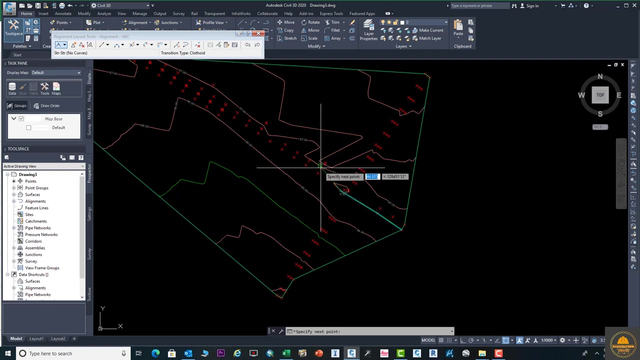 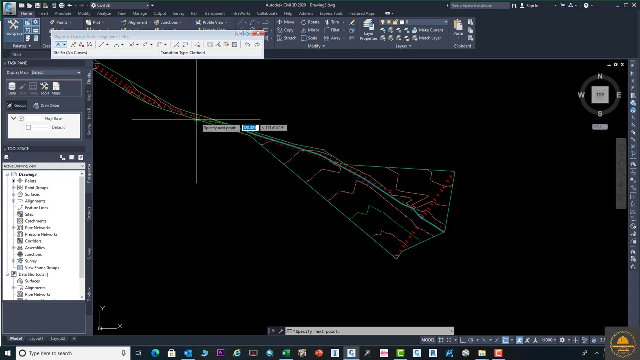 okay, this is the service Road and this one is the main road. Now click here and select the second option, this one. you can see three options to select straight with curl and select your area where you need to draw your alignment: click, click. we need to draw, you can click. okay, just make. this is the 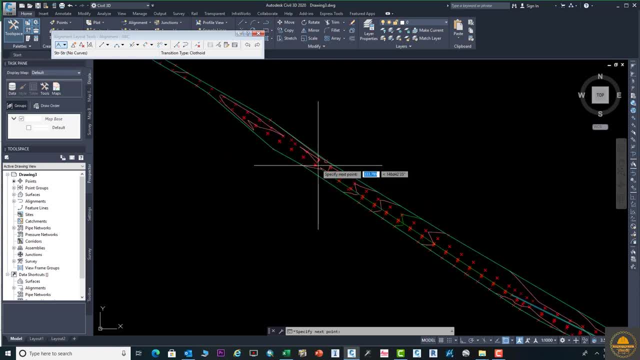 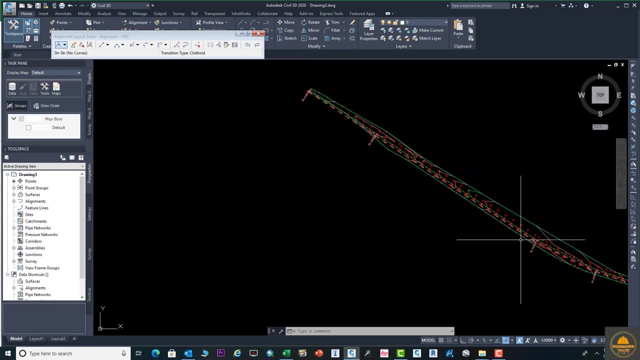 example, if you need, you can do it very purple and as per your requirement. you can do it very purple and as per your requirement. you can do it very purple and as per your requirement and as by your corridor. okay, and as by your corridor. okay, and as by your corridor- okay. now you can see your challenges, your 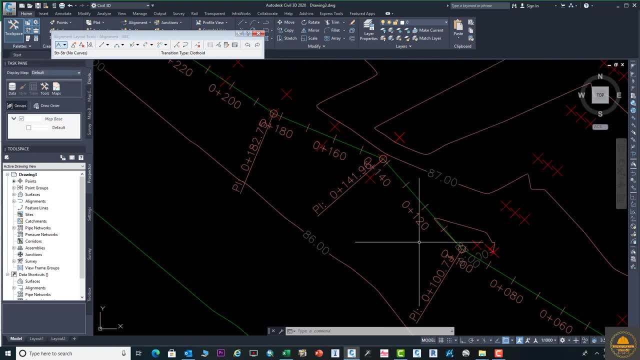 now you can see your challenges. your now you can see your challenges. your alignment is drawn off very well. if you alignment is drawn off very well, if you alignment is drawn off very well, if you need to do some change, you can do your. need to do some change, you can do your. 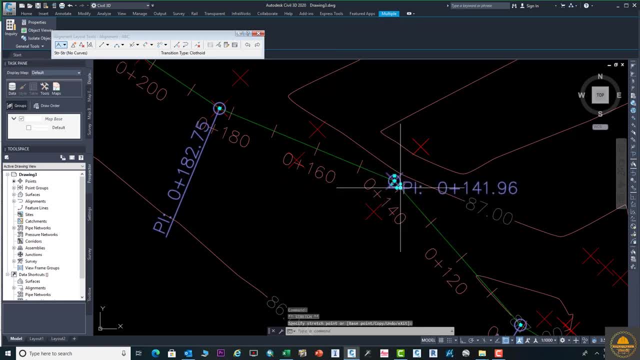 need to do some change. you can do your change from here and you can just click change from here and you can just click change from here and you can just click here and you can move your alignment here and you can move your alignment here and you can move your alignment left to right- any place you can make. 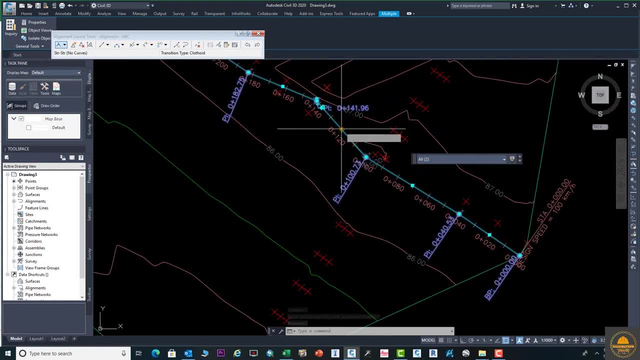 left to right, any place. you can make left to right, any place you can make it. to suppose we need to move here to it. to suppose we need to move here to it. to suppose we need to move here to right or left. we can move it very. 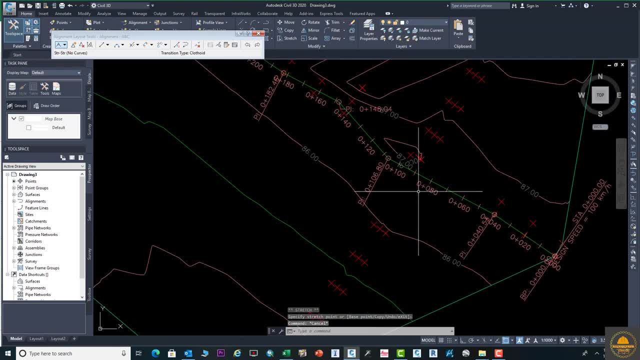 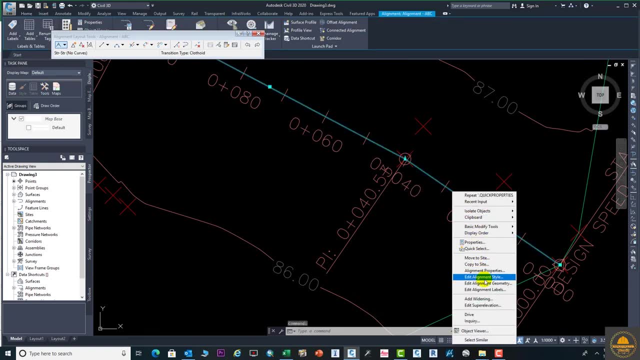 right or left, we can move it very. right or left, we can move it very easily. okay, if you want to check, and easily. okay, if you want to check and easily. okay, if you want to check and some changing you want to do some. some changing you want to do some. 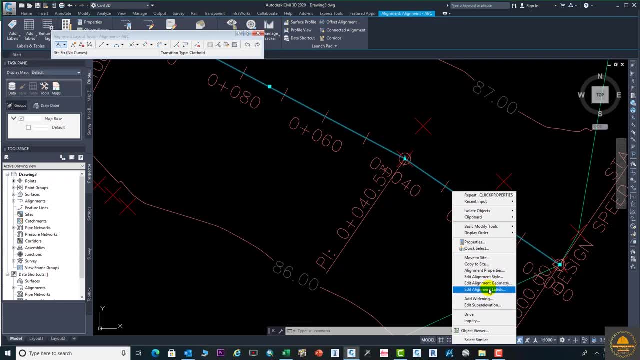 some changing. you want to do some changing? just go to this option: edit changing. just go to this option: edit changing. just go to this option: edit alignment level and from here you can alignment level and from here you can alignment level and from here you can change the challenges. you can see this. 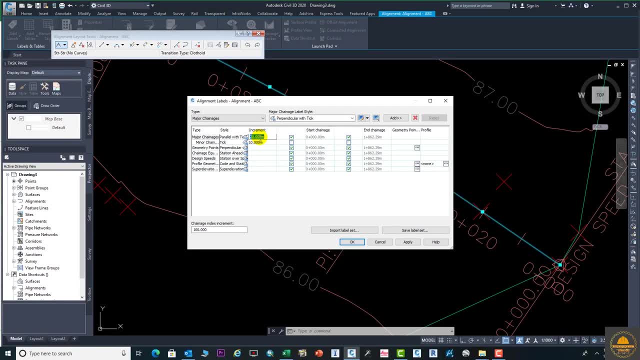 change the challenges. you can see this. change the challenges. you can see this: one, your chain is on 20 meters. if you one, your chain is on 20 meters. if you one, your chain is on 20 meters. if you want to change, you can change if you. 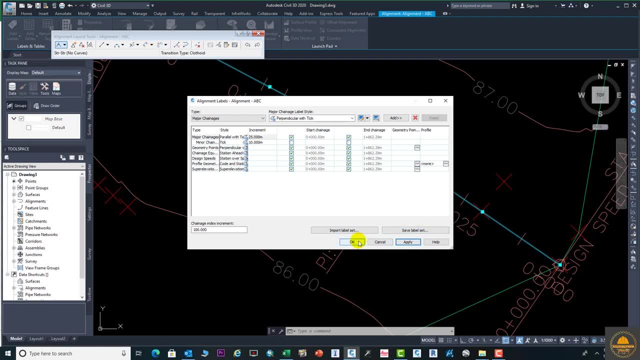 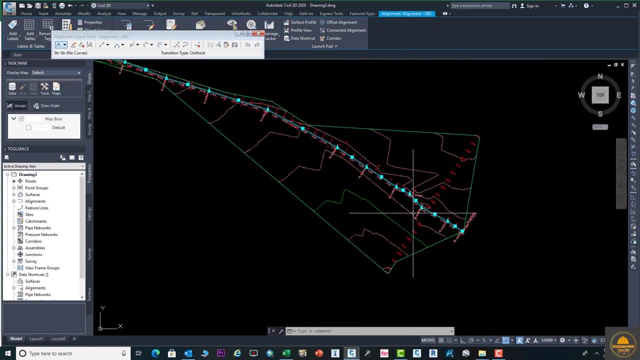 want to change, you can change. if you want to change, you can change. if you need on 25 or 50, you can change from need on 25 or 50. you can change from need on 25 or 50. you can change from here. then again, select the alignment and go. 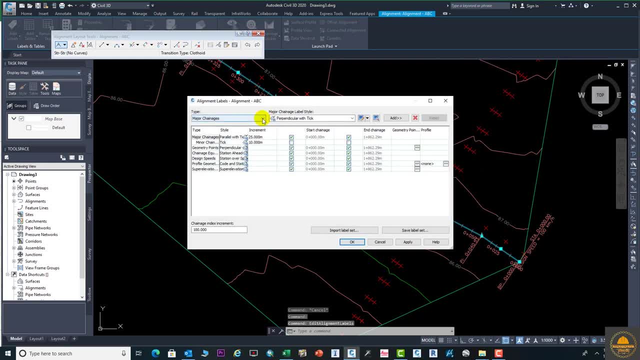 then again select the alignment and go. then again select the alignment and go to edit alignment. from here you can add to edit alignment. from here you can add: to edit alignment. from here you can add this option if you want to add this option, if you want to add. 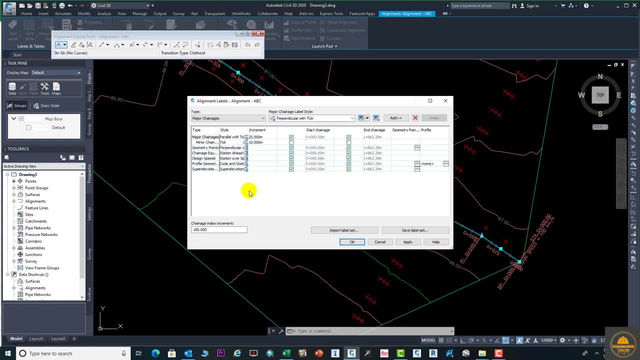 this option. if you want to add it. you can add any option from here. okay and it. you can add any option from here. okay and it. you can add any option from here. okay, and you can also import label set and you can also import label set. and. 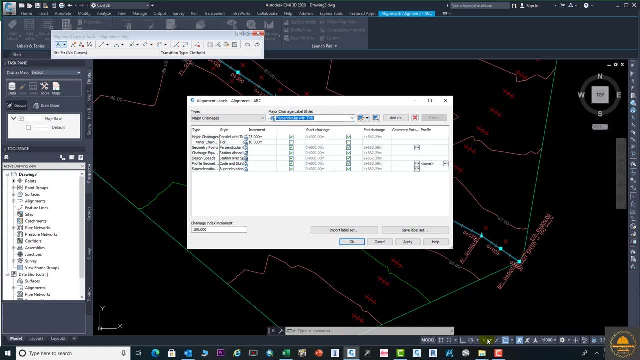 you can also import label set and from here you can select the major. from here you can select the major. from here you can select the major challenges. okay, then you can add from challenges. okay, then you can add from challenges. okay, then you can add from here very easily and here you can also. 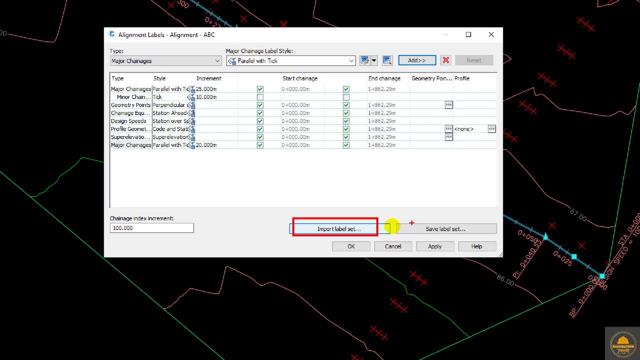 here very easily and here you can also here very easily and here you can also import. if you have any label set, you can import. if you have any label set, you can import. if you have any label set, you can import. but you, if you create your new, 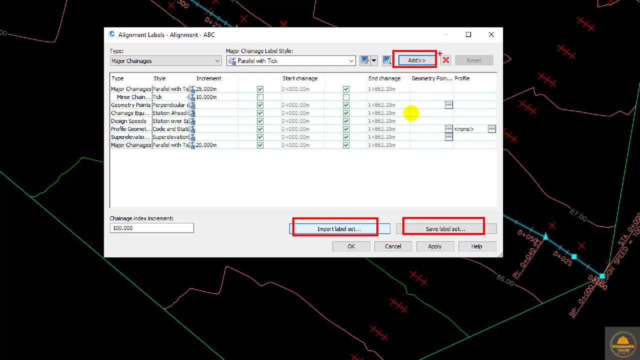 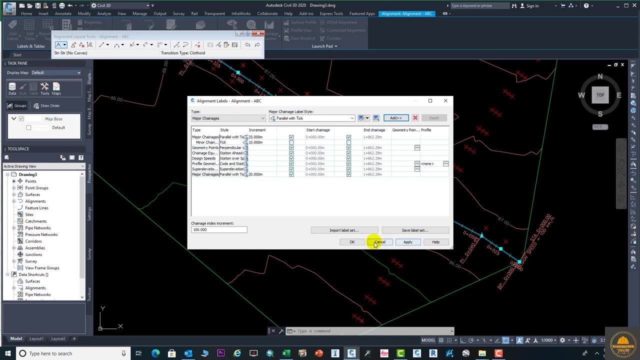 import, but you if you create your new import, but you if you create your new, then you can save from here, or you can. then you can save from here, or you can, then you can save from here, or you can delete. you can add. okay, just apply and click OK button. 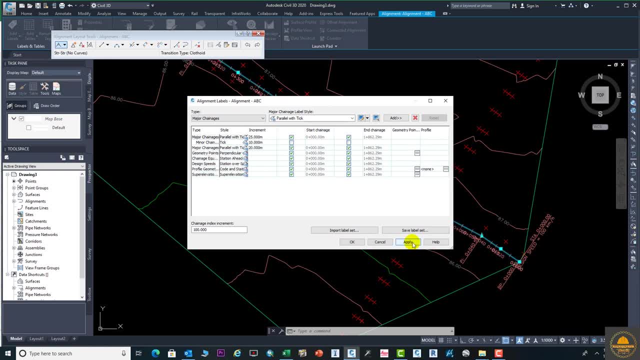 just apply and click OK button. just apply and click OK button. you can see this one is right here, you. you can see this one is right here, you. you can see this one is right here. you can delete. from here you can apply and can delete. from here you can apply and. 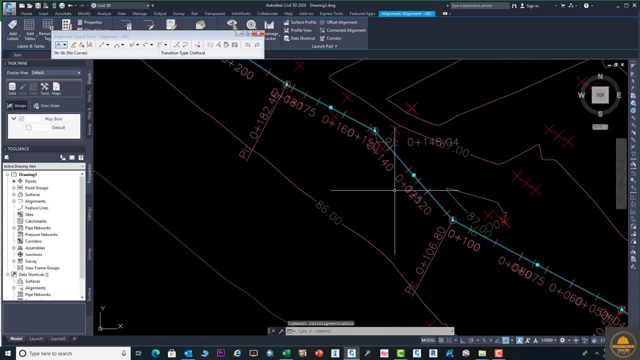 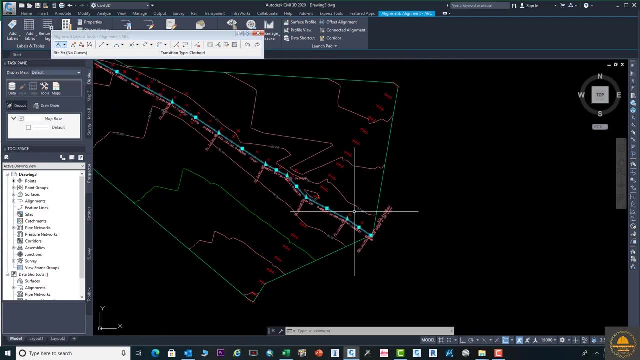 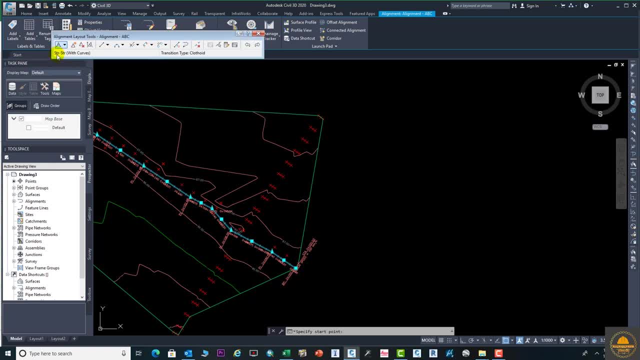 the alignment on the other one road. you the alignment on the other one road. you can do the same procedure. you can select. can do the same procedure you can select. can do the same procedure you can select. it from here: just go to the alignment. it from here, just go to the alignment. 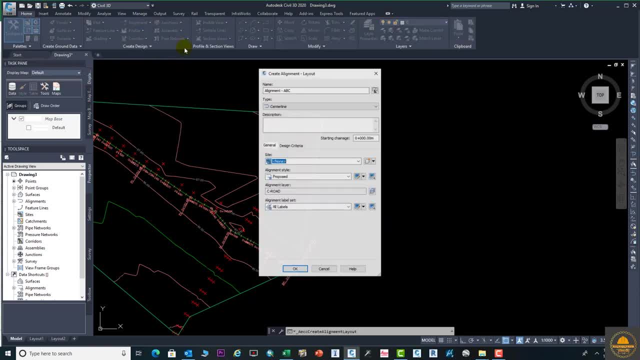 it from here. just go to the alignment same and take this one and give here same and take this one and give here same and take this one and give here alignment ABC to alignment ABC to alignment ABC to the all properties is same, which I explain the. the all properties is same, which I explain the. 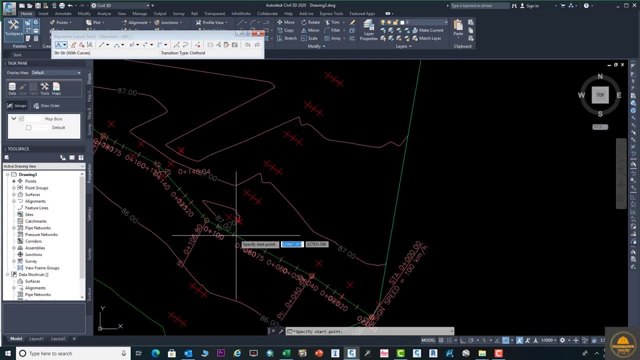 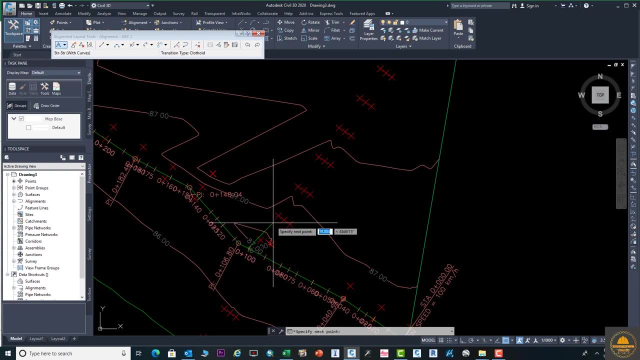 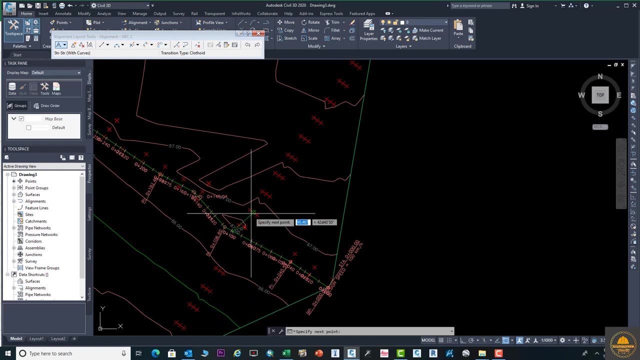 the all properties is same, which I explain. the first one with the details, you can first one with the details, you can first one with the details. you can click and you can select here. just click, go here and start clicking from here to go here and start clicking from here to. 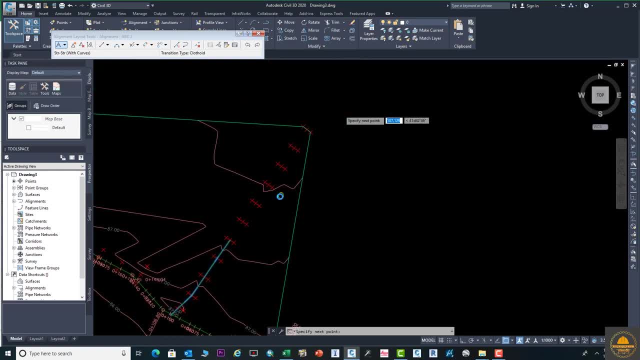 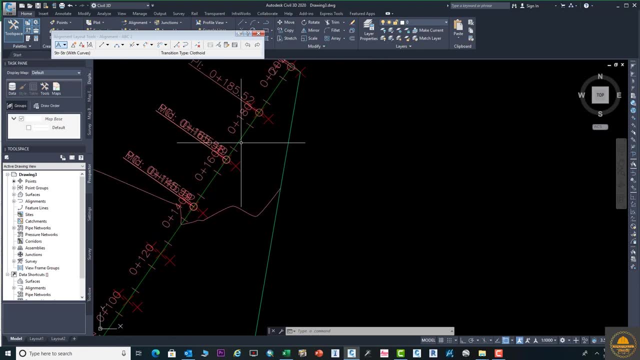 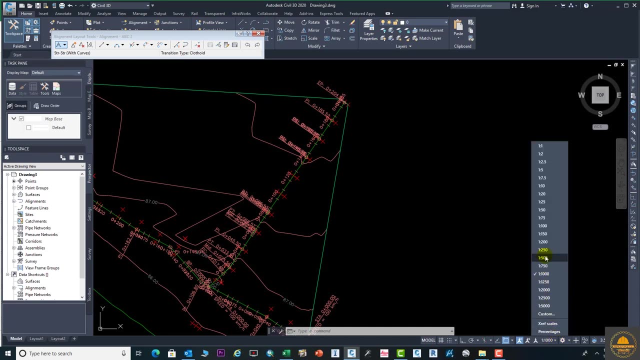 go here and start clicking. from here to here. just click. this one is the your here. just click. this one is the your here. just click. this one is the your. second alignment for the service road is second. alignment for the service road is also draw. okay, you can reduce the scale from here. if it's not clear now, you will. 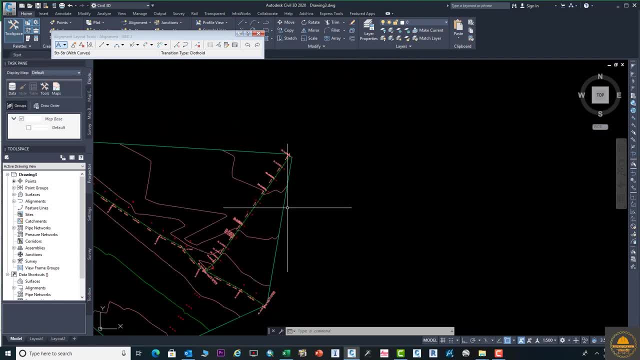 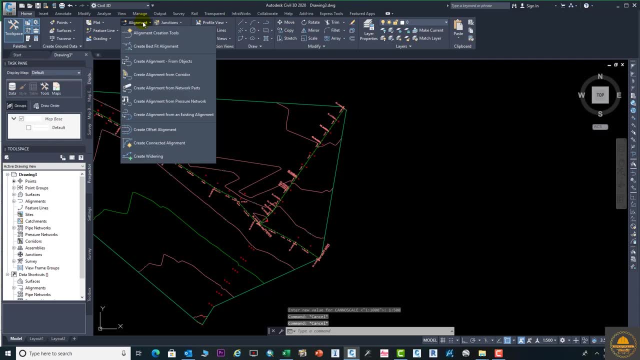 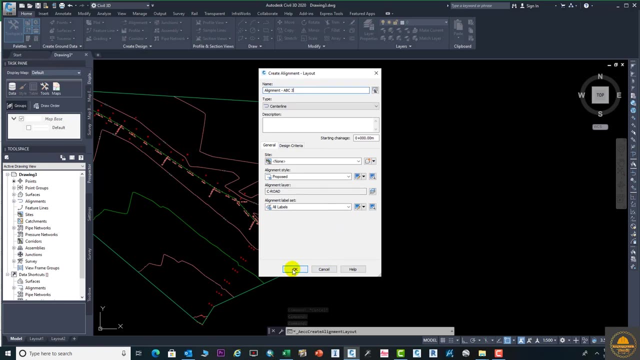 be. see it's very easily. this is 200 meter service road on the right side and maybe 140 or 150 meter will be on the left side. select this third one. we need to draw the third alignment and go to the same option and select the option. 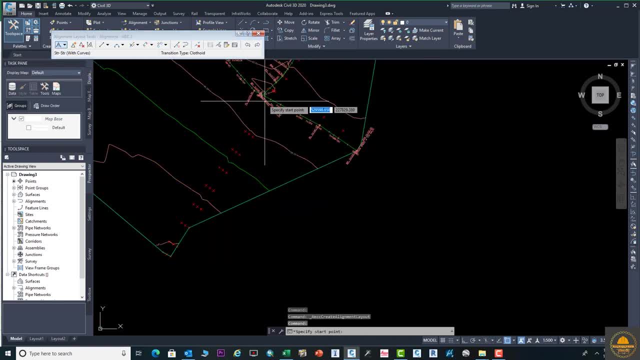 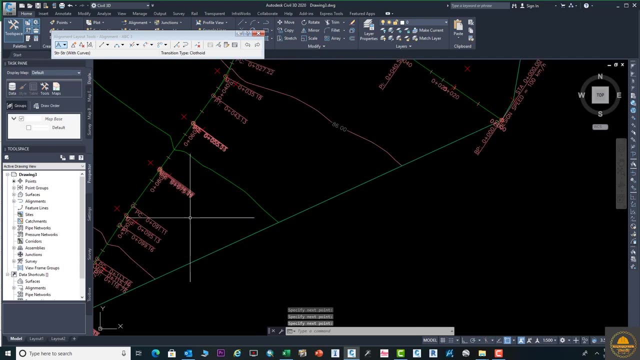 which okay and just you need to click, click and your alignment will be definitely draw. this is the rough alignments which I am going just to explain to you guys. if you want to do a proper job, you must need to do or take care how the alignment is going, how the alignment curve will be. 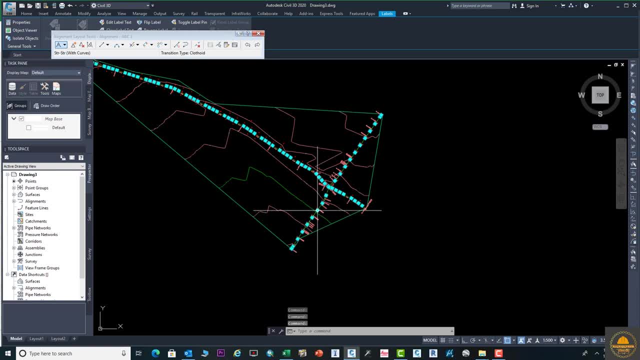 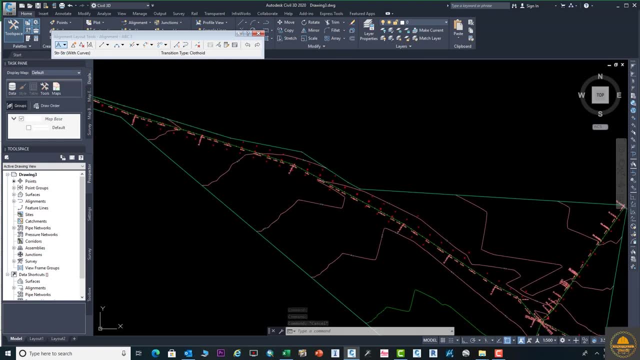 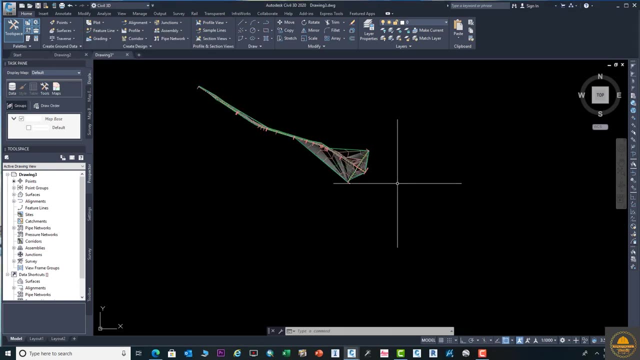 and effect and how you need to maintain this thing. later I'm going to explain this everything. details: okay, no, alignment is Ready. we already created three alignments. the next step will be create the no. you can see on the display. there is three alignment: one is for the main road and 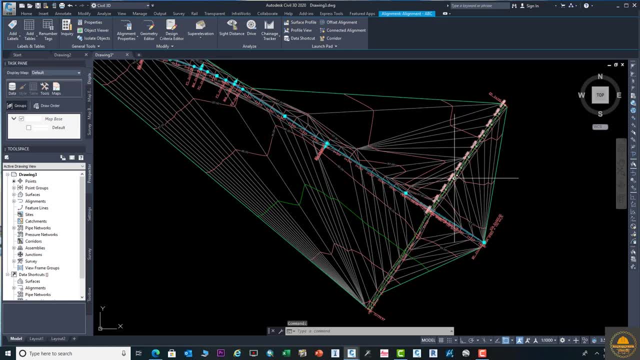 second one is for the service road, which one is or right side up to 200 متر, and the third one is on the left side of service road, which one is on our right side up to 200 meter, and bitch one is our right side up to 200 meter, and the third one is on the level. 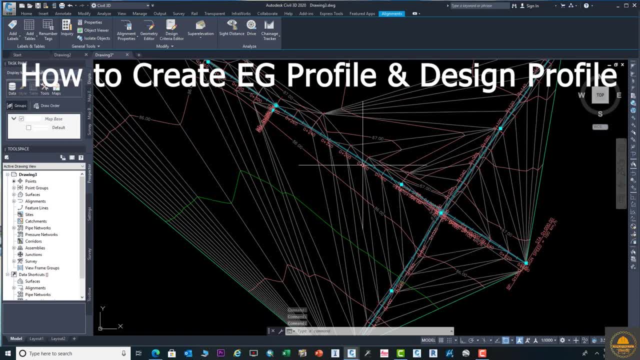 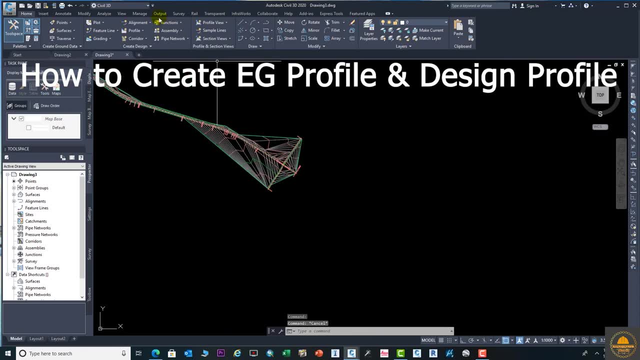 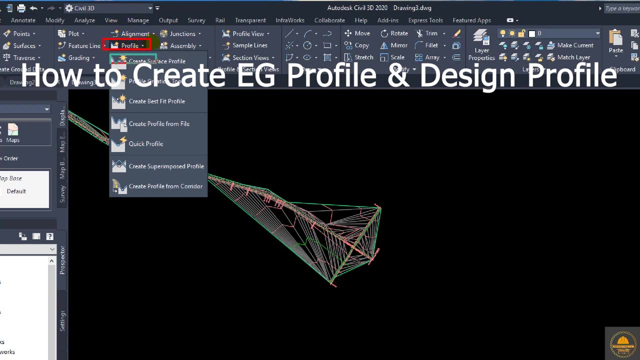 side. we have three alignment and we will create three profile for this. three alignment- okay, but later we will be. do just work on one profile. just here I am going to explain how to create the profile. go to the profile and select this is create surface profile and also you create this all kind. 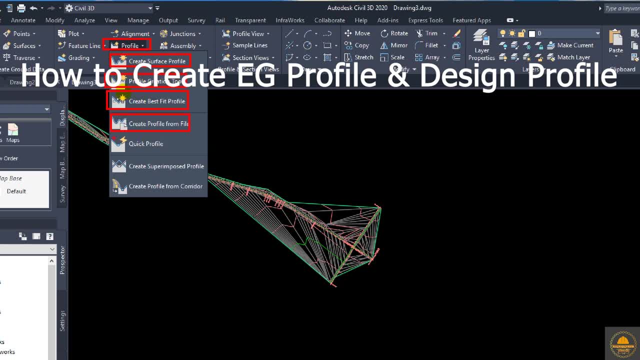 of profiles, which is your requirement, which is your project requirement. I already uploaded too much videos on separate, separate, but in this one I will be explaining the main which we are going to explain from the create surface profile. if you need to see others- others, I uploaded different- 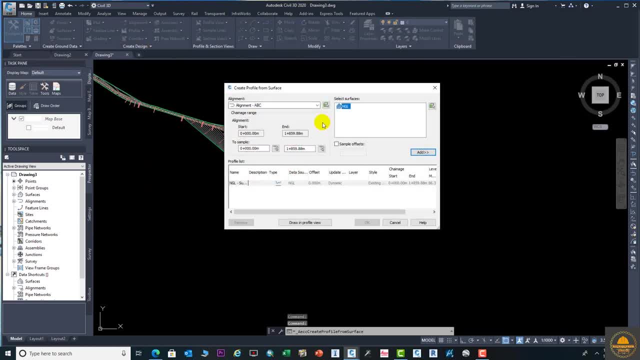 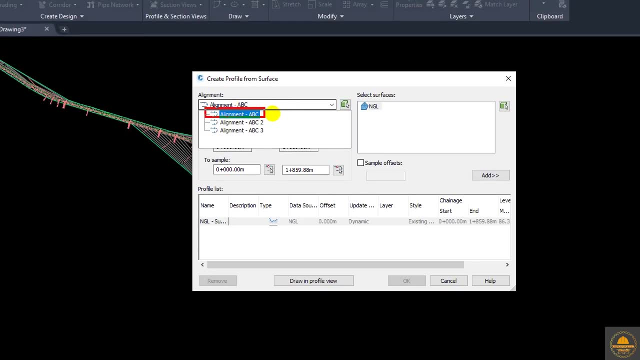 videos in the playlist you can see. so we need to select this. create profile from surface we have. first of all, we need to go to create the profile on alignment ABC. we need to select the surface. from here you can see if you have the different surface here. 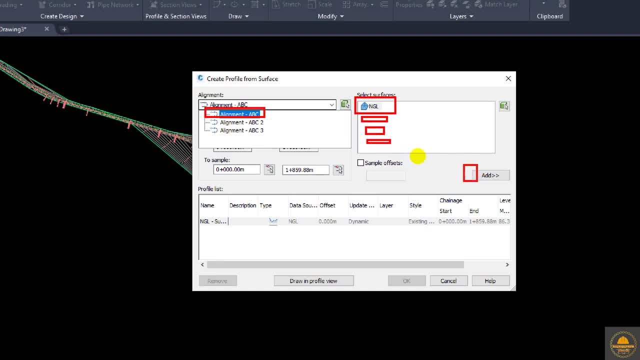 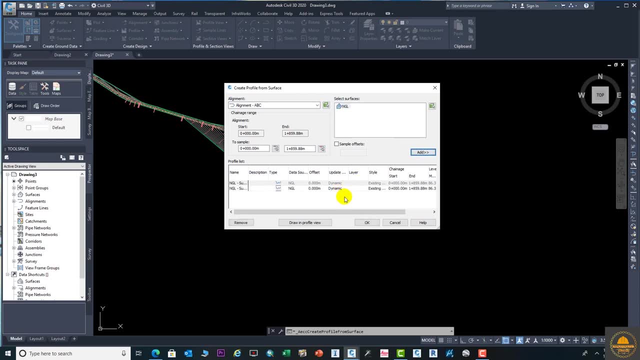 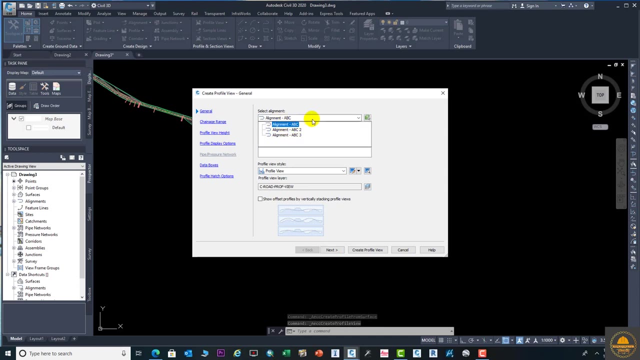 then you can select as per your requirement, which one is need and select, and then you need to go to draw. but we have only one surface here for this three alignment. just we need to click on this and here the pop-up menu will be open. from here you can select your alignment and which you are. 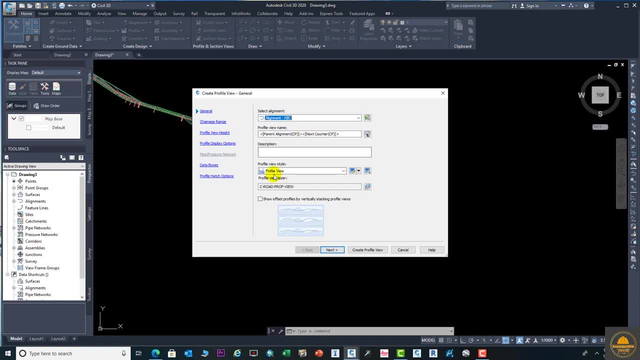 going to draw your profile, okay, and from here you can select a different option, but we don't. we need to remain its profile view and click on next and here is the automatic. this is the automatic start and end. if you need to change this specified from one challenge to another challenge, you can do also, and this is also the 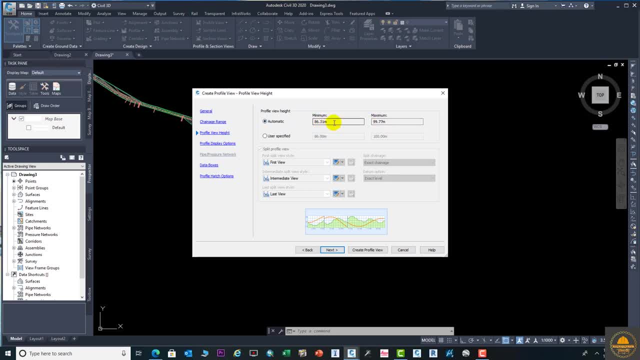 height. this is the automatic height. if you want to do this user specified, you can change by yourself user. and here there is the next thing: profile display. okay, we can, you can change this one, but we don't need to change you already. this will be the same remain. 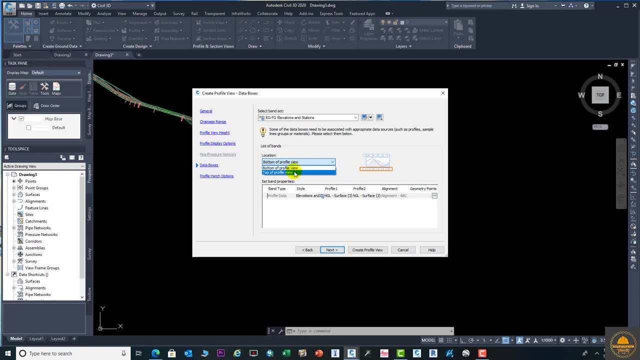 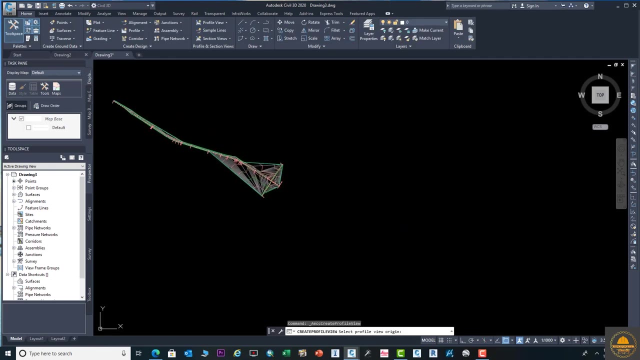 and this is the data boxes. if you need this- boxes on the top- you can select this on the top. if you need on the bottom, you can select on the bottom and from here you can see the hatches. the hatches: I will be explained this later, later. hatching is for the cut and fill. now we click this is okay, our. 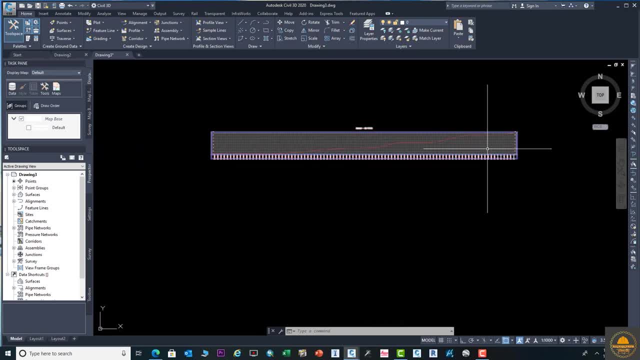 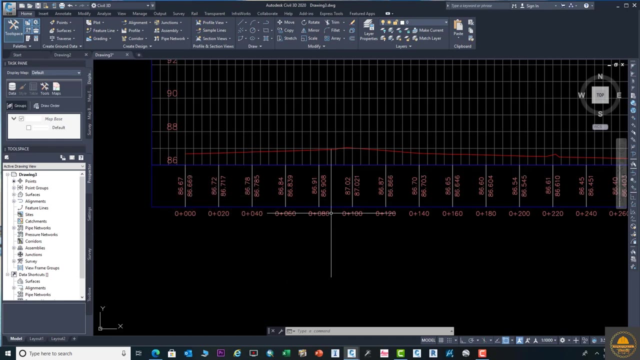 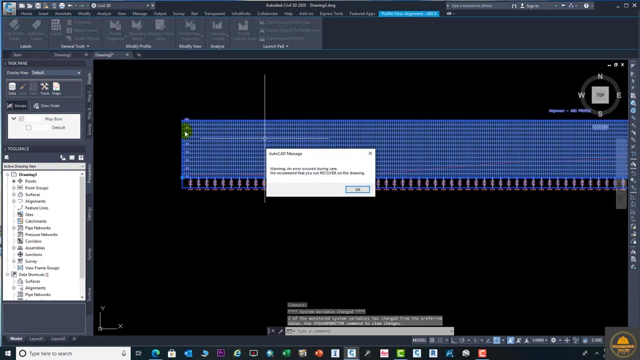 thing is finished. we click an origin and our profile is created. now, okay, you can see, it's very easily, very clear. your profile is here. okay, here you can see the challenges and your levels. okay, you need to select this uh hole. just click this one. just select this hole. 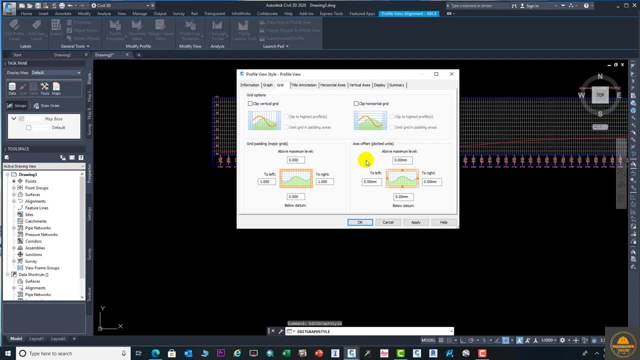 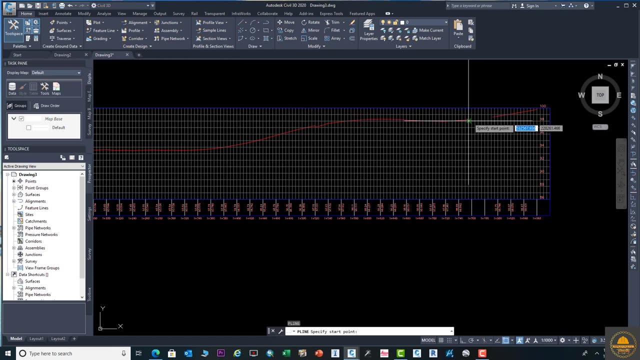 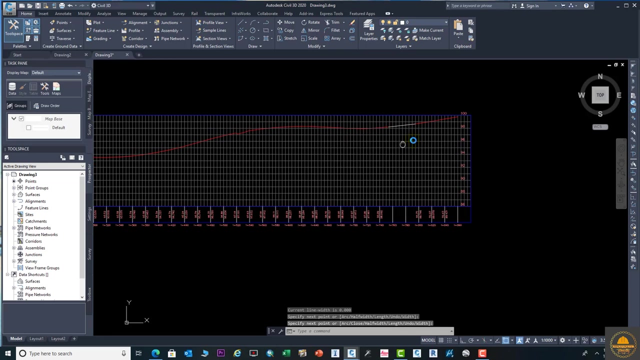 okay and go to edit profile. from here you can change your profile, a view your grid and everything, each and everything you can from here. just I think some levels is missing. any problem may be happening with my file. this is problem with my file, not with the software. you just suppose this. click there and edit profile. 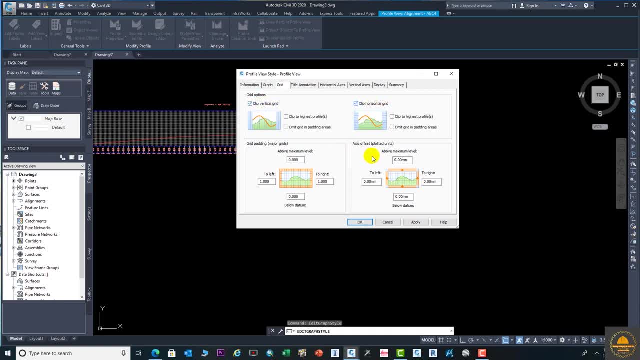 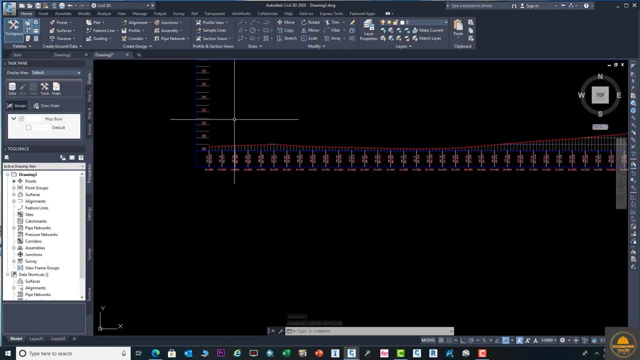 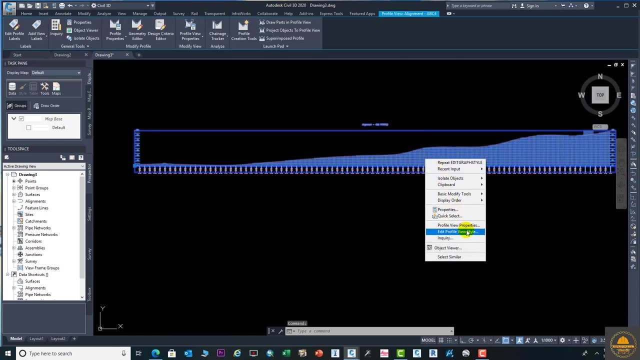 view. you can select him. you can change your grade view in the see this one. okay, now your profile view is look pretty good and the next step will be different. we have to go to create our design profile, but we need to do some changing again here. information. 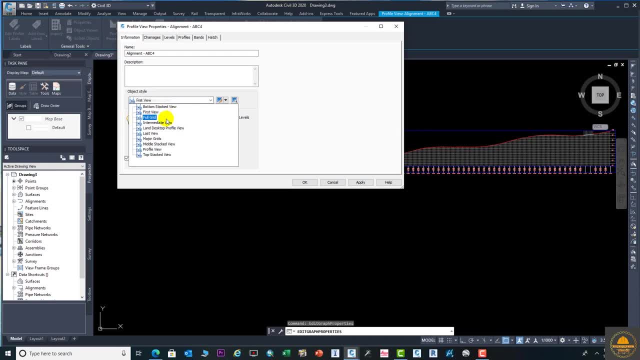 challenges and this thing. if you want, you can select this option. also, if you want to start and end challenges, you can also select this. okay, maximum height and minimum height, which I explained before drawing the profile, you can select this profile view bands, hatches. this thing is coming and next steps will be explained with detail, but here is the only look. 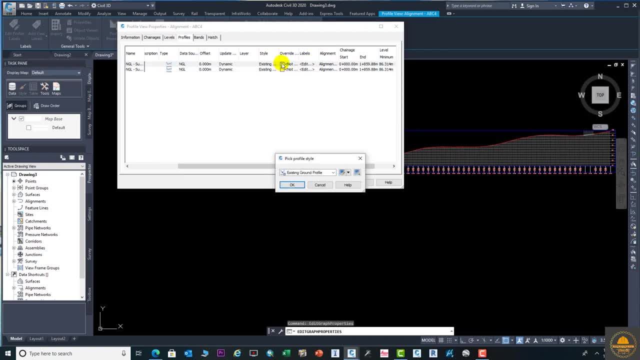 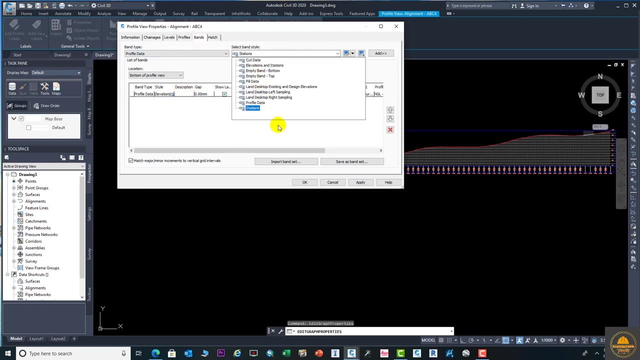 and here you can select this existing round and the other band setting. okay, yes, we don't. you can see the levels. if you see the levels, the levels will be definitely the same if we go there. if you need to import your bands, you can import it, and if you want to create your new bands- data bands- you can create from. 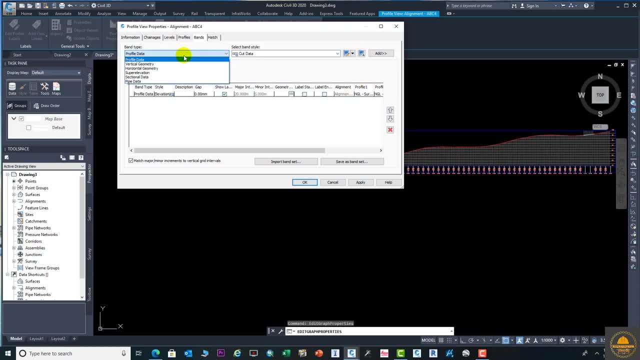 here. later I will explain the detail how to create the bands. okay, profile data or vertical geometry of supervisor bands you can able to learn in this video. I will explain few bands. once I you learn this how to create, you can create all the bands and, as it is which we do, I will explain and from here you can edit the hatches. hatches for which: 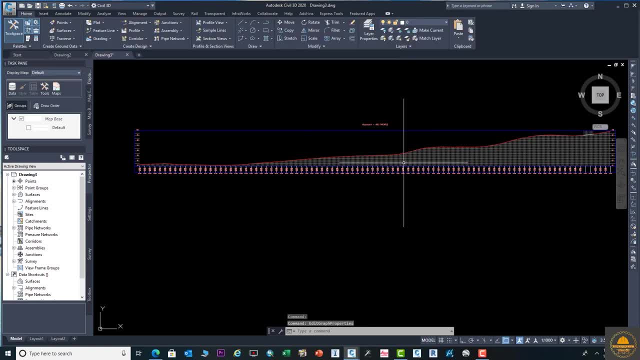 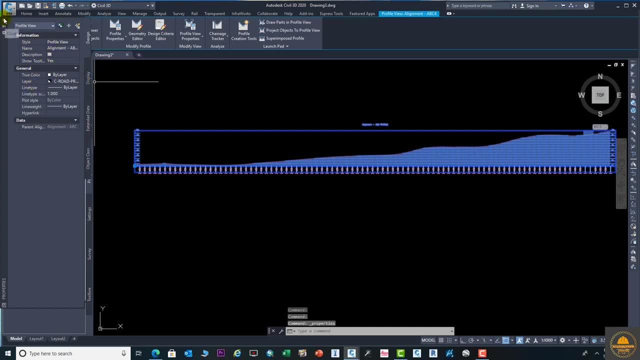 purpose. suppose you need to show the cut and fill area in red and觌 cruellunc runour region space examples needed individualэ need to show the cut and fill area in red and burglar hatches. you can show it's very easily and if you need to go to the properties from here you can see the properties. then again we need to. 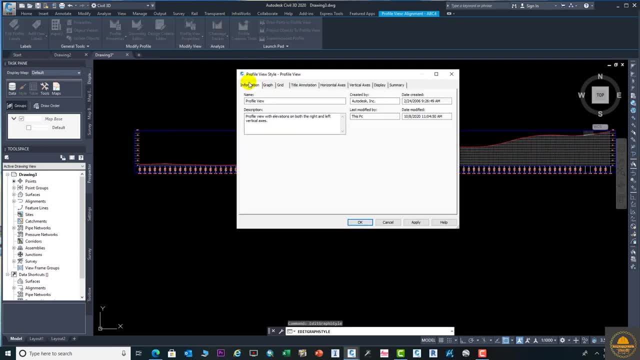 the profile view style. from here we can go to the graph. we can select the graph. okay, and from here we can select the grid. if you need to show grades less, increasing the grids quantity, you can increase very easily. this is the title annotation. you can see how much is the text height. you can change the. 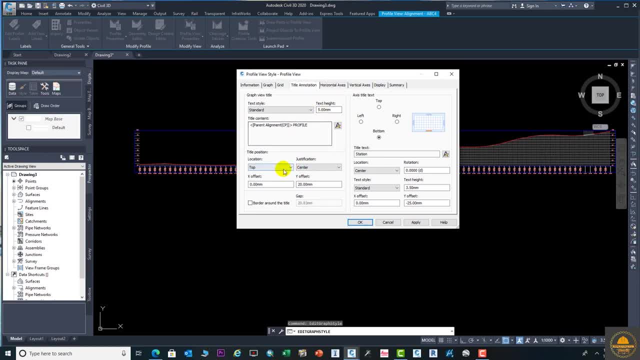 text height from here and from here you can center, left, right, you can change, and this is the horizontal axis which you see. if you need to change the challenges and which changes, showing your details, you can do it. this is with the 20 meter external and external. this is a vertical. 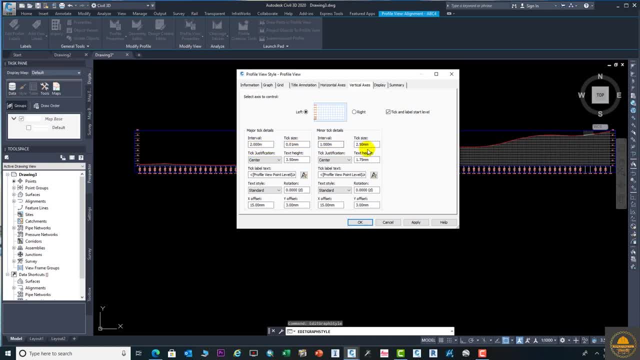 vertical grade. if you want to change the vertical heights which you see on the left side, which my icon is going, you can change from here. here is the display, a lot of things you can make it hide. you can make it able to turn on your some layers on in this, okay. 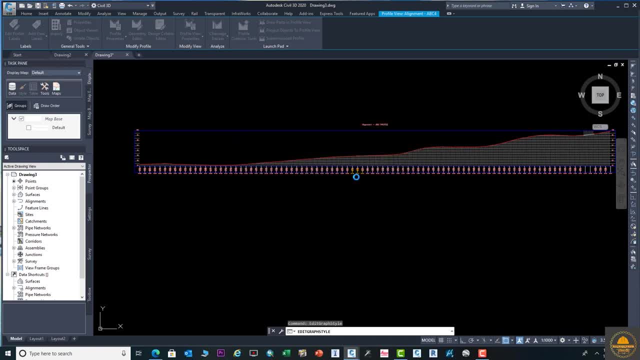 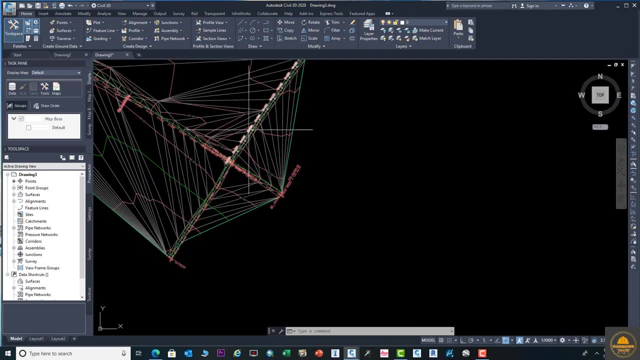 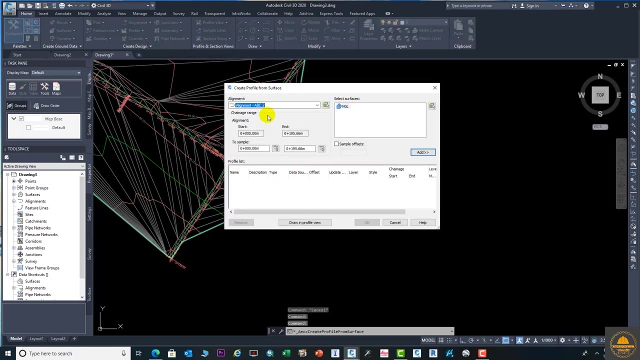 so this is the summary. i think i hope you guys understand from this thing a little bit. i'm doing quick because this is a very lengthy video. i am trying to finish as well as soon possible. try to understand. and the next: we need to draw the next profile on the same way which i explained the first one. 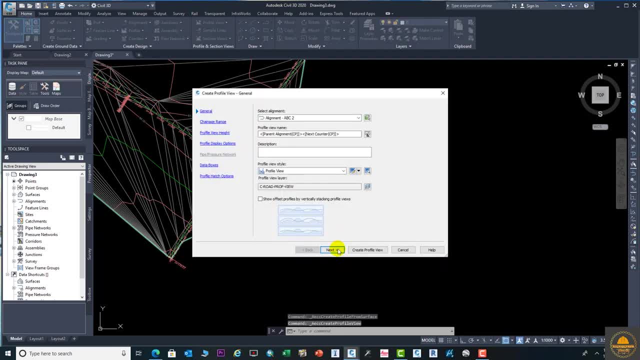 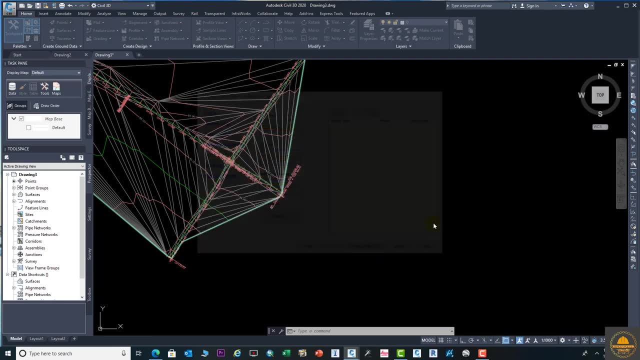 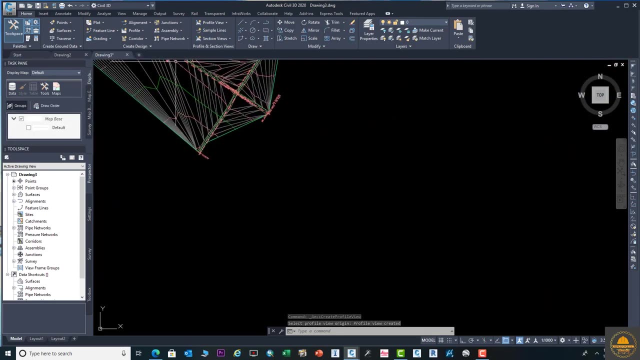 we need to draw profile on the abc2 alignment, which is the service route on the right. next click, and next click, and next click, create and draw. you can see, oh, your small road profile is created now. now we will go to do the same thing with the a, b, c, 3 element. okay, and 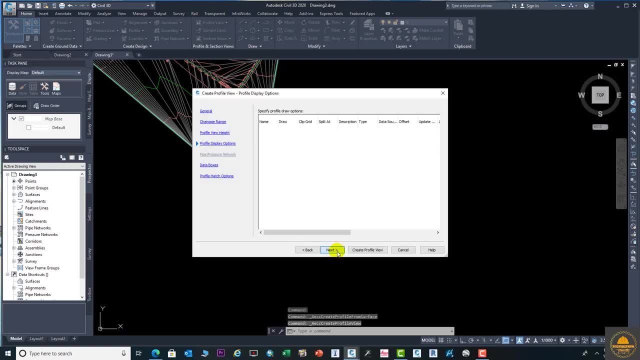 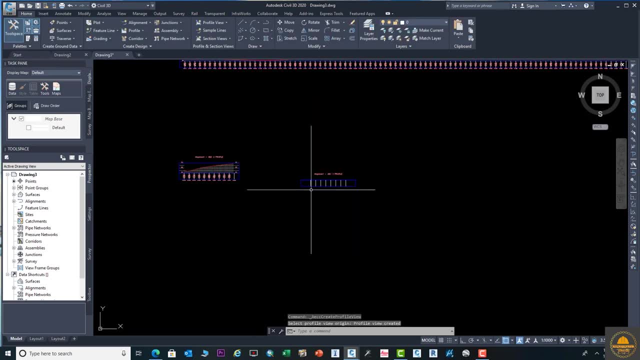 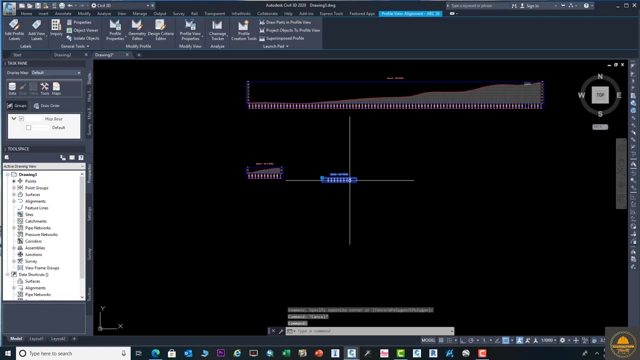 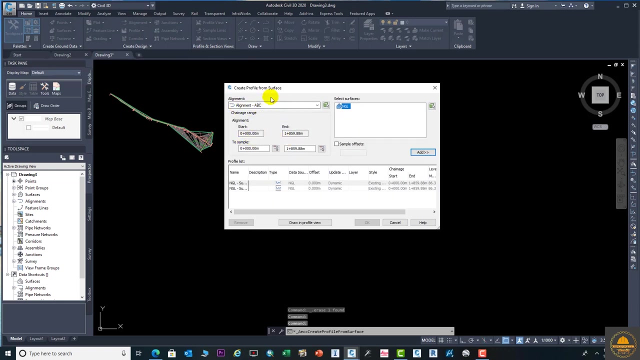 next, next, next, next, now. select your origin. oh, your third baby. sorry, i do a mistake here. okay, let's let let me delete this one, let's delete this one. okay, go again, create surface profile and select from here your third alignment abc. and before i forgot to add the 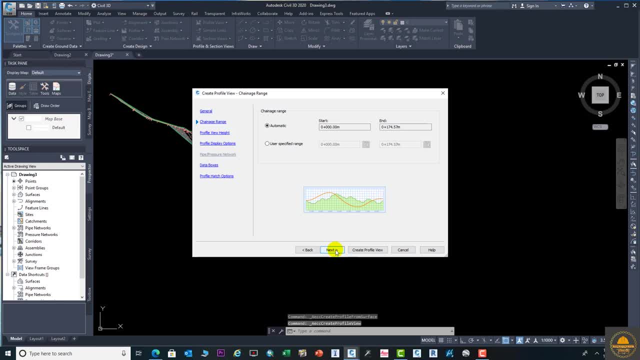 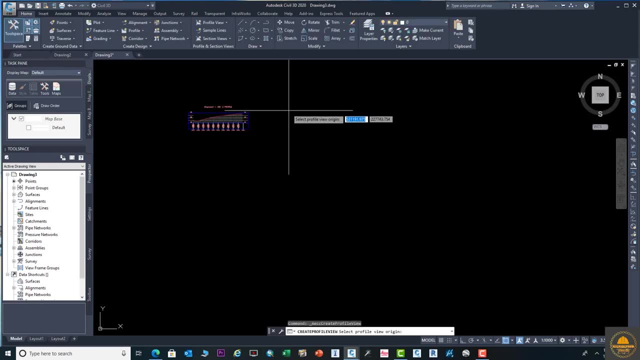 surface engine. don't do a mistake, like me, be careful. next, next, next, create profile. okay, very good, click here. no, your profile is done very well. you are three profile and three alignment is done very well. okay, i hope, guys, from here you understand everything. if anyone you have question, please throw a comment or question and comment. 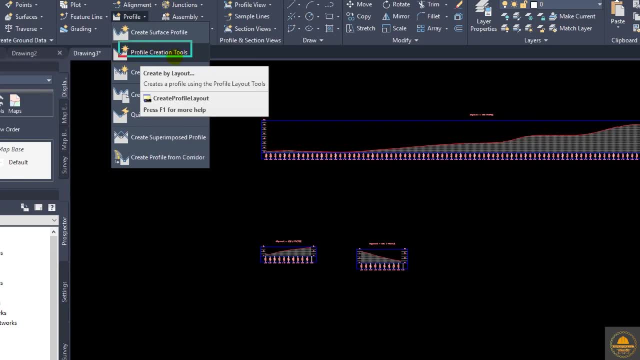 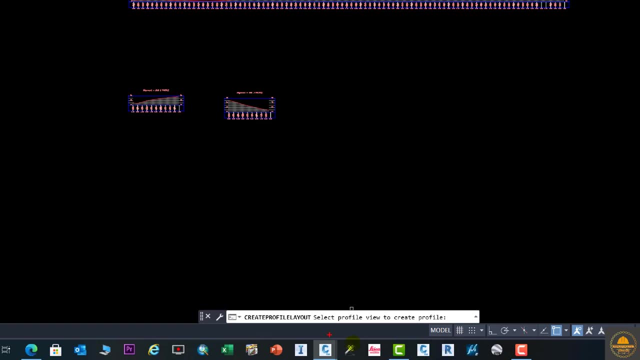 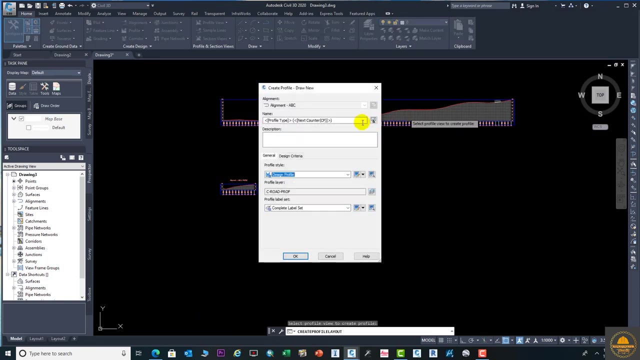 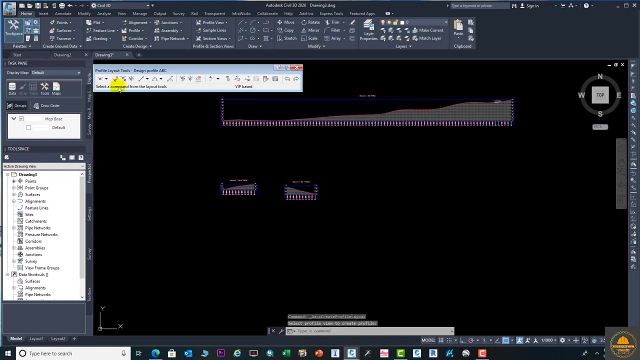 I will try to explain. I will try to explain. and the next: you can see we are going to draw a design profile. okay, select this one. create profile. new profile: okay, DP suppose this is a design profile. you can enter the name. okay, design profile ABC. now you see, profile layout tools is open. you can open this. 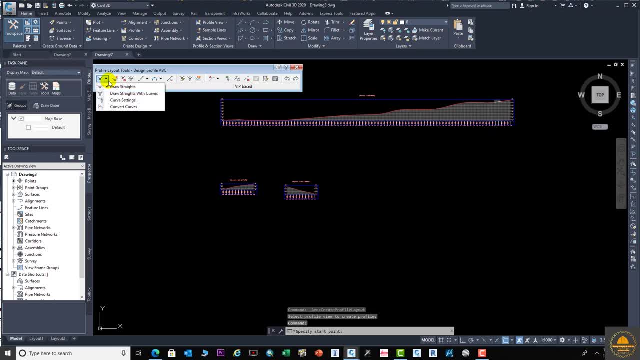 is from the profile profile tools. okay, just come to the draw this one second. okay, just come to the draw this one second. okay, just come to the draw this one second option. draw straight with Karo option. draw straight with Karo option. draw straight with Karo Karo's. okay, just like this one option. 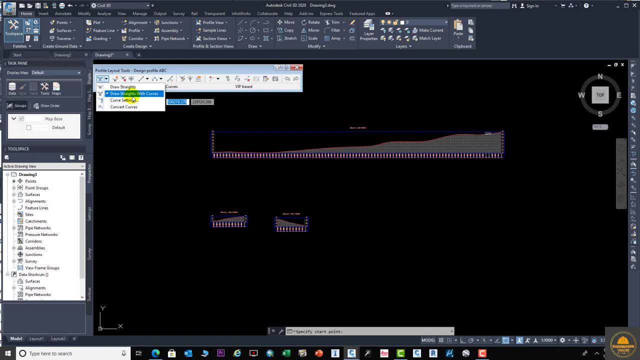 Karo's okay, just like this one option. Karo's okay, just like this one option: Carlos, yes Carlos, or this one. okay, Carlos, yes Carlos, or this one. okay, Carlos, yes Carlos, or this one. okay, now we need to draw our design profile. okay, now we need to draw our design profile. okay. 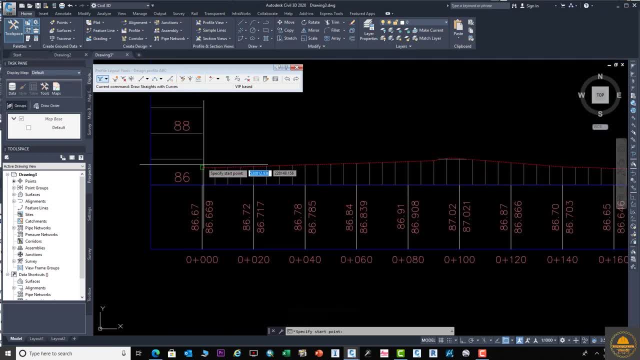 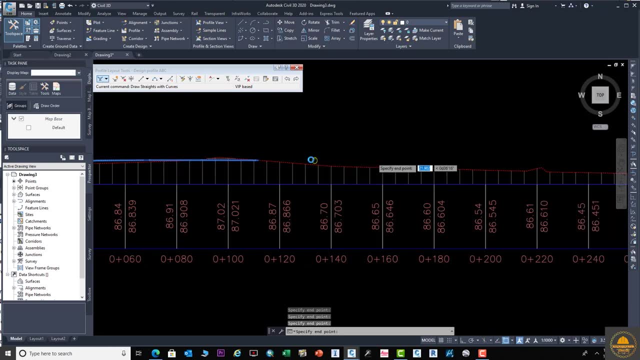 now we need to draw our design profile. okay, sure, our existing profile is drawn. sure, our existing profile is drawn. sure, our existing profile is drawn or draw already. no, this is the design or draw already. no, this is the design or draw already. no, this is the design profile as you need, as your requirement. 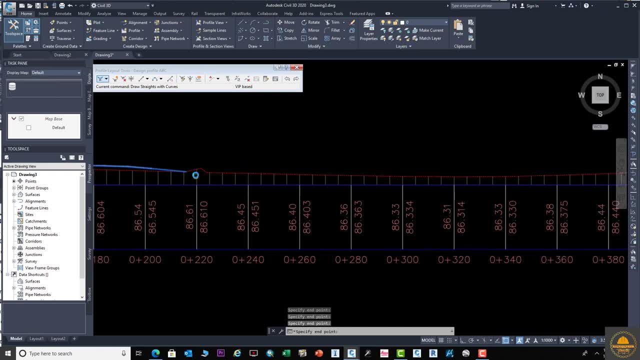 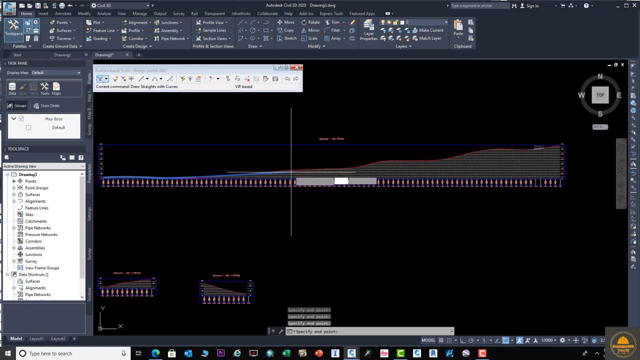 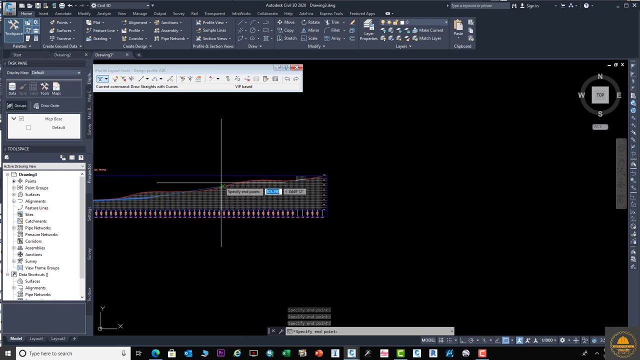 profile as you need as your requirement. profile as you need as your requirement. you can, you can. you can draw this very easily. okay, click, click and click how much cutting. draw this very easily. okay, click, click and click how much cutting. draw this very easily. okay, click, click and click how much cutting, how much feeling you want to do, you can. 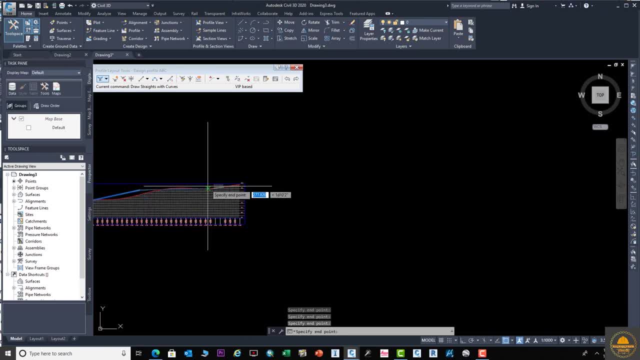 how much feeling you want to do, you can. how much feeling you want to do, you can select this one. this is just example to select this one. this is just example to select this one. this is just example to explain okay and click now you are able. explain okay and click now you are able. 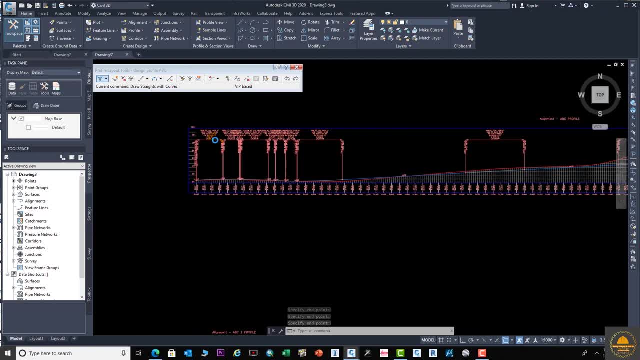 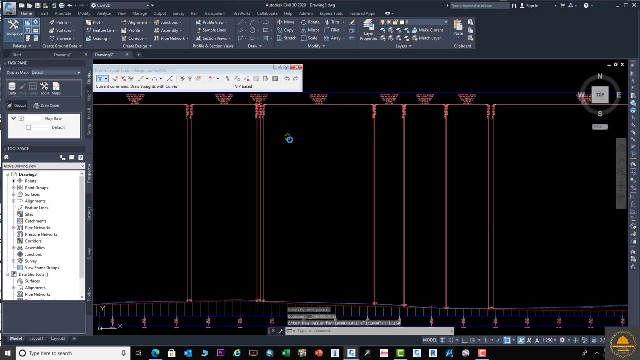 explain. okay, and click. now you are able to see the details here, to see the details here, to see the details here. but, but, but we need to reduce our scale to make it very clear. okay, we need to reduce our scale to make it very clear. okay, we need to reduce our scale to make it very clear. okay, now it's very clear. 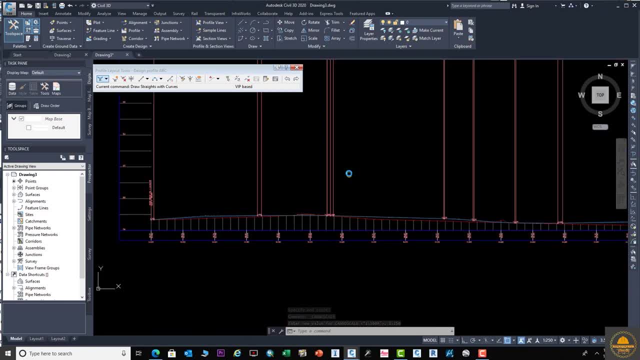 now it's very clear. okay, now it's very clear. okay, now it's very clear. okay, now it's very clear. you can see you can do. now it's very clear, you can see you can do. now it's very clear. you can see you can do some changing from here. 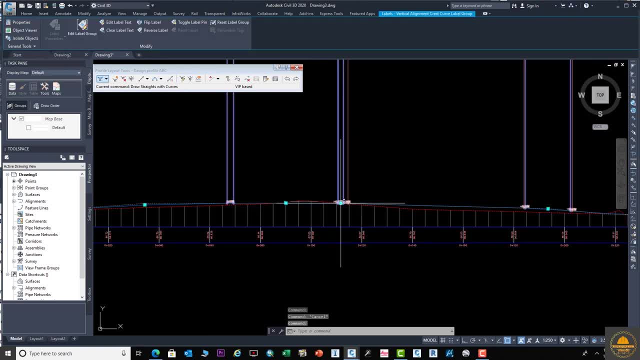 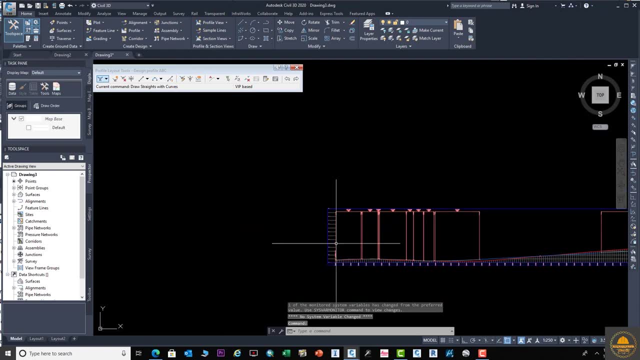 some changing from here, some changing from here with easily you can do changing. if you with easily you can do changing. if you with easily you can do changing. if you want to move here to here, want to move here to here, want to move here to here. okay, 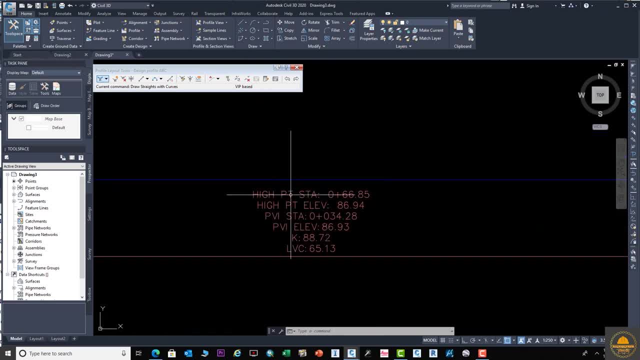 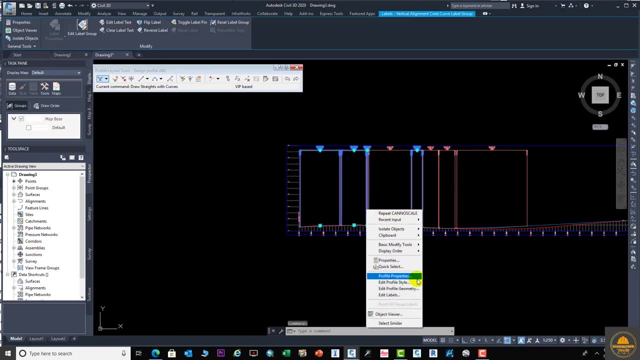 and and, and, and. just let me explain this one here. you can. just let me explain this one here. you can just let me explain this one here. you can see your channel and your K values. each see your channel and your K values. each see your channel and your K values. each details of your profile geometries will. 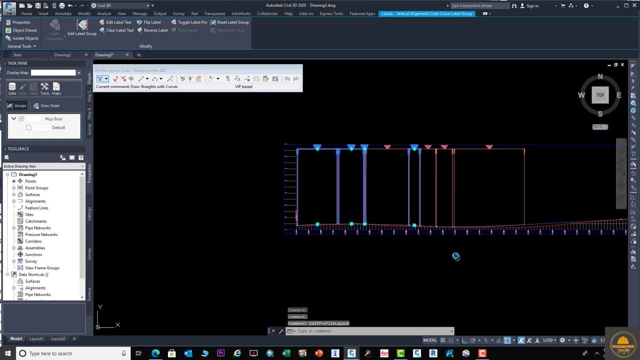 details of your profile geometries. will details of your profile geometries will be displayed here on the top of this. if be displayed here on the top of this. if be displayed here on the top of this. if you need to go to the profile geometry, you need to go to the profile geometry. 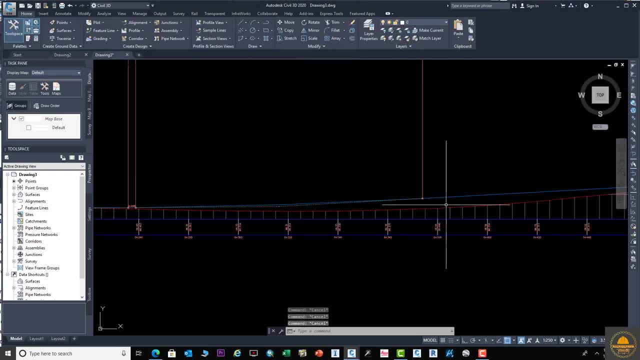 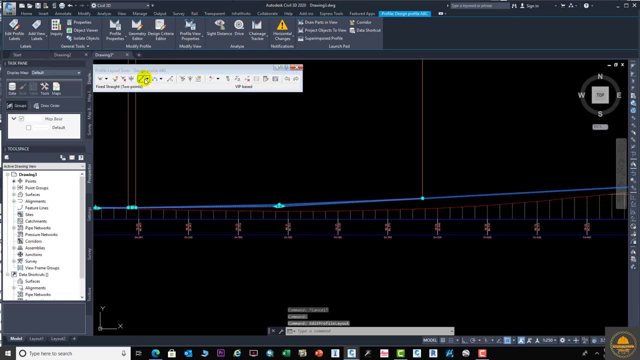 you need to go to the profile geometry. you can select here and this thing is: you can select here and this thing is: you can select here and this thing is common: just go to here and from here you common. just go to here and from here you common. just go to here and from here you can select this one. yeah, this, this. 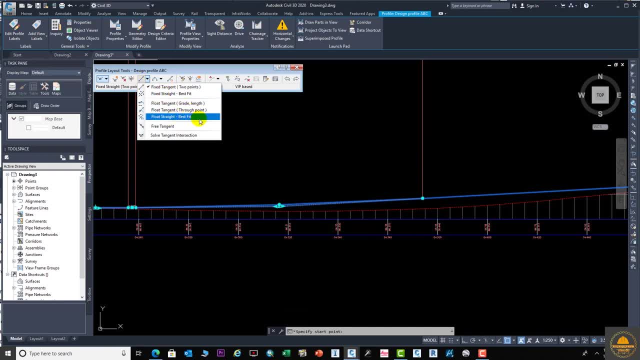 can select this one. yeah, this. this can select this one. yeah, this this regarding the geometry, and from here, if regarding the geometry, and from here, if regarding the geometry, and from here: if you see profile grid view, you can see the. you see profile grid view, you can see the. 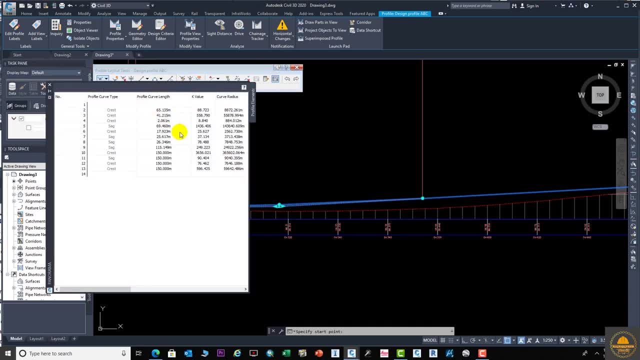 you see profile grid view. you can see the profile grid view and which is your profile grid view and which is your profile grid view and which is your profile curl length and K value. profile curl length and K value. profile curl length and K value- curl radius. you can see this is the 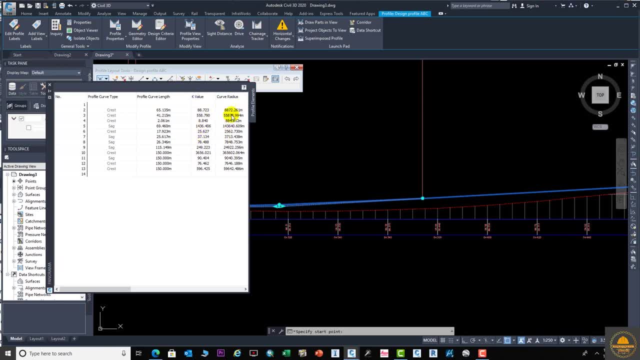 curl radius. you can see. this is the curl radius, you can see. this is the details, okay, and already. which is details okay and already. which is details, okay and already. which is mentioned in the profile, which on the mentioned in the profile, which on the mentioned in the profile, which on the top of each changes. you can see here: 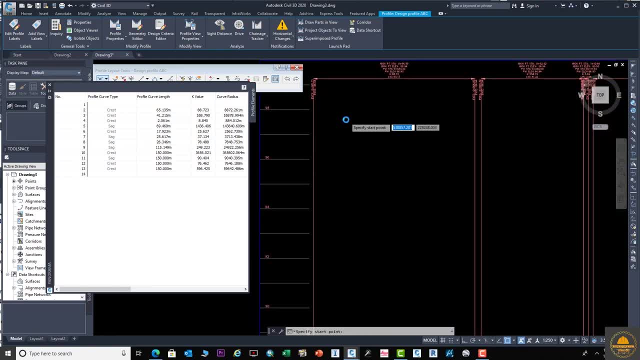 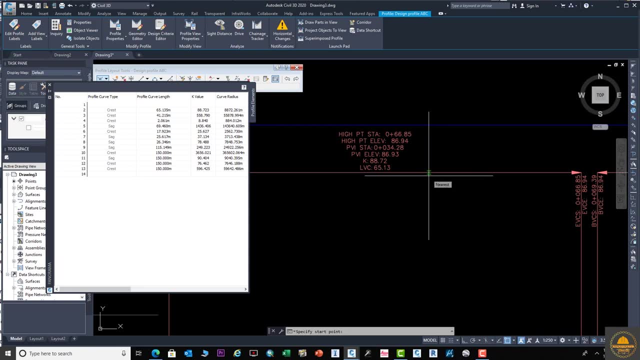 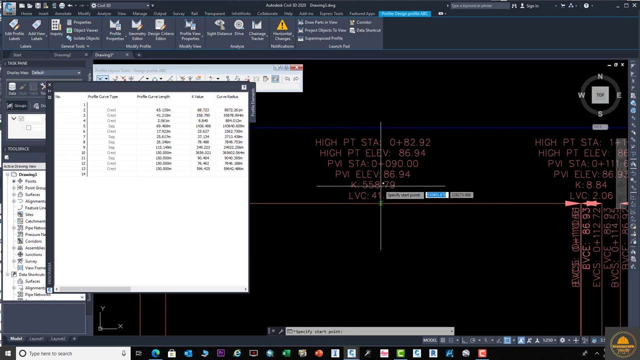 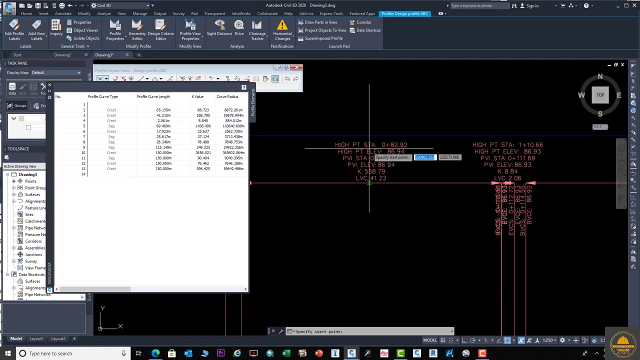 top of each changes. you can see, here, top of each changes. you can see here, here, here, here, here, which everything is the same. this is a which everything is the same. this is a which everything is the same. this is a self-created table for the geometry. self-created table for the geometry. 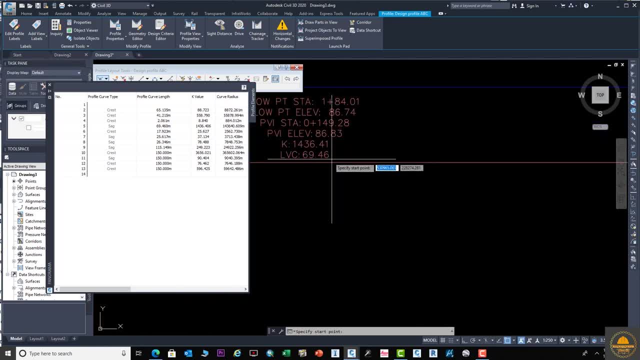 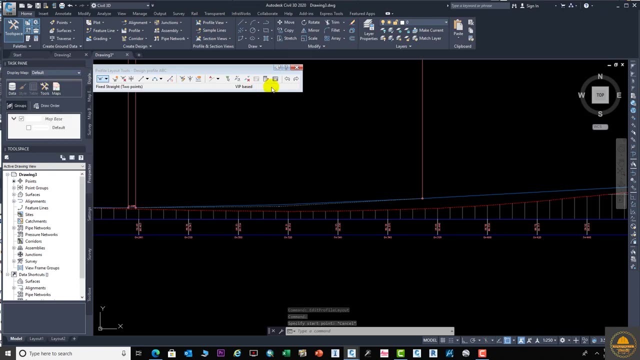 self-created table for the geometry. okay and sake, this is sake and quest. okay and sake, this is sake and quest. okay and sake, this is sake and quest. values okay, values, okay, values, okay. I think you hope you guys understand, I think you hope you guys understand, I think you hope you guys understand regarding these things, and this is: 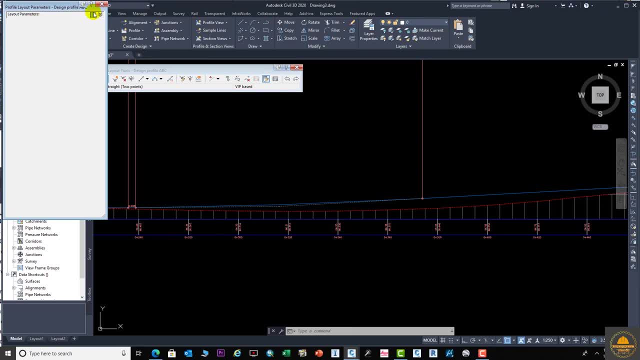 regarding these things, and this is regarding these things, and this is nothing to do. this is a layout. nothing to do. this is a layout, nothing to do. this is a layout. parameters- you can change. you can. parameters you can change. you can. parameters you can change, you can add. this is by itself, but we don't need to. 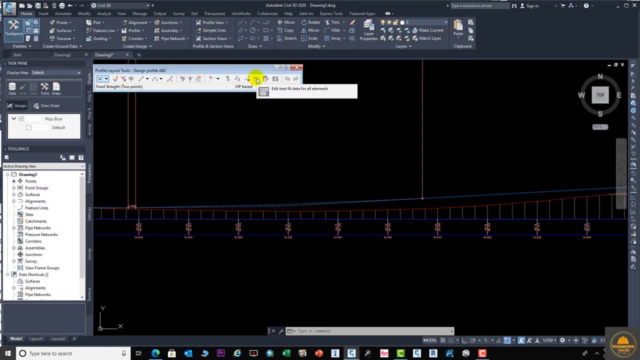 add. this is by itself, but we don't need to add. this is by itself, but we don't need to undo and explain this. I did best fit undo and explain this. I did best fit undo and explain this. I did best fit data. if you have the data, you can add it. 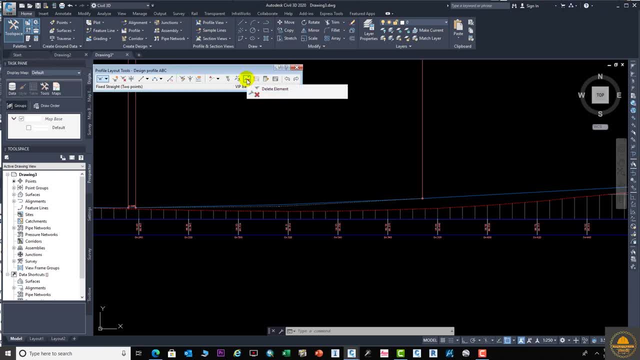 data: if you have the data, you can add it. data: if you have the data, you can add it. and if you need to delete any element. and if you need to delete any element. and if you need to delete any element, you can delete. if you need to extend it. 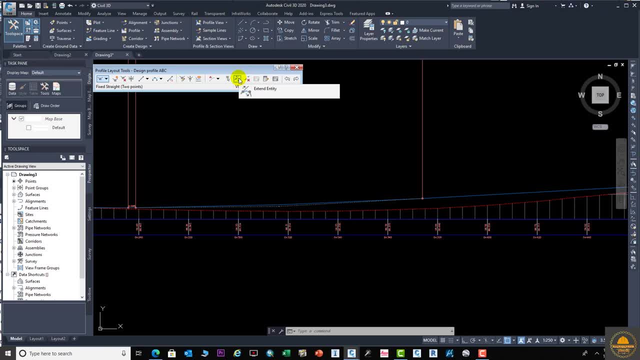 you can delete if you need to extend it, you can delete if you need to extend it. any intensity, you can extend. okay, if you any intensity, you can extend. okay, if you any intensity, you can extend. okay, if you go to this next option, select VIP. and go to this next option, select VIP. and. 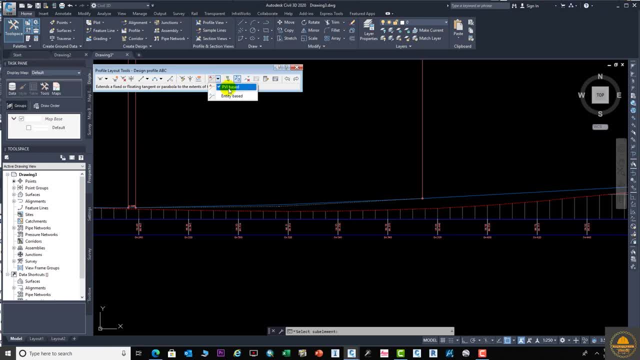 go to this next option, select VIP and from here you can select PV I based and from here you can select PV I based and from here you can select PV I based and entity based, and from here this option entity based and from here this option entity based and from here this option. you can see. copy profile: you can copy. 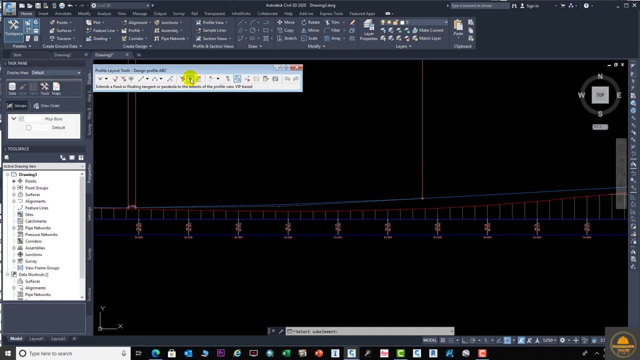 you can see copy profile. you can copy. you can see copy profile. you can copy your profile from this option. you can your profile from this option. you can your profile from this option. you can check your VIP rice alone. okay, and this. check your VIP rice alone. okay, and this. 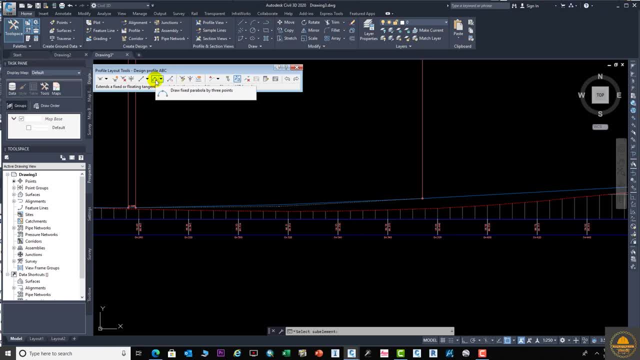 check your VIP rice alone. okay, and this one is option graphics points which you one is option graphics points which you one is option graphics points which you need to if you want to mix and draw any need to. if you want to mix and draw any need to. if you want to mix and draw any points fixed, you can draw. 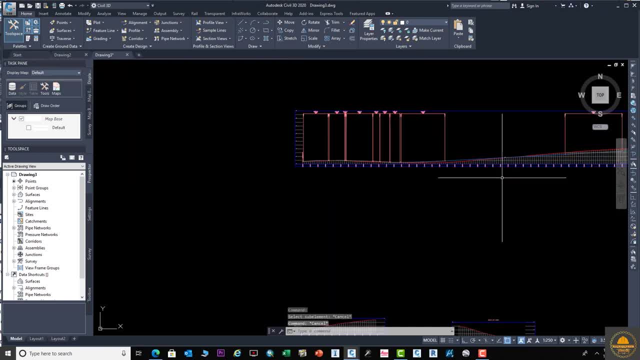 points fixed. you can draw any points fixed. you can draw any and we need to close this one. I hope you and we need to close this one. I hope you and we need to close this one. I hope you guys just understand these things. the guys just understand these things. the. 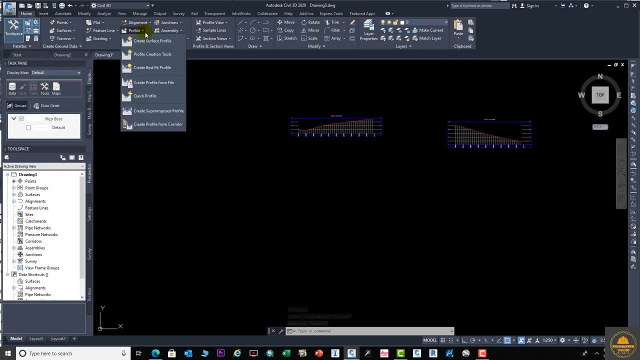 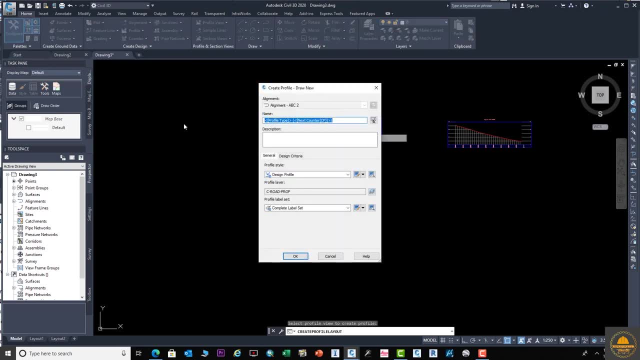 guys just understand these things. the same thing, the same design profile will same thing, the same design profile will same thing, the same design profile will be created in this. go to this profile. be created in this. go to this profile. be created in this. go to this profile and select the profile data and give to. 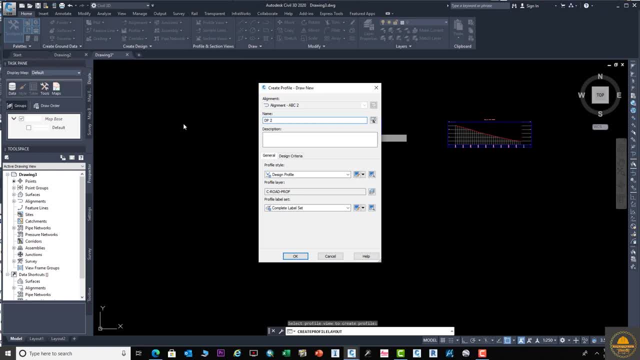 and select the profile data and give to. and select the profile data and give to the DP to create again: same okay, and go the DP to create again- same okay, and go the DP to create again- same okay, and go to this option. select the second one to this option. select the second one. 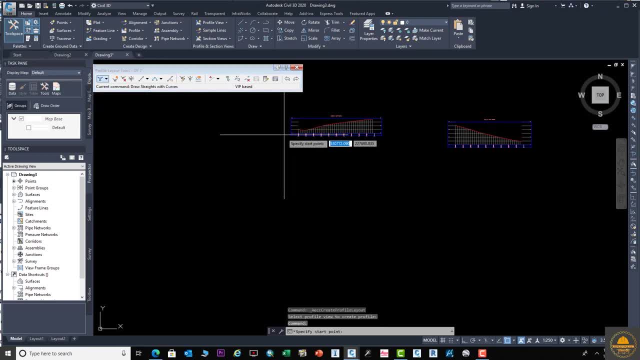 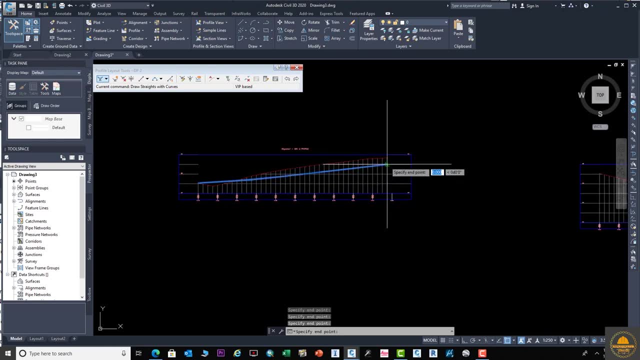 to this option. select the second one with curl, and click where you need the with curl and click where you need the with curl and click where you need the option okay, click, click and click. okay. option okay, click, click and click okay. option okay, click, click and click. okay. so go to the other one we need to draw. 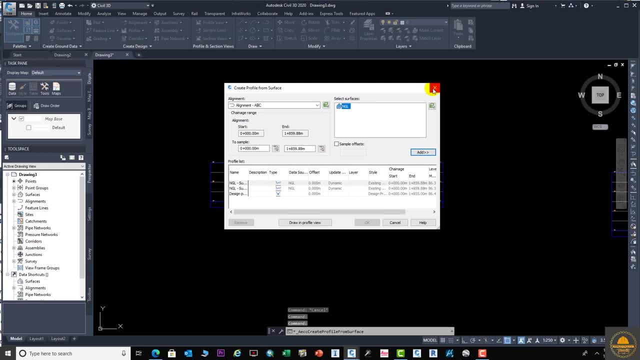 so go to the other one. we need to draw, so go to the other one. we need to draw the same profile. another. so we go to the the same profile another. so we go to the the same profile another. so we go to the profile and select profile creation. 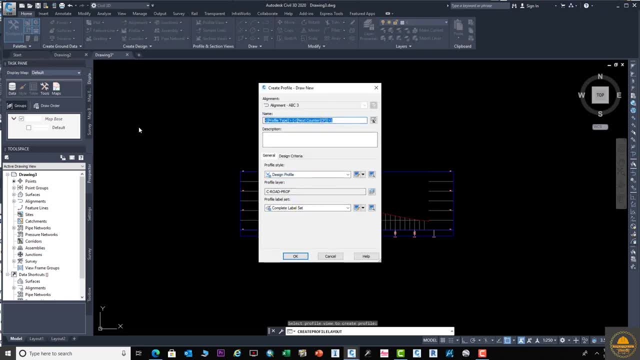 profile and select profile creation. profile and select profile creation. tools. just give the name here: DP. I think tools just give the name here: DP. I think tools just give the name here: DP. I think this one is thought: yeah, this one is. this one is thought: yeah, this one is. 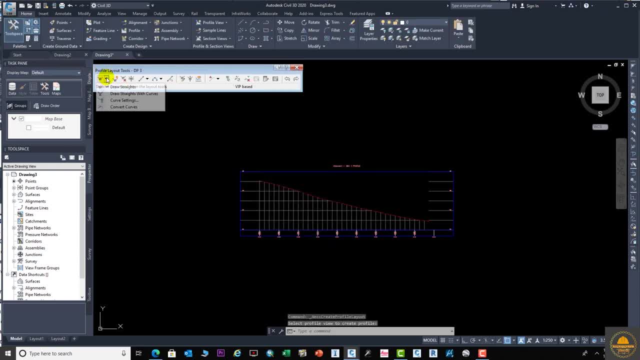 this one is thought. yeah, this one is thought. go to the same option and we need thought. go to the same option and we need thought. go to the same option and we need to draw on the ABC 3 to the same option and we need to draw on the ABC 3. 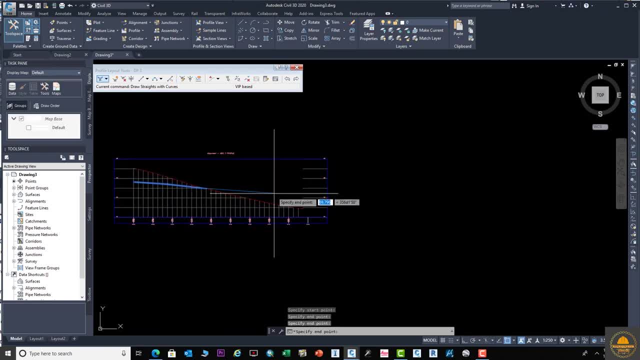 to the same option and we need to draw on the ABC 3 profile. okay, click here and click profile. okay, click here and click profile. okay, click here and click here. sometime you need to see if there is here. sometime you need to see if there is here. sometime you need to see if there is much cutting and filling. you need to. 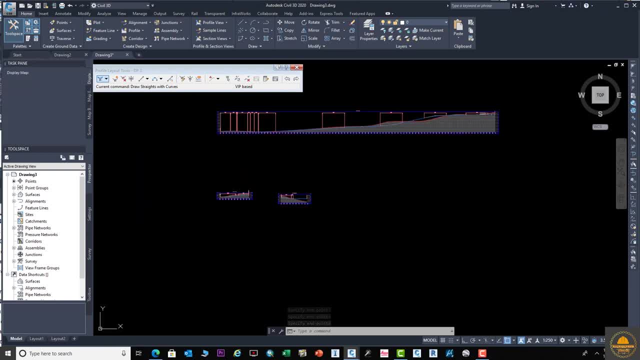 much cutting and filling. you need to much cutting and filling. you need to maintain. suppose if you need fillings, you maintain. suppose if you need fillings, you maintain. suppose if you need fillings you need to maintain your cutting, then need to maintain your cutting, then need to maintain your cutting, then your current cutting material will be go. 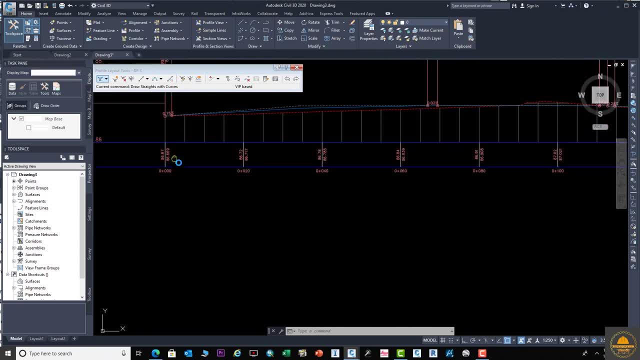 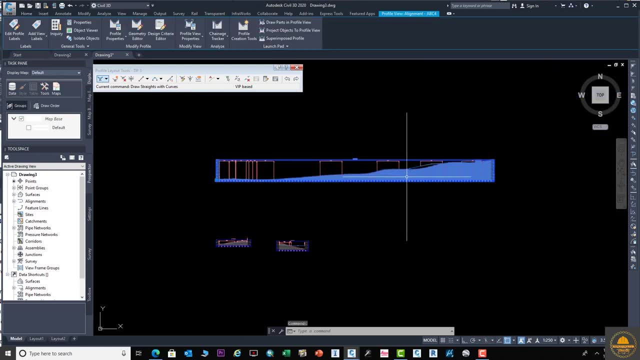 your current cutting material will be go. your current cutting material will be go inside your project. this thing is very inside your project. this thing is very inside your project. this thing is very common. try to understand, suppose you common. try to understand. suppose you common. try to understand. suppose you, and you need to try to do this up to 25. 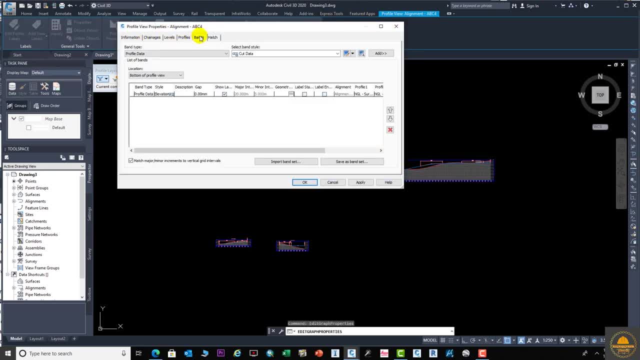 and you need to try to do this up to 25. and you need to try to do this up to 25 to 30 filling. so it should be going good to 30 filling. so it should be going good to 30 filling. so it should be going good. okay, now something is we need to change. 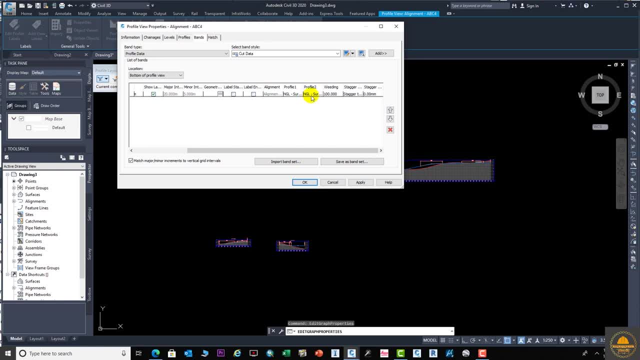 okay, now something is we need to change. okay, now something is: we need to change the levels. we have the same levels in the levels. we have the same levels in the levels. we have the same levels in the bands profile: one is the same and the bands profile: one is the same and. 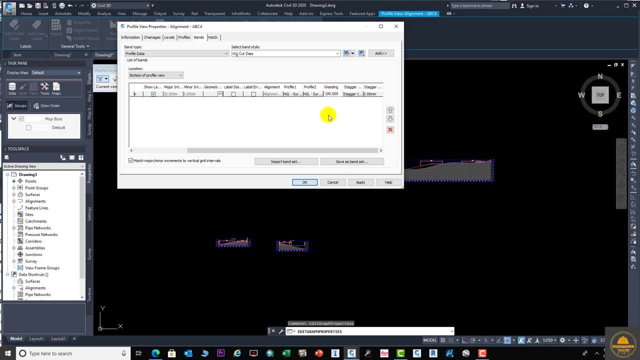 the bands. profile one is the same and also profile two is the same. we need to also: profile two is the same. we need to also: profile two is the same. we need to change in the profile one. we need to change in the profile one. we need to. 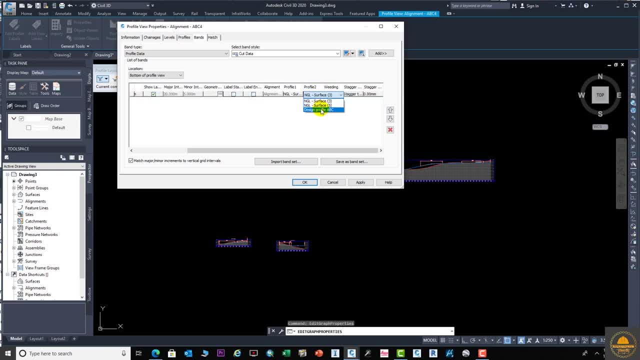 change in the profile one. we need to select the NGL and the profile to. we select the NGL and the profile to. we select the NGL and the profile to. we need to select the design level. okay, so, need to select the design level, okay, so. 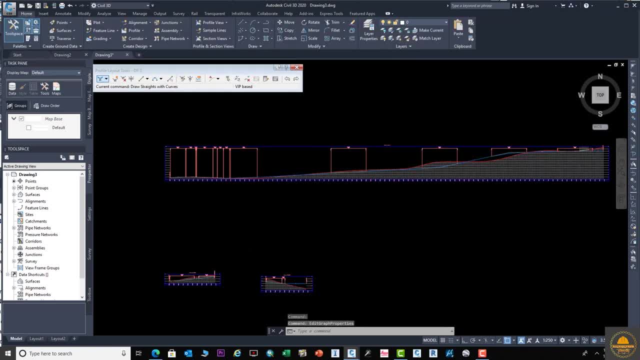 need to select the design level. okay, so now you can see the levels will be. now you can see the levels will be. now you can see the levels will be definitely change and you can see these definitely change and you can see these definitely change and you can see these things. okay, you can see no, before is the. 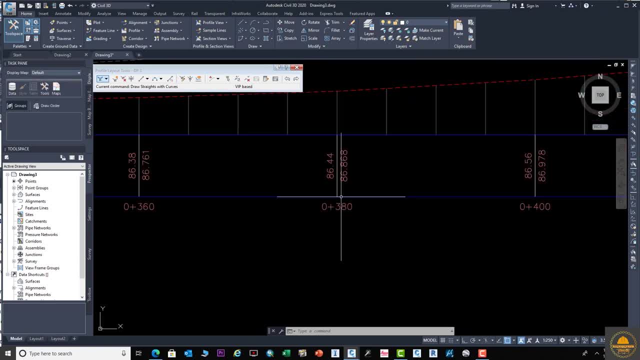 things okay? you can see no. before. is the things okay? you can see no. before is the same. the hair is shown only the NGL. same the hair is shown, only the NGL. same the hair is shown only the NGL loads. but now we change from the band. 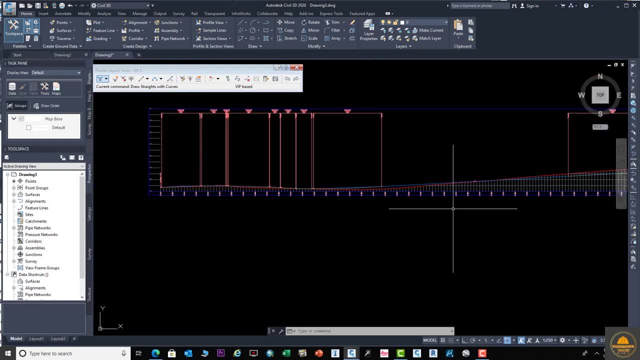 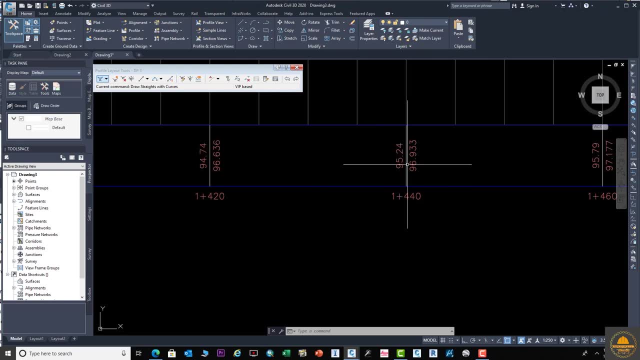 loads. but now we change from the band loads. but now we change from the band. setting now the levels is changed. setting now the levels is changed. setting now the levels is changed already nine five point two, nine three already nine five point two, nine three already nine five point two, nine three, and the band is no shown for the those. 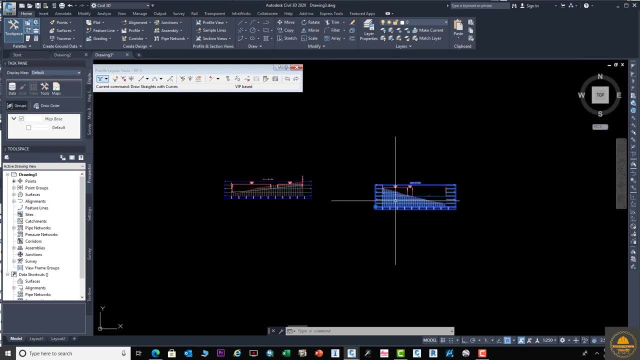 and the band is no shown for the those and the band is no shown for the those. this one is also. you do the same. this one is also. you do the same. this one is also. you do the same process. go to profile view properties process. go to profile view properties. 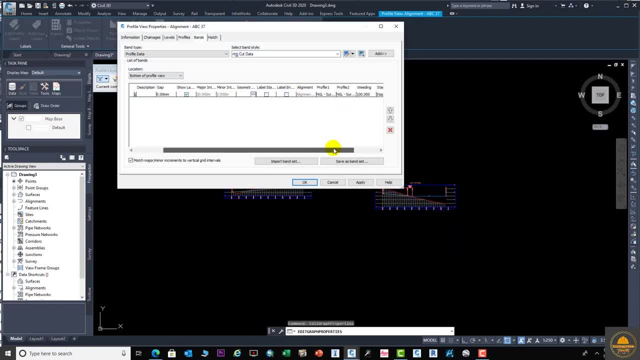 process. go to profile view properties and from here you can change for the and from here you can change for the and from here you can change for the profile one and profile two. you can profile one and profile two. you can profile one and profile two. you can change in the profile one a set angel. 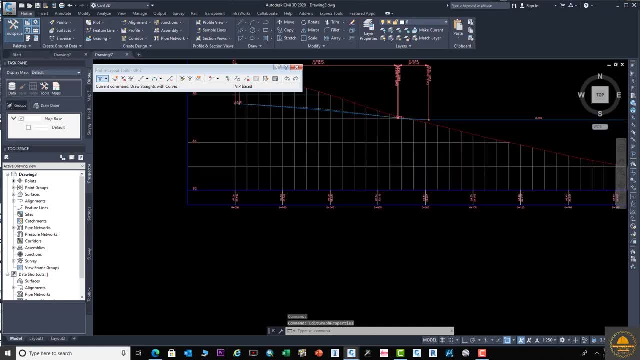 change in the profile. one a set angel. change in the profile. one a set angel and the other one is you can set the and the other one is you can set the and the other one is you can set the other one design level. then you can see. 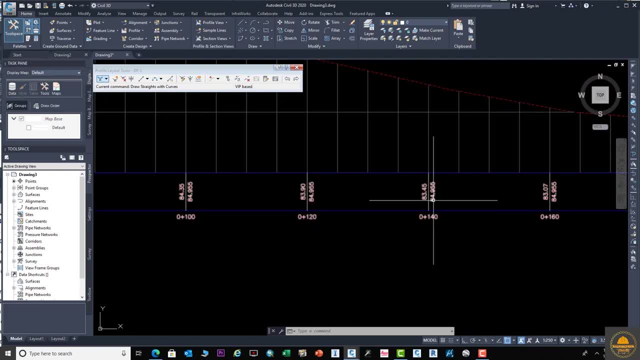 other one design level, then you can see other one design level, then you can see level is change and do also same for level is change and do also same for level is change and do also same for this. just click here and right click. and this: just click here and right click and 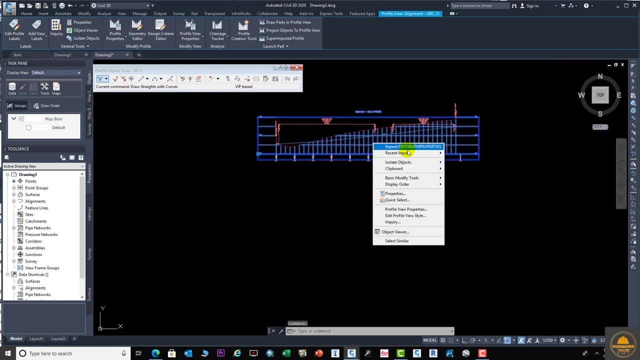 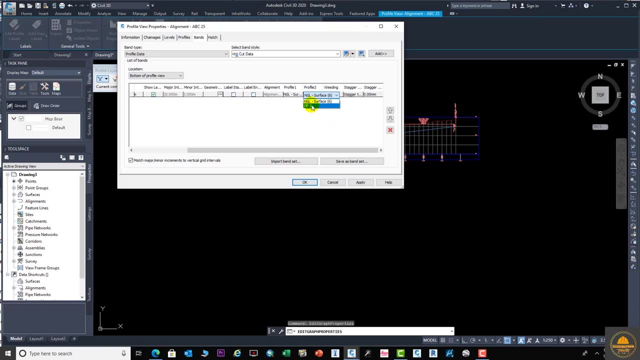 this: just click here and right click and go to file review properties and go to go to file review properties and go to go to file review properties and go to this option and change here the design- this option- and change here the design- this option- and change here the design. okay, now you can see your all level is. 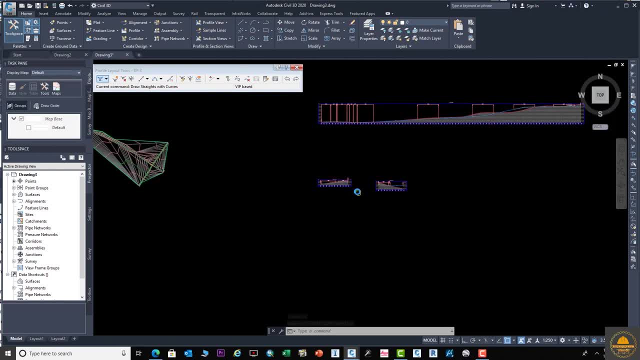 okay, now you can see your all level is okay. now you can see your all level is. change in the band: you will be see able change in the band. you will be see able change in the band. you will be see able to to change in the band. you will be see able to see the existing ground levels and 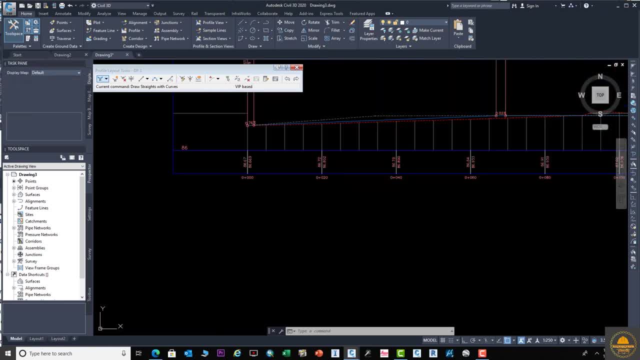 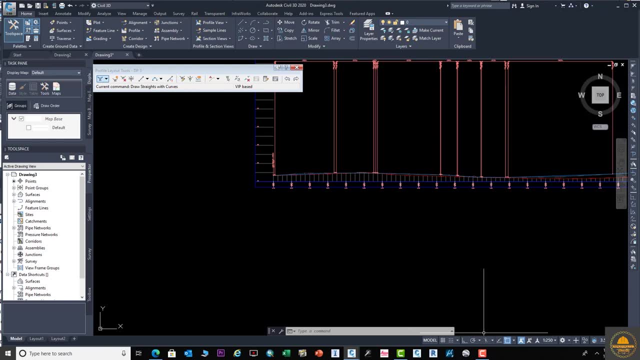 see the existing ground levels. and see the existing ground levels and there is nine level. okay, later in next. there is nine level. okay, later in next. there is nine level. okay, later in next. steps will explain bands now you need to. steps will explain bands now you need to. 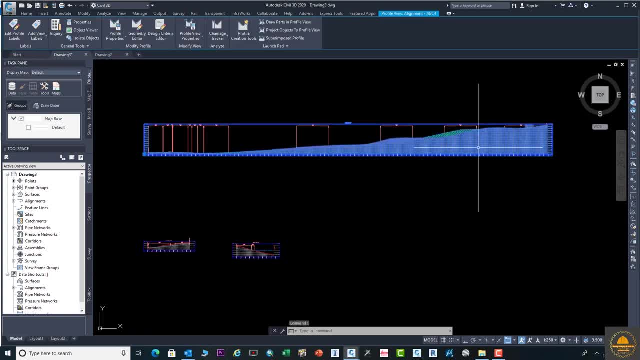 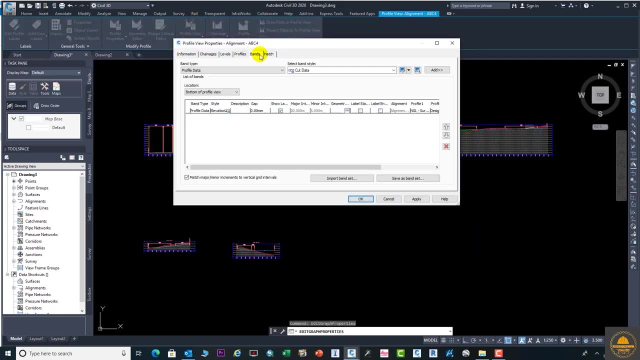 steps will explain bands now. you need to go to select profile view properties. go to select profile view properties. go to select profile view properties. okay, go to the band we need to go to. okay, go to the band we need to go to. okay, go to the band. we need to go to eight or on bands. but for this purpose 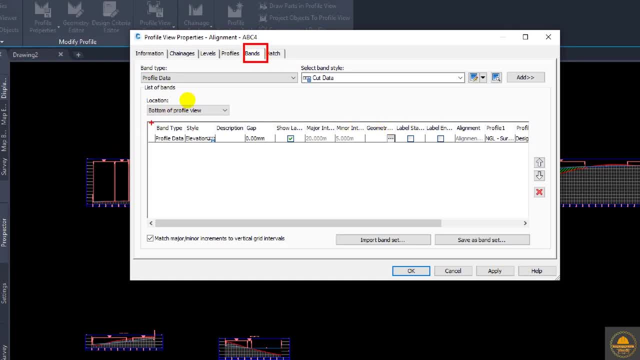 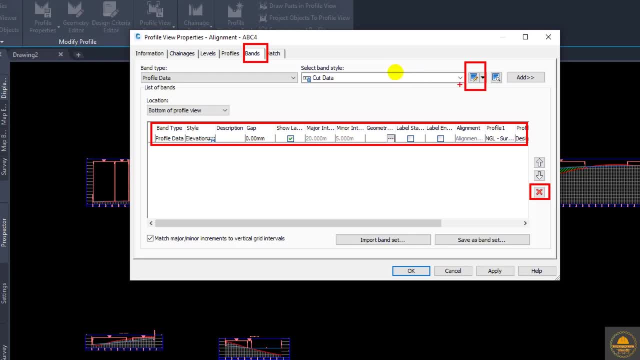 create our own bands. this is very: create our own bands. this is very important section. okay, if once you learn important section. okay, if once you learn important section, okay, if once you learn how to create your own bands, you can. how to create your own bands, you can. 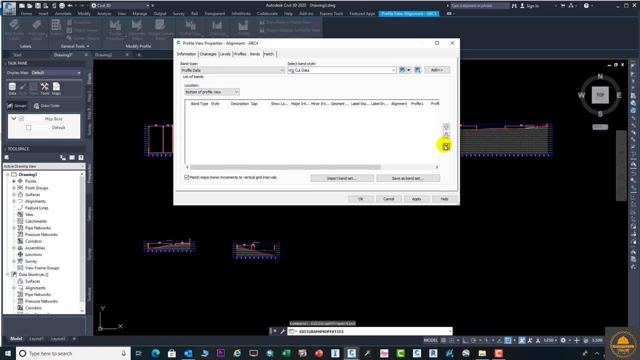 how to create your own bands. you can able to do all know you can see, or a able to do all know you can see, or a able to do all know you can see. or a current or a default band is no delete. current or a default band is no delete. 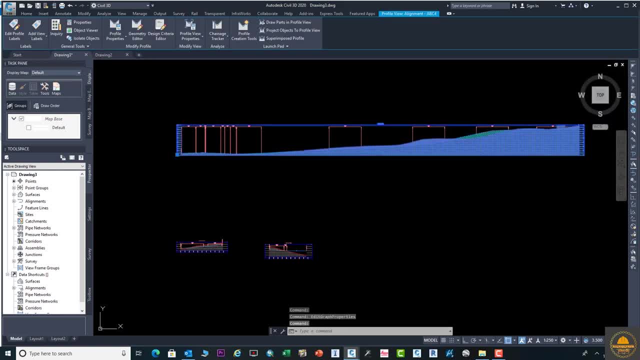 current or a default band is no, delete it. okay, go to this option, and from here it okay, go to this option, and from here it okay. go to this option, and from here you need to just focus. I want to zoom. you need to just focus, I want to zoom. 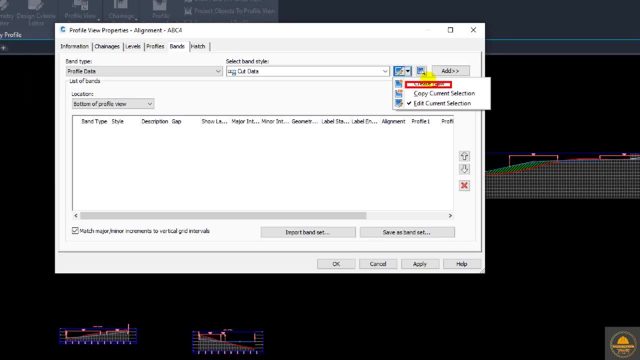 you need to just focus. I want to zoom it and create new. okay, go to this, create it and create new. okay, go to this, create it and create new. okay, go to this, create new. and this will- this is a little bit new and this will- this is a little bit. 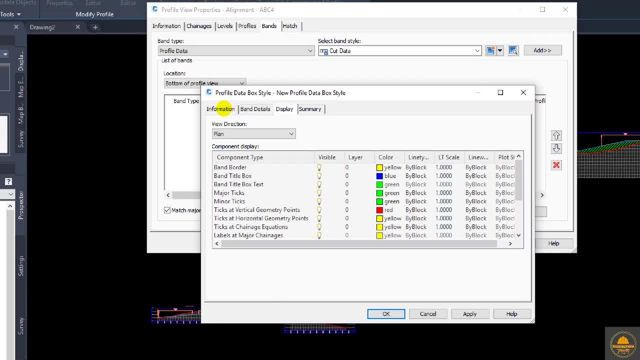 new and this will. this is a little bit complicated, but once you focus on this, complicated, but once you focus on this, complicated, but once you focus on this series one, you can easily understand it. series one: you can easily understand it. series one: you can easily understand it. go to the information here you need to. 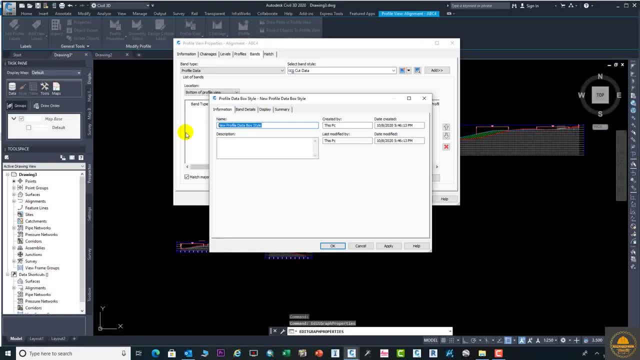 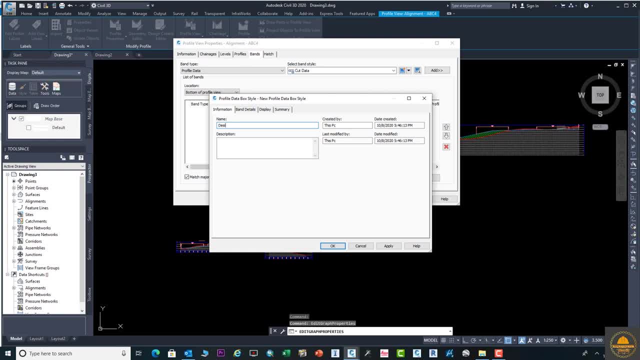 enter the design: okay design. just select this one and copy: okay. go to okay design. just select this one and copy: okay, go to okay design. just select this one and copy: okay. go to this option main details and this option main details. and this option main details. and here is you can see this is composed. 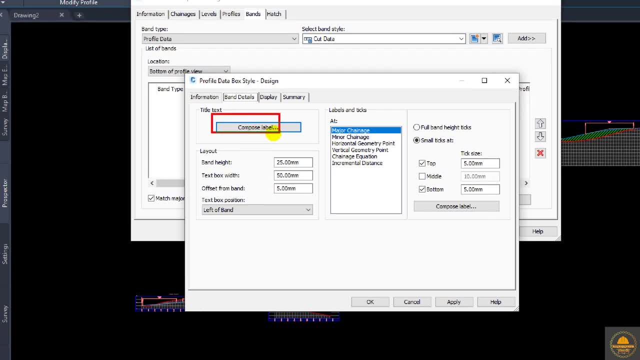 here is you can see this is composed. here is: you can see this is composed level. you need to go to the compose level. you need to go to the compose level. you need to go to the compose table. okay, and here is also composed table. okay, and here is also composed. 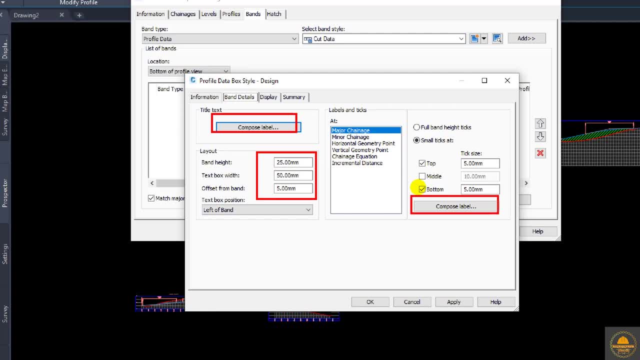 table okay, and here is also composed: never first of all, we need to go to never first of all, we need to go to never first of all. we need to go to this. compose labels, okay, and here we need this. compose labels okay, and here we need this. compose labels okay, and here we need to just control. 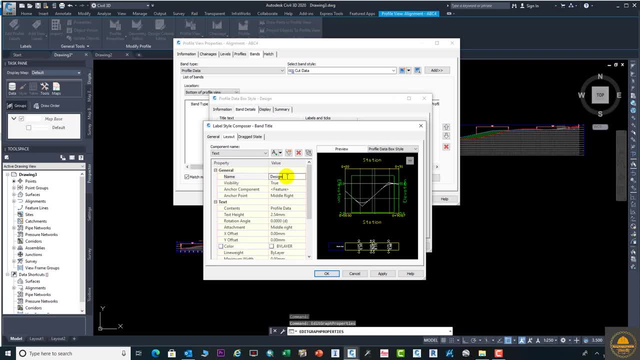 to just control. to just control v. before we copy the name control v: v. before we copy the name control v: v. before we copy the name control v. and from here you can select the options and from here you can select the options and from here you can select the options we need to select. this is middle center. 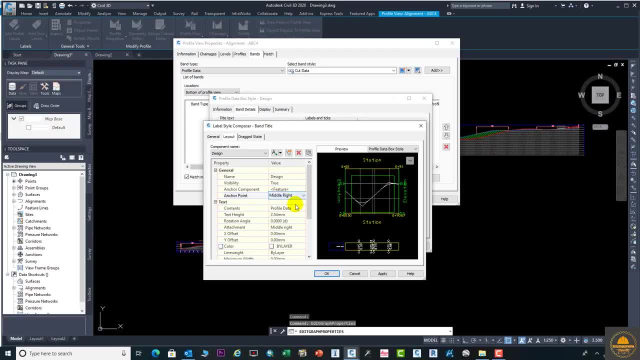 we need to select: this is middle center. we need to select: this is middle center. okay, select this one is middle center. okay, select this one is middle center. okay, select this one is middle center. and here you can enter the height as per. and here you can enter the height as per. 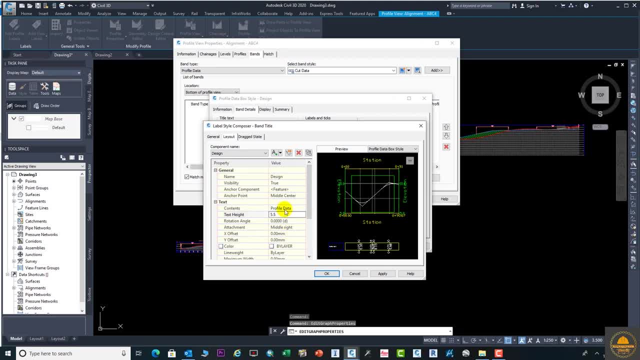 and here you can enter the height as per your requirement. let me just put 5.5 your requirement. let me just put 5.5, your requirement, let me just put 5.5. and also here select middle center and go. and also here select middle center and go. 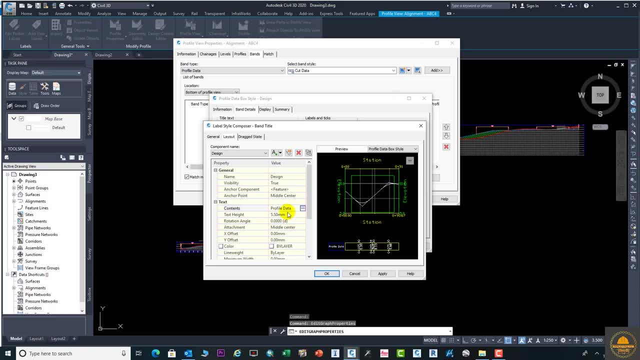 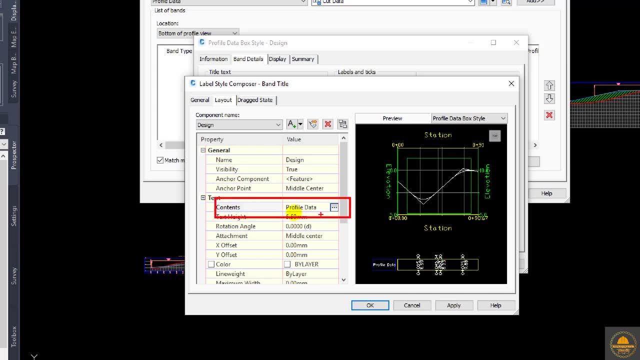 and also here, select middle center, and go to the contents and click on these three to the contents and click on these three to the contents and click on these three: dot, dot, dot. okay, let me click, okay, let me click, okay, let me click and go here, select this one. 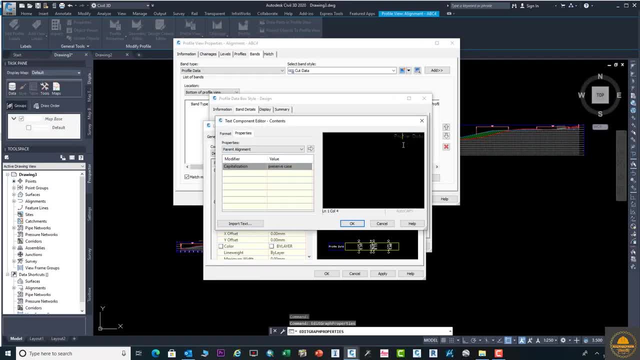 and go here, select this one and go here, select this one. select this all and delete. select this all and delete. select this all and delete. okay and control v. okay and control v. okay and control v, which we copy. this is the name which we copy. this is the name. 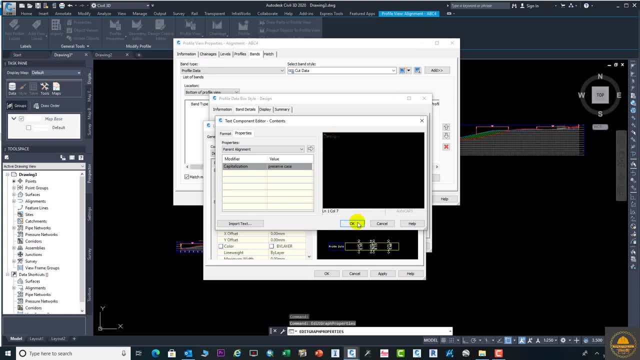 which we copy. this is the name, okay, and from here you can change the color. and from here you can change the color. and from here you can change the color as per your requirement. you can change as per your requirement. you can change as per your requirement. you can change the color. which color? 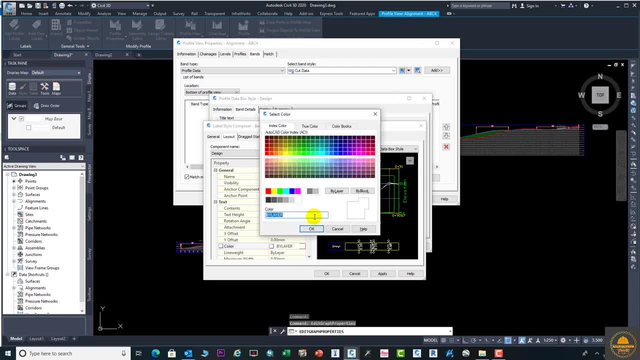 the color? which color? the color, which color do you need? you can change. do you need, you can change? do you need, you can change? and click on and click on and click on. apply and okay. no, your first step is okay. apply and okay. no, your first step is okay. 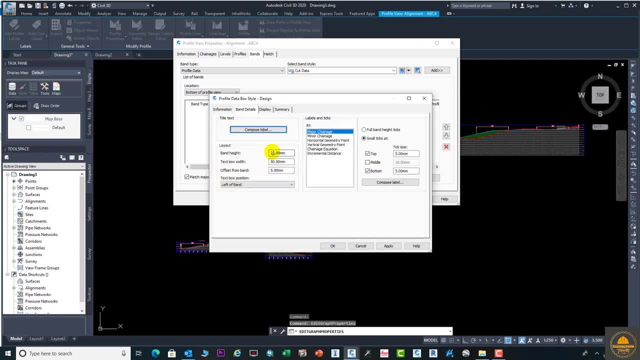 apply and okay, no, your first step is okay, you can see the band height, you can. you can see the band height, you can. you can see the band height. you can select the band height of 50. select the band height of 50. select the band height of 50- 75 as. 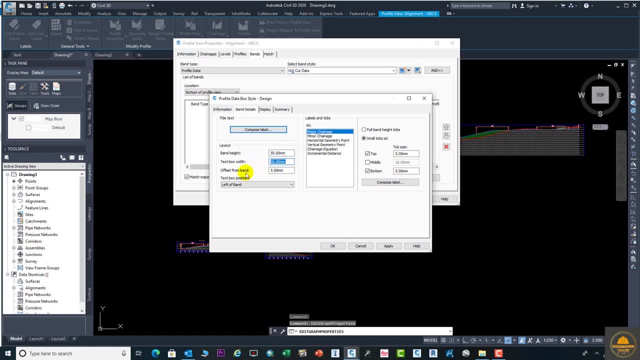 75 as 75, as as much as you need, as much is your, as much as you need, as much is your, as much as you need, as much is your text height. you can select it like that. so text height, you can select it like that, so. 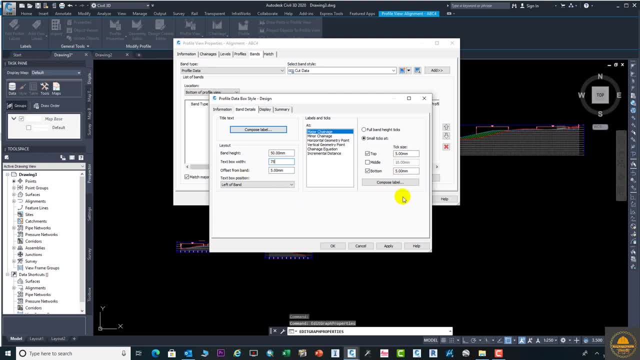 text height. you can select it like that. so let me put this 75 and 50, let me put this 75 and 50, let me put this 75 and 50 and go to the compose label and go to the compose label and go to the compose label. the other one option which i mark initially: 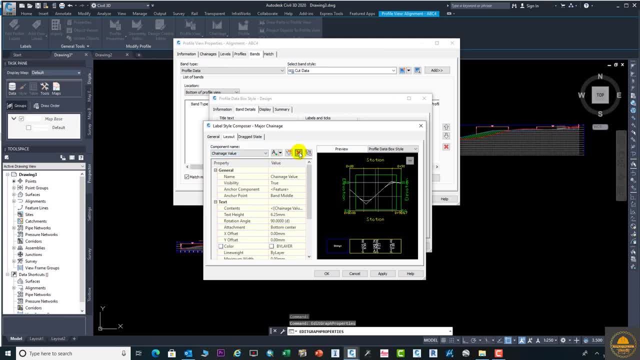 the other one option which i mark initially. the other one option which i mark initially: just delete the first, just delete the first, just delete the first. and control v, which we initially copied, and control v, which we initially copied, and control v, which we initially copied. control v. the design name is display go. 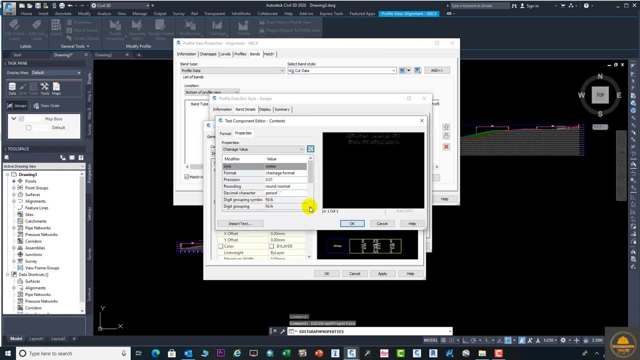 control v. the design name is display: go control v. the design name is display: go to this tree dot. to this tree dot, to this tree dot. this option here, you can see this one. this option here, you can see this one. this option here, you can see this one- contents again the same step which we do. 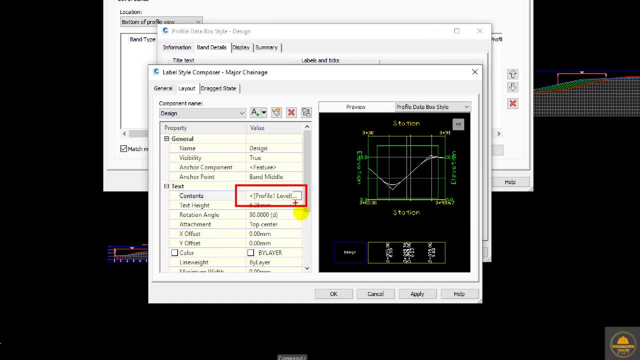 contents- again the same step which we do. contents- again the same step which we do: in for the first compose label option, in for the first compose label option, in for the first compose label option, and just click on this and just click on this and just click on this. it's a little bit complicated. 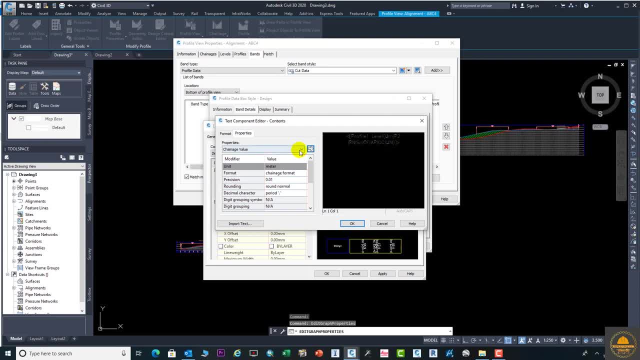 it's a little bit complicated. it's a little bit complicated. you need to just select this one and you need to just select this one, and you need to just select this one and delete this one. delete this one, delete this one and from here you need to select the. 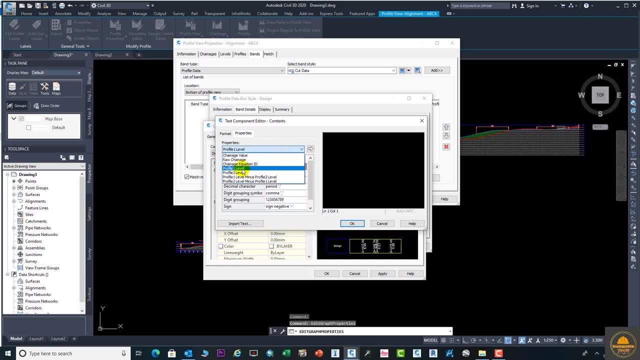 and from here you need to select the and from here you need to select the profile level one, profile level one. profile level one or profile level two, which one you enter? or profile level two, which one you enter? or profile level two? which one you enter in your bands and which? where is your? 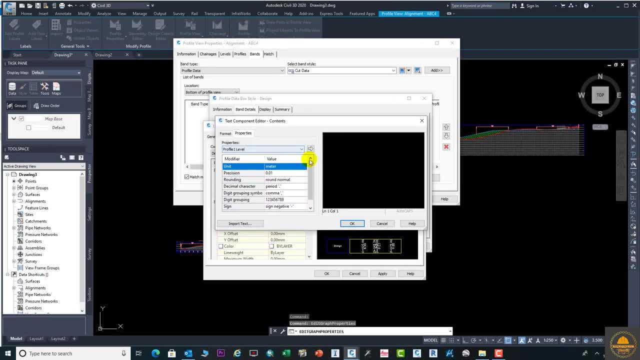 in your bands, and which, where is your in your bands? and which, where is your design? because we are going to design, because we are going to design, because we are going to explain the design level. so explain the design level. so explain the design level. so click on this arrow button. 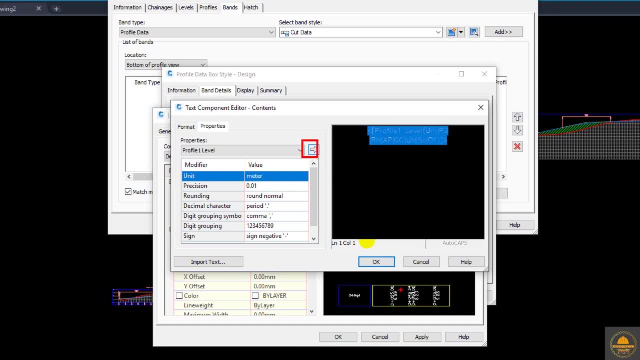 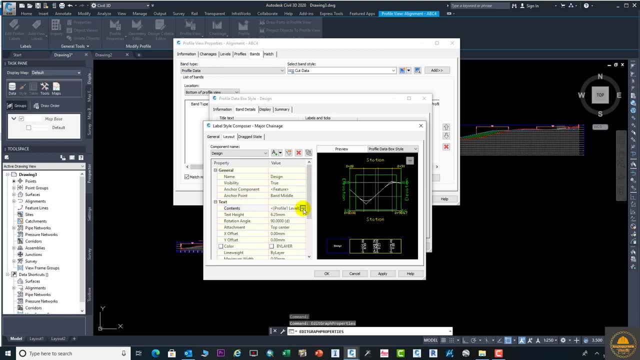 click on this arrow button, click on this arrow button and click ok, okay, go here. okay, go here. okay, go here. and here select the option. and here select the option and here select the option: delete this, delete this, delete this and and and arrow arrow arrow button button. 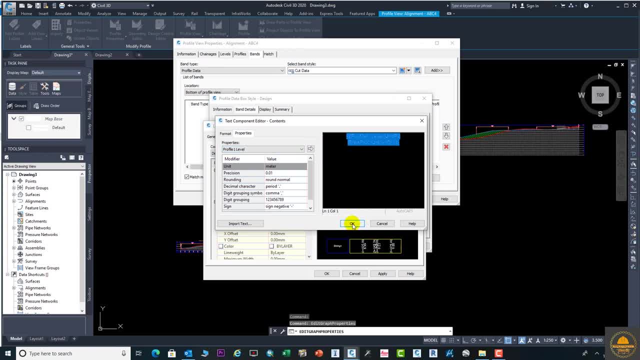 button. okay, okay, okay, and from here you can select, and from here you can select, and from here you can select this option. how much of the point you need this option? how much of the point you need this option? how much of the point you need the digit two, three or four. 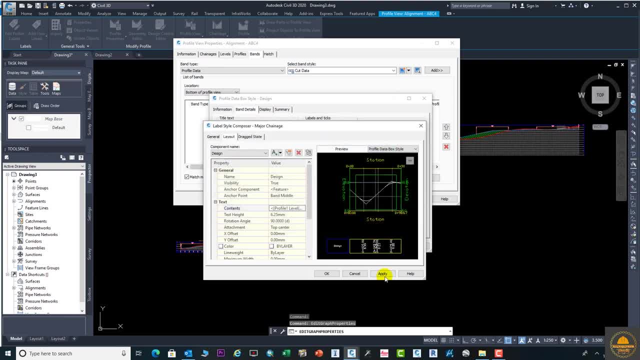 the digit two, three or four. the digit two, three or four. it should be provide to you. it should be provide to you. it should be provide to you. okay, click here you can select colors. okay, click here you can select colors. okay, click here you can select colors and click on apply. 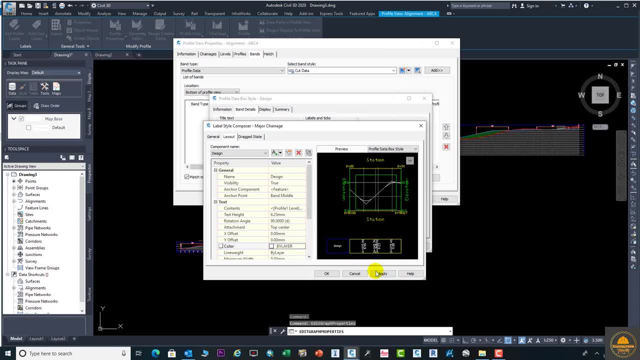 and click on apply, and click on apply, and okay, and okay, and okay, and and okay, and here you can select text height. here you can select text height. here you can select text height by end. okay, by end, okay, by end. okay. now we need to go to display. now we need to go to display. now we need to go to display to turn on some layers from here. we need to turn on some layers from here. we need to turn on some layers from here. we need to to turn on some layers from here, we need to. 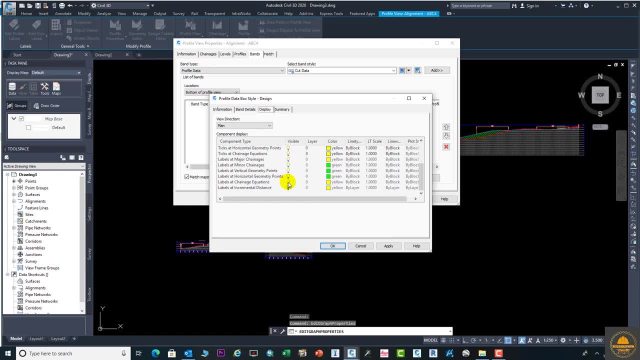 to turn on some layers from here we need to turn off, turn off, turn off some unnecessary layers, some unnecessary layers, some unnecessary layers. suppose we need to turn off this all. suppose we need to turn off this all. suppose we need to turn off this all and we need to turn on this one. 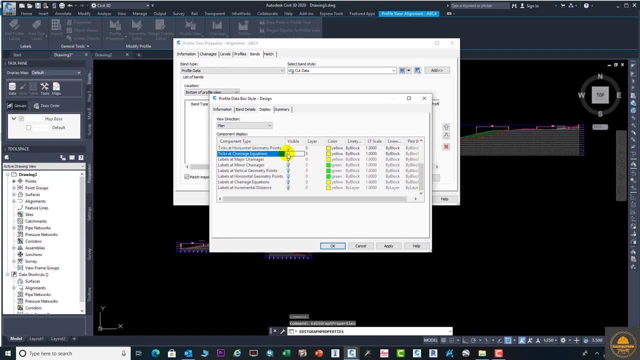 and we need to turn on this one and we need to turn on this one: the major tick, and here this four start the major tick and here this four start: band, border, brand title and major ticks. we need to turn on this and one, this one, so need to apply. 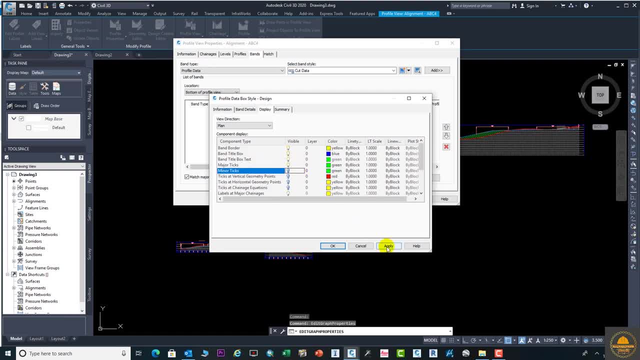 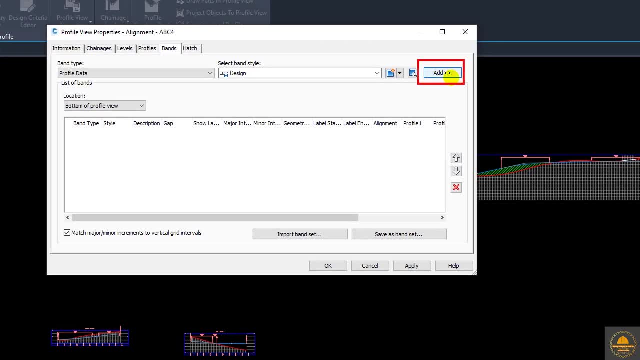 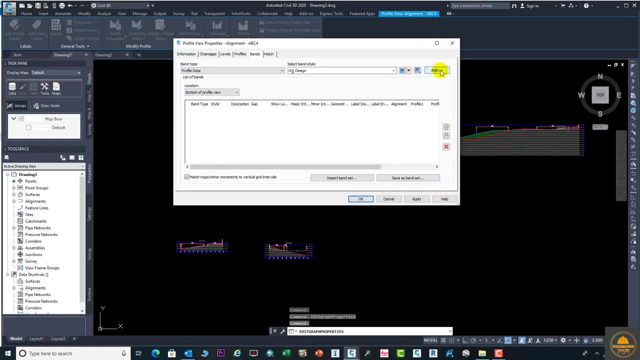 and okay. from here you need to add: uh, this option, our band is ready, just we need to add in our profile and apply, and okay. so let me just add from here and you need to put this okay and apply, and okay. now you can see your band is added to your profile. now your first design band is ready, okay, 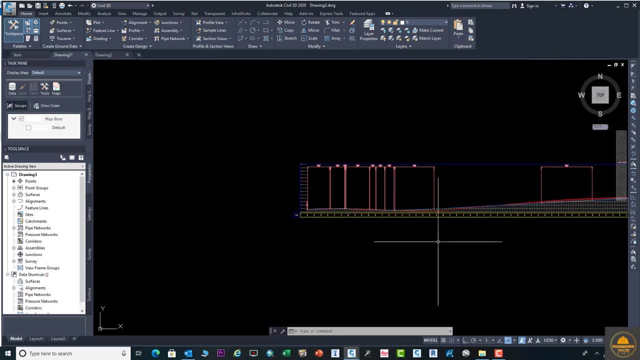 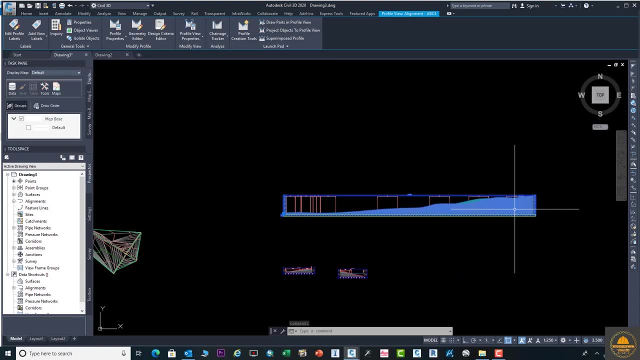 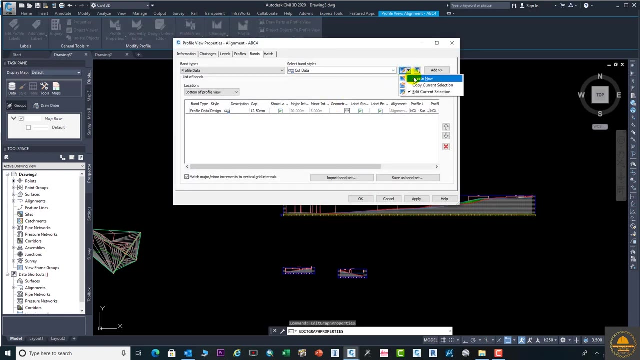 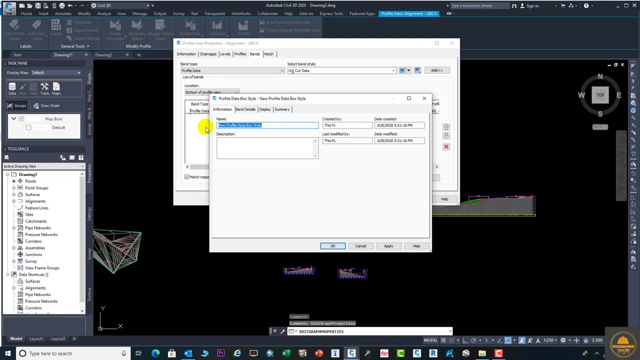 sorry, now we need to click again and need to add our next existing band. go to the same procedure- profile properties- and from here you need to select create new and here go to the information and enter the name of band. suppose we need to enter. this is existing band, so copy this name later. if you copy, it's very easy. 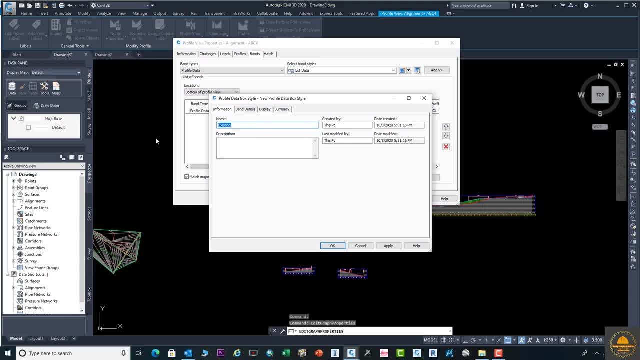 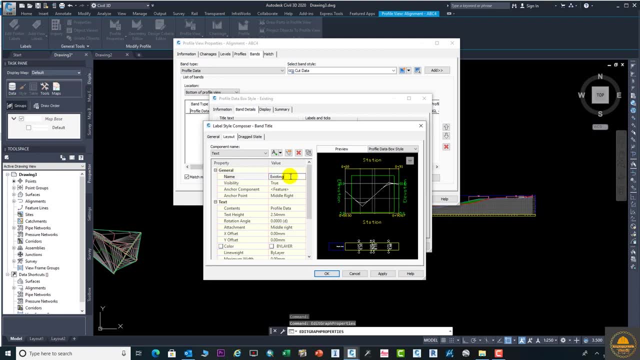 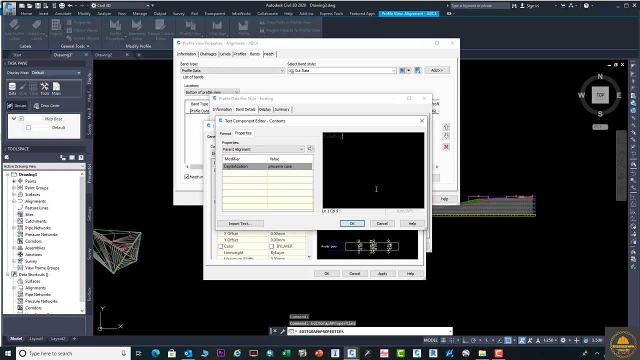 to paste in the some steps. go to the compose label and paste here the name which you copy earlier and here, middle center. from here you can select the text height for and here go to the content and delete the first one and enter the name and okay. select here at middle center. okay, apply and okay. 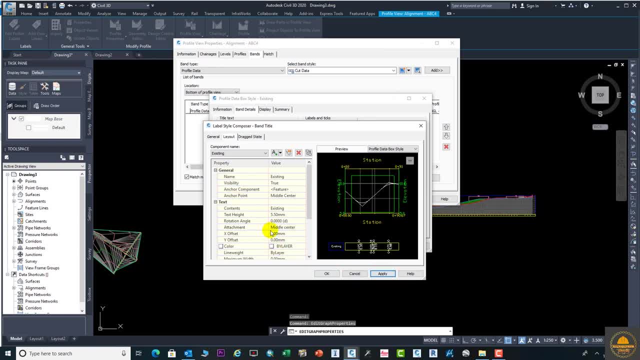 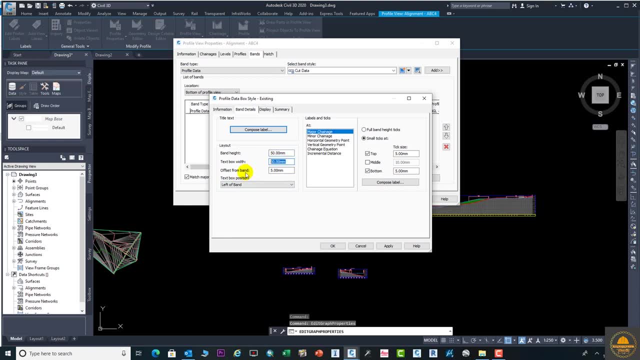 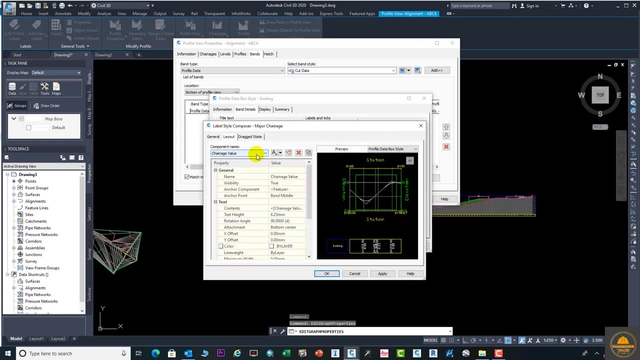 node. the first step is clear. we need to enter here the height and, uh, band width. okay, and go to the third step: compose label. okay, delete this name and paste the name which we copy earlier. and here you need to go this three dot in the content and then click OK. 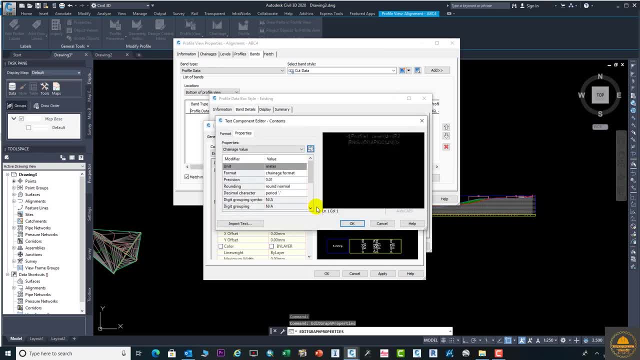 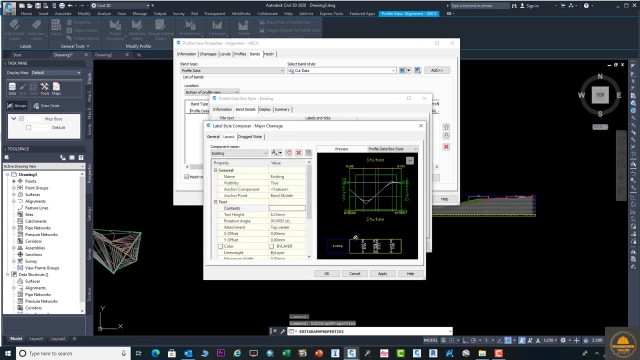 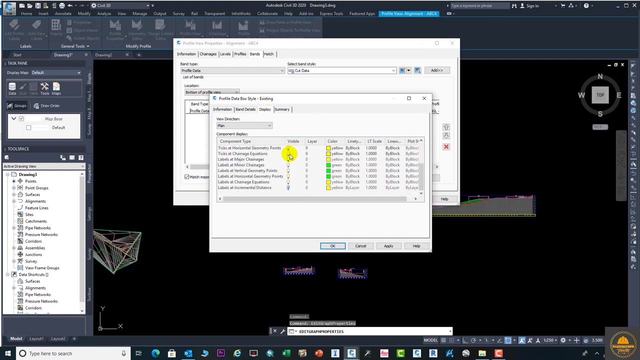 delete this one. and from here you need to select the profile to level, and here you can select the digit after the point to select these three and click on like. and here you need to enter the text height: like. and okay, now we need to go to the display in the same procedure, turn off this necessary layers, the one 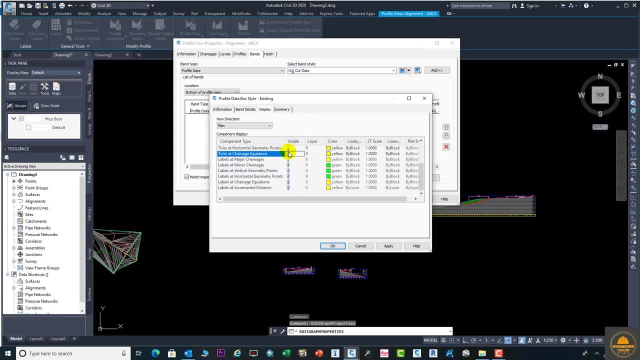 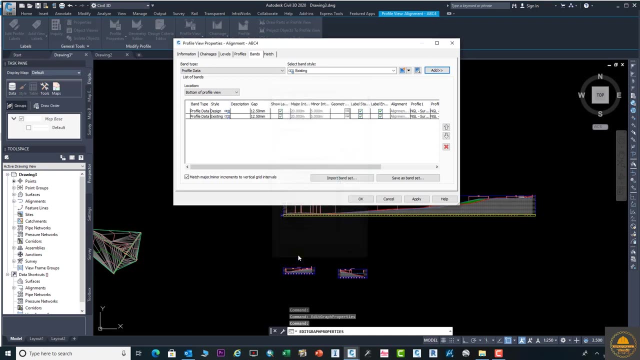 is remain five layers. you need to remain open. first, four and this one level at major change. and now we need to do the same procedure: add and okay. so from here you need to apply and okay, now your existing band is open, but the problem is that there is nothing, no indicator. you need to go to the edit. 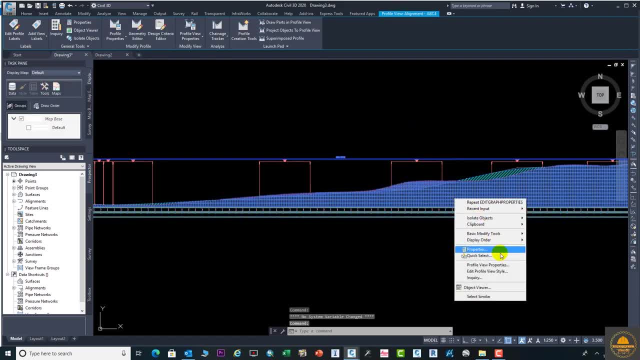 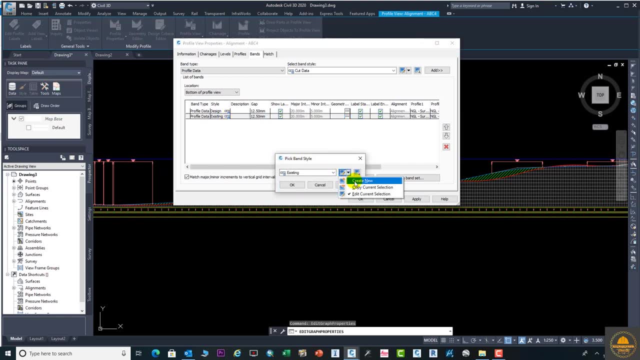 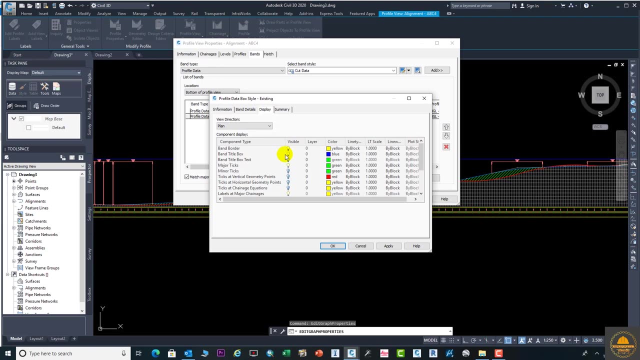 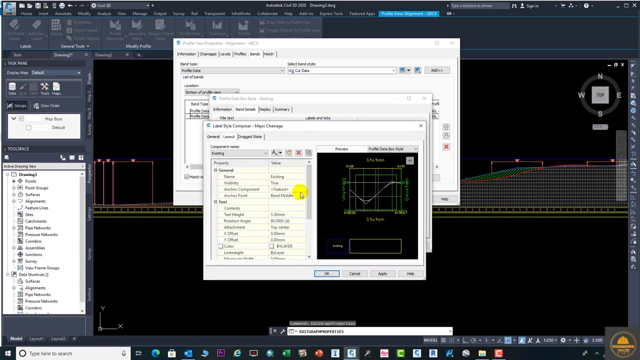 and from here you can edit the same band, which where we add: go to this option and create edit current section. this is plus point for you. you can change if you need to do some changing. the same thing is open. go to the compose label here and click on three dots. we forget to add this profile. you need, you don't need to. 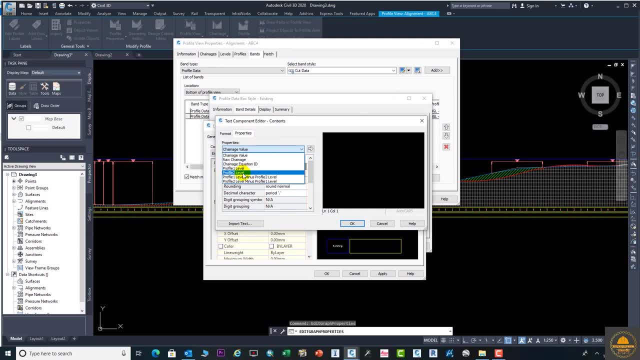 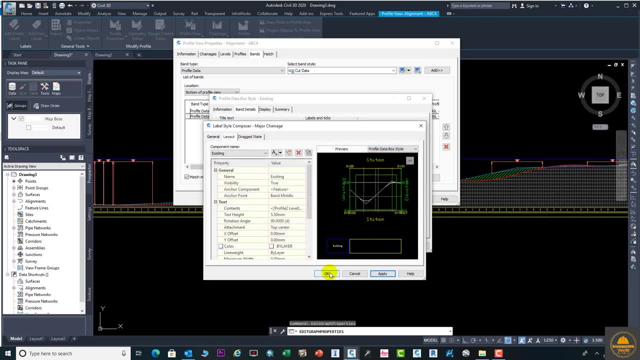 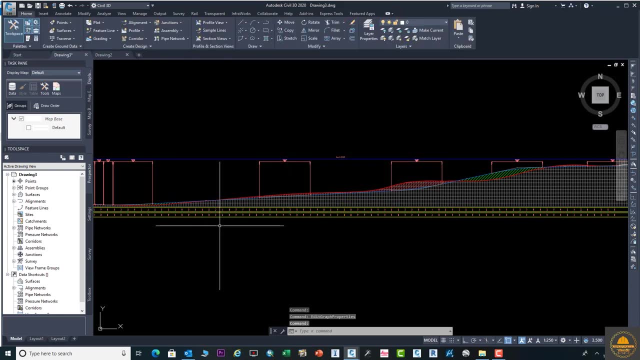 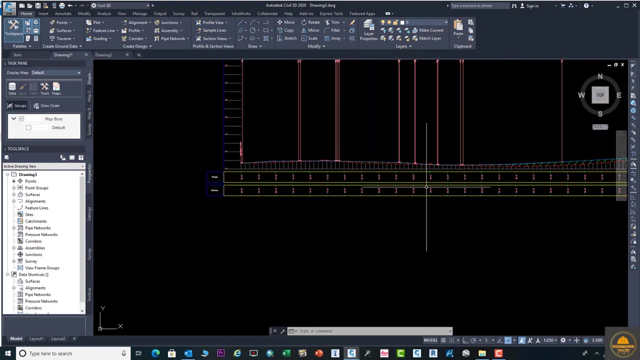 forget this. suppose you need to and apply, and okay, be careful, don't forget, like maybe child mistake need to must. click on the arrow, then your data will be show here. now you can see your proposed design levels and existing level is created now. okay, but you know. 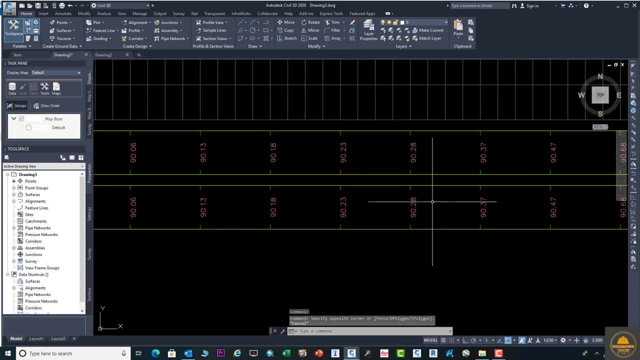 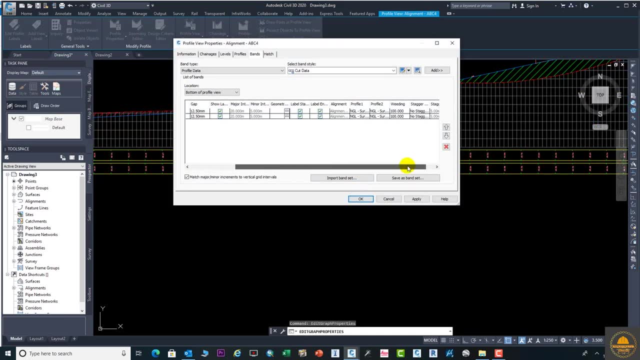 you see that there was the same. I need to go to the profile from. here is an important point because in our both band the level is same. we need to change. in the first band, suppose we need to enter in GL, and in the second when we need to. 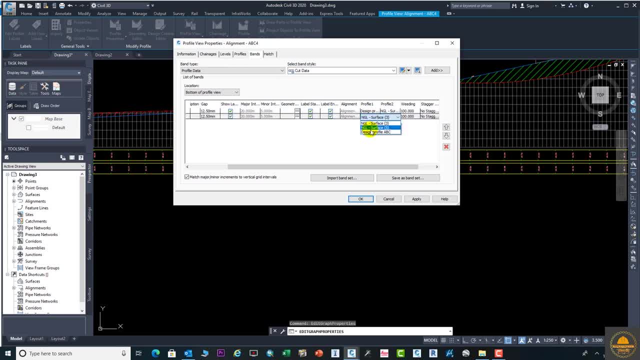 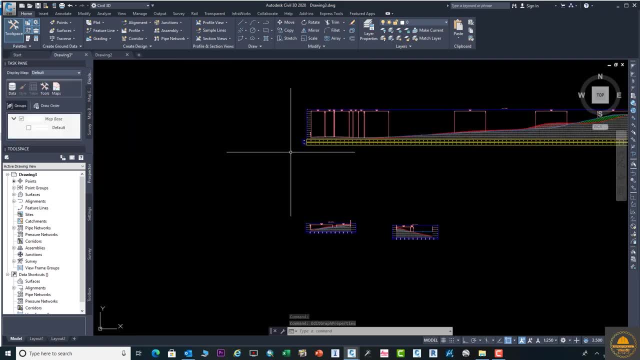 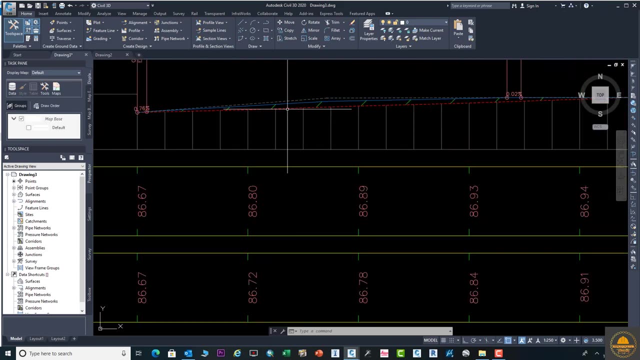 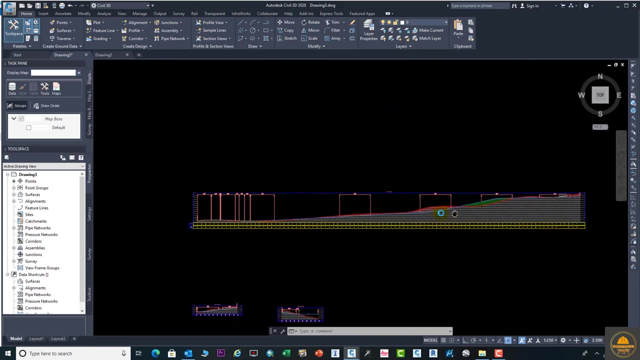 enter the design levels. now you can see your level is changed. in the first one is the design and in the second one is the existing. okay, now we need to go. the second step is that we will be add or cut and fill. cut and fill, band and the same procedure. just go to this one profile view. 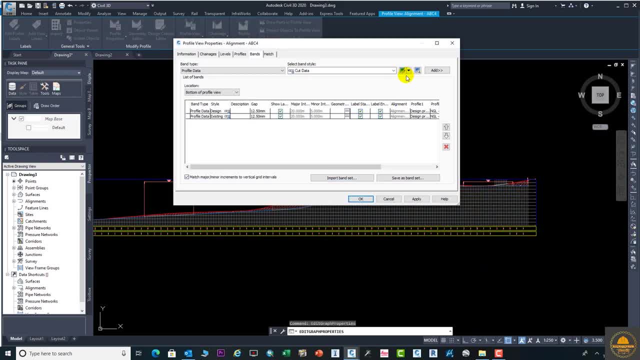 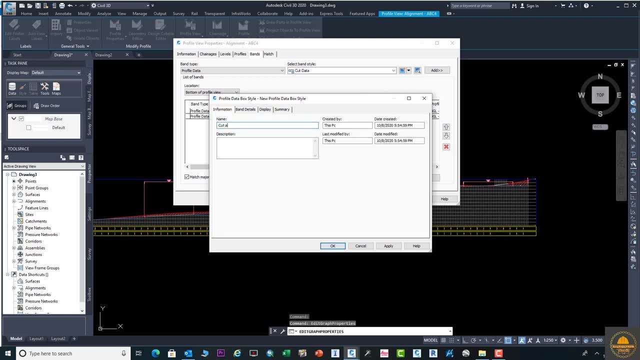 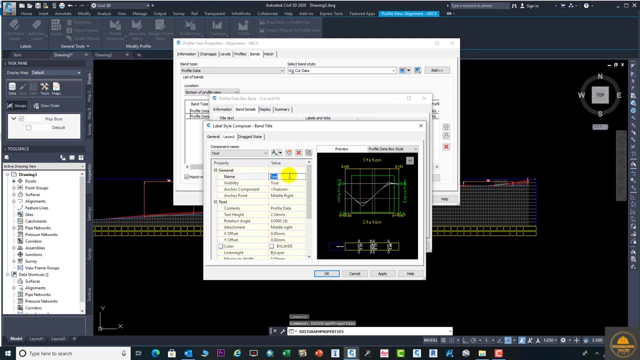 properties and select new and here enter the name. cut and fill and copy the name same as before. we do this. okay, we'll go to the band details for the first step: compose level and from here I passed the name which you copy before and here middle center and here 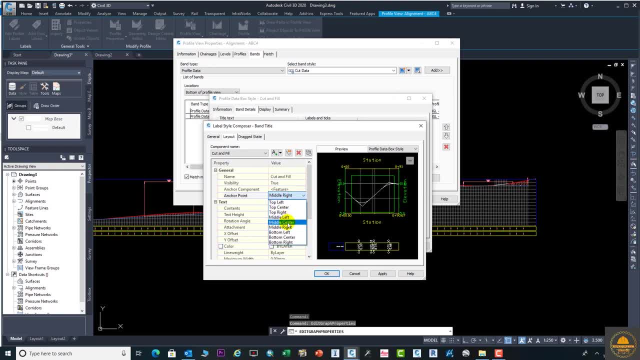 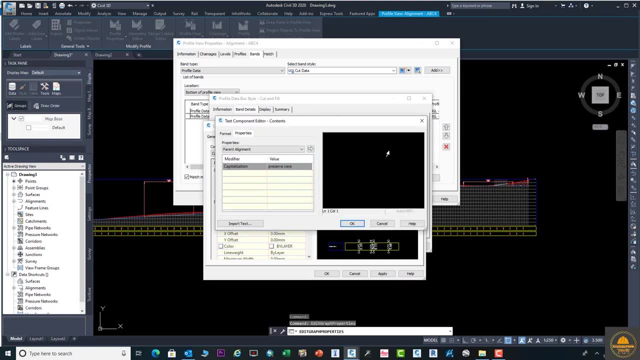 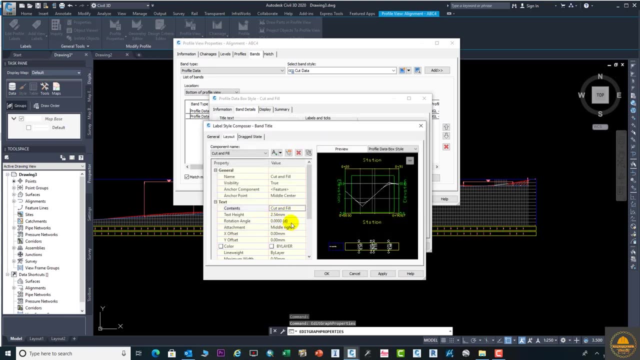 from the three dot. you can just delete this one and paste the name which you copy and click on the arrow button. you must click okay and here enter the text height 5.5 and apply okay, here you need to enter the 50 meter and 75 meter. this is the 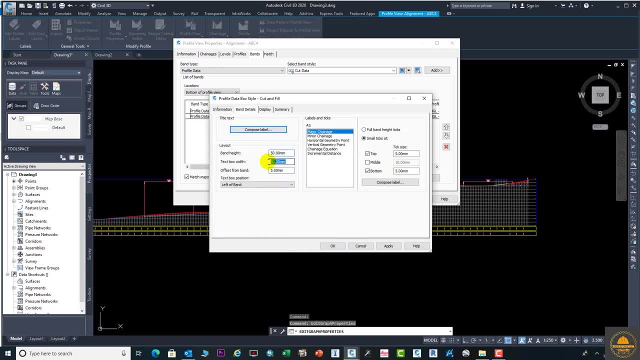 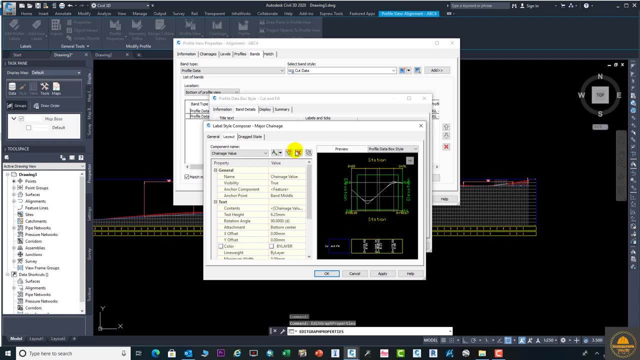 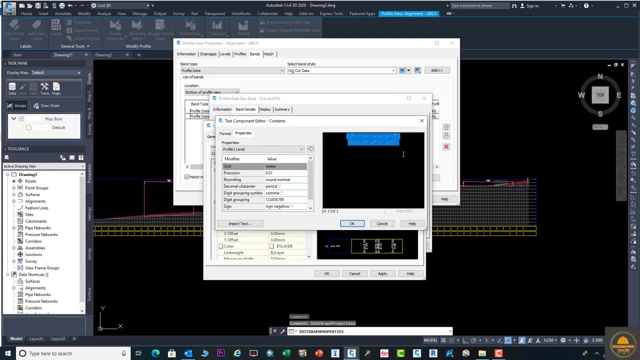 text band height and bandwidth. and from the third step, again we need to go to levels. here we need to enter the name and from here the three dot. you need to delete this option and to go to from profile 1 to profile 2. this is the. 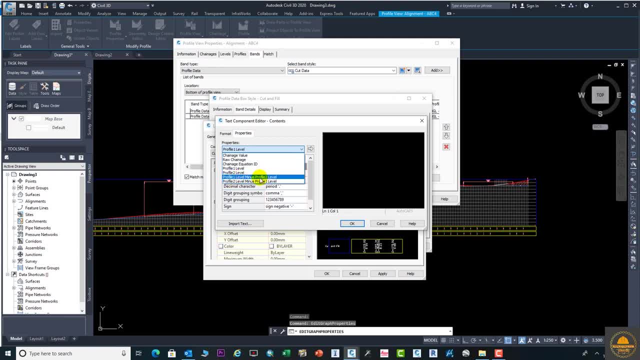 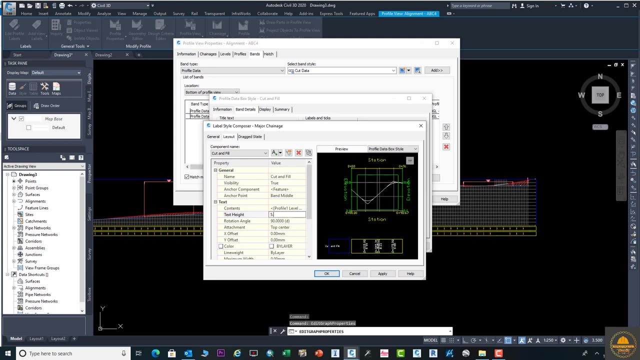 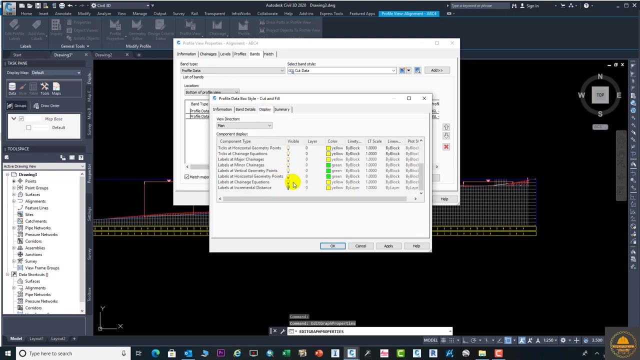 important step to profile 2 and paste. click on arrow and select digit and here you need to apply. here you can also change the text height. okay, and okay, from here display you need to turn off some necessary points like this and turn off unnecessary layers and apply. 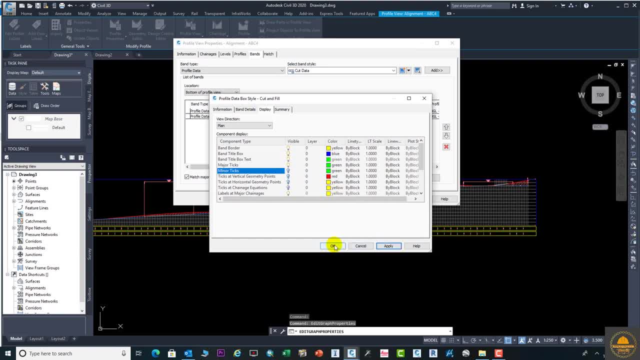 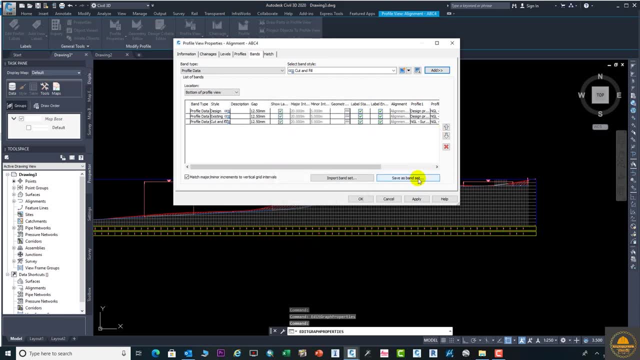 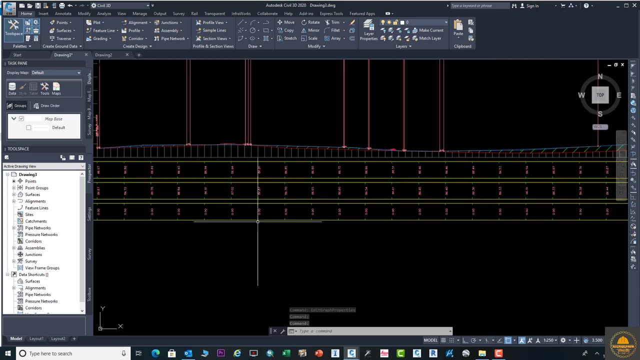 okay, and from here you need to enter same as before. we do the process and here you need to apply and okay, now you can see the band is added, but the data is c-4, c-5 0 0, so the thing is that we need to do again the same procedure. 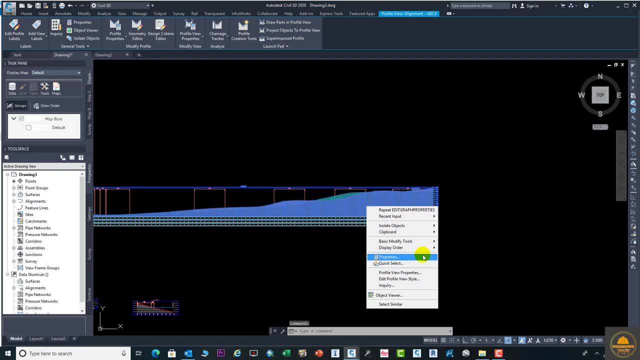 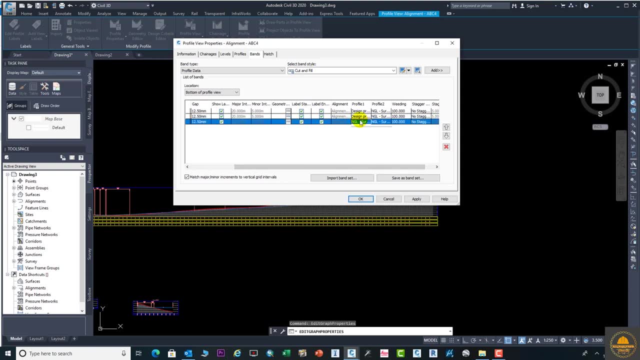 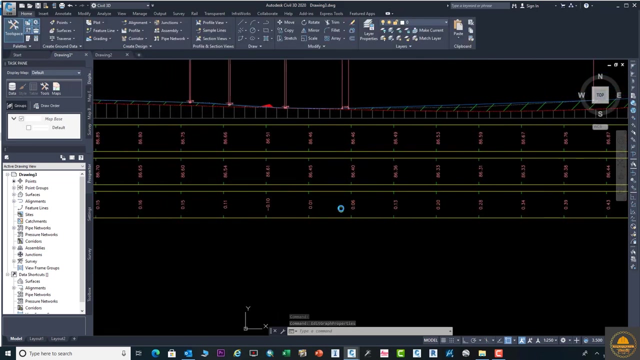 profile view properties. and from here this is the third band which we had. we need to change: in the first profile is NGL. in the second design, then you are. difference will be display in your cut and fill band. okay, now you can see your differences here with your cut and fill, all differences here: where is required the cutting and where is required the. 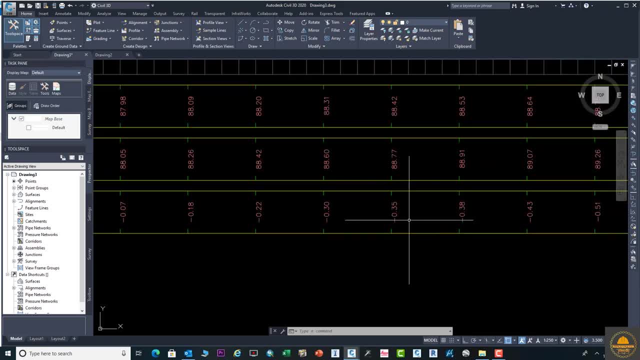 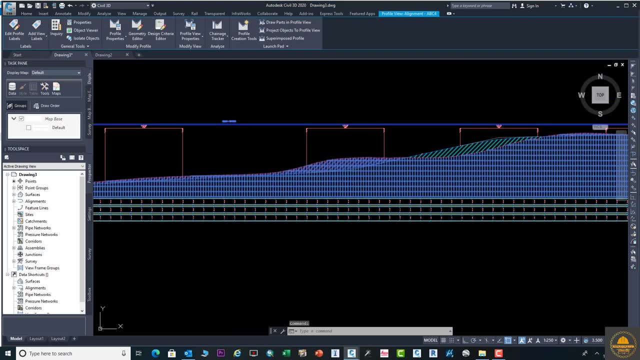 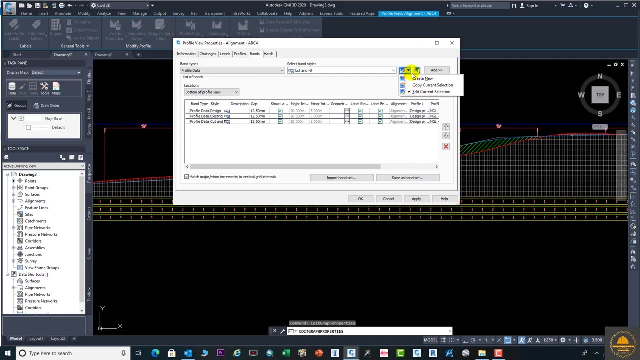 filling. you can see the hitches which i told you. i will explain before the red and blue. it's been cutting and filling. now we need to go to again to the property. we will add the last one band which is called stationing. we will show our station here. you need to enter the name: station. 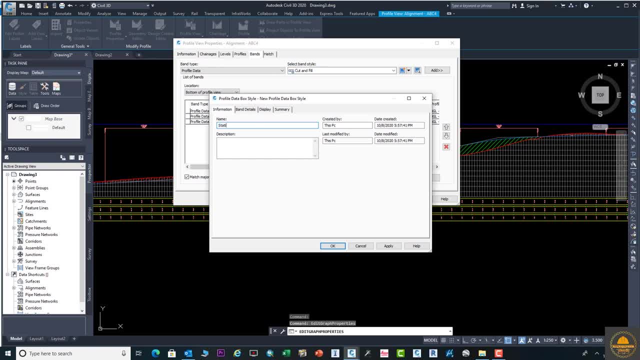 but maybe this one is added before, so it will not support. okay, you can see the option. just we need to enter station one, station one. okay, band입니다. add label here: поз商. the label. go to the 我の出口75777, copy the name and go to the band details and compose labels. paste the name here. 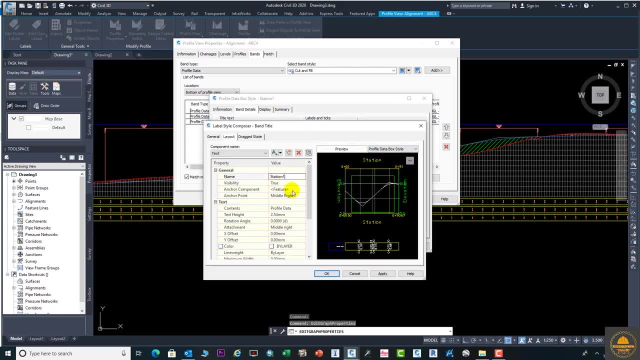 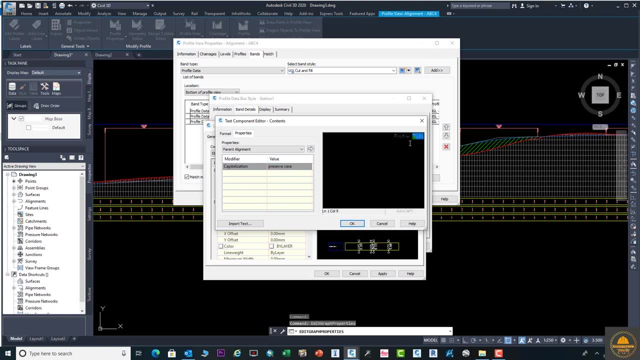 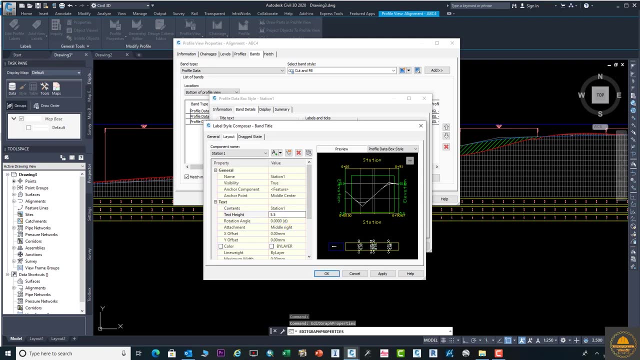 same process and go to the middle center from here. three dot. you need to delete the first one and paste hyperlinks and paste the name of the band and okay, and here is the text孩子' gravушка 1. here you can select the color, but we don't need to select lie and okay, here go to the this one. 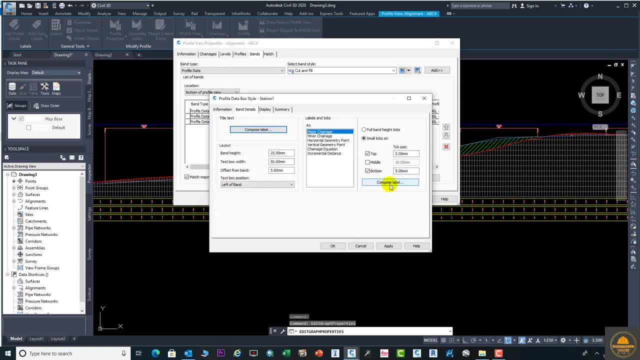 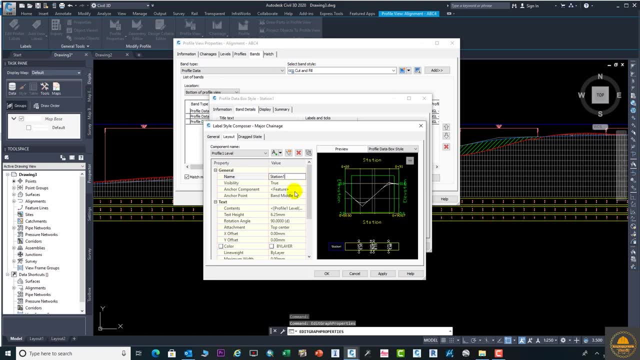 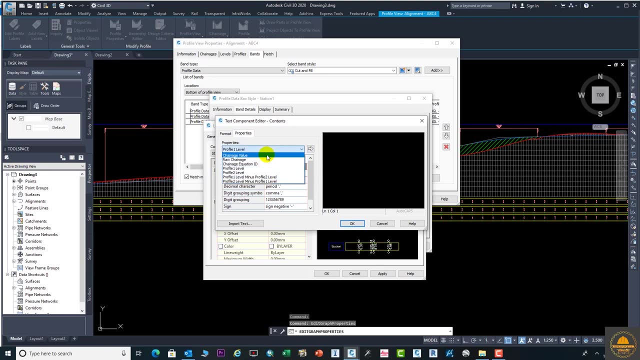 option: compose, label and delete the first name and paste the other one, which you copy out here and here you need to. this one is the most important step. from here, you need to select the changes and must click on the arrow. okay, and okay if, when you click on the arrow, you are. 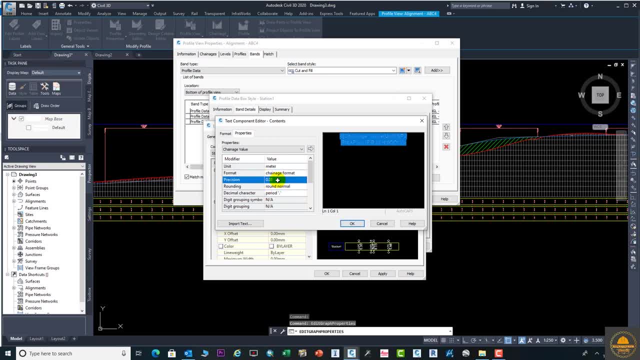 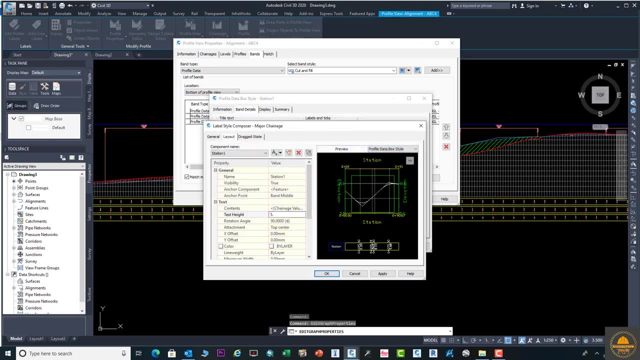 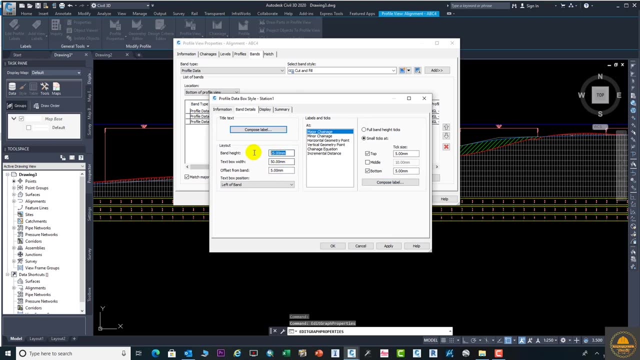 um, requirement is edit, so here you can change also the height, uh, 5.5, and apply: okay, apply and okay. here you need to change the band height and band width, okay. another step is go to display to turn off some unnecessary layers, because we don't need to display the unnecessary layers. 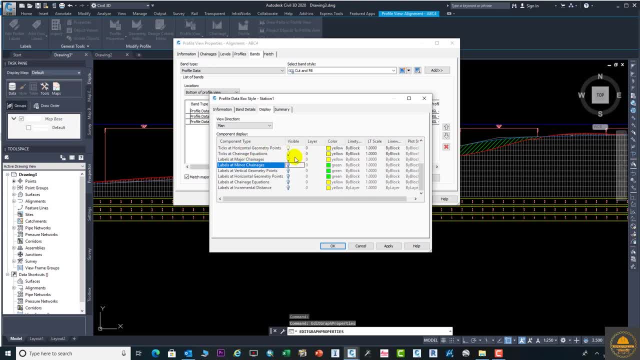 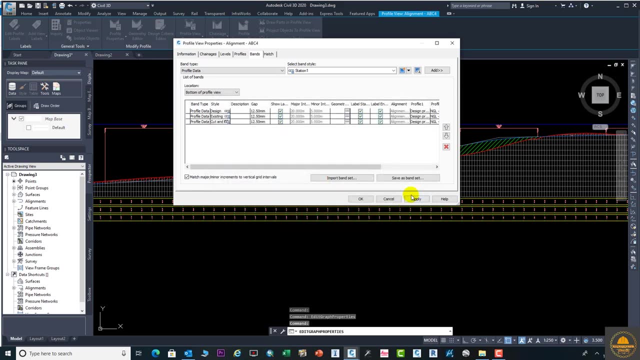 the five layers which explain in the first step we need to open. uh, turn on the first steps. okay, apply and okay. now you need to go to the add button and go to ok and apply and ok button. now you can see your stationing is eight. okay. 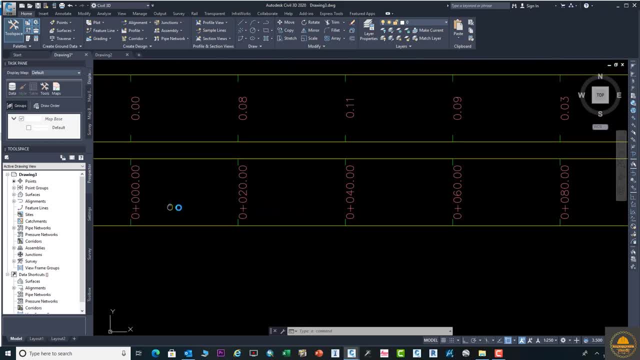 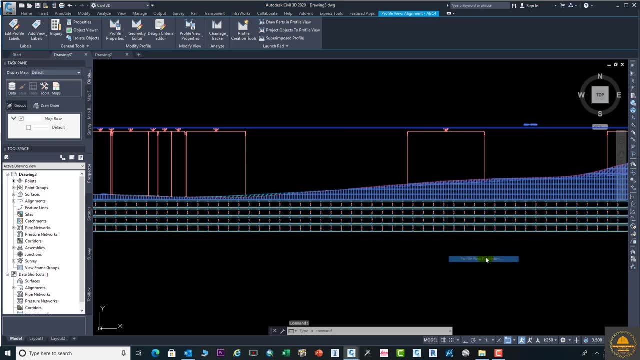 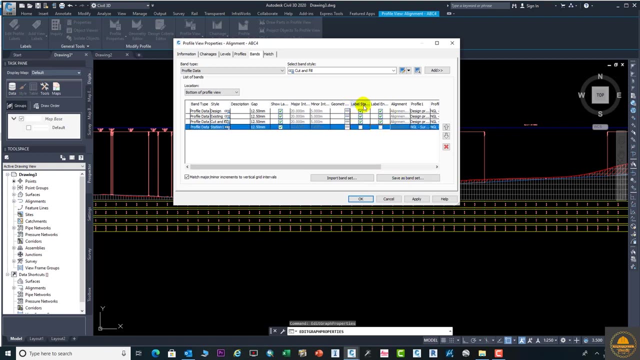 20. uh, once two station is extra added, we need to turn off this two stationing. just start and end. uncheck this two point on the band. okay and apply. and okay, now your station is start in, the extra is removed for 2020 is our stationing. you can see. 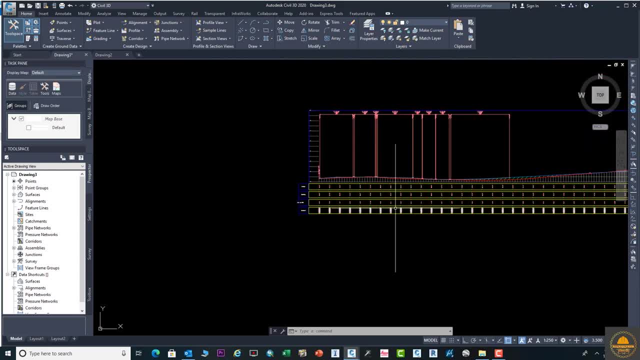 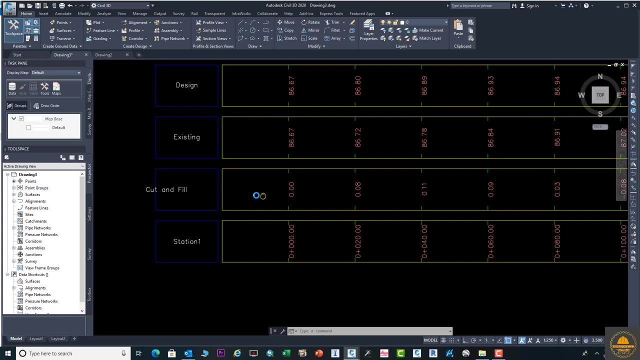 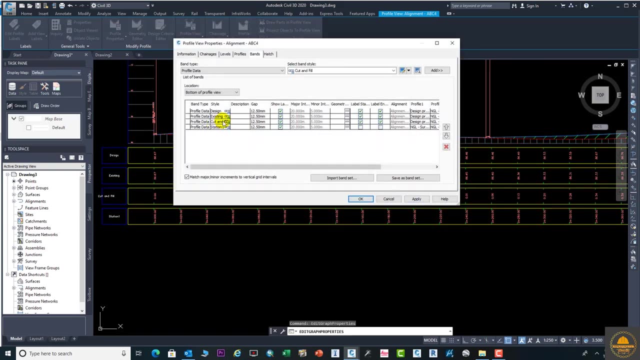 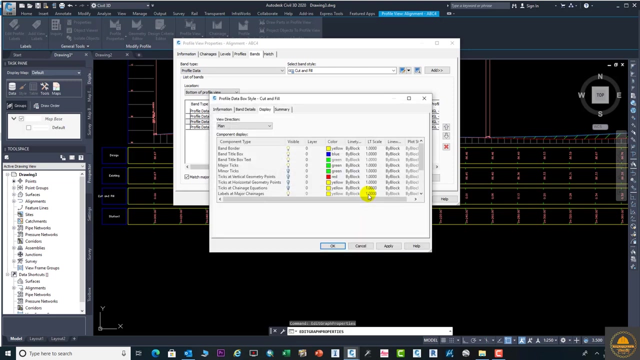 very well. oh, this is the problem over this height this band is. we need to increase this length. you can see, just go to the this bend, to the cut and fill bend and go to the edit current section. you can change because the yes, okay, 60 and anyone you can change now. 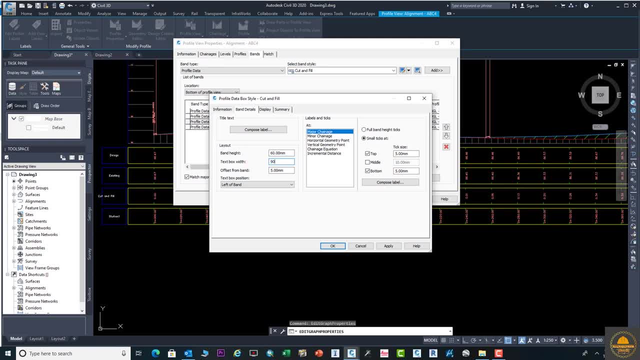 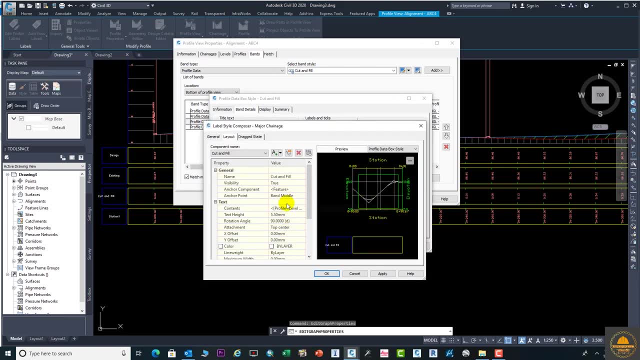 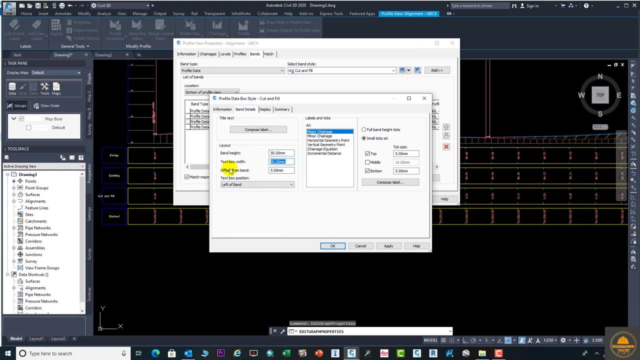 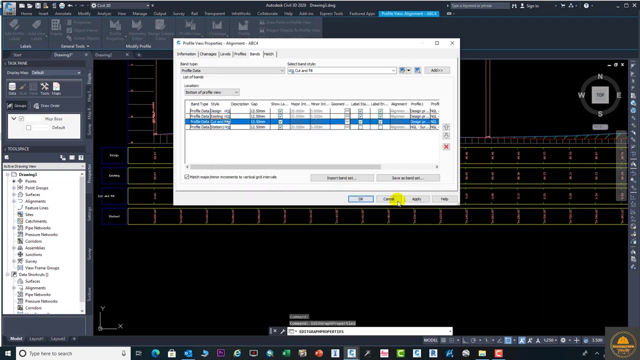 arts. okay and go here also. no need to change this. okay, compose the middle center, middle center. this one is also okay, apply and okay. um, okay, 50 and 75. okay, okay, apply and okay. now you can see there was the problem in the middle center, we not? 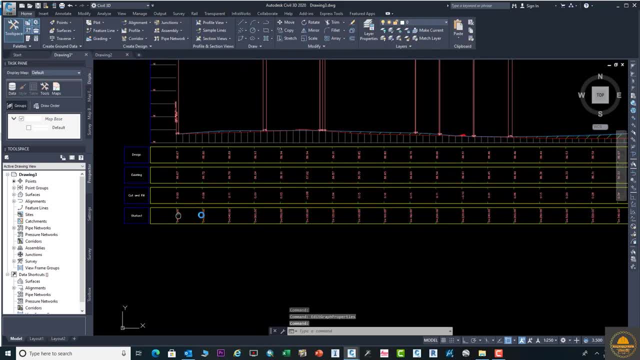 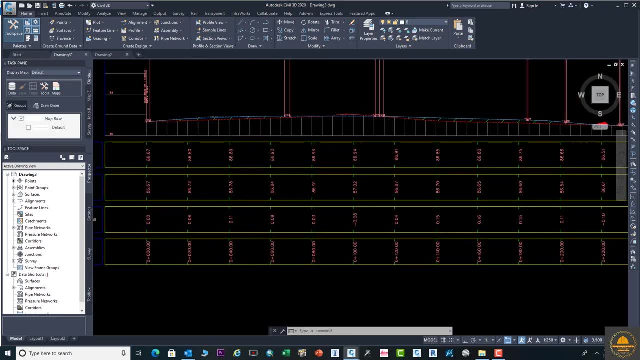 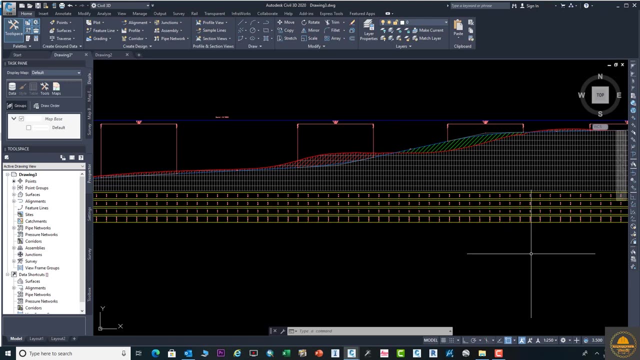 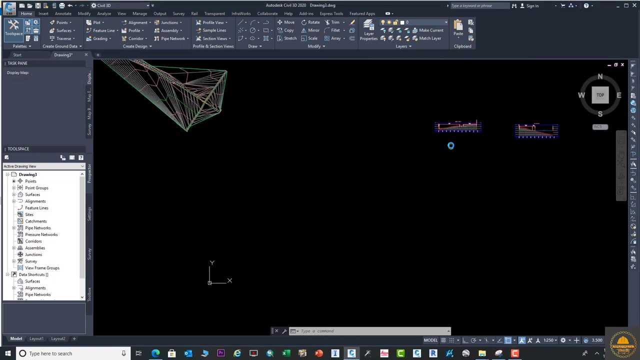 select the middle center. so when we select the middle center, the text is coming to the center. now you can see your all bands is ready, same as you can edit in the other bands: geometric bands and super elevation band. okay, in this step we will be create surface or alignment. we need to go first of all to 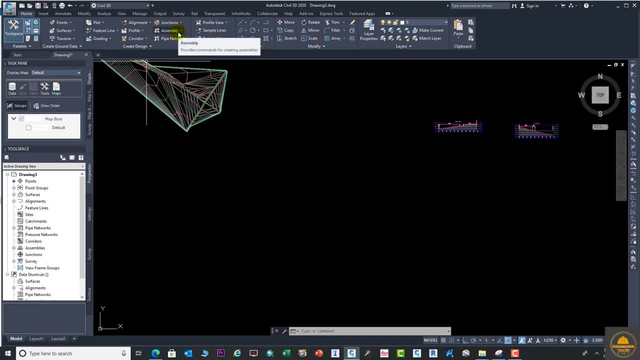 the assembly. first we will be create or assembly from here, then we will be create our surface. just see, this is the important step. you can create your assembly from here and just enter the name of assembly here. suppose we need to enter a be assembly in here. you need to select. 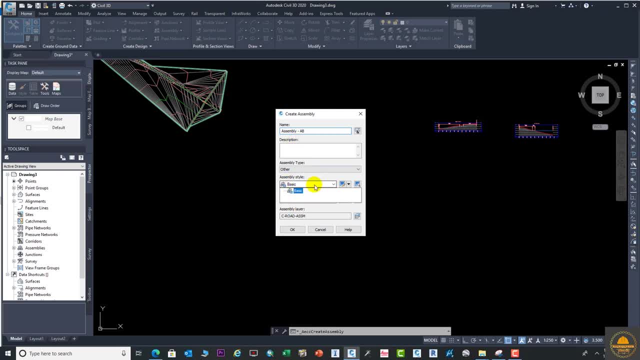 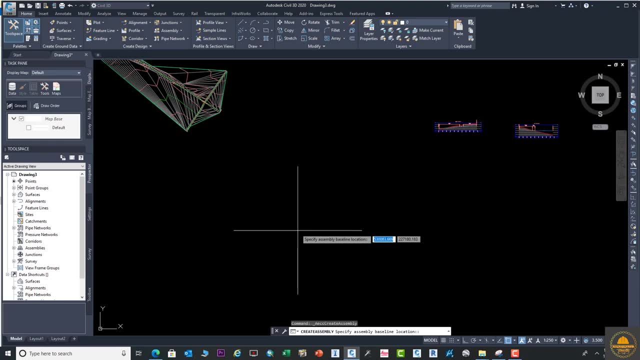 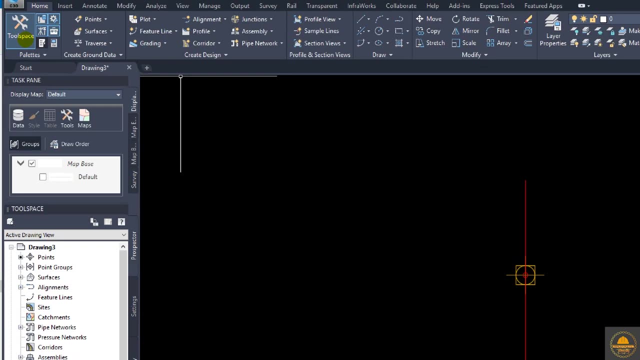 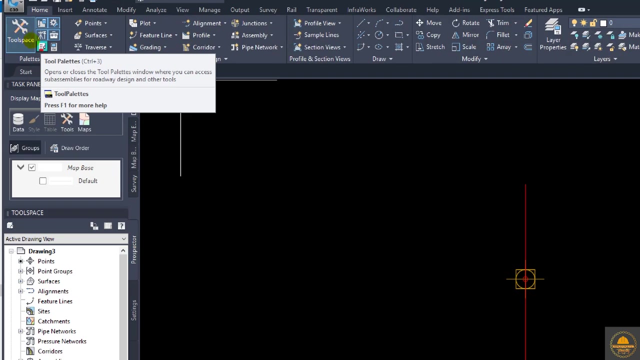 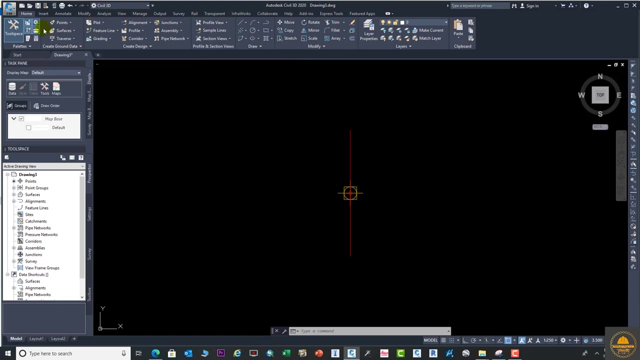 a basic and here all code and okay. so select the place where you need to create. okay, here you need to go to this option. yeah, this one tool palettes, this one is the assembly tool palettes. or you can enter ctrl 3, select yourself, and your tool says open. from here you can see basic lane. 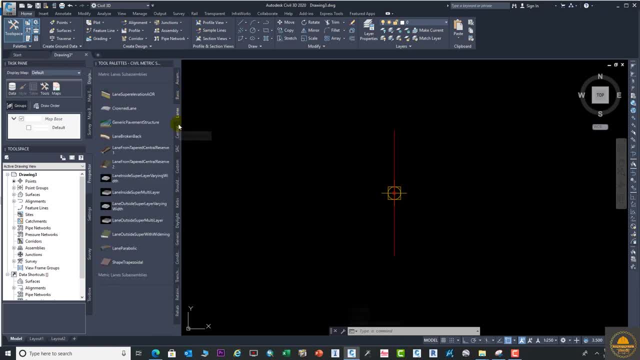 corridors, a custom shoulder, curves, daylight, and you can also customize your assembly, which one you import from the outsource. and here is curves. okay, here is daylight. this all detail we will explain later one by one. okay, basic, first of all, we need to go to the lane. yes, lens, and from lens we need to. 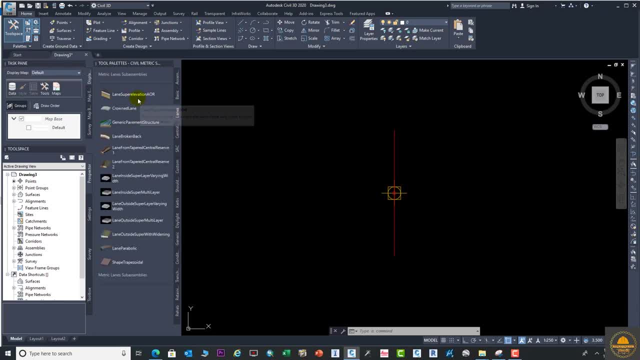 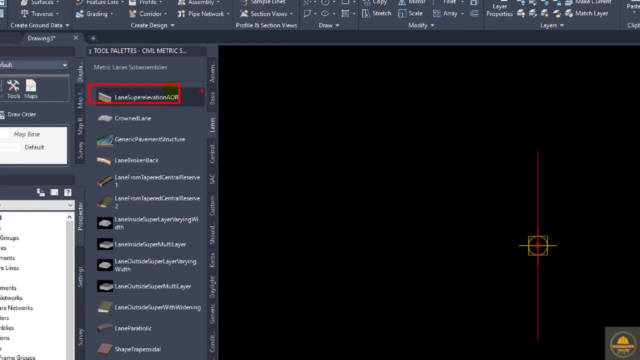 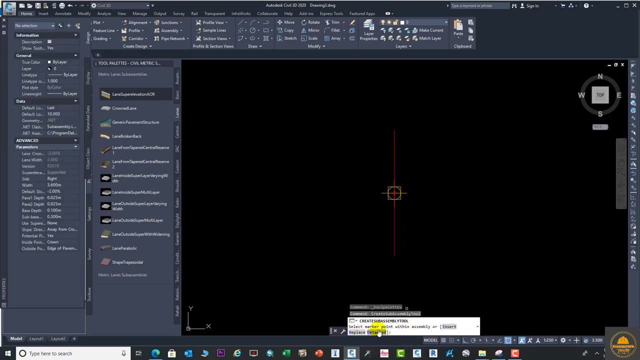 select the first one, this one, then super elevation, a or s, per your requirement. you can select the lens. okay, here is the shoulder and daylight. we will be explained these few steps. click here and you can see here the command bar and that replaced. okay, just click here at the center. okay, and if you 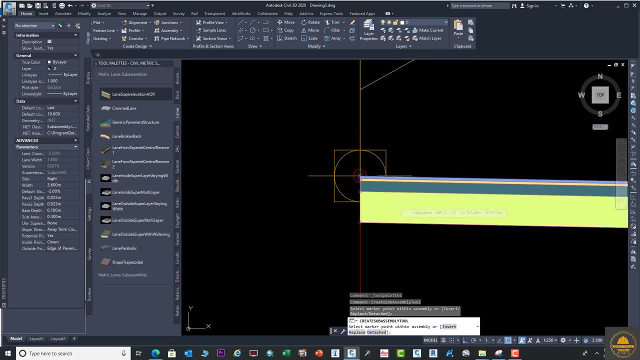 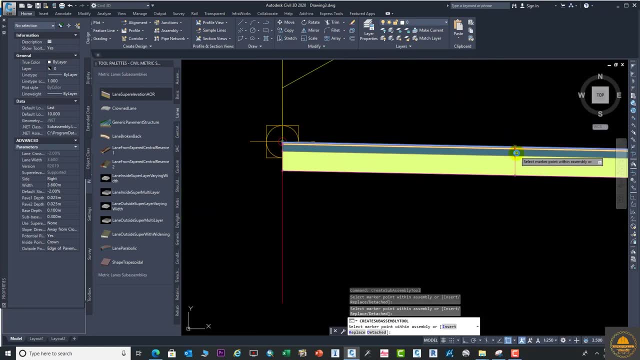 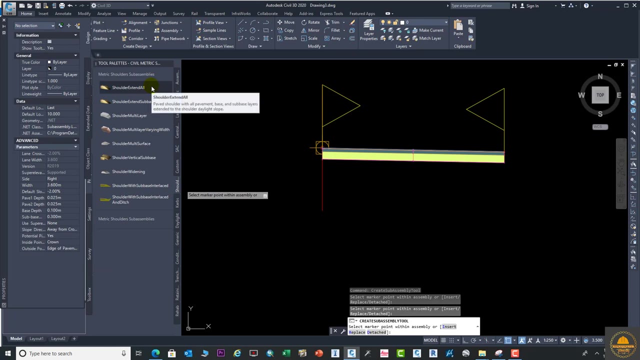 need to double lane, you need to select. click here again on this option. okay, know, your tool lane is created and if you need to add your shoulder, just go to the shoulder and select is for your requirement- shoulder option. and you can add shoulder option. just let me select the first one. go to the daylight, if you. 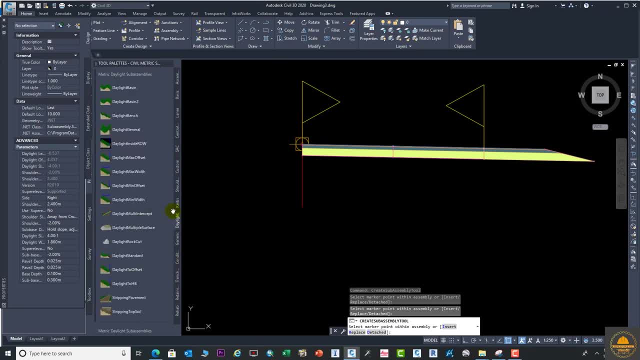 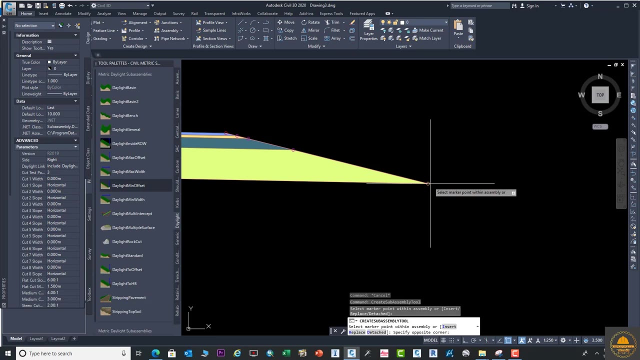 want to add the daylight. i am going to select the daylight journal and click here. here is the properties, okay, let try we explain the properties. so click now. your daylight is here, okay, and the properties also here when you click on this and go to property and control. 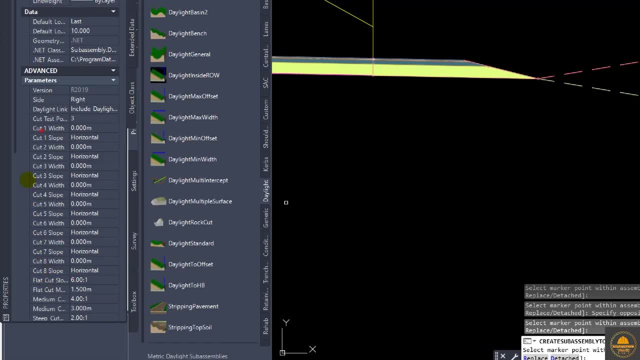 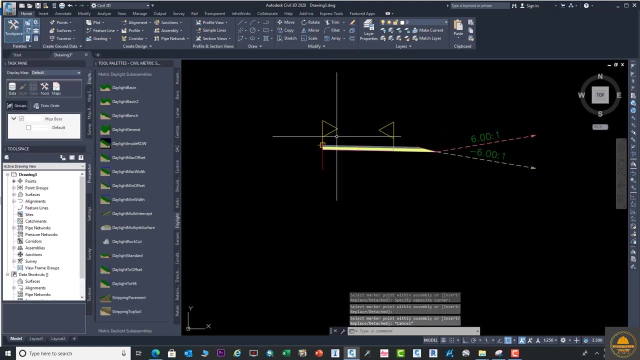 one property will be display here. how much is the requirement? how much is your slope? is your project specification you can enter. okay, let's select. let me select this three option and go to the mirror command- and we need to. this is on the left side- and click here. okay, no, you can see your. 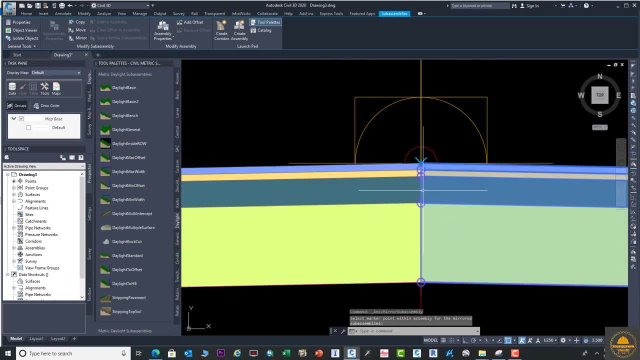 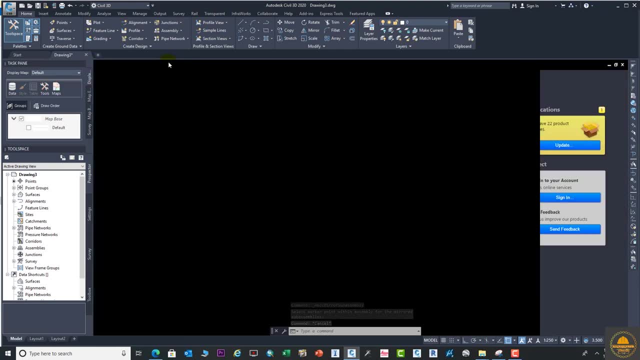 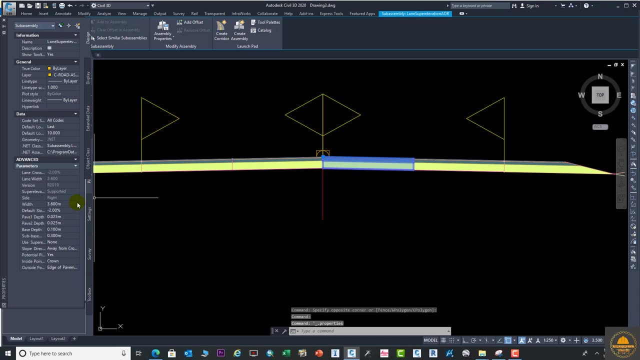 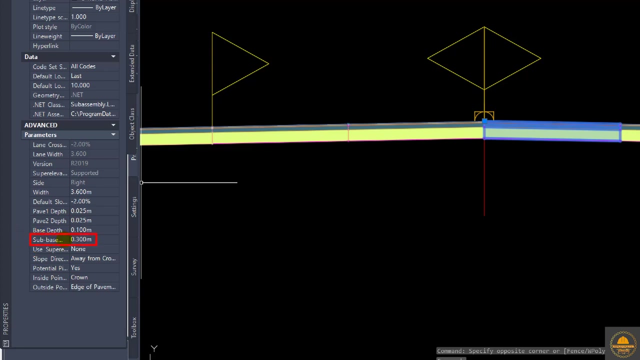 partially sauteed because all those ligne is delete. there is a double line, is what n is on the left side, and then take one the axis. is you see it? okay, now click here here. one page is hidden from the electrical module and there is an overframe chemical. area. also注意 here: double chin here also give you 3 ر purchased. the body, of course, is one, double line is in one side and double is on another side. let close this option and the only important thing that you can see here: the property, your depth of sub base and base. 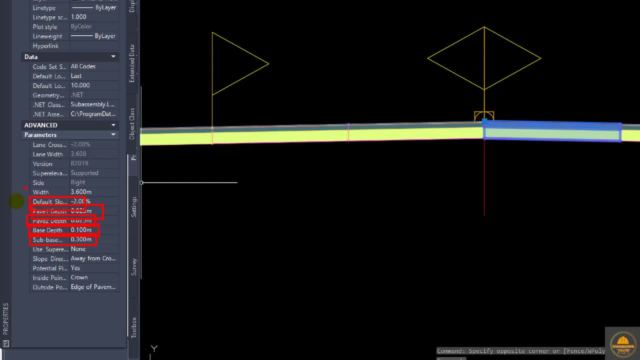 see this one, a base. how much depth is your project base, sub base, permanent and wearing course your one carriageway? super elevation, cross lane, cross slope. these are details you can enter on the property. suppose you need to enter the one and lane width? 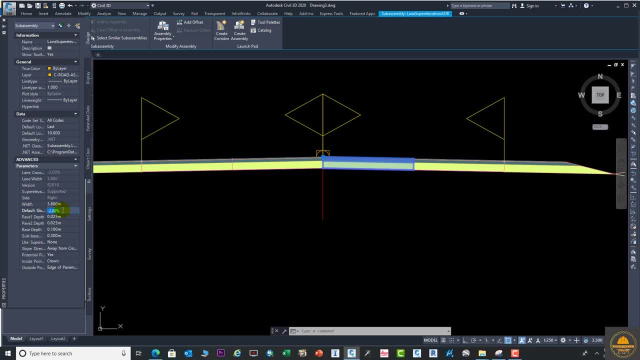 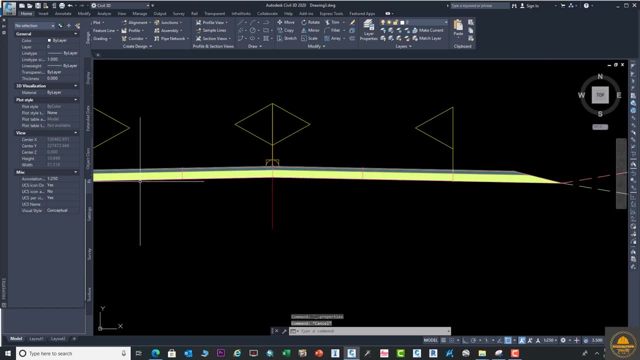 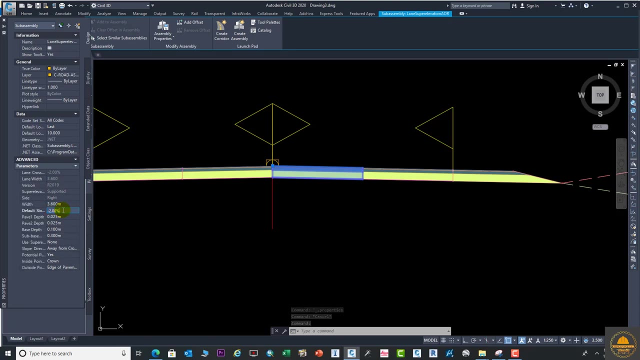 and you need to enter your varying course: 10-15 centimeter base. anyone with you can enter in this properties. okay, here you can change the cross slope. you can see this. okay, you can see the slope is change. we enter this one. we change just for the first length. 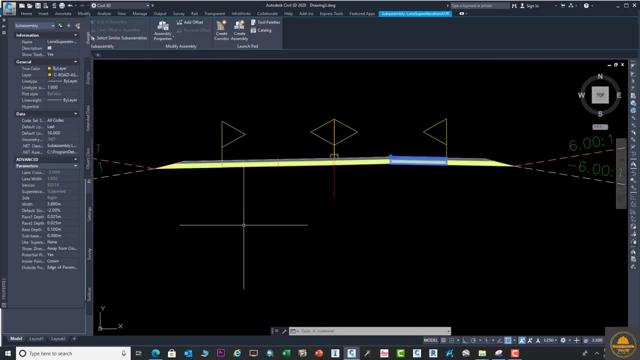 it's same as you can change for the second one and the slope will be smooth. here you can change the depth of your pavement and here you can change the depth of your base and sub base as per your requirement. just 20 centimeter, 15 centimeter. you can change this. okay, so you can see, and now it's okay, the slope. 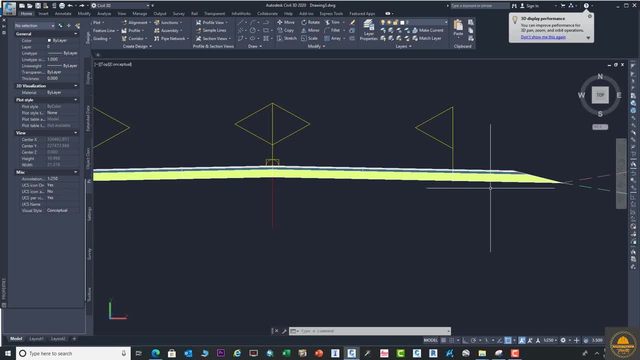 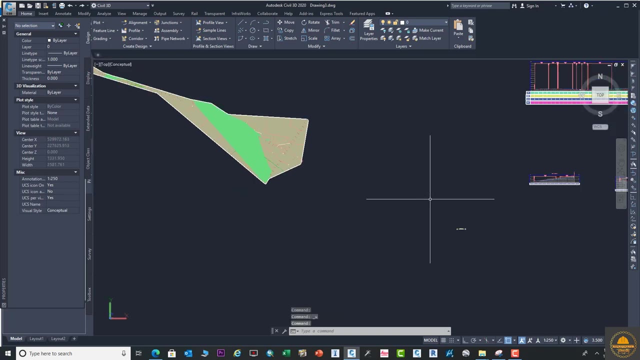 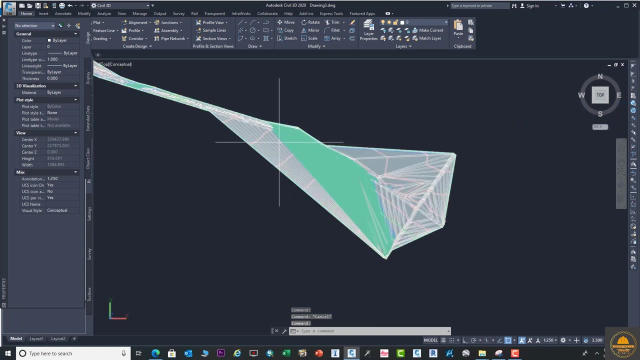 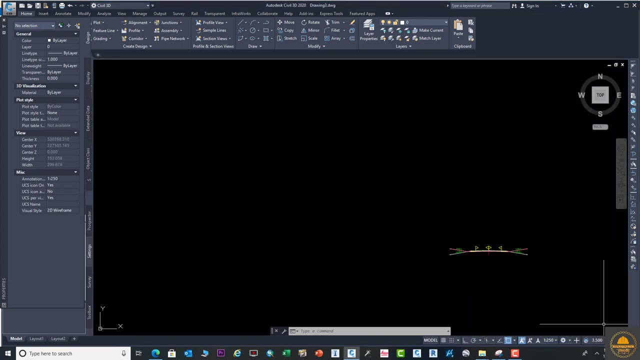 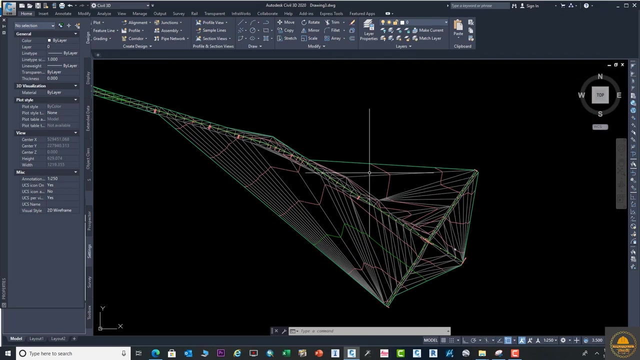 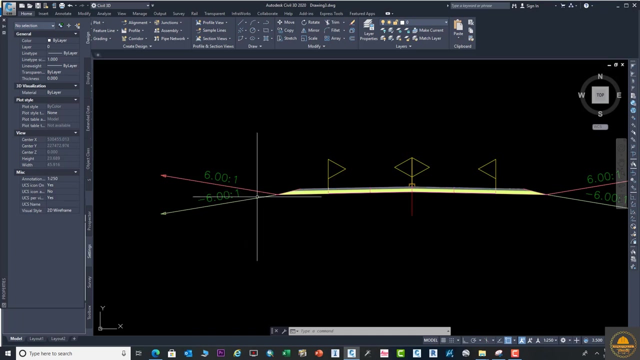 before I change, just for you, for your confirmation. and now we need to do the step. our assembly is ready and the next step we will go to: okay, just select this option on this one. okay, now we will create all surface and the same corridor. okay, corridor surface for this purpose. just close des로ction and go to the. 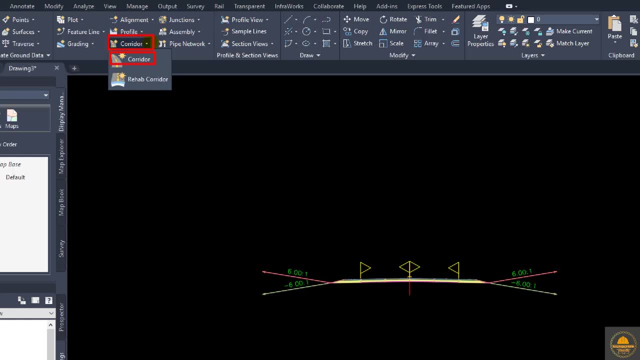 ok, this odor option from here. let's pop up manage, open it. of course, the same for this purpose. just close this option and go to the corridor. first of all, we need to it a corridor. okay, this 거예요 option from him. let's pop up, manage, opening what? 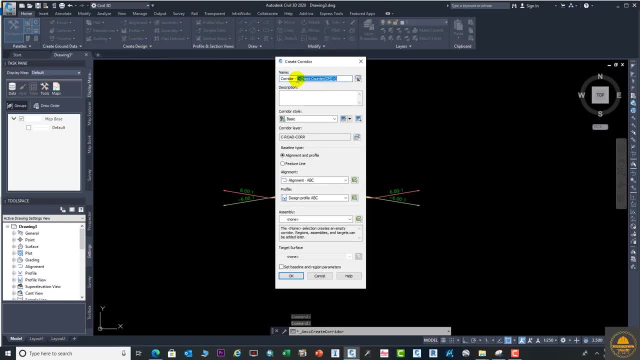 of this. what you can do is, if this doesn't work, go to the private app, sort the simples of view. you need to change the name. suppose we need to enter our corridor ab. here is the basic. here you can select the layer and here is the alignment. on which alignment you want to try. 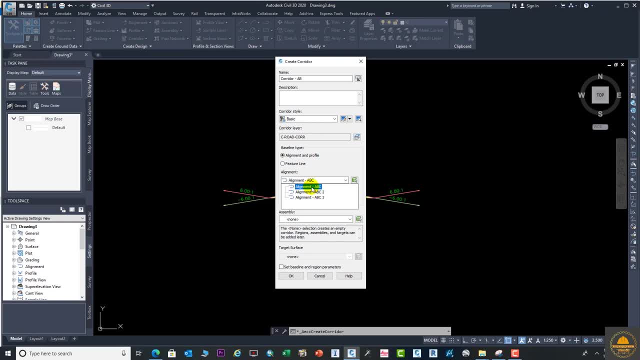 your corridor because we have three alignment. we need to add our first one and here, if you have much surfaces you can select. and the levels we need to select the design profile and assembly ab and which assembly? if you have view assembly, which we create before, you can select your current assembly. and here you need to select the mgl and press ok. 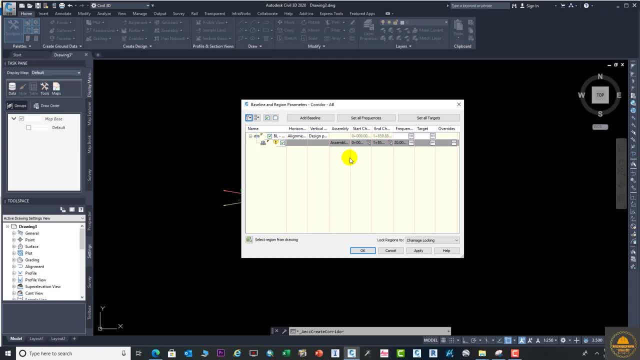 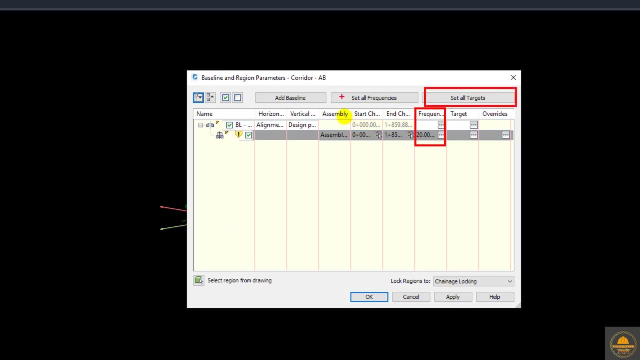 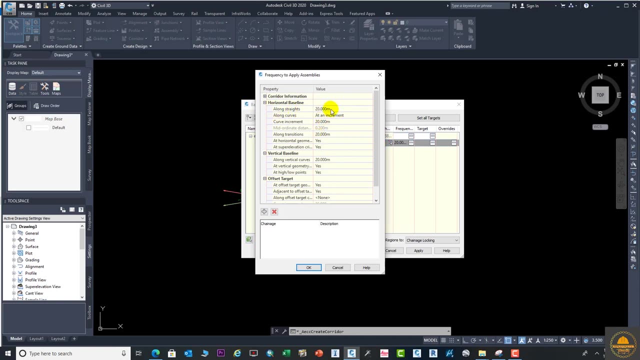 the stop pop-up menu is open. here is some information which we need to clear in this session. we'll go to this option- the frequency- and set all targets. click on this. there is some few information. as per your requirement, you can change. here is row increment, if you want to change this, and here is a long stretch and the other option is. 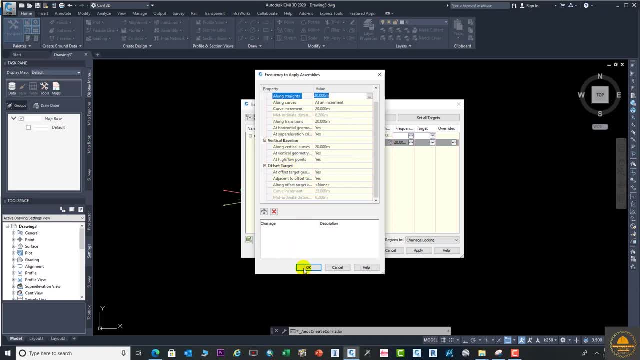 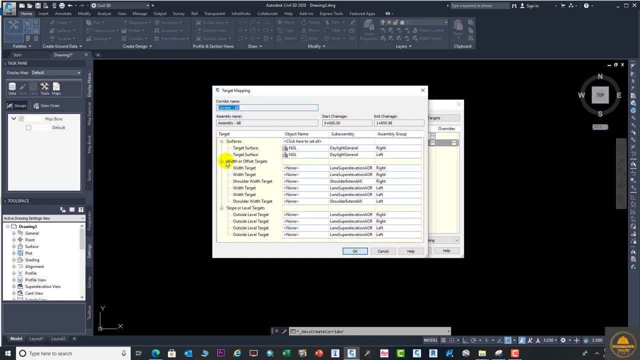 few, some you can change from here and also you need to go to set all targets. here are some few points. if this one is not as per your requirement, you can change from here. target surface, target surface with target and with target shoulder width target. you can change this right to left and left. 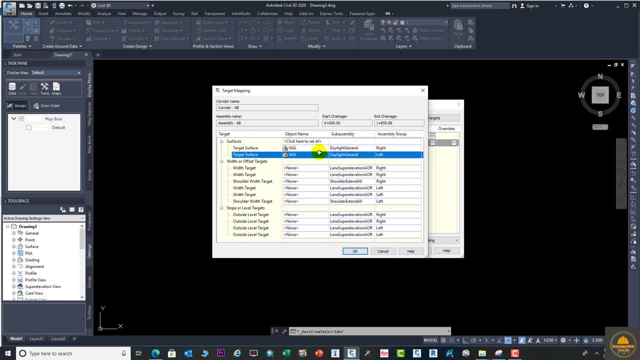 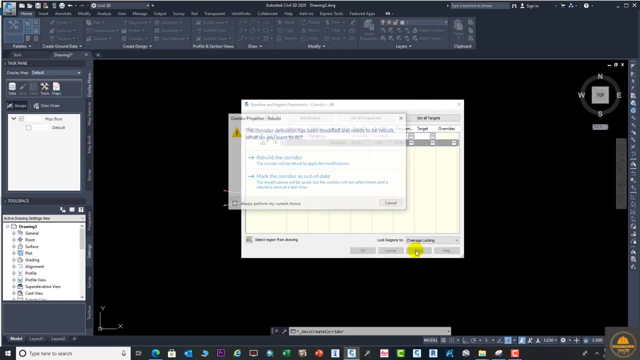 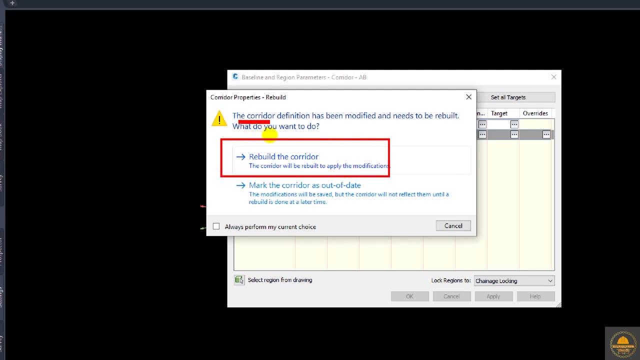 is your requirement and you can change this headlight. you know this message in front of you: rebuild the corridor. if you click on this, your corridor will be rebuilt. the corridor definition has been modified and needs to be rebuilt, and click on this option. you can see. you can see. 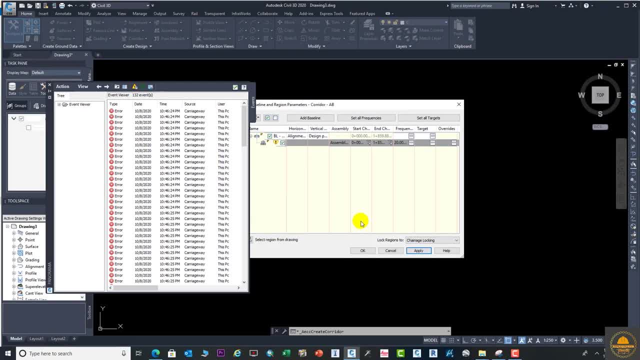 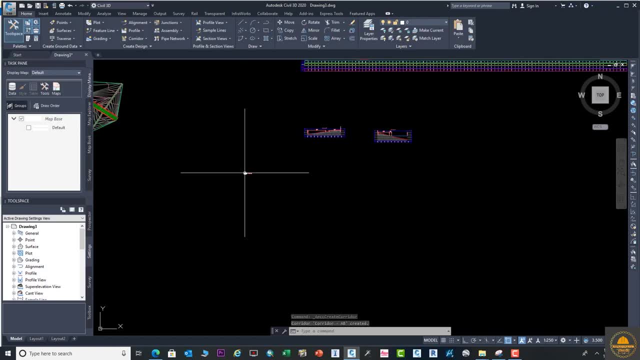 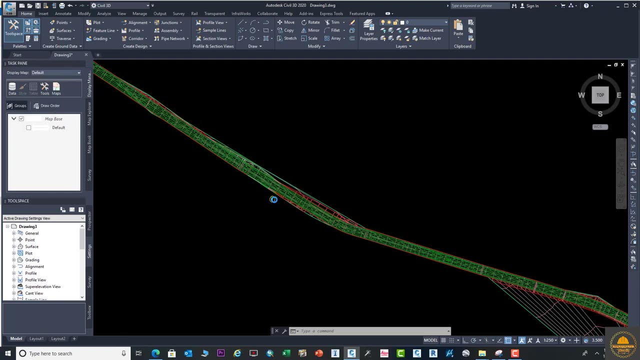 some areas you need to close. this is click and if you go to the alignment, your corridor is done. you can see your corridor. this is your road corridor. that's mean the road corridor is that how much is your road weight which you create the assembly. it's mean this is your road width and corridor. 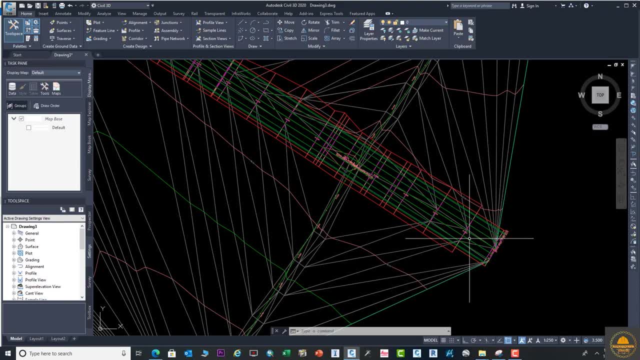 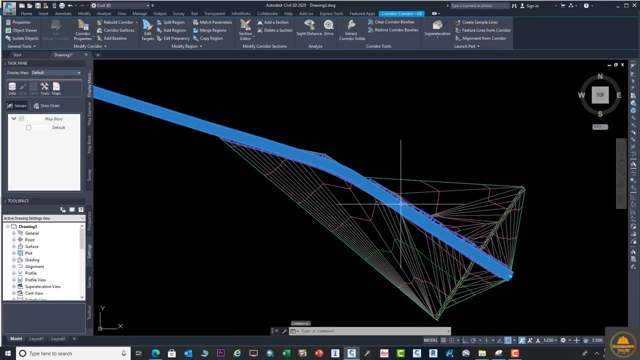 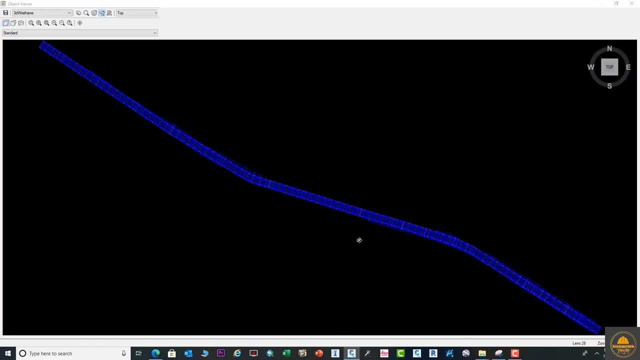 yes, for your assembly. your corridor will be built before corridor. you must ensure to draw and create your assembly. go again to select this- your road corridor- and go to the object view. we will see our model road model. from here you can change the difference option. this is the object viewer. you can see this is now realistic and this is x-ray. 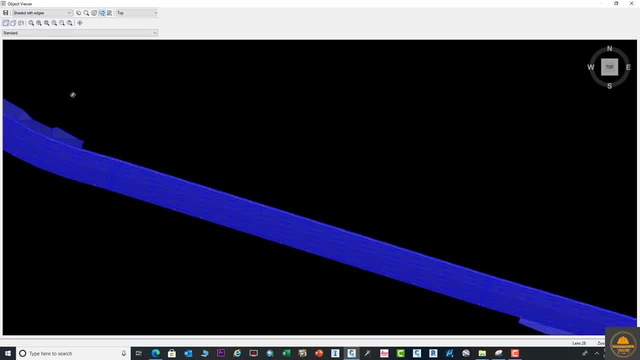 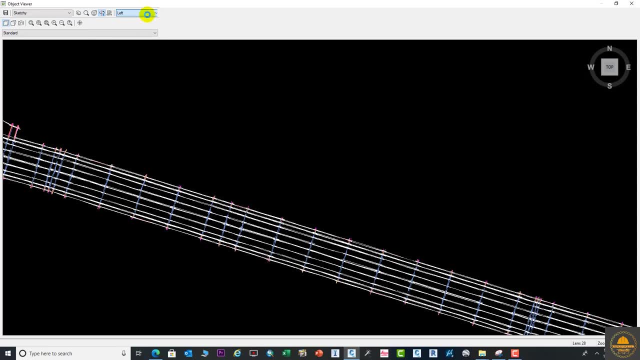 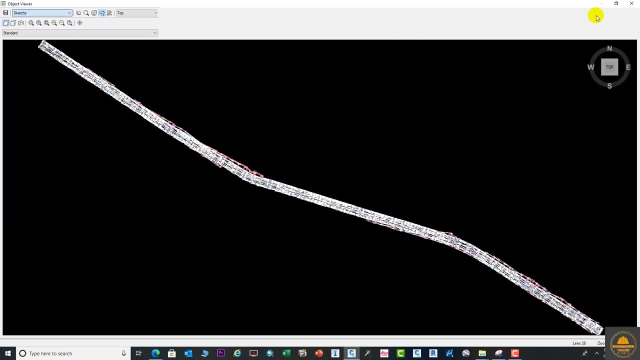 and this is shaped. and here is you can left to right and left to bottom top. you can see all the views from here. this is the object view and the next step we will be play and see how our cut fill is looking. this is a good step. 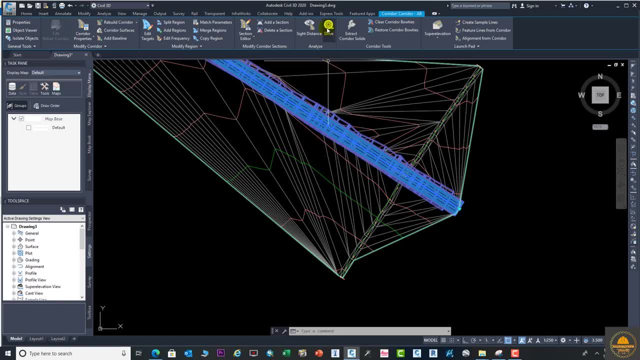 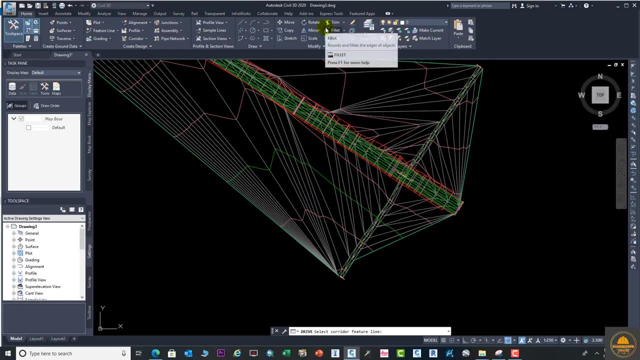 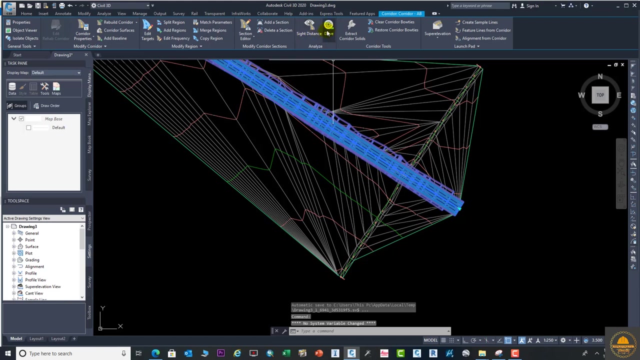 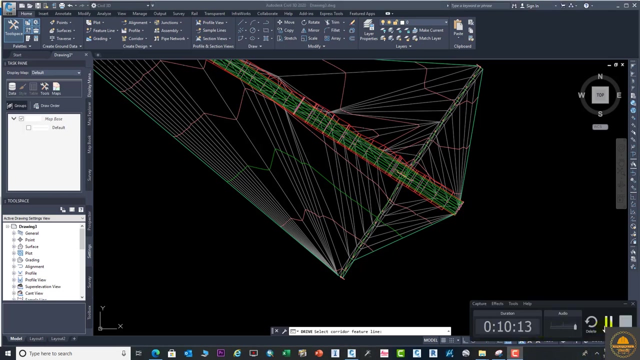 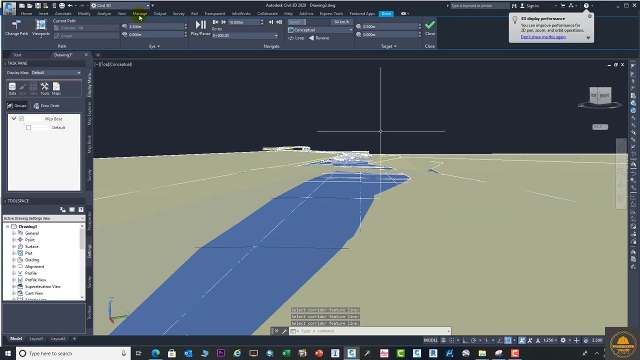 interesting and go to this drive. we need to see our road uh face, how it will be looking and how is our cutting and feeling. okay, let me select this option. okay, i'll draw you. and again, okay, select this option and okay, and now you can see when you click on this player, push, you can start from here. so we'll take. 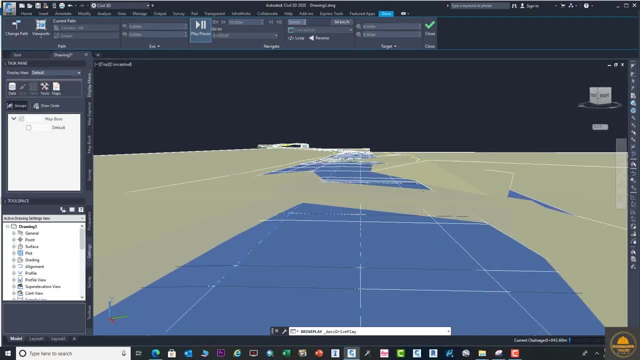 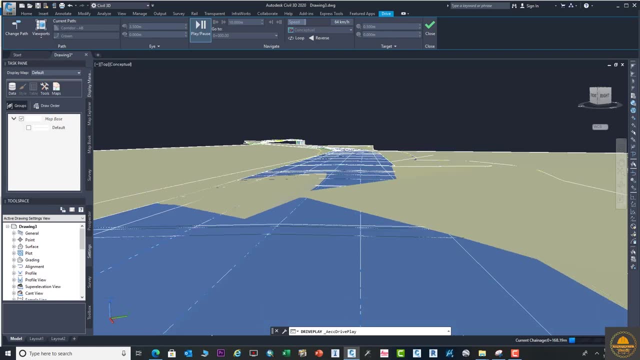 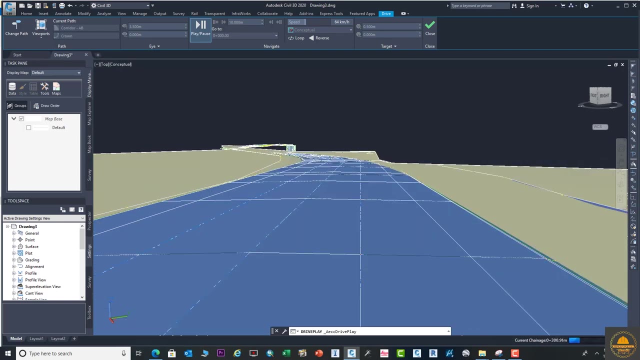 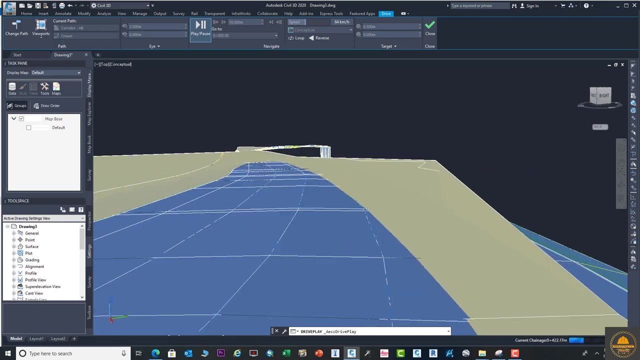 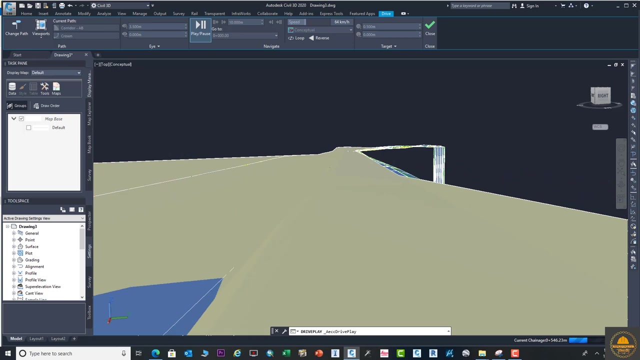 now you can see. this is your road corridor which you create, and from here you can easily see where is your cutting, where is your feeling, where is your finish level. this is your road corridor. very important. these things usually you can see. okay, you can stop and close. this is from the option which you see on the screen. 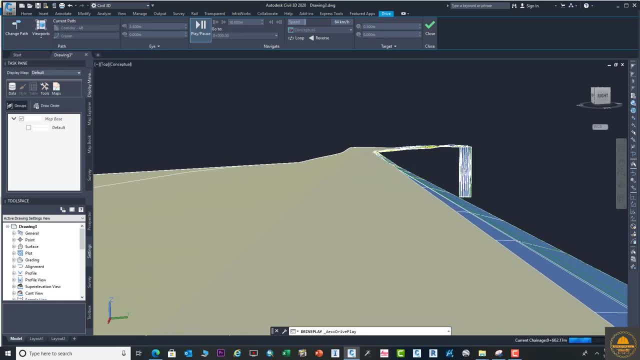 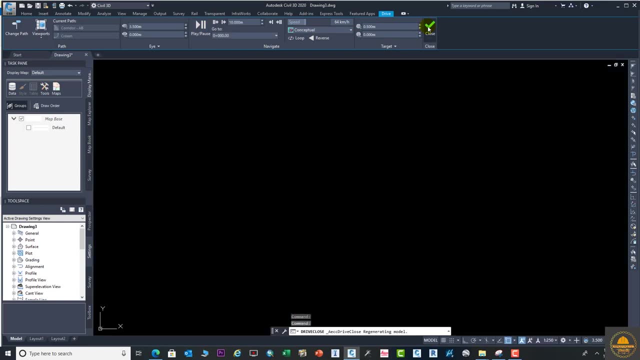 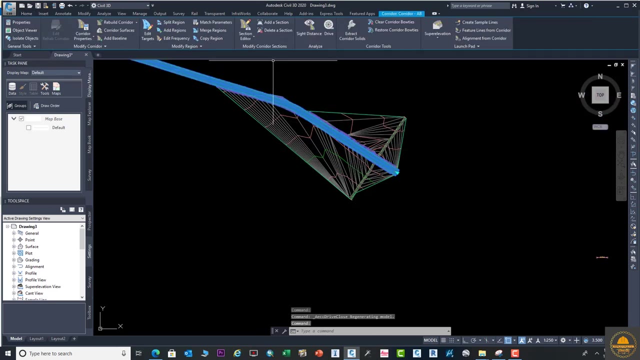 top. okay, very interesting this thing. let's close this one. i close this. okay, hope you guys understand from this. now we need to select this and go to this option selection editor, where i want to show you something. go this option and edit view report. from here you need to select vertical, here you need to select the plan and here you need to. 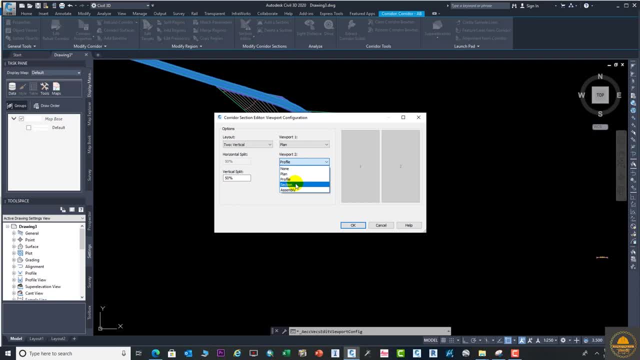 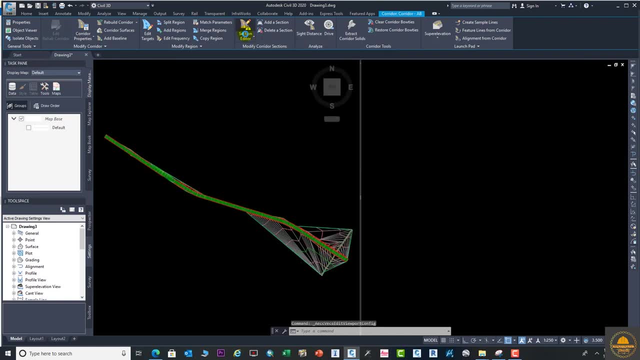 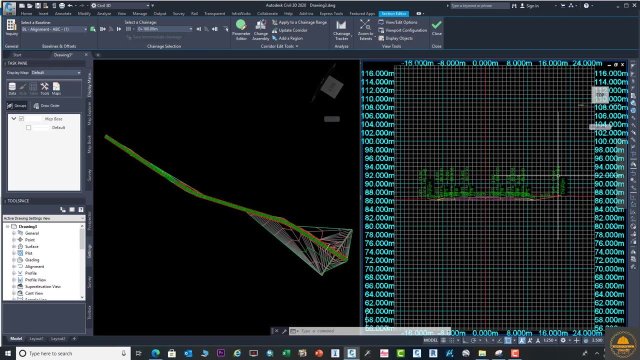 select a section. now you can see your section view of your about corridor. if you click on the corridor, this is your view of a section for your road corridor. you can see this edge and everything. how much is the average left and right and from the one is zero is the center and left and right is. 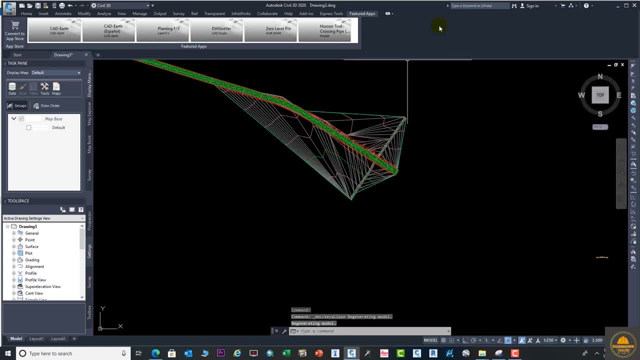 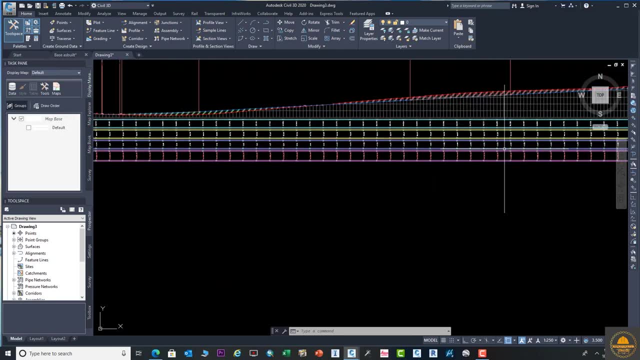 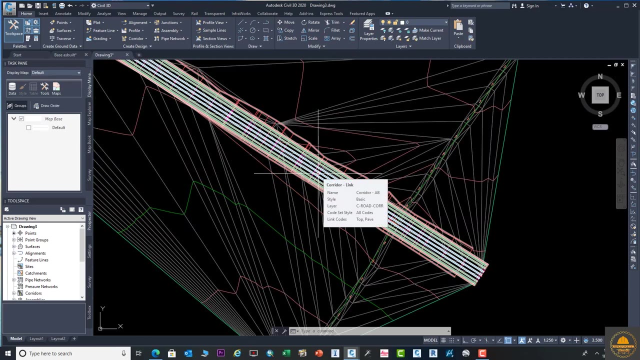 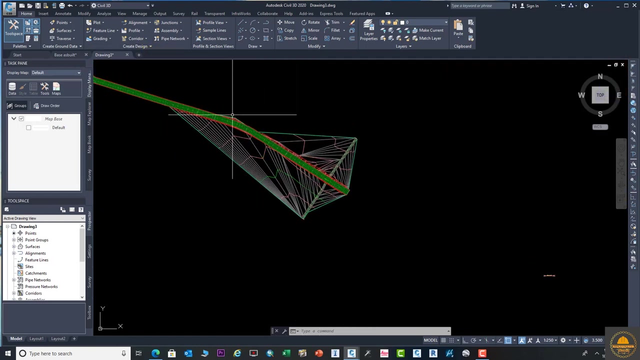 the width and levels up to where. okay, in this all step, we will be create our corridor surface, all the things. our requirement is finished, so we need to add a corridor surface to our corridor. let me just click here. yes, you can see. you want to zoom here? 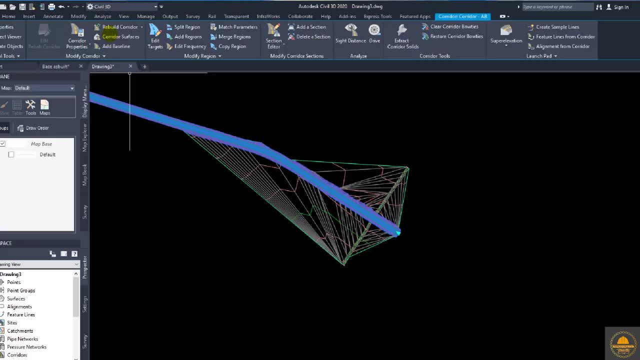 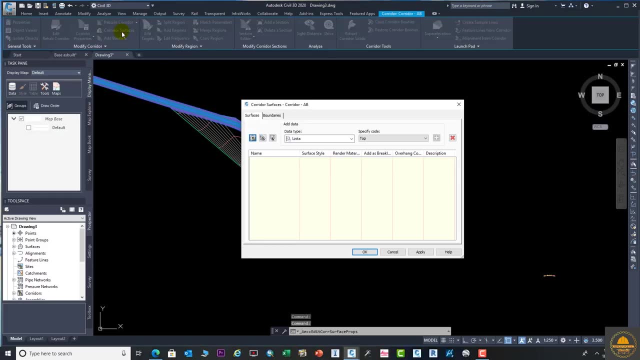 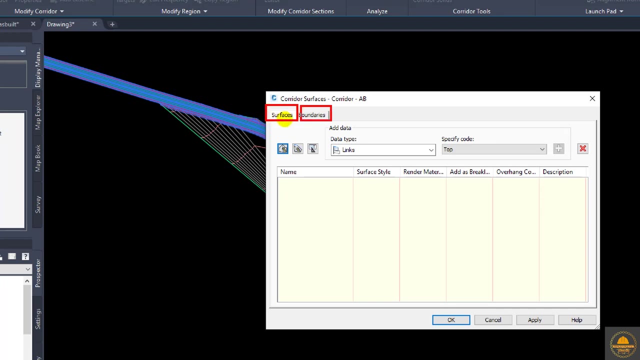 okay, select this one and you can see from here the corridor surface. we will add our corridor surface from here, from this option. we'll go to this and click. the pop-up menu is on. here is surfaces and boundaries. on these two options. we will explain this. okay, and go to this option, the first one. 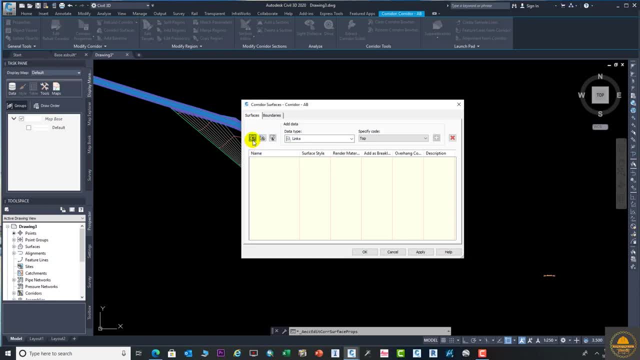 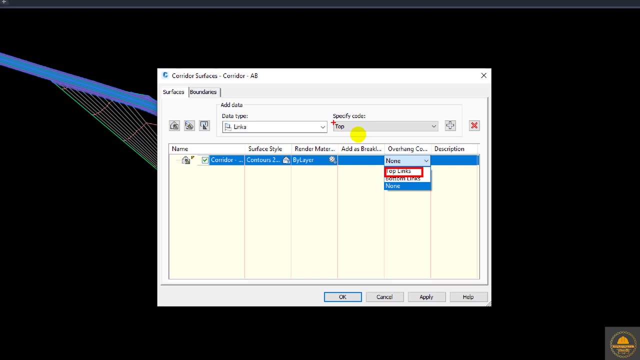 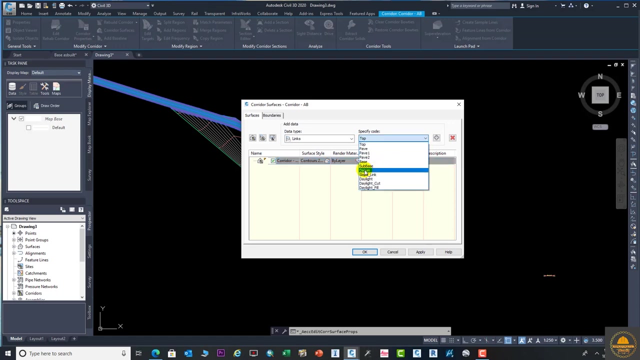 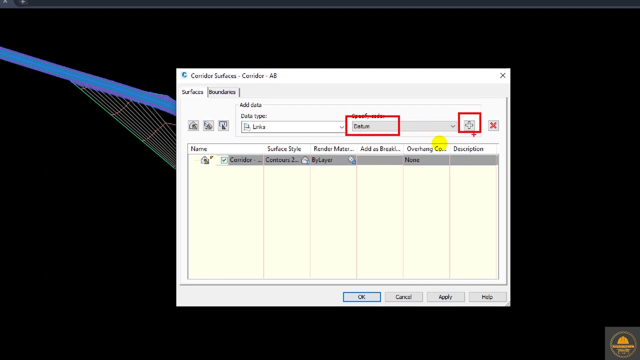 surfaces and here you can see, create a corridor surface. click and your surface is added and from here you can select the stop links. okay, let me click this. and from here again you need to add. plus button is meant to add, so select here the bottom. okay, the dot is here and the plus button is here. okay, and click and pop link and add. 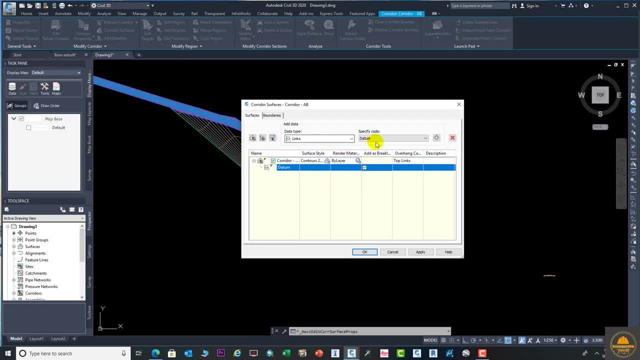 click this tick mark and here you can enter the boundaries. this is our corridor AV and go to add automatically to this option daylight. you need to select the daylight option from here. ok, now this is added to your surface. apply. apply for here and here you can see the message rebuild corridor surface. if you once click your corridor surface. 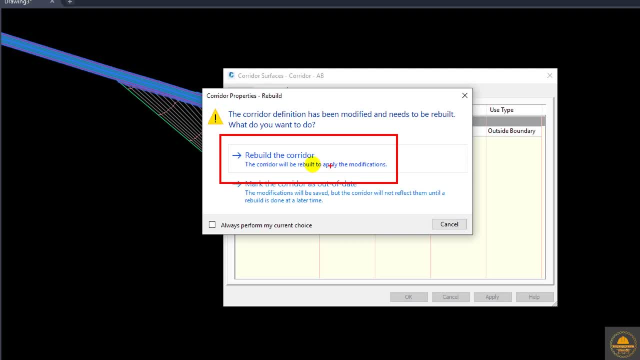 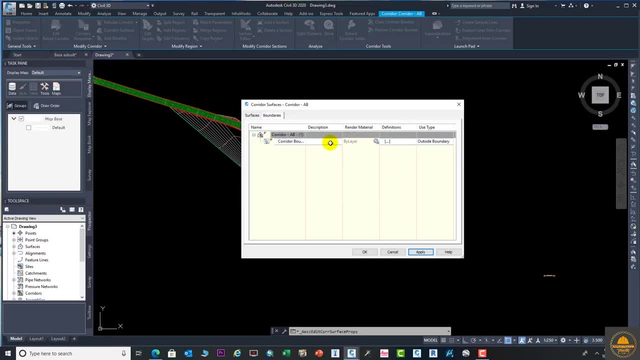 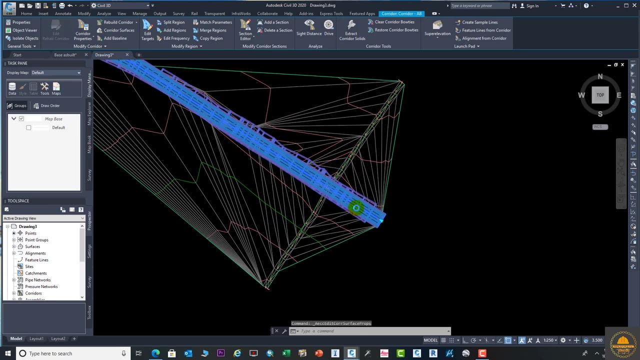 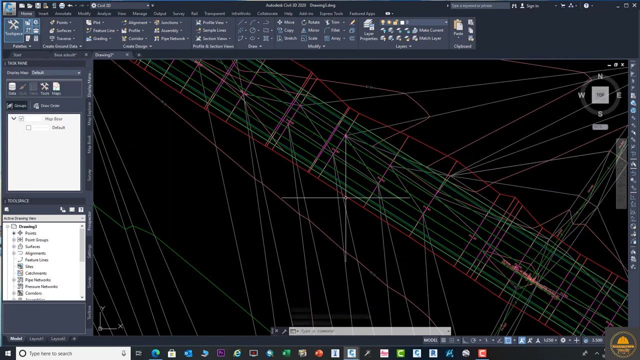 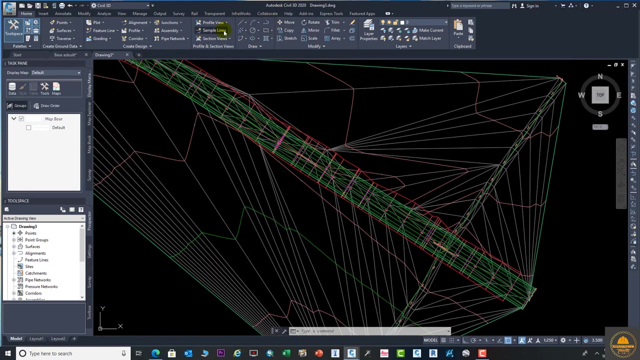 will be created. ok, and click this and apply, and ok, now you can see here: your corridor surface is added to your corridor. ok, the next step. we will go to the sample line. the step is cleared. we will be added our sample line, the sample line we need to create on the alignment. 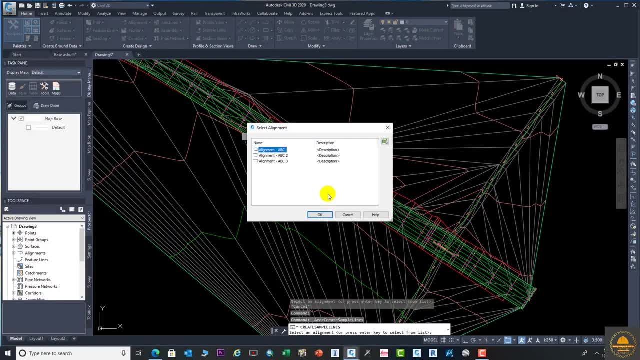 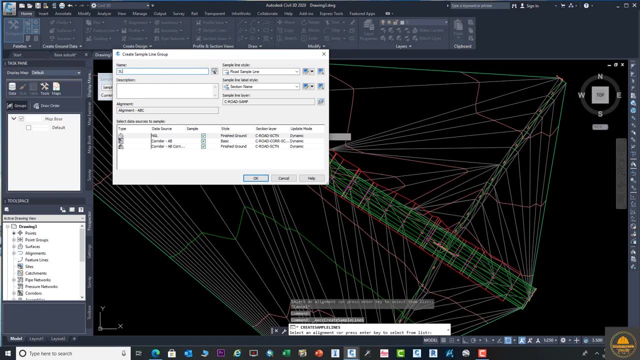 ABC sample line. if you create the sample line, your each sample line, you can create your section and you can view your cut and fill details here into the sample line name, suppose SL1, and from here you need to select: this is finish ground and ok again. ok, the pop up is open. 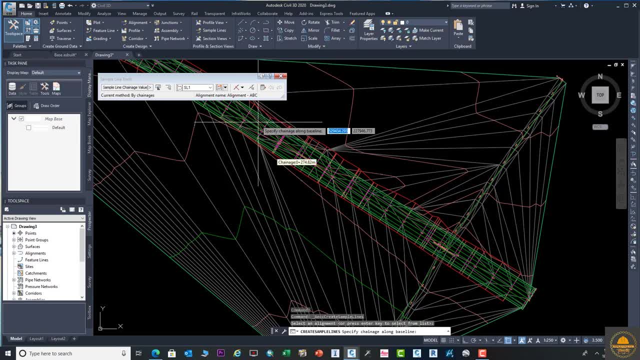 and from here you need to go to this small icon and here select a range of challenges and click on this one and here you need to enter your challenges range and here you need to enter your challenges range and you can select it. ok, now if you want to go to your 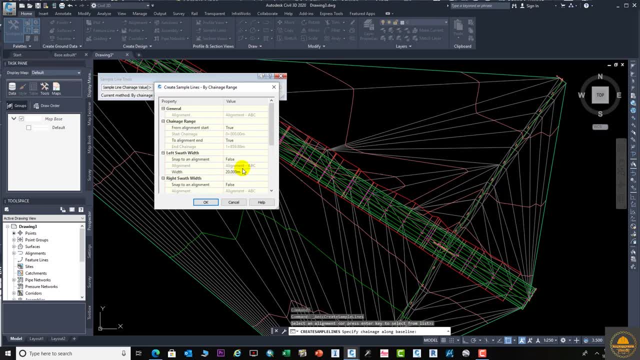 sample line. you can go to your sample line name and here you need select the range of how much is your channel range? suppose this is 20 meter, 25 meter width. you can change this. your cross-section detail, which is required to you. okay, where you create your sample line. under each sample line, let we will create a cross. 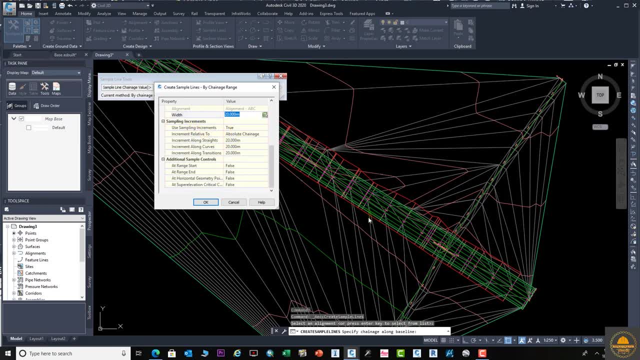 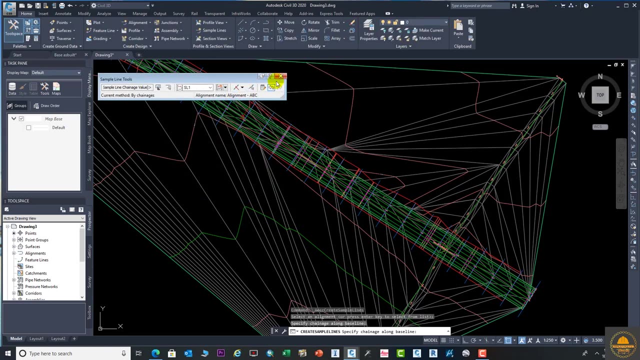 section and you can check the cross section detail. cut and fill on each cross-section easily. you can calculate your volumes from there. here you need to select the start and end with true option. before it's with the false, apply and okay, and now you can see your sample line is created on each chain edge. okay, and the. 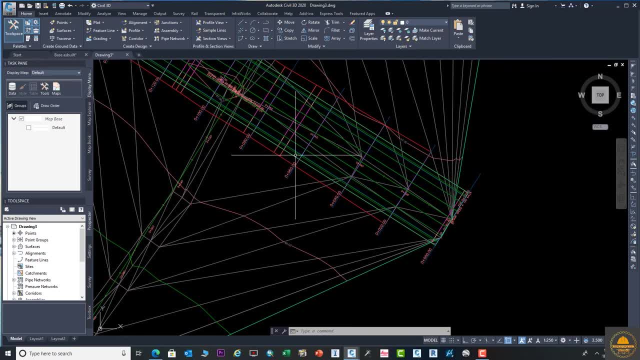 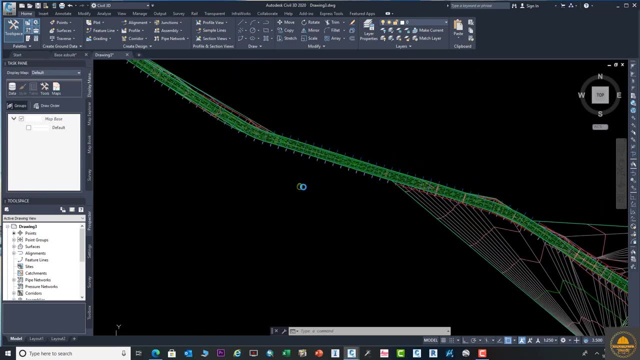 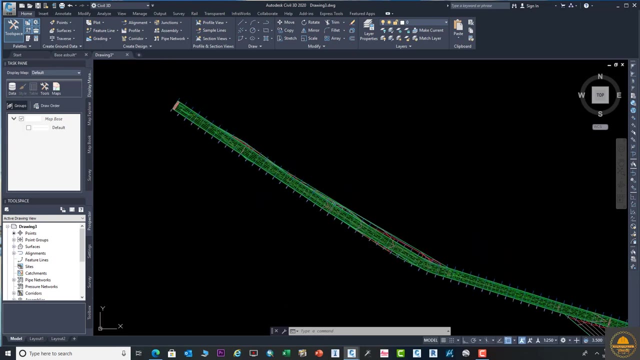 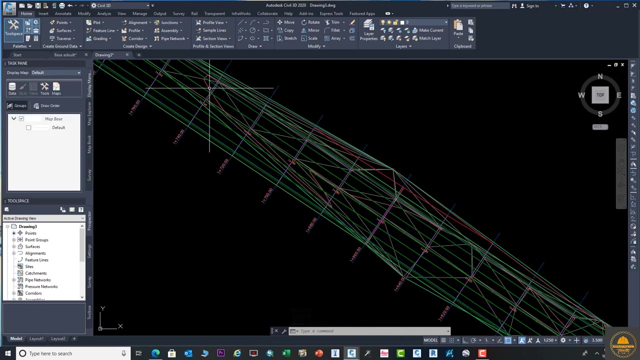 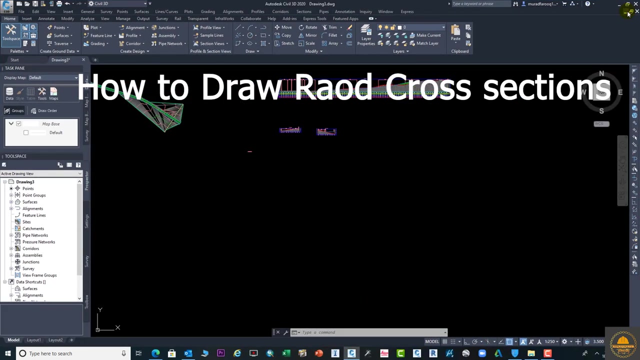 same chain edge. you can also get the cross-section without sample line. you cannot create your cross-section, cannot able to create. sample line is here throughout. or alignment changes are each 20, 20 meters. okay, this one, this option, very important step in this step, we will be create, or 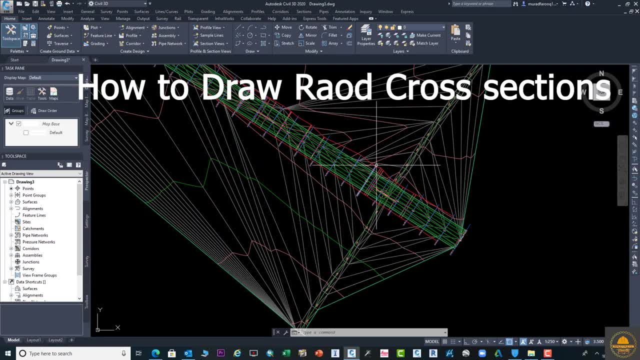 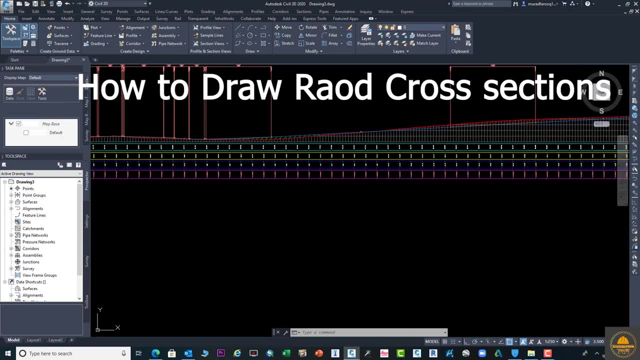 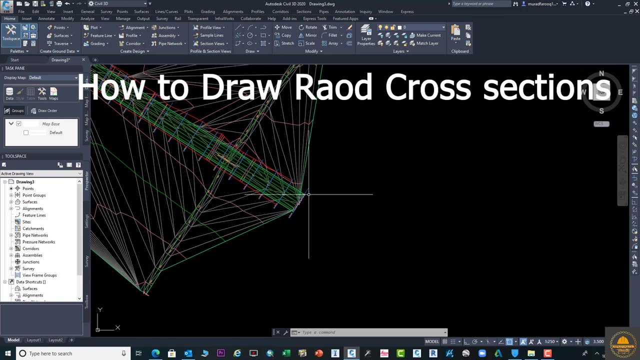 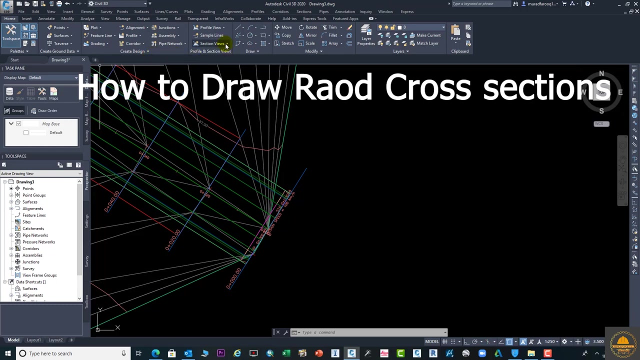 cross-section. this is the important step on each a simple line which we create before we create a cross-section on eachthen edge and 20, 20 meter. okay, this is a sample line. you go to the option. this is the section view. here is create a multiple views and here is create. 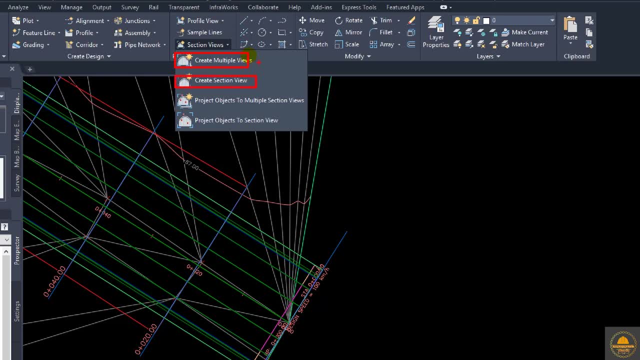 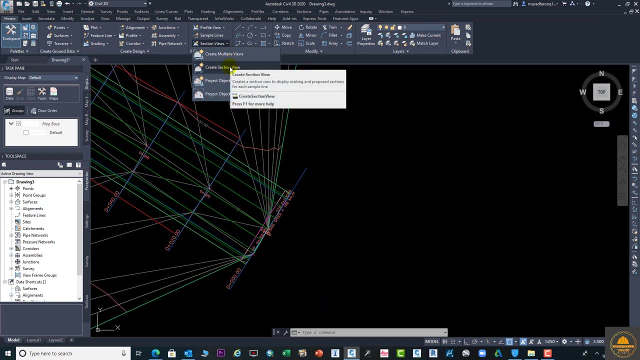 section. if you need, on each image you need to select the first one option. if you need to need an only one, you can create an. only create one section. you can see here. the details is here. okay, here you will see the same thing. you will follow a process. 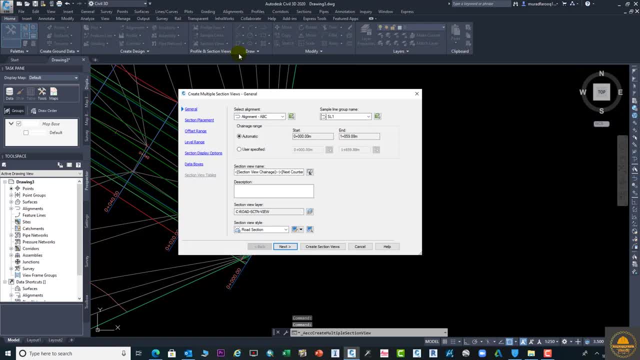 very important and click now. the pop-up menu is open. here you need to select your alignment and which alignment you need. definitely we have only one alignment, we have three, but, uh, we create our sample line and one alignment and we have the sample line group one. if you have few, you can select your sample line on which you want to. 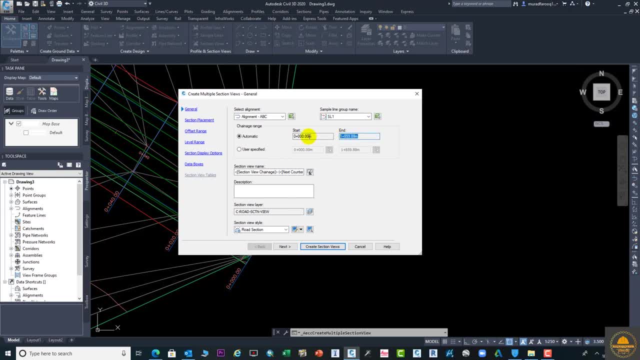 draw your cross section. here is the automatic option and which change to which channel you need the cross section if you need, so you can select. this is as per your requirement and user specified change to change, but we need to on all and then then select the automatic option. 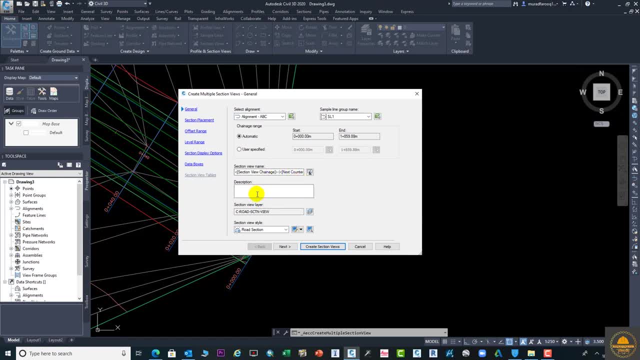 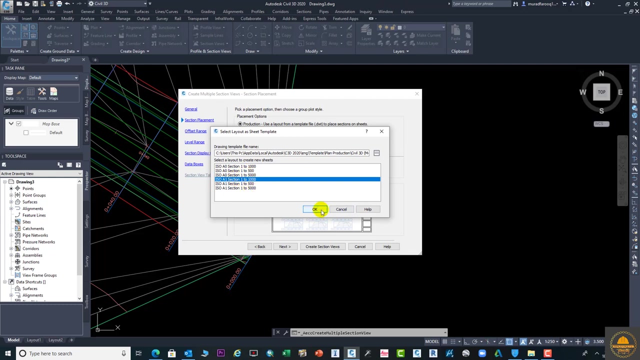 okay, here is section view name and you can select here description and here you can add the layer and here we need to select road section and next, okay, so this is the option. from here you can select the scale, layout, scale and you can click ok and this option. 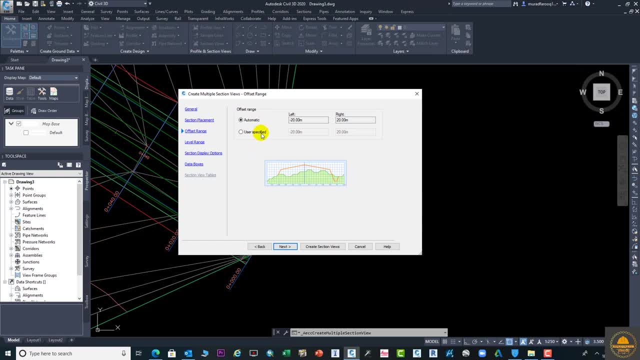 okay, we can also select this user specified. and here you can select left, right, how much, how much you need in the details: automatic and next, and here you can use a specified if you want. enter this one: okay and automatic and next, okay. here you see these all details. uh, if you want you. 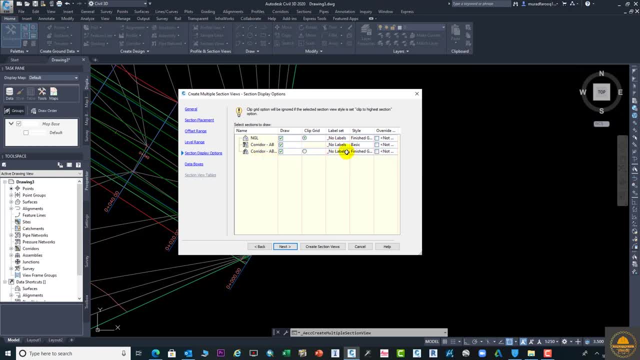 can change this. go to the potato ab and this one. select the finish ground from here. okay, here we need to end the existing ground, the first one and here basic, sorry, okay. and now we need to click this. one assembly is a view edit. we need to enter assemblies as a view edit- okay. 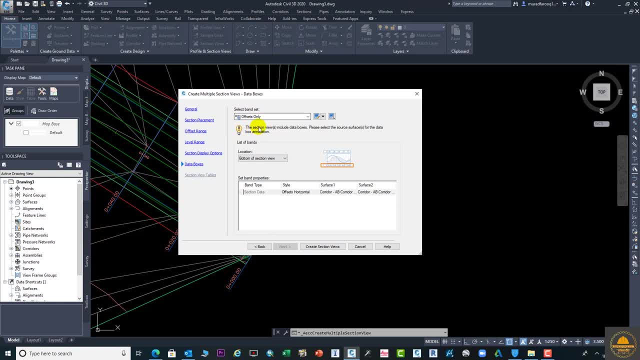 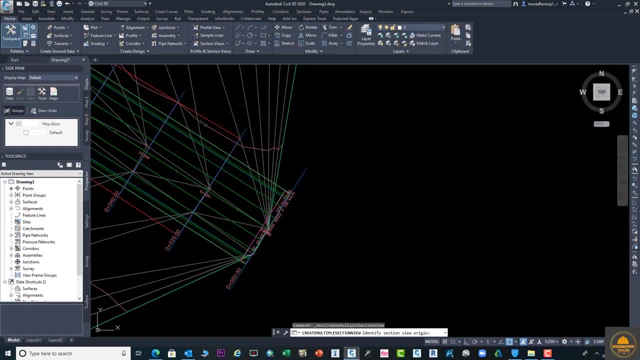 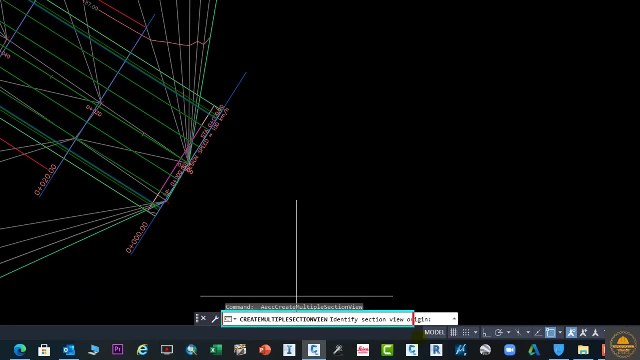 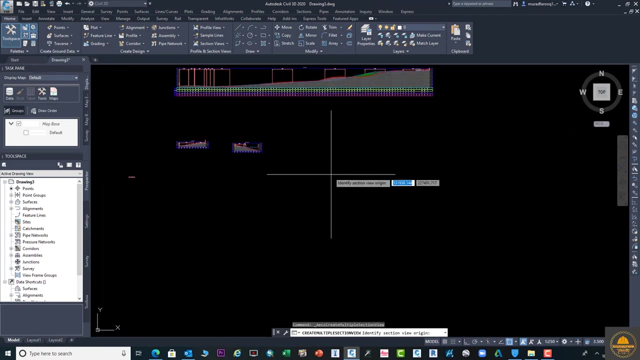 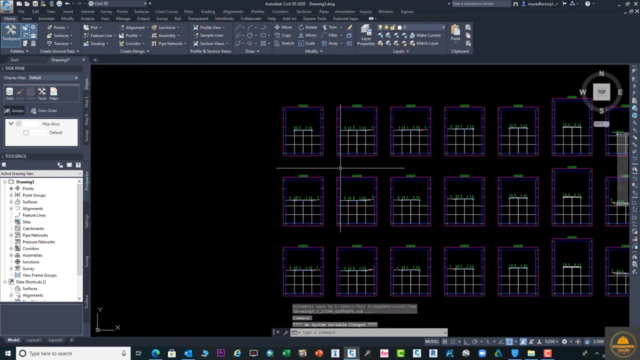 and click on next and from here you can select your select band set. but we don't have any band set. we will create it later. here you can see from the command menu: select your origin where you need to draw your cross sections. okay, go to this option and click. you can see your all cross section for each challenge is: 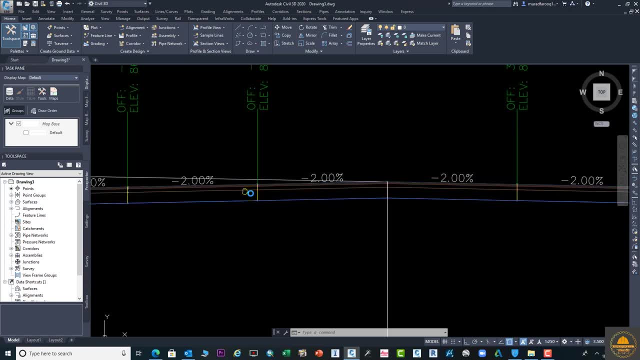 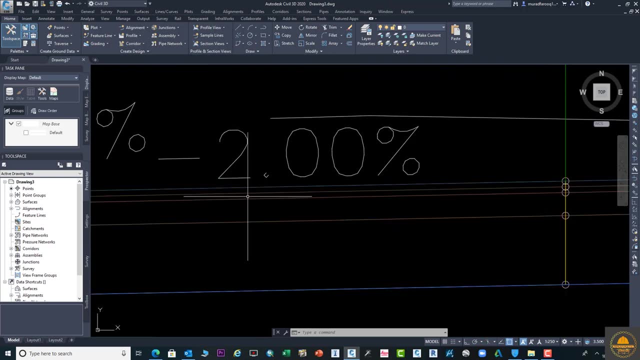 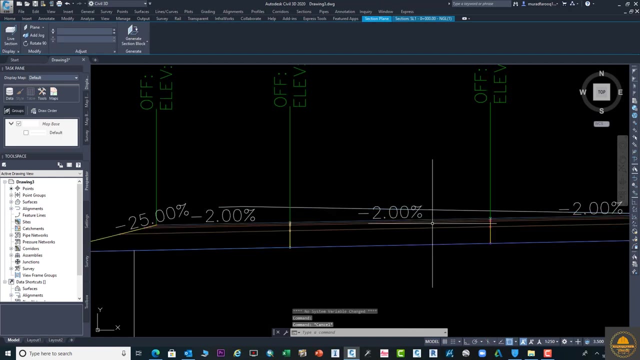 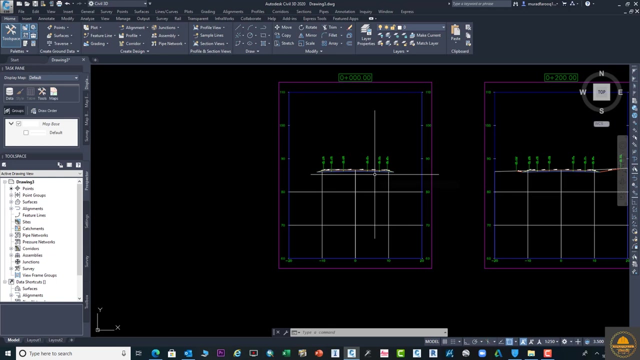 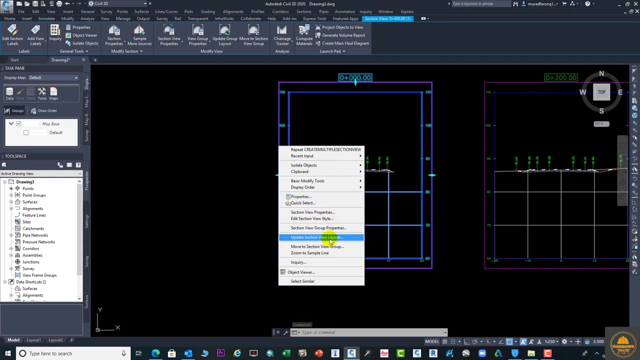 created and draw. okay, you can see the slope. this is all the details which we enter earlier in our assembly: cross row and our width of base space and pair one point two. this is all the things we need to do. some changes in our view? just go to the. 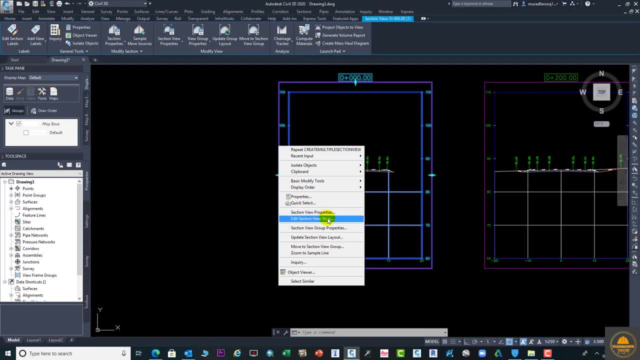 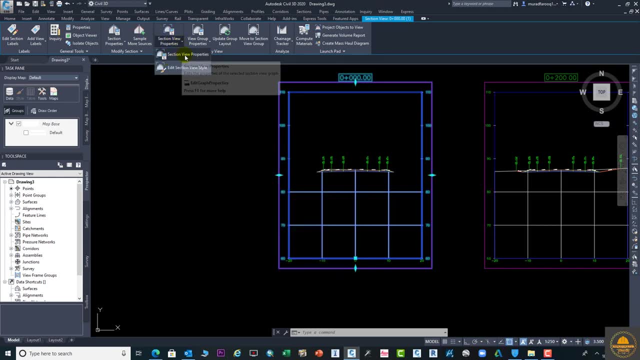 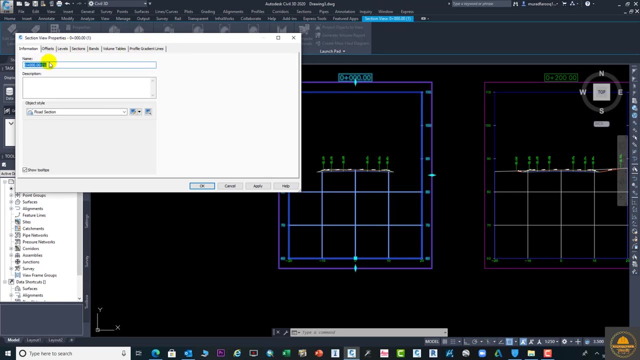 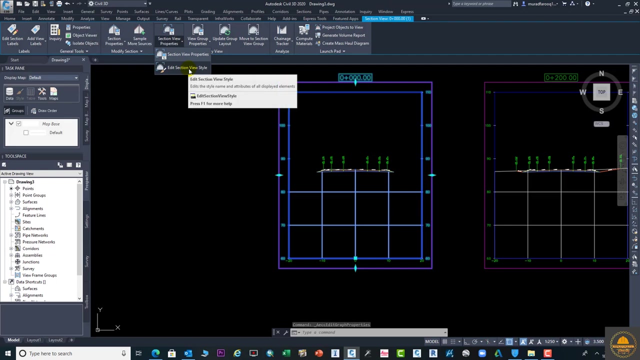 ️ view탄. you can take action from here and you can change the name: available properties. here you can change the name. a few steps and which we need to do and also you can and do. this is from here: go to here. you can change the name of setting levels and section. and from the other option, edit section view property, you can change the information graph. go to from the arrow in the top to the video data. vi accept section and checker section-view-property-edited them. the first property is the section view properties and then選 architects view properties. so if you have any, 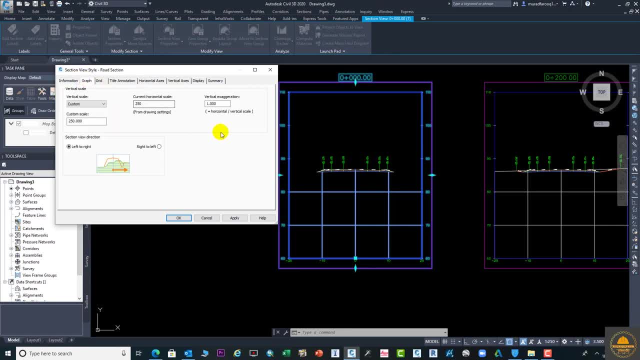 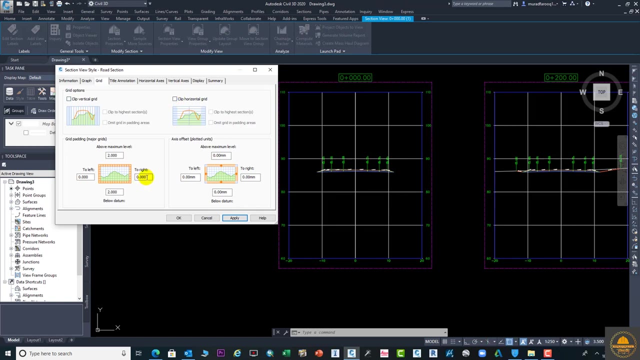 graph and grid title notation. this all information is here. you need to change this one. click this and copy. you can see your grid graph is display on whole cross section on here. you can change this left and right along maximum levels. so it's mean and it's related one by one, but we need to. 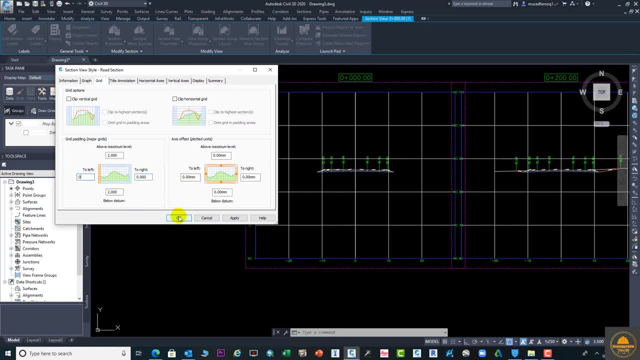 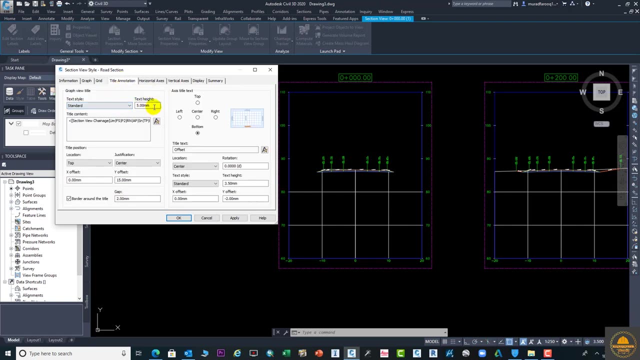 remain, it's on zero. uh, the before view is okay. now we need to click again this one fly and okay. when you go to the title annotation from here, you can do some changes like text height, top and right and bottom in this- some changes. access is title, which will be display on each option. 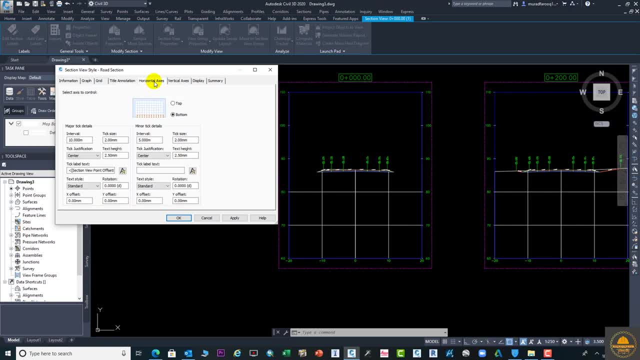 okay, and here you can select the horizontal axis. in horizontal axis you can change the interval between the two points here to here from zero to five on five. ten you can select. if you into five, that will be definitely on five. if you need to enter ten, it should be definitely on the. 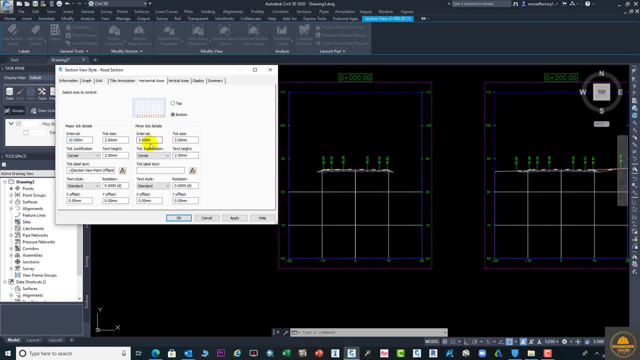 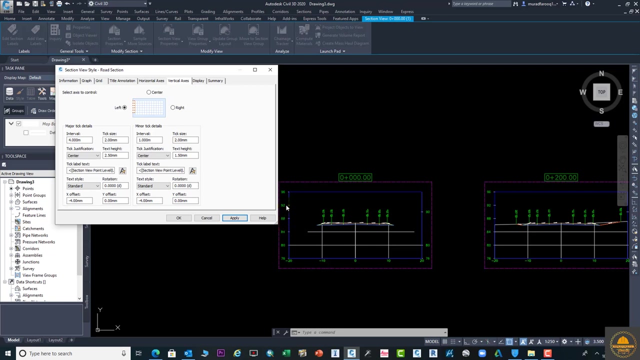 10.. okay, and here you can select the tick size and in the vertical you can change the vertical truth, vertical distance from here to here. okay, just suppose, enter here two, three or four reply what should be definitely changed. you can see. okay, this is known for four meter, you don't need to enter or same. sorry then. 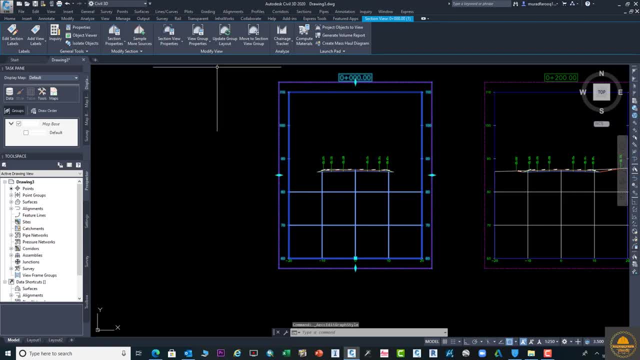 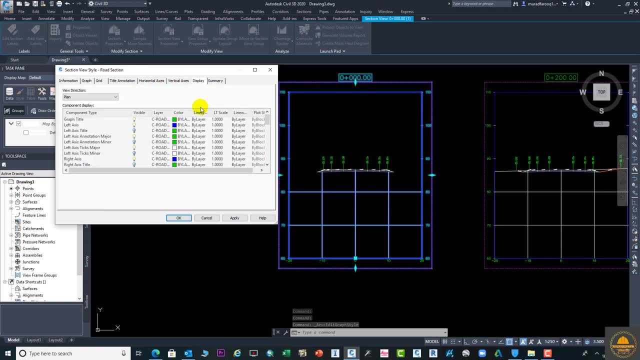 apply and okay, this will be changed automatically. this is some basic change. and go again to this option: vertical axis display. from here you can change your graph colors, your text color, your title colors- anyone need you can change the color. you can turn on the layers, you can. 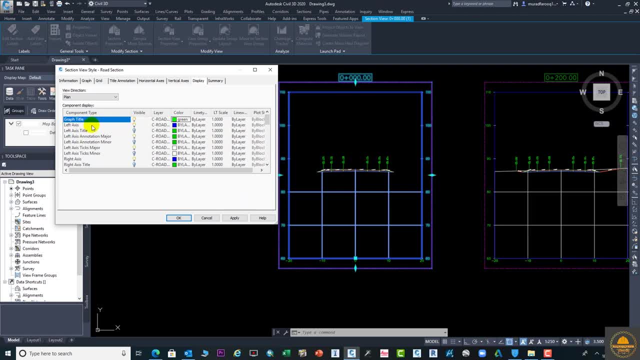 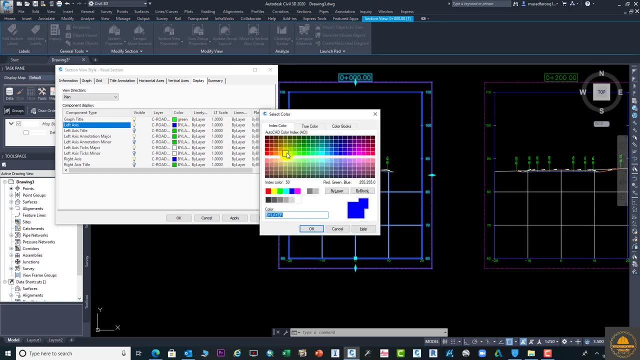 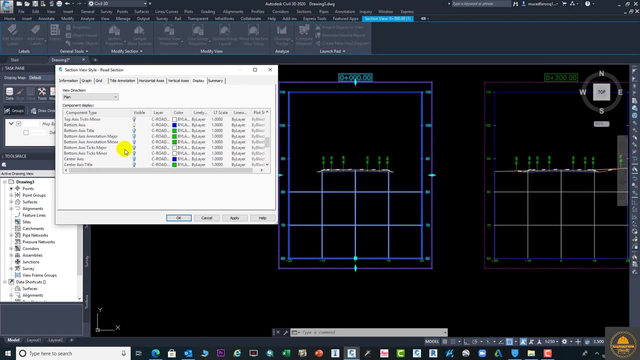 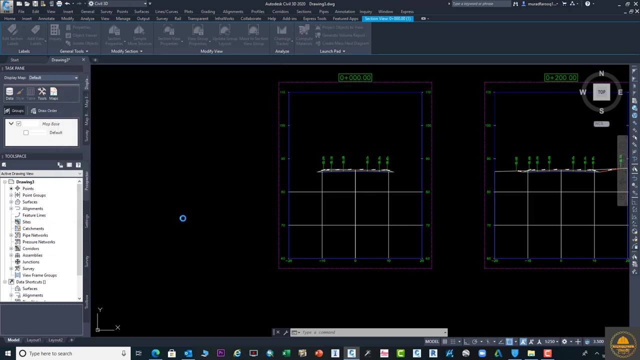 turn off the any unnecessary things left axis colors you can change. if you do your own practice on this, you can be able how to change the colors and boxes. if it's very easy and simple. okay, we just need to change some colors and apply and okay, click on ok button and you will change in colors at display. now, okay, 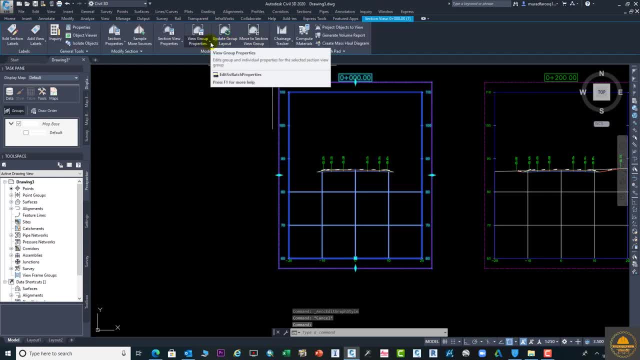 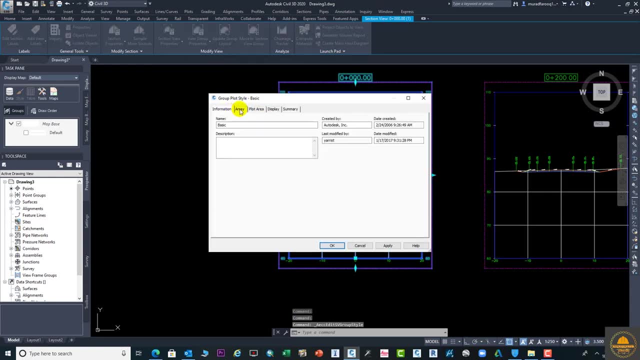 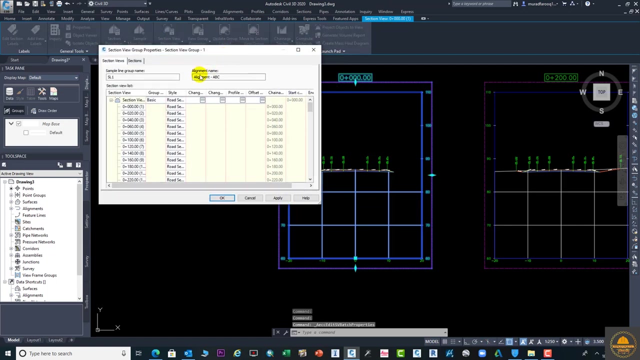 now we need to go to select to this view and it will give you a little bit of a look- and go to the information. there is a plot area display summary. this is the other group plot style- and then again go to this option- yeah, this one. and 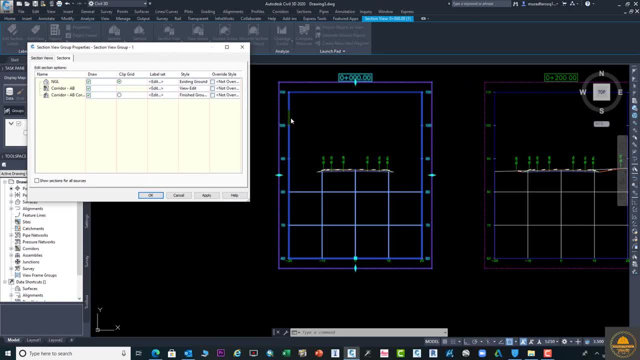 section view. okay, here, just let me clear this option. if you close the view, just let me clear this option if you close this one. and then you can see like this: you close this mgl and corridor ab and corridor abc, your assembly, things will be closed if you. 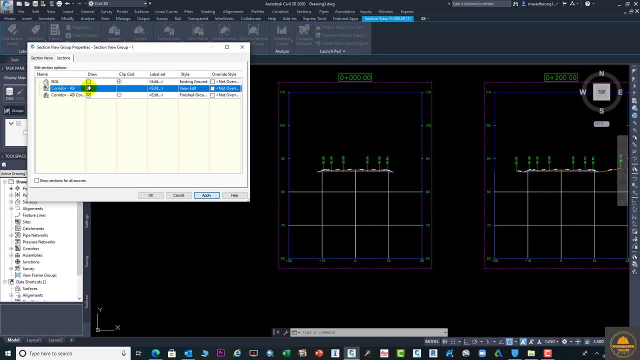 click apply. your this option will be hide, you can see, because we uncheck this. and if you uncheck this surface, your surface will be: and yeah, this one. let me just select. click this one and apply. now your thing is display same as before. from edit view you can change the difference. look of. 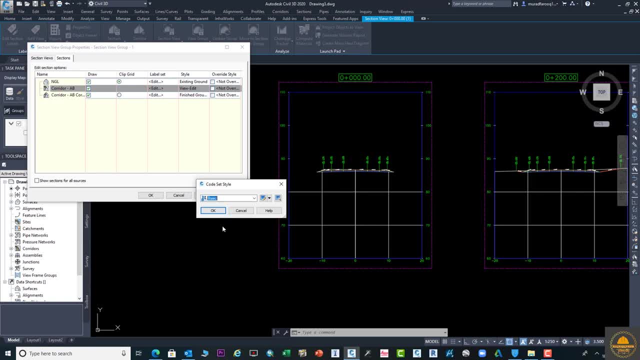 your assembly. suppose you need basic, it will be shaded and the level is hide. now okay, and here we need to select this, all codes. this will be display again the same as apply, and it will be okay from here. you can also select this view and edit. then it will be same as that before. 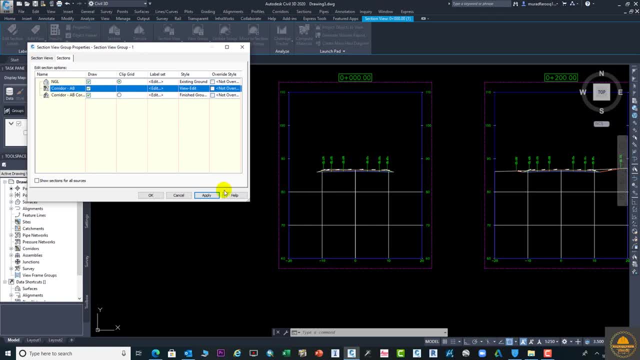 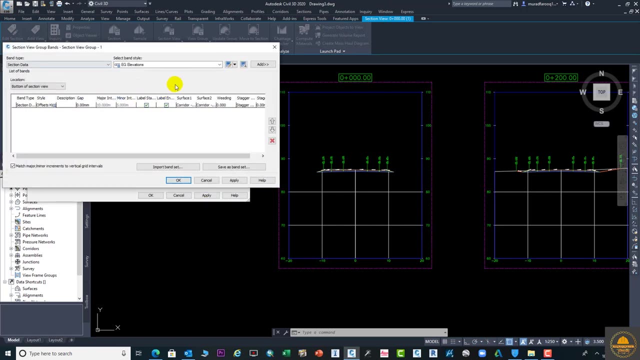 and apply. okay, know your cross section is okay and click on. okay. this is just for the information. if you need any time, as per your requirement, from here just go to the section and from here you can add your bands, as per your requirement, to the each class section. 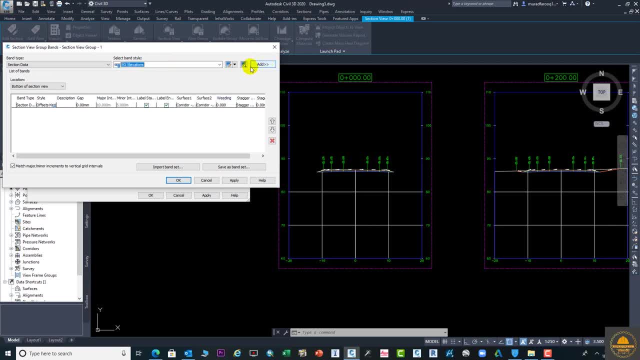 suppose eg elevation and fc elevation, from here you can add, suppose we need to add, and you can also create your own bands, which i explain with the profile bands, and here you can also select the fc elevation band and you can apply this and okay, like and okay. 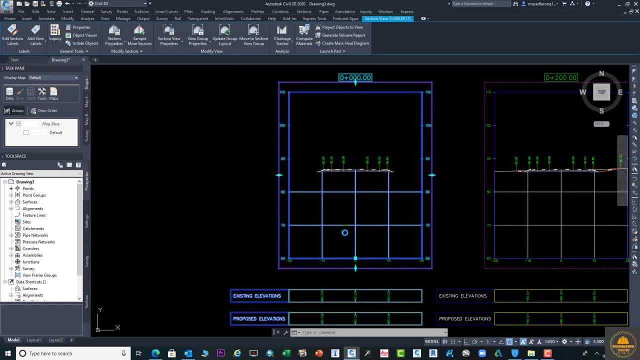 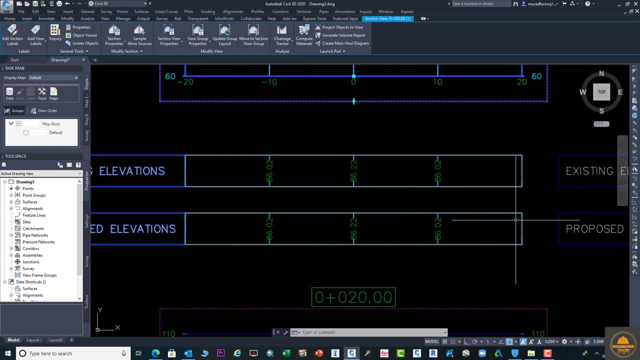 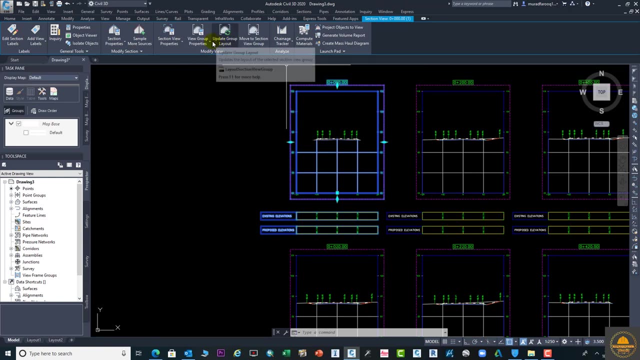 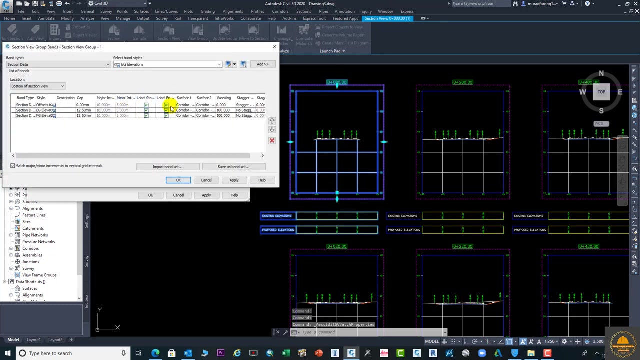 yeah, now you can see, but we- this is your existing elevation- we have few points in our data, three points. that's why the sum level is created. go to the update group layout because we need to update, so it will be look pretty good. and here we need to go again because we need to change our some levels. 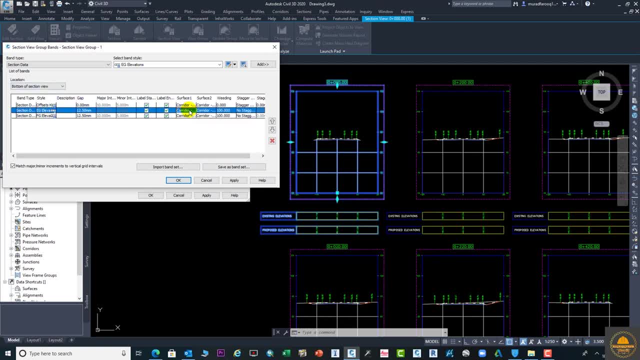 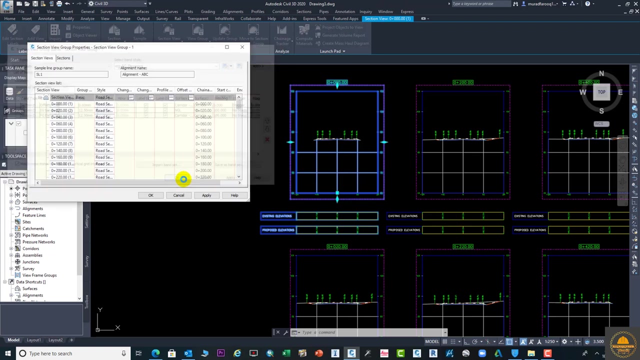 in existing and in proposed, because this is looking same. in one we need to enter the ngl, another we need to enter the design level. then all levels will be looking well, okay, apply and okay, yes, here, apply and okay, click on. okay. so, above all, later we need to check our data. yes, 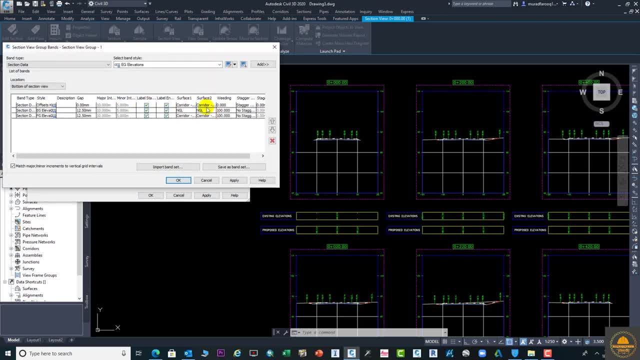 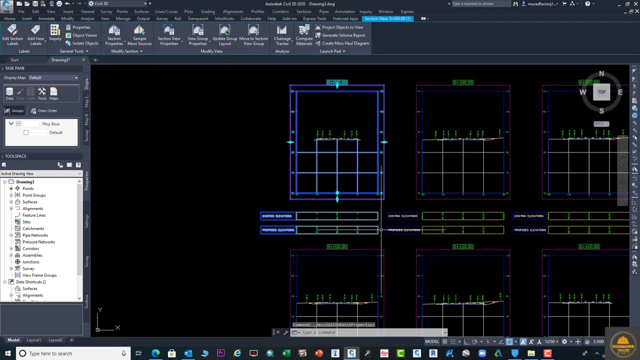 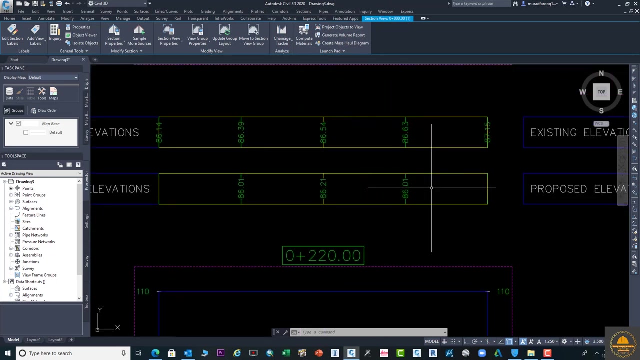 again. for example, you can just use. if you don't expect, then whenever you add anything in your tags, you can add anything as per your requirement. yes, for exampleCSR into this ал extension to work and from here self load. This one is just for one. for other, you can do as a group. when you do as a group, it should. 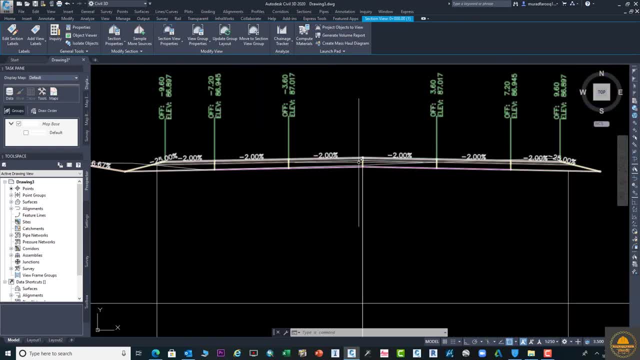 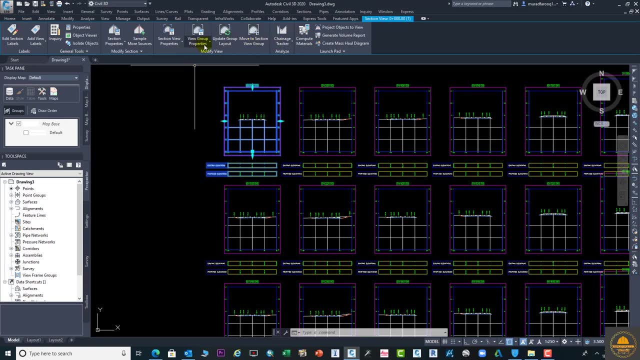 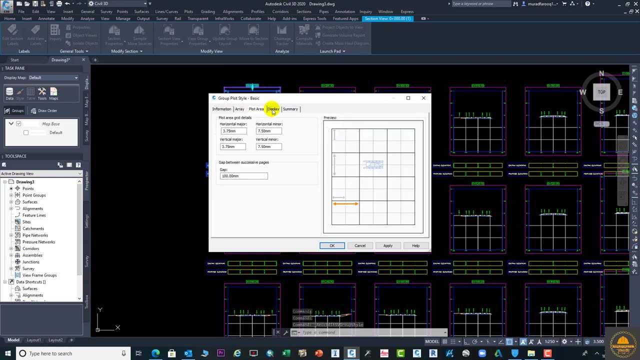 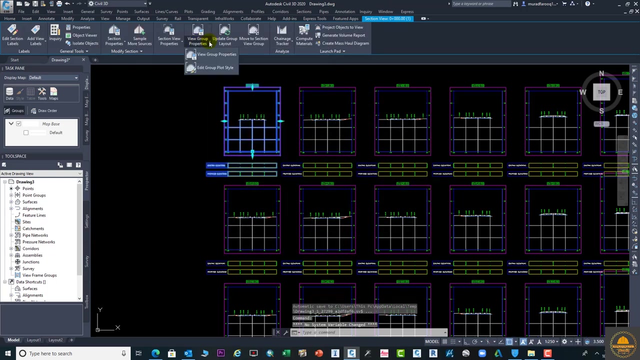 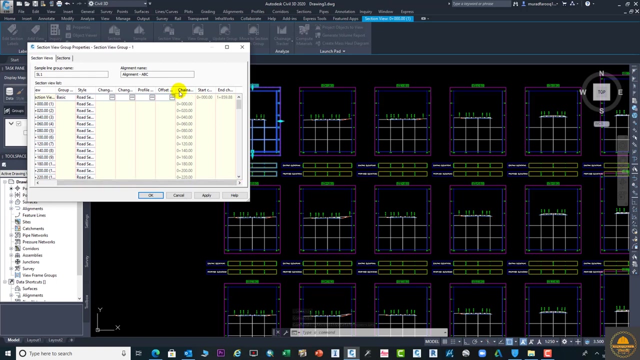 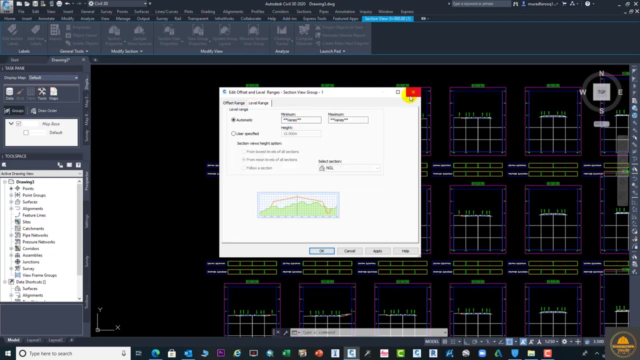 be change in all And go to review group properties, edit group properties and here you can select this plot area, display summary and close this option. We need to go again to property section, view property, and go to this option, offset- Here you can check the level range if you need, and also here is the profile profile. 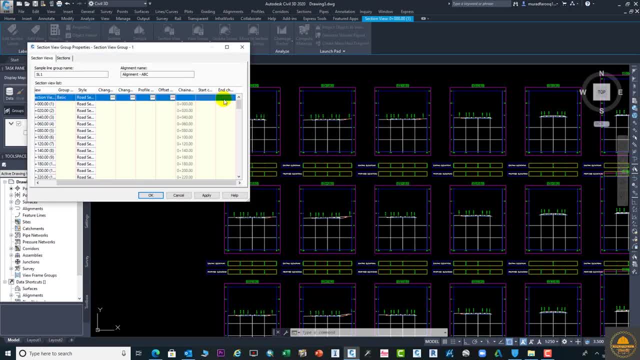 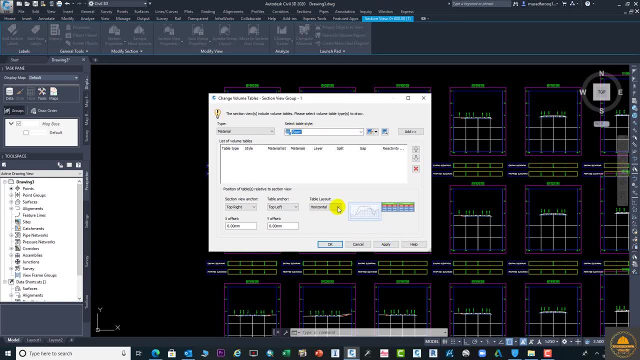 you can. You can add these things and here is the change volume table. if you need to add your volume table to your section, you can change, but first you need to assign your material from here. then you can able to add: Ok, and here you can enter and ok. 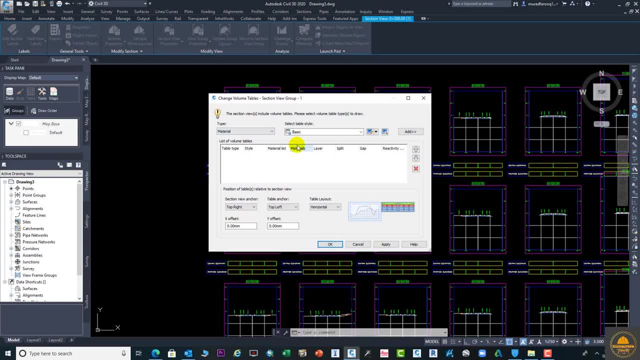 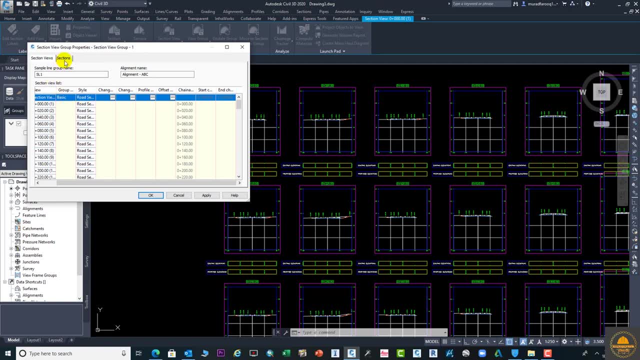 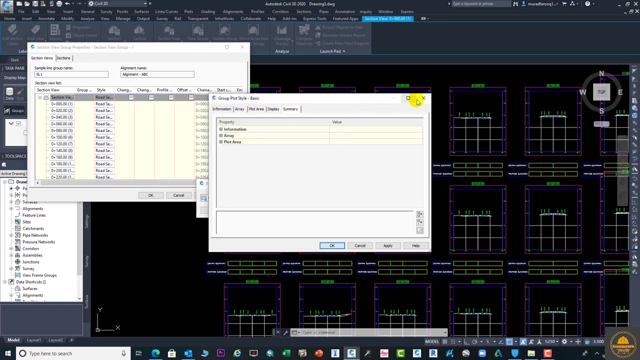 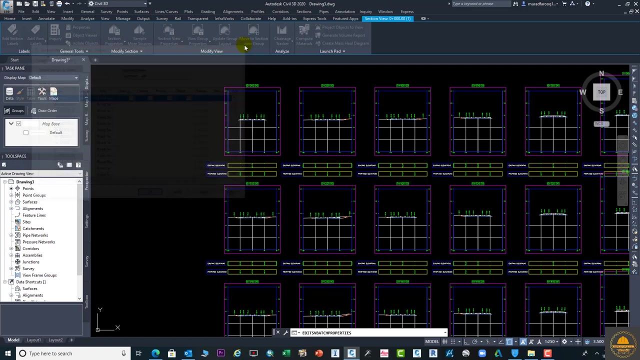 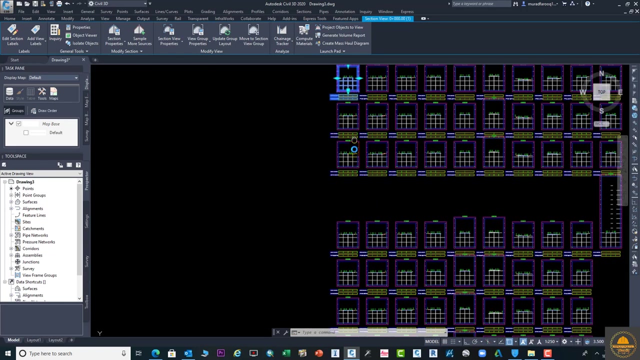 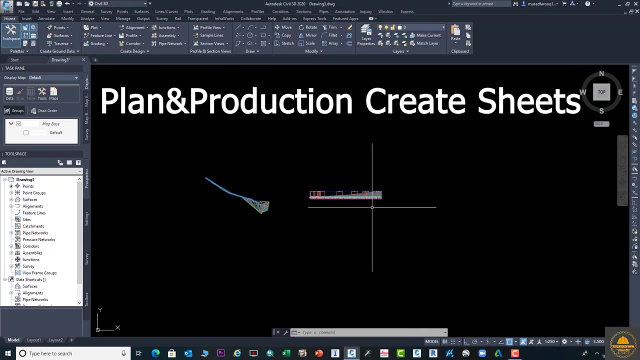 So the next step is Go to section here and go to the basic. from here you can go to array, display, summary, ok, Ok, And here you can see. your art section view is now created. All detail is here, Ok. the last option is: we will create our plan and production. 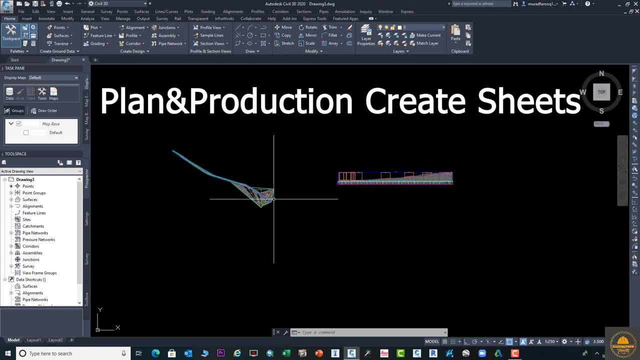 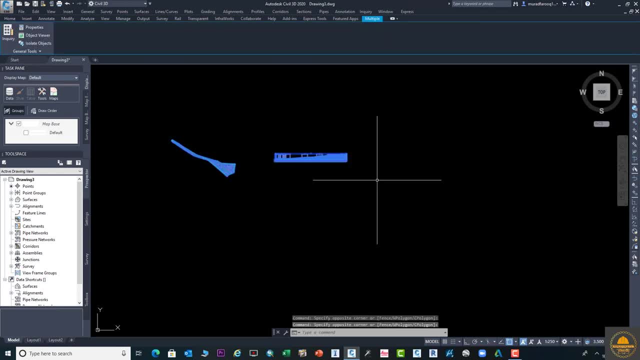 We will create our sheets. I did it some few steps, just I wanted to show to how to do the plan and production. We will bring this on the same sheets And we will create different sheet for this. Go to this option to the output and again you need to go to the create view frames. 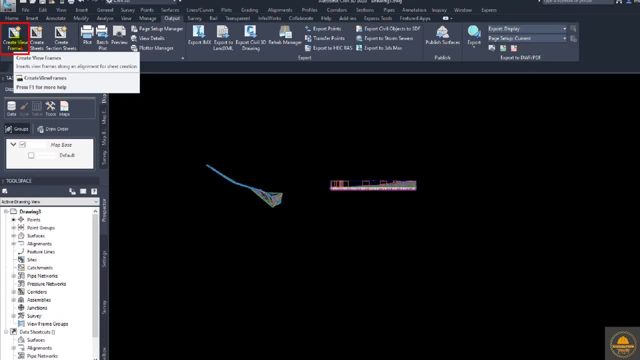 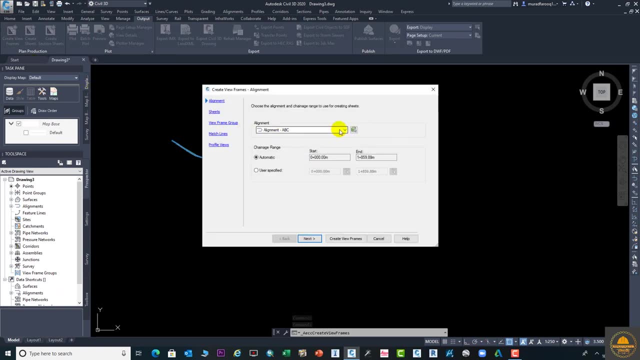 From here, you can create your view frames. Click on this option and go to this. From here, you can select your alignment. Definitely, we have three alignment and we need to create- This is on the alignment first- Which one is our main road? 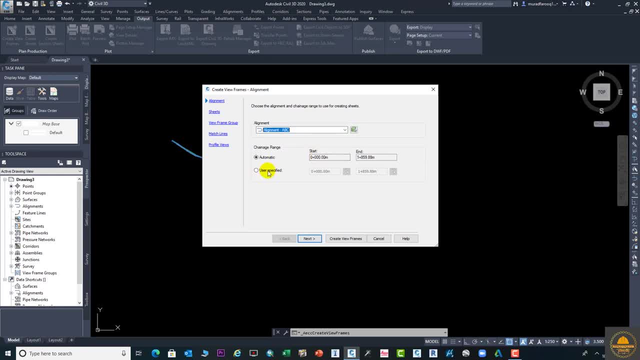 ABC, And here you can select this as user specified or automatic. But we need to remain this same as is with automatic, Because we need further total alignment plan and code sheets, And this is the important things. You can select this plan and profile from here. 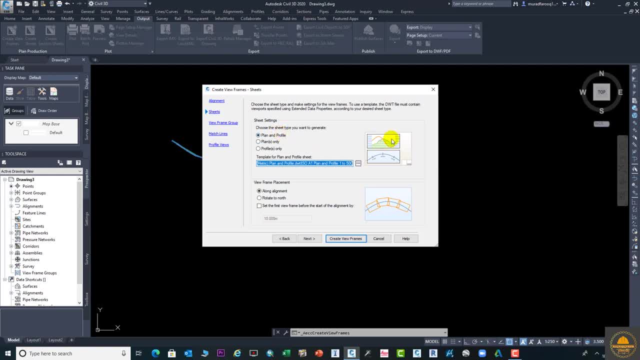 If you need only plan, you can select only plan. If you need only profile, you can select only profile. But we need both of them: The one sheet and one page, And template. here you can select the template from here. Just go and select the scale, or you need to go to this: three dots. 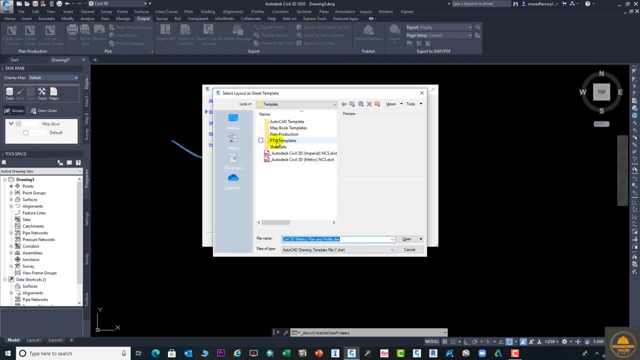 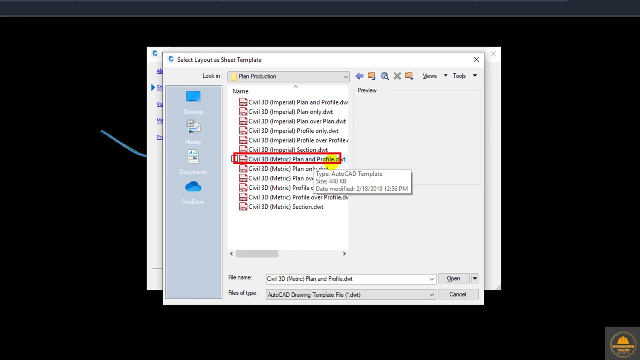 From there, you can import your template. Go to the plan and production option- This one is SEO3D folder- And go to the metric one, Because we are doing work in meters. Go to the 3D metric plan and production. Let me select this one. 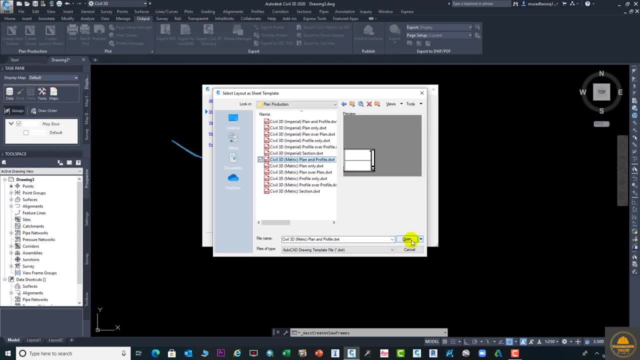 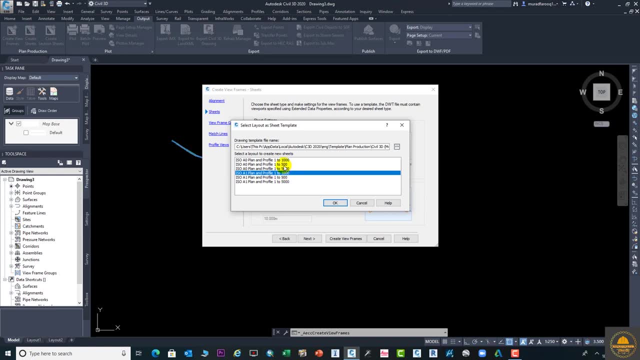 And click apply And here you need to select your scale And which scale as you need And suppose you need to select the one into 500.. Okay, And click on ok button And from here you need to select this view frame. 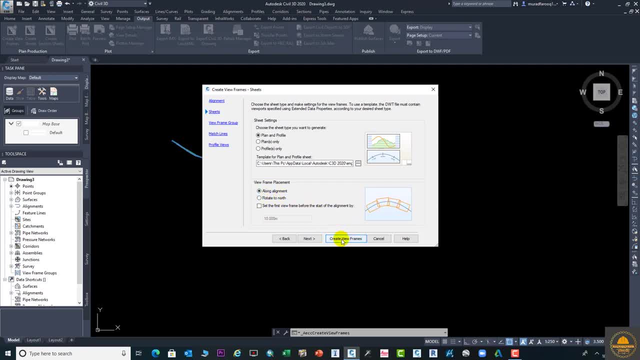 Rotate to north or along with alignment. We need to select along with alignment. And the next step. Here you can enter the name, Here is description, Here is layer And here again name and basic. Okay, Here you need to select the basic one. 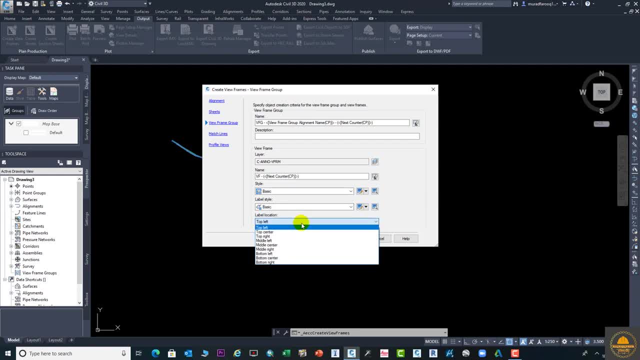 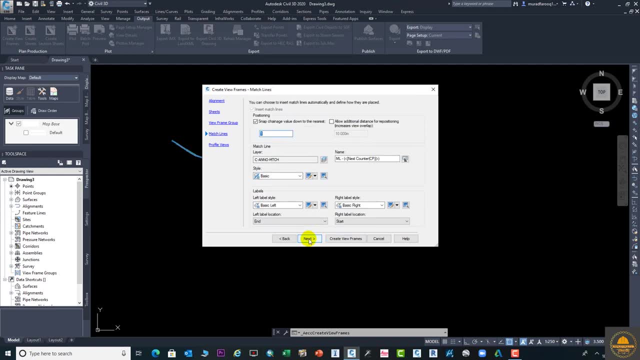 Okay, And here you need to remain it same, as it is: Top, left and next. With this click again, next Date come back And this one is okay. Just we need to do some change here And create frame. Now you can see. 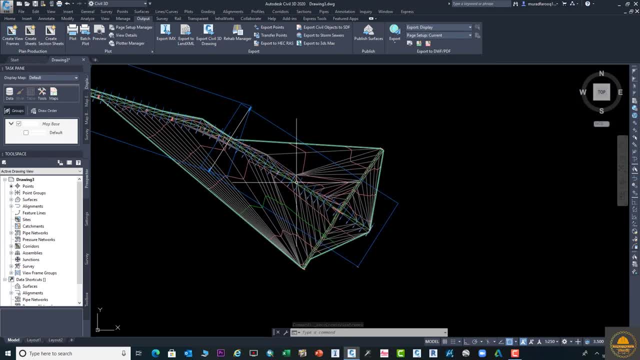 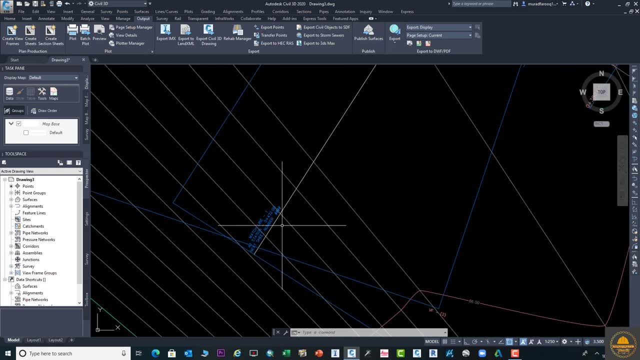 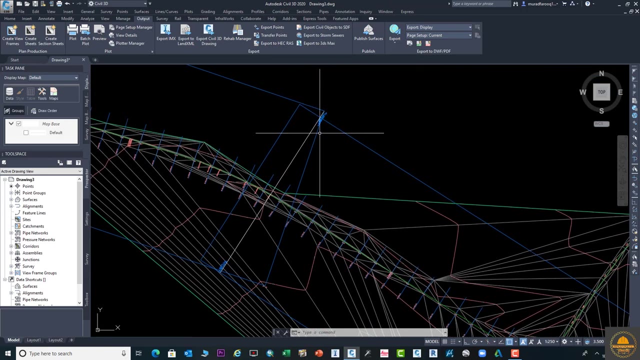 Your frame is created here. Here is your some matches. Where is your frame And the same frame. your detail will be In one sheet. Here is your match line. And this match line you can move as per your requirement If you want to fix on some specific change from where it need to start. 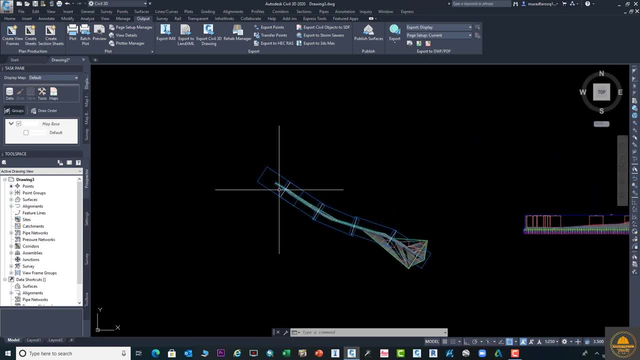 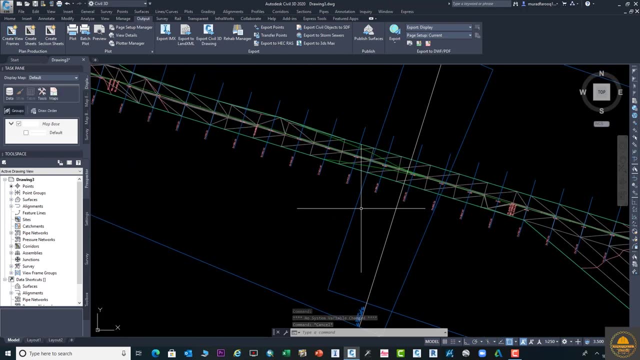 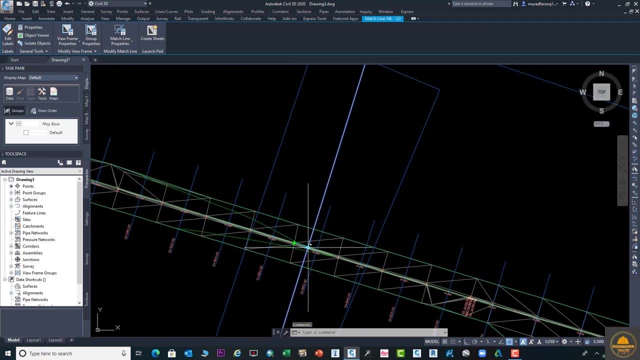 Then you can change this. Once you click, You can move this very easily from one place to another. Okay, Suppose We need to click here. You can move it right or left From here. From this icon you can select here. 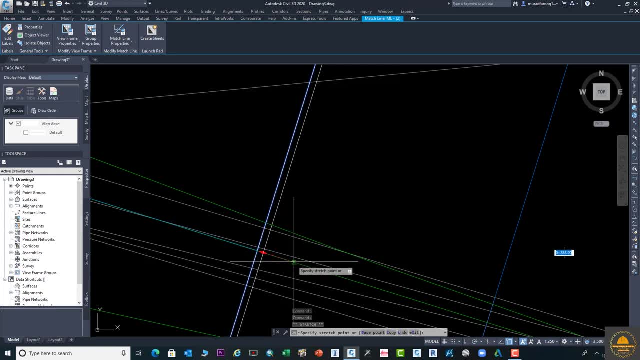 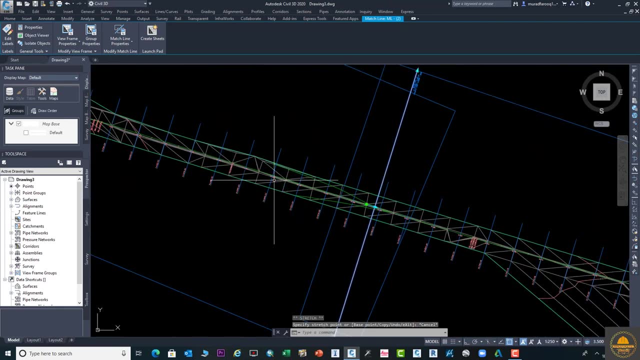 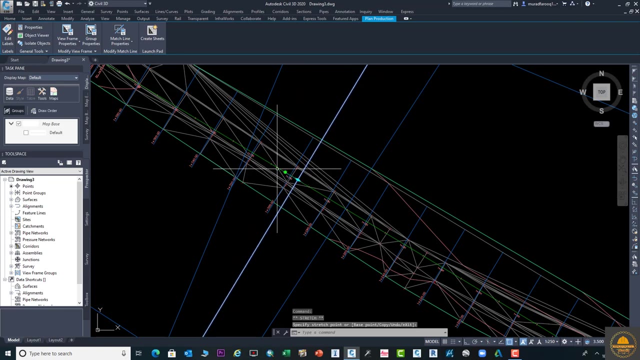 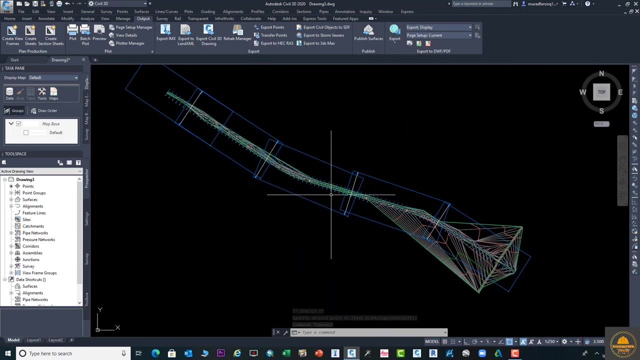 You can move your match line from here to here, But we don't need to move And you can set it as per your required change. Okay, Also, you can move this From here to here, To left, To left, And you can set it as an unchange. 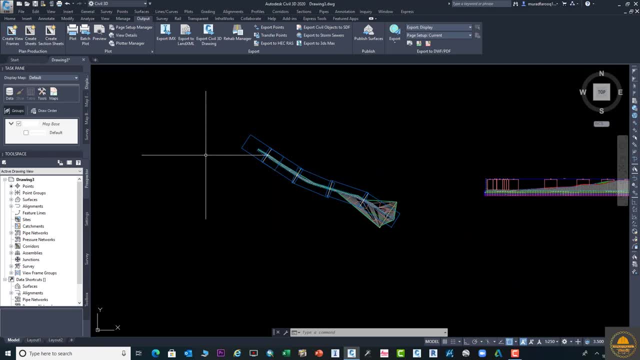 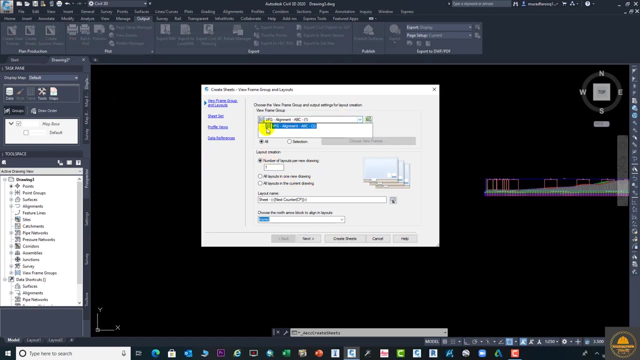 So now this our frame- is created, We need to create our sheets in same frames. Go to create sheet And click Here. we need to do some changes. Upup menu is here. Just select this first one And on you need to. 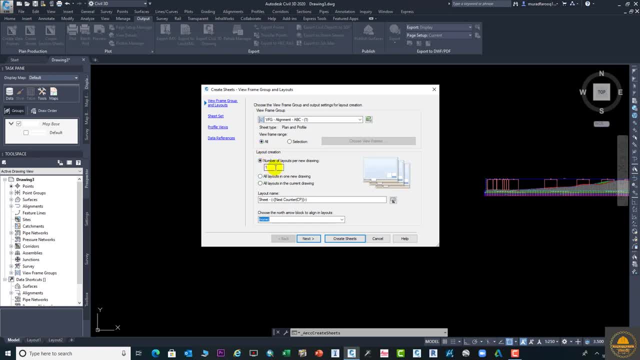 On all you need. how much is number of sheets, for each sheet will be number. if you need to do 10 numbers, then, but if you need to do one numbers, we need only one copy. and here this is important. you need to need a new drawings or you need to. 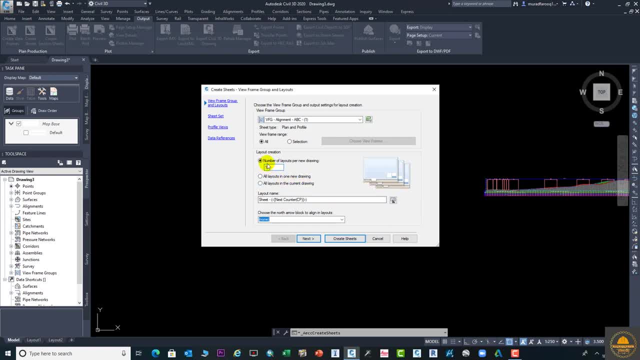 add. this is in the current drawing, which one is open. this is the important step we need. this is in the layout, which one is open already. here you need to select the layout name and here select the north. okay, select not and click on next. from here you can select this option. 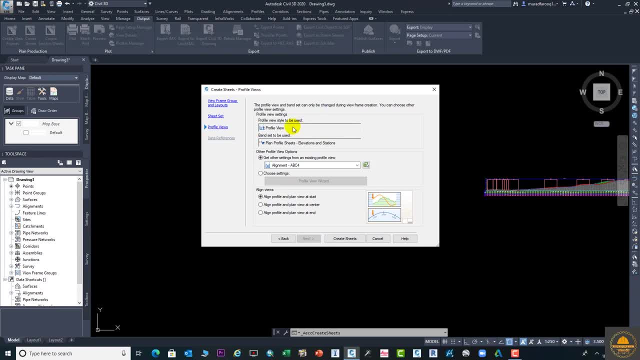 next this I meant, and here and then profile, and long you were, it start talking time. it will be start a line and so we start with, and it will be moved to the end, what we need to select the first one option to the start and create sheet. this one is open, the complete process. 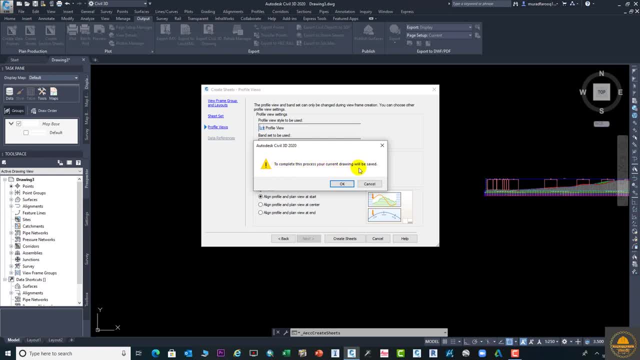 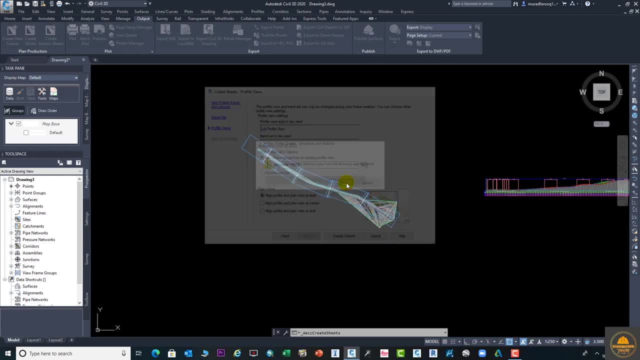 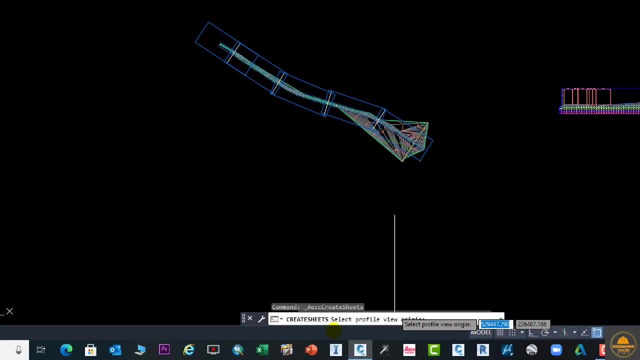 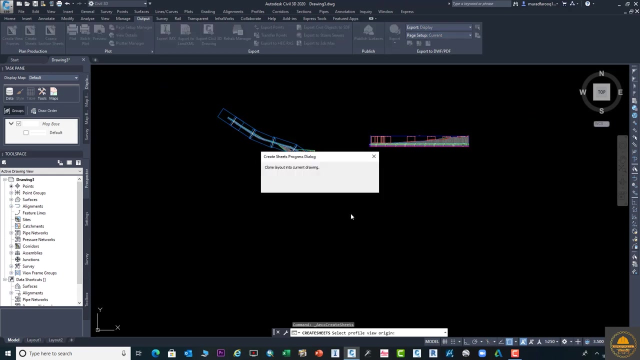 Your drawing will be saved if you click on the ok button. click ok, now you can see the option just profile view: click. click here. now you see your process start and your sheet is created here. you can see on the bottom: ok, we created our sheets here you can see. 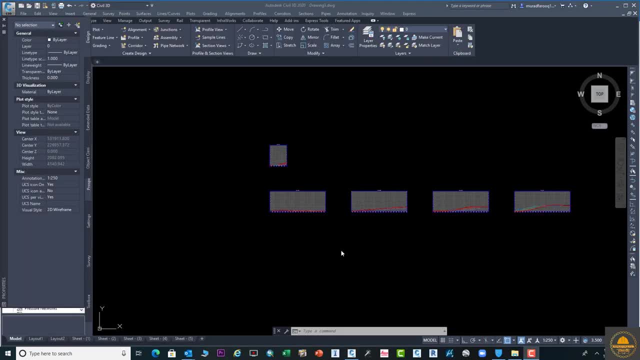 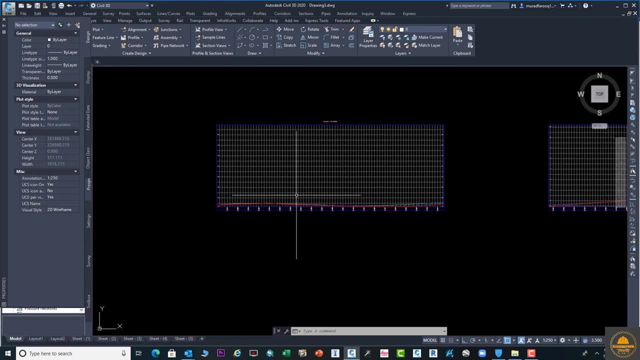 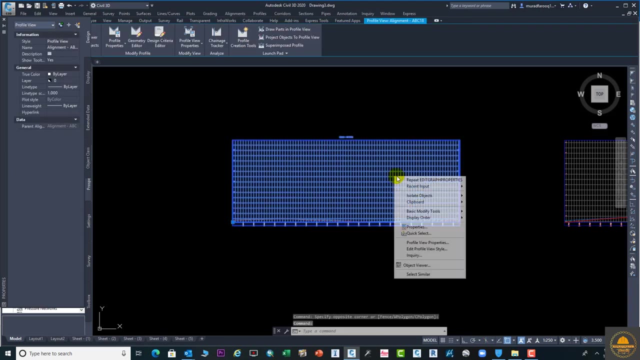 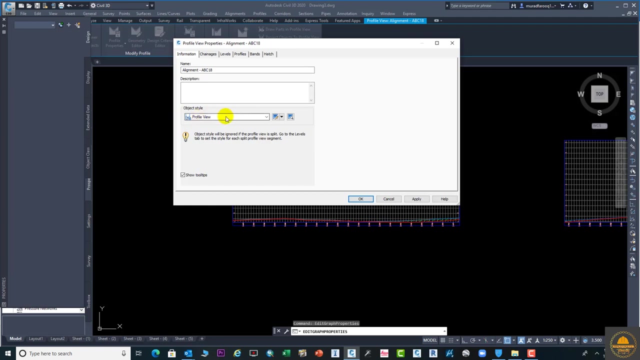 and graphs, everything we created very well. ok, now we need to do just some changing to make it clear. just select the graph and go to profile view properties. ok, from here you can change this information, Change this levels profile. you can change this automatic or user specified range. then 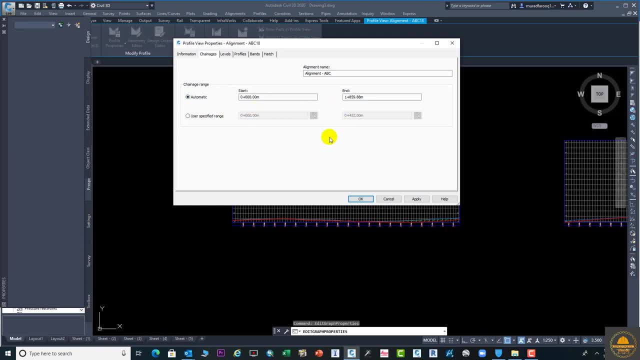 here you can enter and here you can check the levels. if the graph is not show, you can show from here, from the automatic and from this option. This is the band details. Ok, From here you can add the bands. suppose we need to add our bands here. this is just. 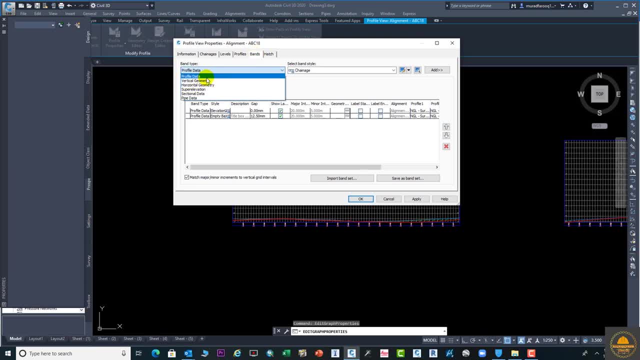 for the example from here: click on add and then again select any other and again click on add- ok, and then again click and add The last one, Ok, And apply, and ok. now you can see your band is created like your profile, which we created. 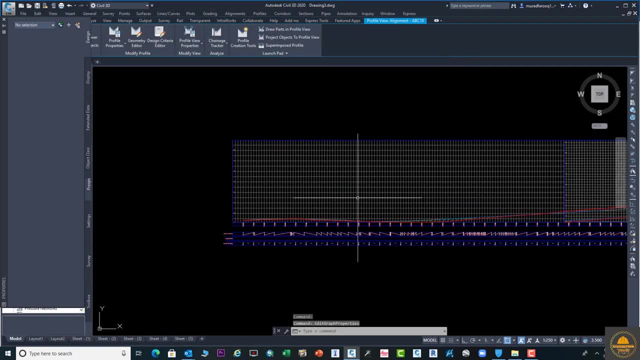 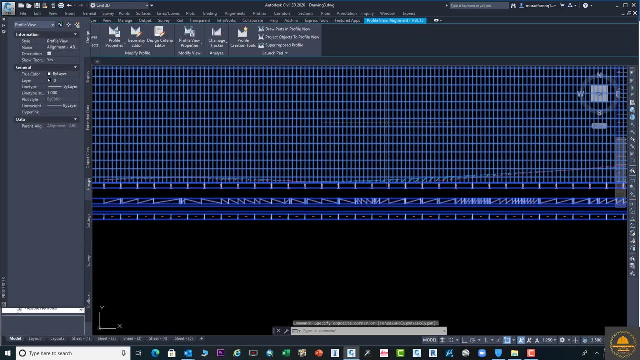 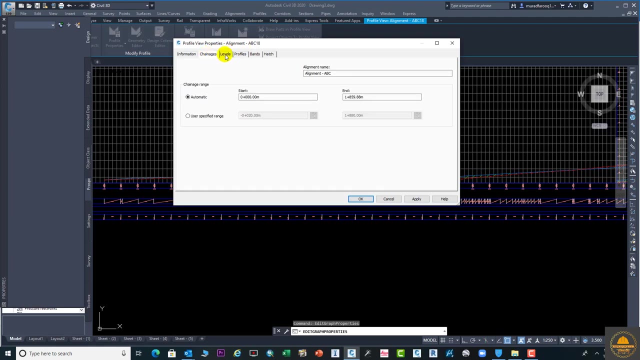 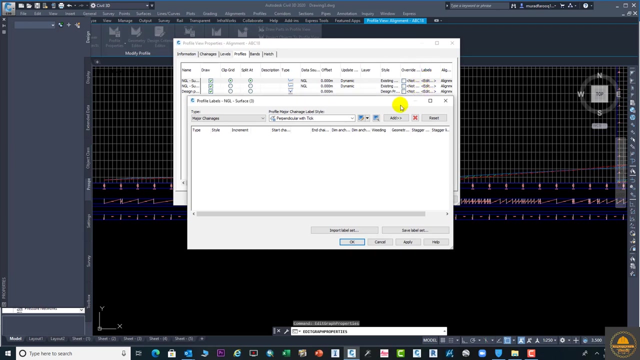 before. ok, now we need to go again to the setting profile view, set properties, and here, from here, we need to add some levels from the levels option. go here and add some levels from this option. add the measure is: add already. add this one: horizontal geometry. 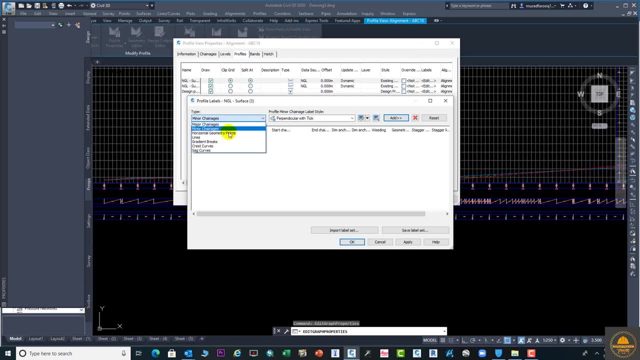 points and seg crest. you can add any kind of level on your profile, because there is no. any level is show on the sheets, apply and ok, Ok. Now you can see your level is set. Ok, Ok, Ok. 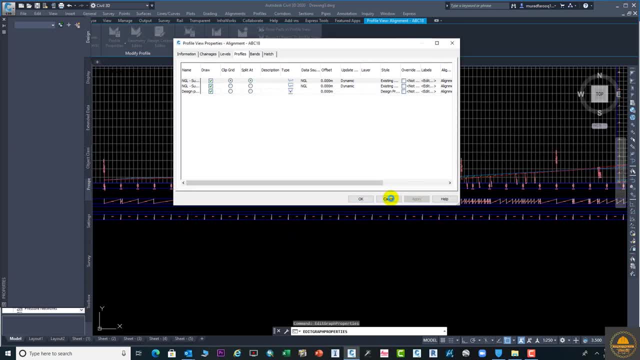 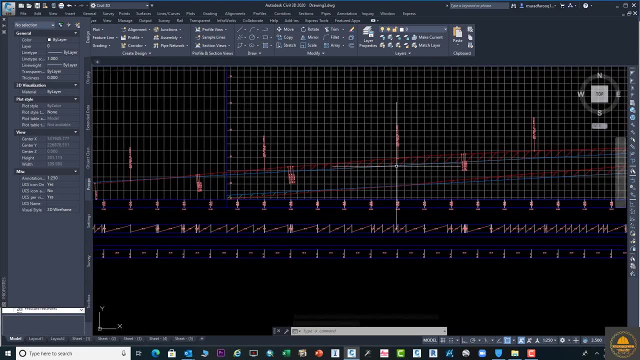 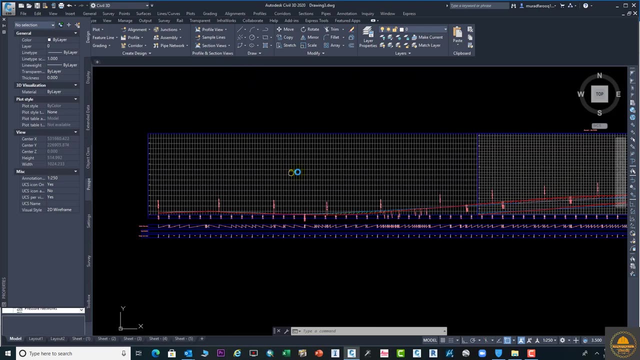 Ok, So now you can see your sheet is applied very clearly. you can see this is your sheets and everything is applied very clearly. ok, Here is our sheets. this one: this is sheet number 1, sheet number 2,, 3,, 4, 5, all sheet. 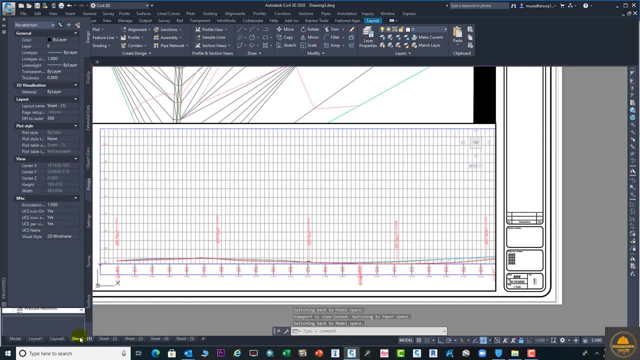 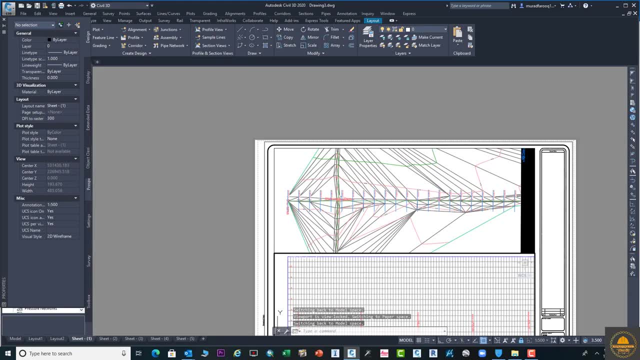 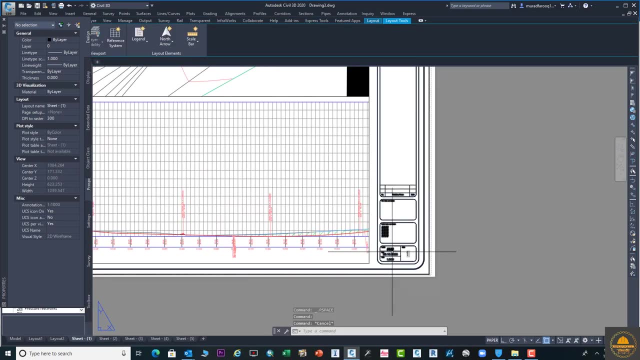 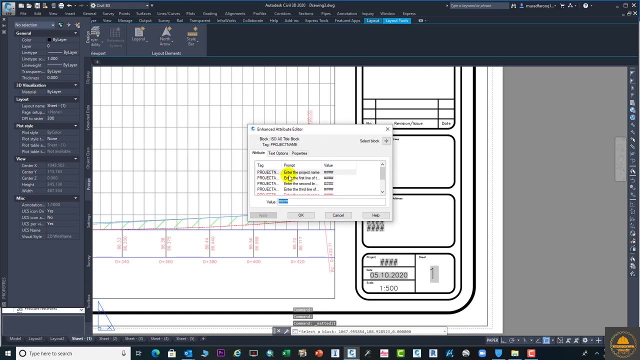 is created very clearly. This is your alignment And this one is Ok. Here is our sheet, Here is your and here you can add your company names. Just click here. You can add the project name details. who is the one to create this? any kind of information? 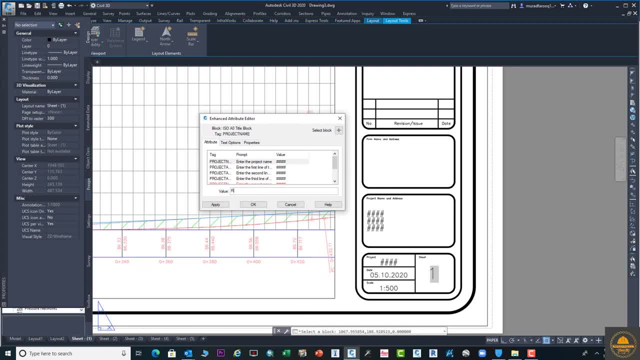 you can put here: suppose this is road project A, B, C, D and for the next you can give the next option like that and enter here: Here, delete this hashes and enter the name for the. okay, suppose this again, which you want to you, ABCD or any name you can give. okay, you can see on the right the 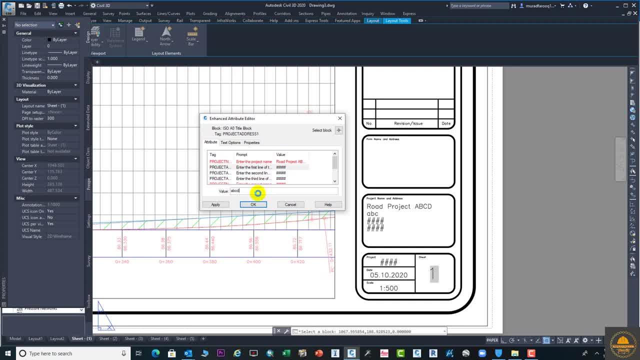 text is added in the works. okay, okay, and enter here again. xyz. anything you can enter is for your project requirement, idiot. project specification, names, codes, project cause. you can enter in this box: okay, here, project. and the other one is for the date. if you want to enter the date, you can enter the date. 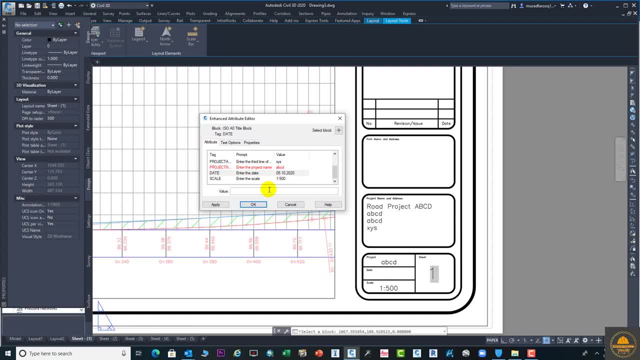 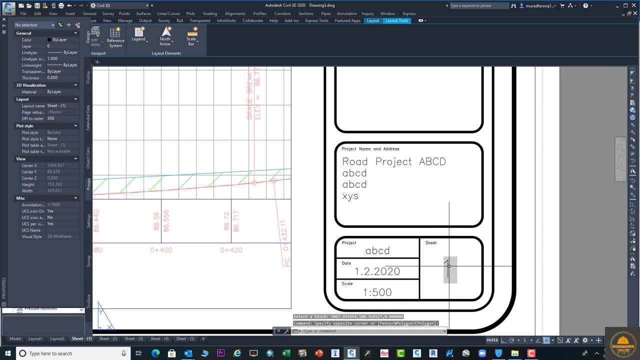 on which date you create the sheets. okay, and here in the last, you can enter the scale: on which scale. we already created this in 1 into 500 and we need to select this one and copy this one. select and control c: okay and paste here. here is your company name and address. you can enter your company name and address here.